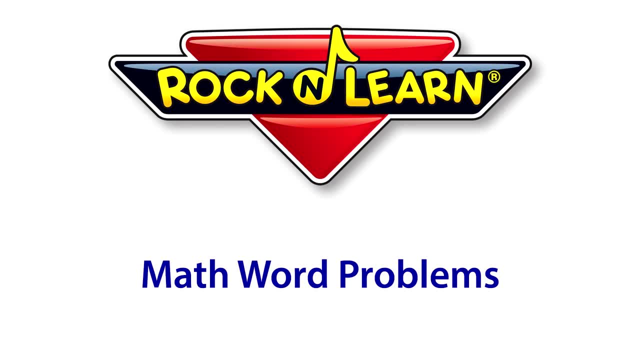 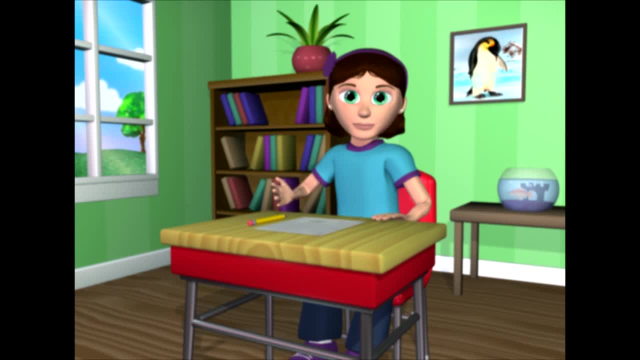 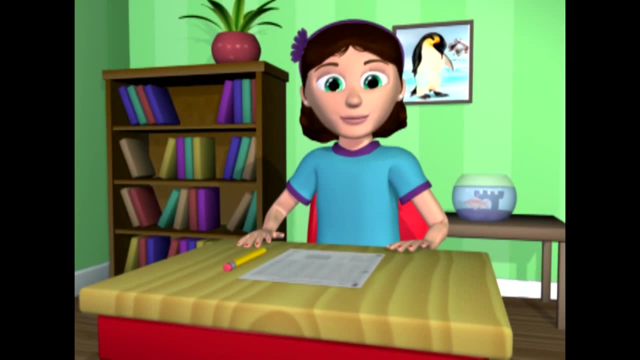 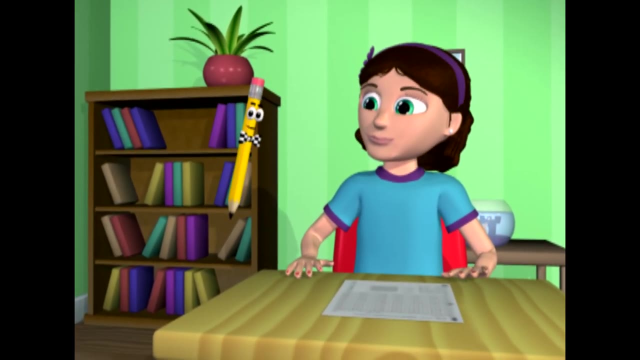 Rock and Learn. I have a math test coming up and I want to do really well on it. Here's this practice test to help me get better at taking math tests. I wish my friend Marco was here to help me. Did somebody call for me? 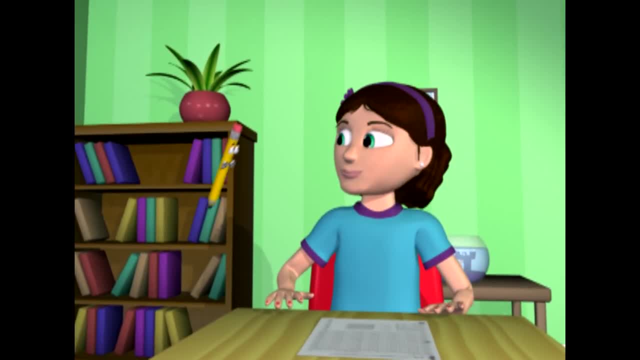 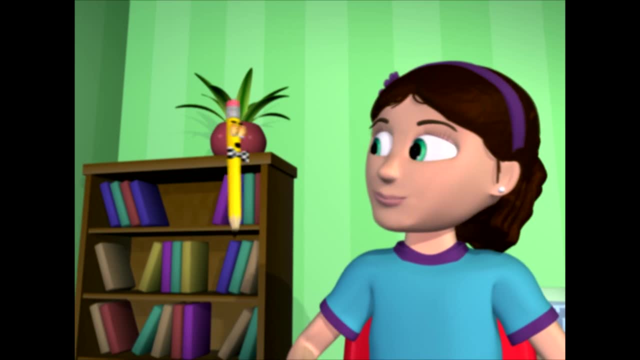 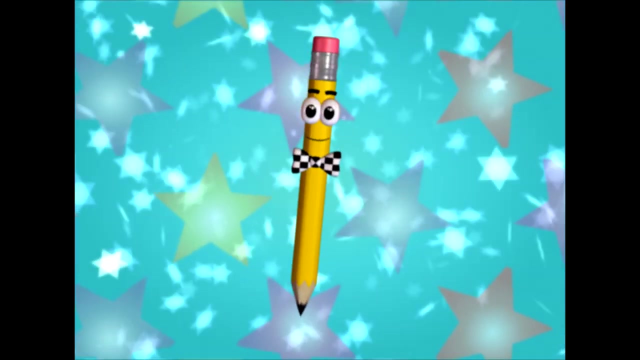 Marco, Can you help me with this practice math test? Well, let me check my schedule. Looks like I can pencil you in for a session right now. I'm Marco the Pencil. Take some tips from me To do the best on your test. here are some strategies. 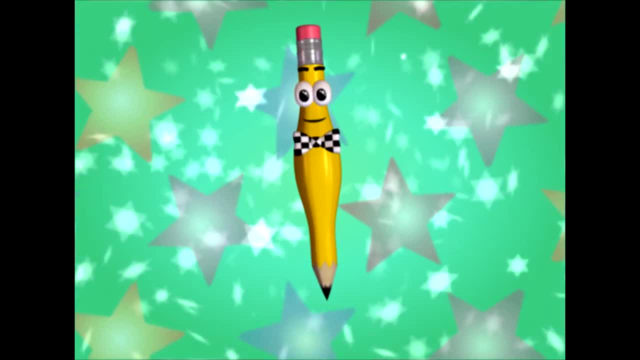 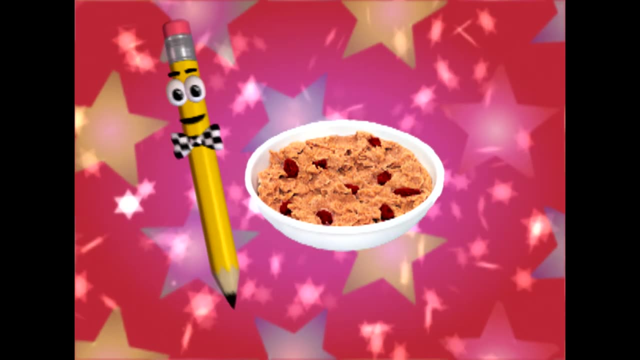 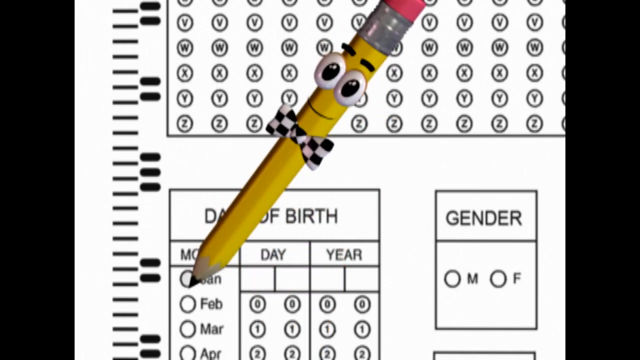 Take a big breath and let it go. Taking a test shows what you know. Eat something healthy, but don't overeat. When you mark your test, be sure to be really neat The night before. get a good night's rest. 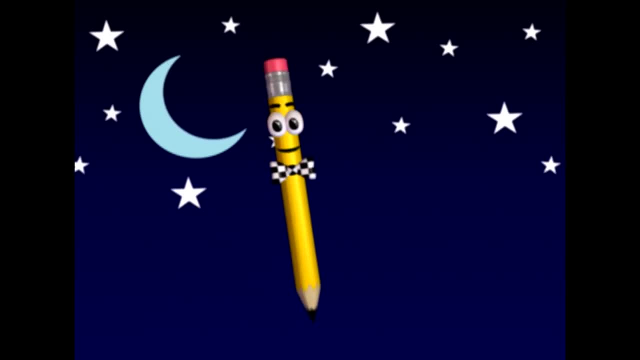 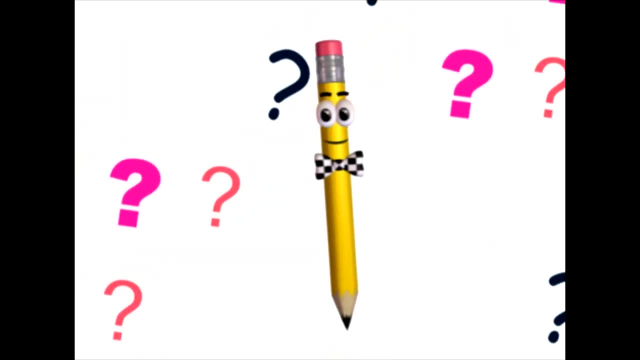 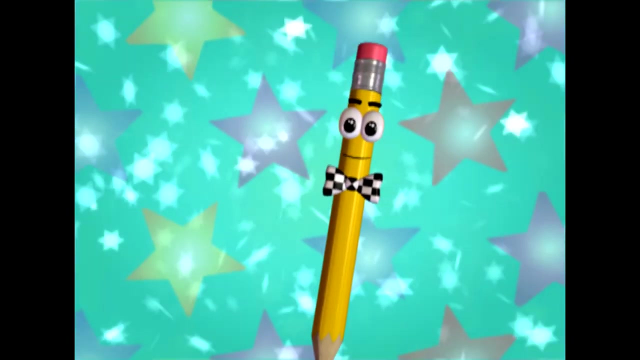 So you can do your best on the test. Read the questions carefully, Be sure to look for clues, Eliminate wrong answers before you choose. Stick around and I'll show you some more So you can make your very best. That's good, Yeah. 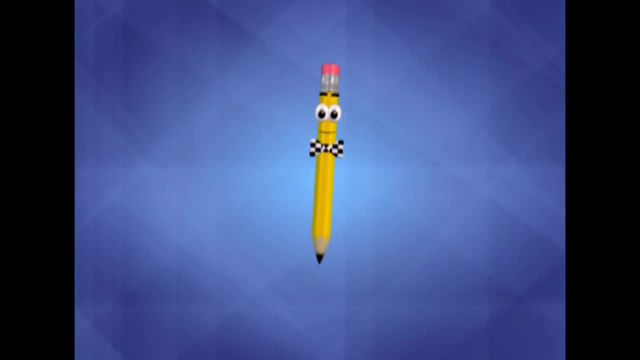 That's just what I need, Magnifico. I will show you some tips to help you do your best on a math test. Of course, the most important thing is to know your math, But I have some tips to help you make the most of what you know. 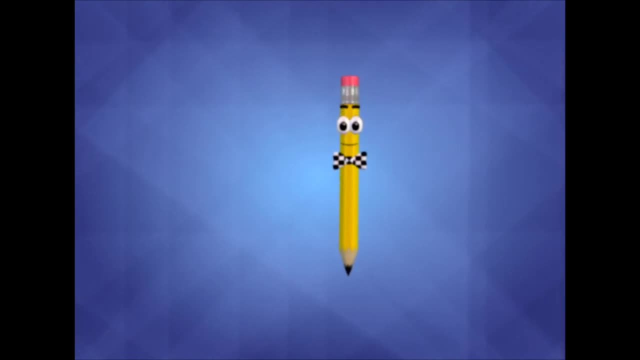 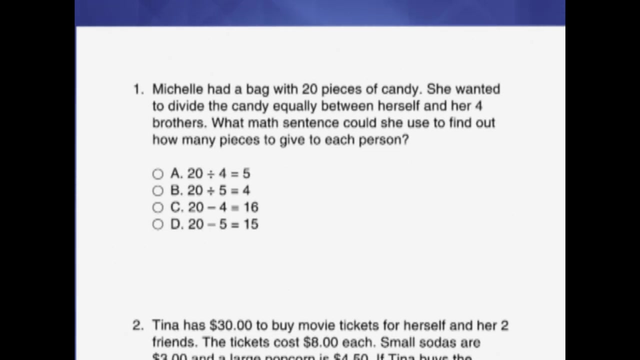 The first thing you should do is read the problem carefully. Let's look at an example. 1. Michelle had a bag with 20 pieces of candy. She wanted to divide the candy equally between herself and her four brothers. What math sentence could she use to find out how many pieces to give to each person? 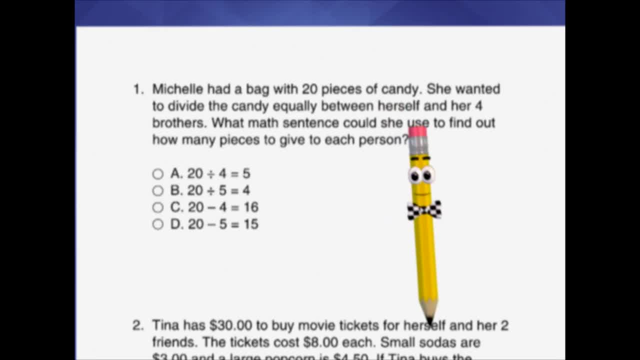 In this case we are looking for a math sentence. Let's see, We have 20 pieces of candy, herself and her four brothers. That gives us 5 people. Don't be tricked by the number 4. 1. 2., 3., 4., 5., 6., 7., 8., 9., 10., 11., 12., 12., 13., 14., 14., 15., 15.. 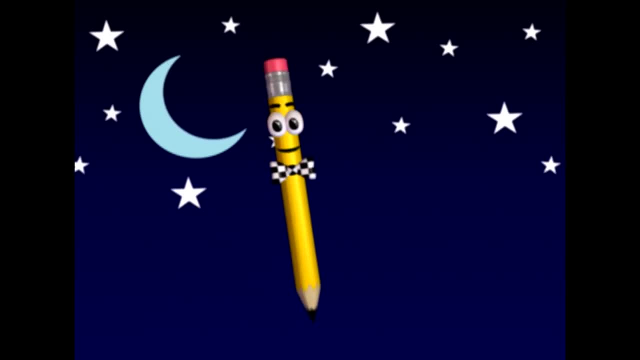 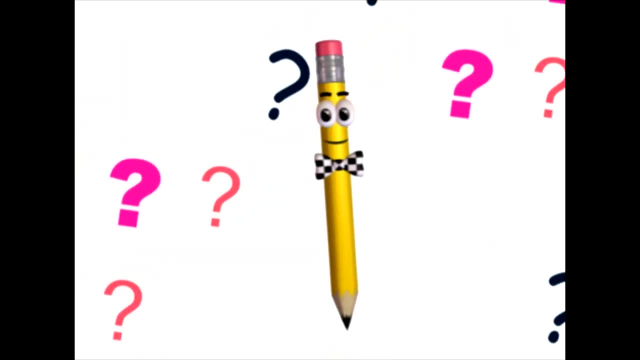 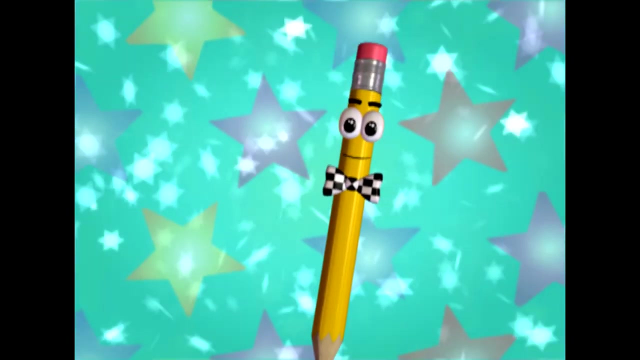 So you can do your best on the test. Read the questions carefully, Be sure to look for clues, Eliminate wrong answers before you choose. Stick around and I'll show you some more So you can make your very best. That's good, Yeah. 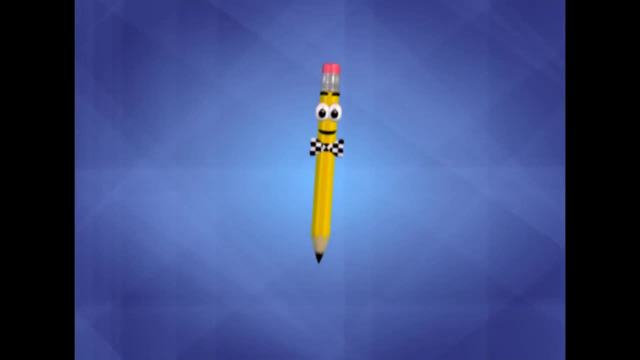 That's just what I need, Magnifico. I will show you some tips to help you do your best on a math test. Of course, the most important thing is to know your math, But I have some tips to help you make the most of what you know. 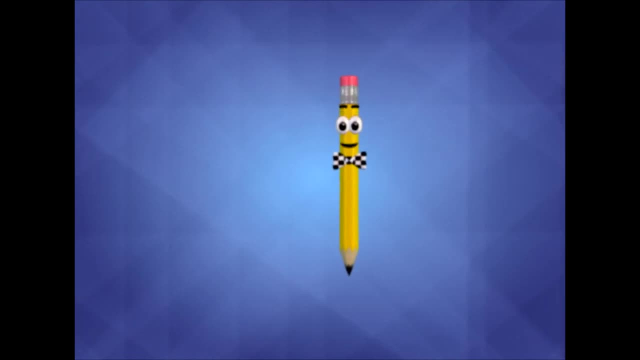 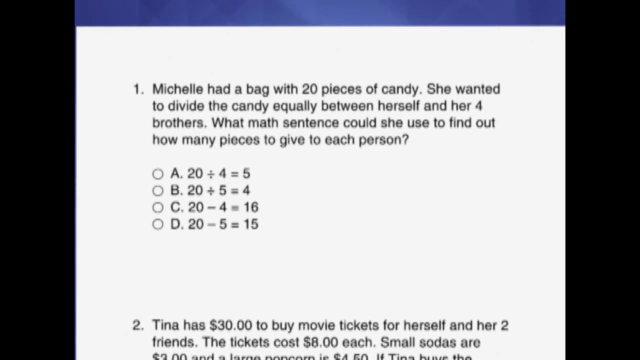 The first thing you should do is read the problem carefully. Let's look at an example. 1. Michelle had a bag with 20 pieces of candy. She wanted to divide the candy equally between herself and her four brothers. What math sentence could she use to find out how many pieces to give to each person? 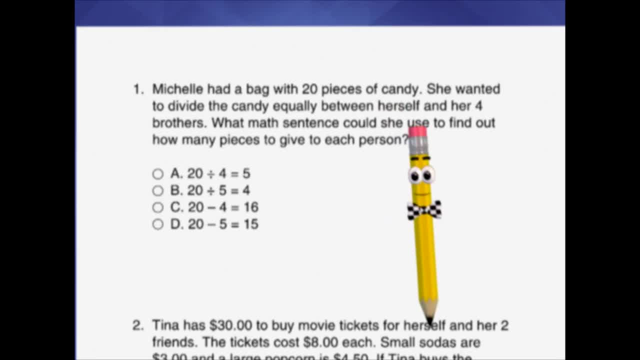 In this case we are looking for a math sentence. Let's see, We have 20 pieces of candy- herself and her four brothers. That gives us 5 people. Don't be tricked by the number 4. We need to read the problem. 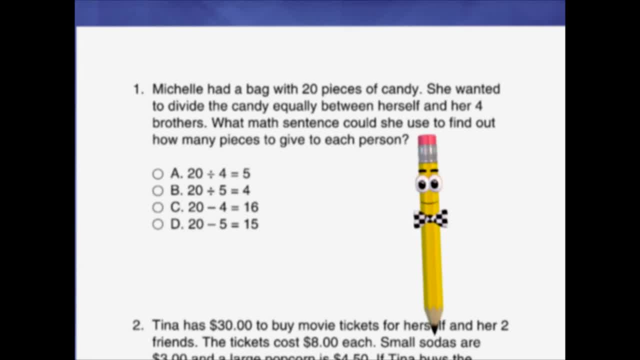 We need to read the whole problem, which tells us to add in, Michelle, and we want to divide the candy equally. so that tells us this is a division problem. Now let's consider the answers. A 20 divided by 4 equals 5.. 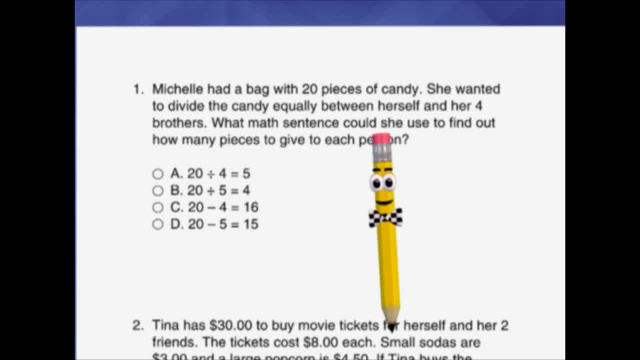 This one does not include Michelle when dividing the candy, so it is wrong. B 20 divided by 5 equals 4.. This one does not include Michelle when dividing the candy, so it is wrong. That looks right: 20 pieces of candy divided by 5 people would give each person 4 pieces of candy. 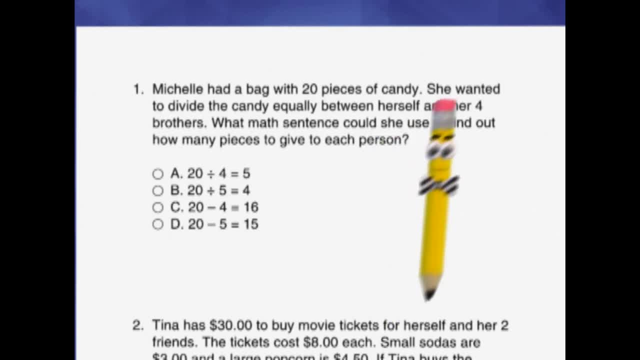 But let's read all of the answers just to be sure. C 20 minus 4 equals 16.. While this equation is correct, it does not answer our problem at all. D 20 minus 5 equals 15.. This one won't work either. 15., 16., 16., 16., 16., 16., 17., 17., 18., 19., 20., 21., 22., 23., 24., 25., 26.. 27., 28., 29., 30., 31., 32., 33., 34., 35., 36., 37., 38., 39., 39., 39., 40., 40.. 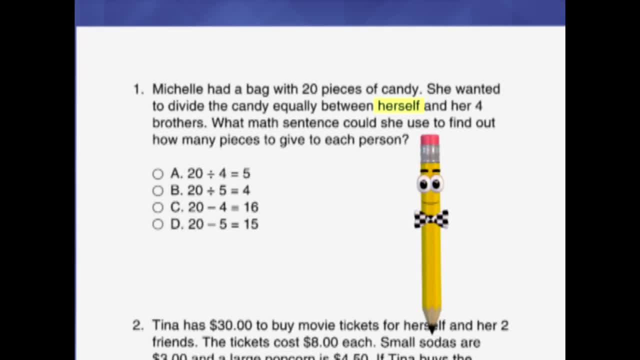 41., 41., 42., 43., 44., 44., 44., 45., 46., 46., 47., 47., 48., 49., 49., 50.. This one does not include Michelle when dividing the candy. 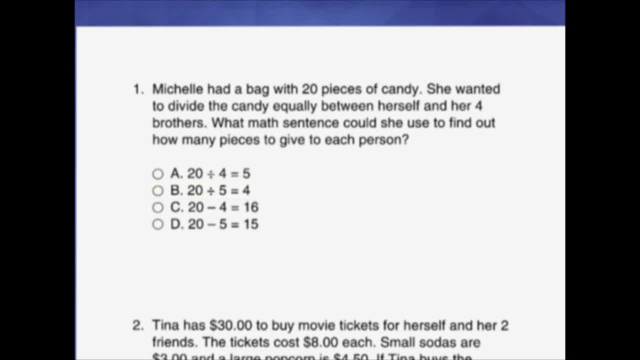 So it is wrong. B 20 divided by 5 equals 4.. That looks right. 20 pieces of candy divided by 5 people would give each person 4 pieces of candy. But let's read all of the answers just to be sure. 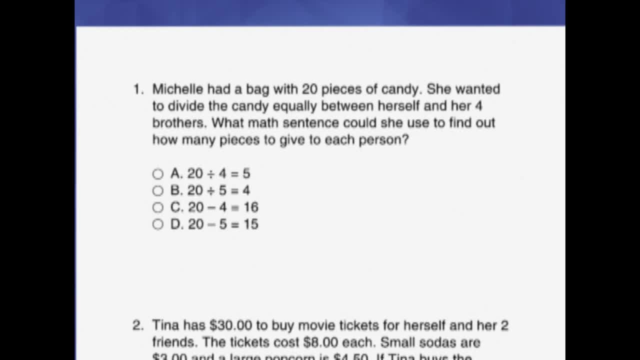 C: 20 minus 4 equals 16.. While this equation is correct, it does not answer our problem at all. D: 20 minus 5 equals 15.. C: 20 by 15 equals 16.. This one won't work either. 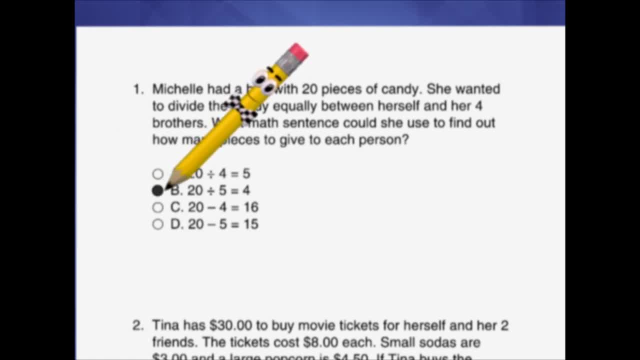 So the answer is: B 20 divided by 5 equals 4.. Notice how I am careful to fill in in the circle completely and neatly絴tał in the lines. You should do that too, So all of your correct answers get counted. 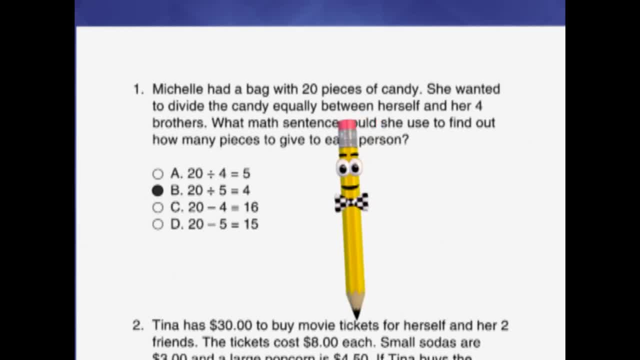 On some tests you may have to fill in your answers on a separate sheet, But on this test we are supporting you to try. and Garrett's questions to the end, the one that is actually quite effective. See you in the next one. Cheese alluded to it. 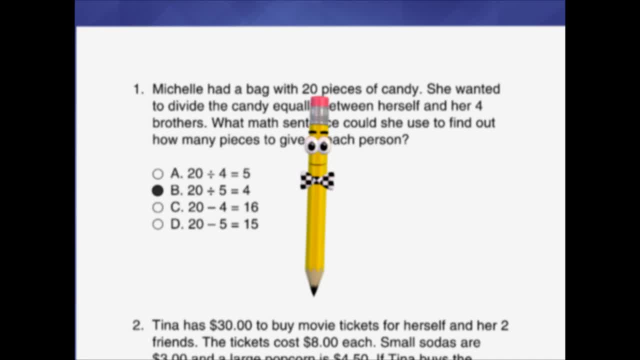 Bye, Bye, Bye, Bye, Goodbye, Bye, Bye, Bye, Bye. supposed to fill in the answers in the booklet. What happens if I get out of the lines when I mark my answers? Be sure to erase any stray marks completely. 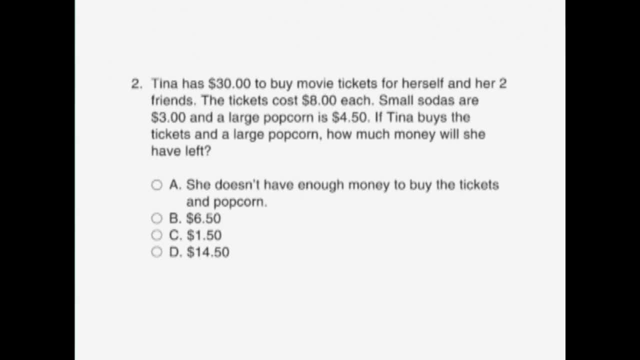 Let's do another one. Tina has thirty dollars to buy movie tickets for herself and her two friends. The tickets cost eight dollars each, Small sodas are three dollars and a large popcorn is four dollars and fifty cents. If Tina buys the tickets and a large popcorn, how much money will she have left? 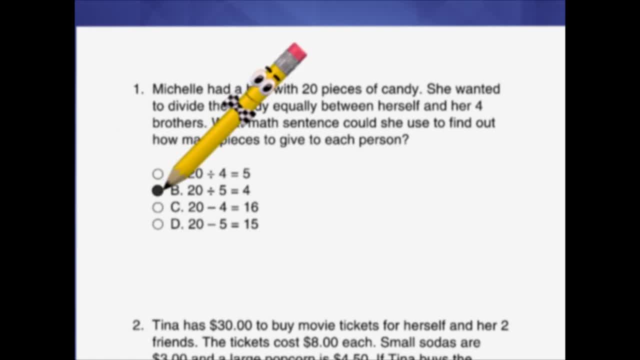 So the answer is: B 20 divided by 5 equals 4.. Notice how I am careful to fill in the circle completely and neatly, staying in the lines. You should do that too, so all of your correct answers get counted. 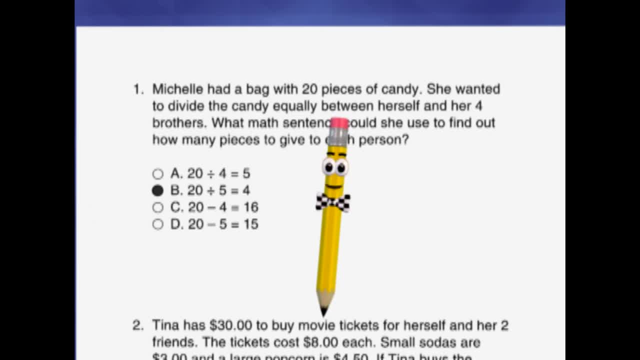 On some tests you may have to fill in your answers on a separate sheet, But on this test we are supposed to fill in the answers in the booklet. What happens if I get out of the lines when I mark my answers? Be sure to erase any stray marks completely. 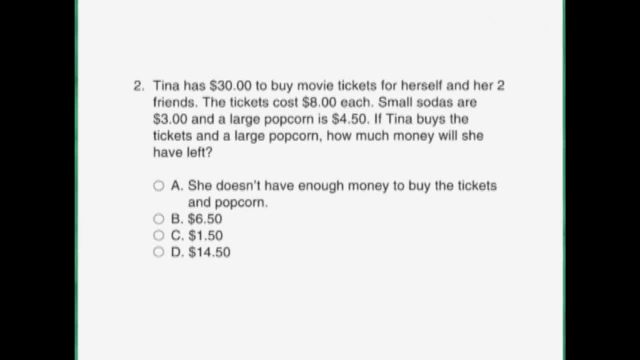 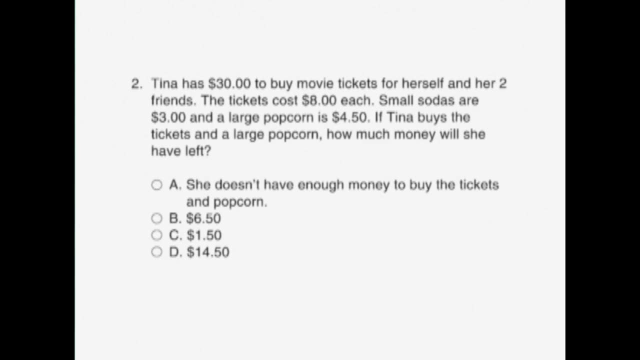 Let's do another one. 2. Tina has $30 to buy movie tickets for herself and her two friends. The tickets cost $8 each, Small sodas are $3, and a large popcorn is $4.50.. If Tina buys the tickets and a large popcorn, 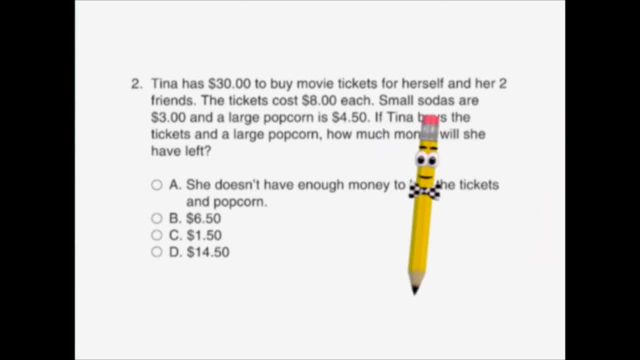 how much money will she have left? So we need the price of the tickets and how many tickets. we need the price of the popcorn and how much money Tina had in the beginning. Hmm, we don't need the price of the soda. 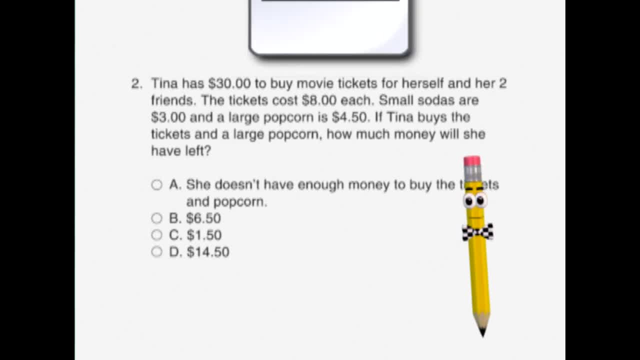 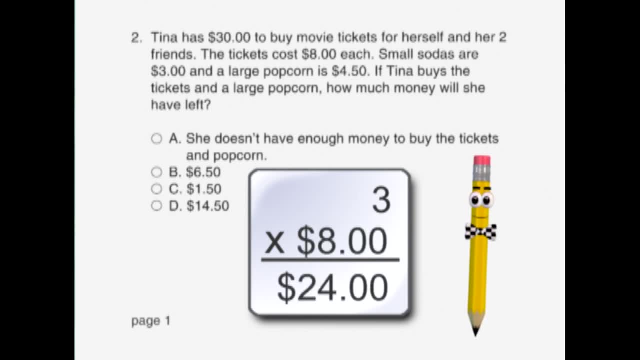 You're right, But we do need to know how much Tina would be spending. so 3 tickets times $8 each equals $24.. Add in $4.50 for the popcorn to bring us to $28.50.. But the question is: 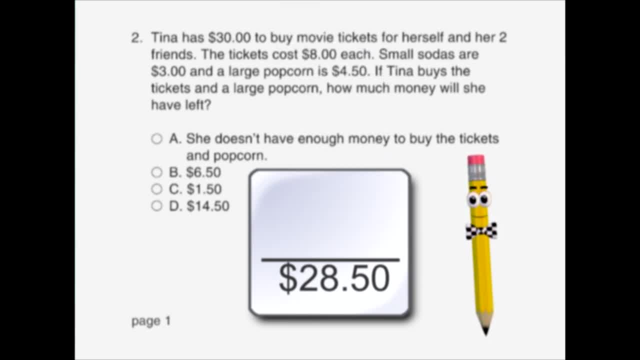 how much money will Tina have left out of $30? $30 minus $28.50 leaves $1.50.. Let's see if one of the answers matches that A She doesn't have enough money to buy the tickets and popcorn. 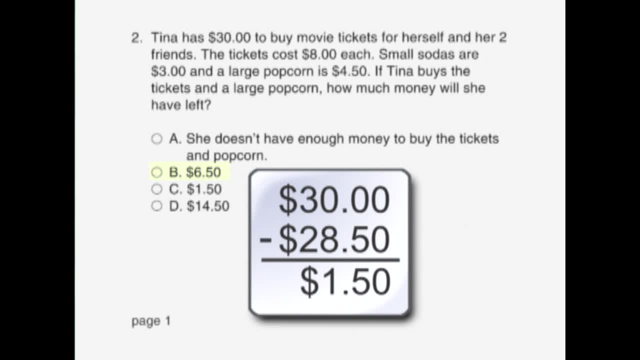 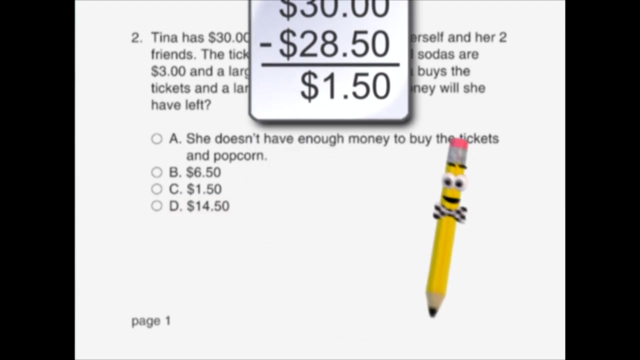 That's not true. B- $6.50.. That's too much. C- $1.50.. There's our answer, And the last one, D- $14.50, is too much as well. So the answer is C- $1.50. 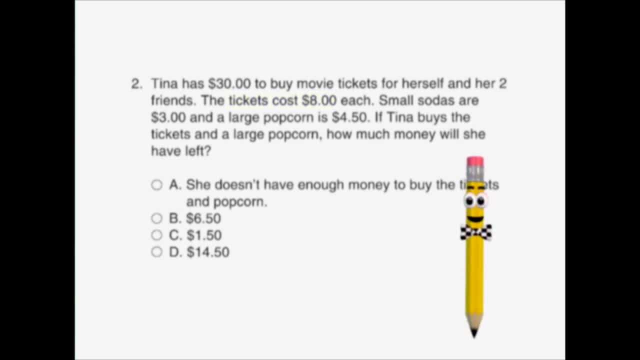 So we need the price of the tickets and how many tickets. we need the price of the popcorn and how much money Tina had in the beginning. We don't need the price of the soda, you're right, but we do need to know how much, Tina. 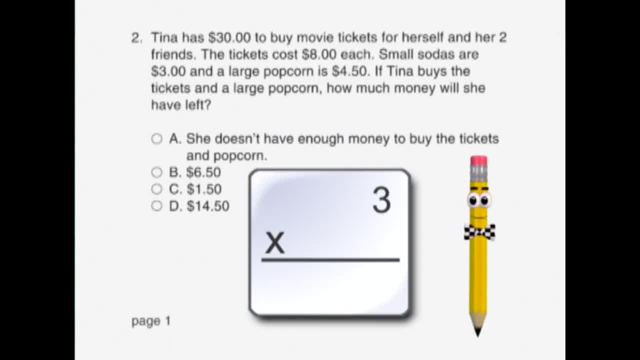 would be spending. So three tickets times eight dollars each equals twenty-four dollars. Add in four dollars and fifty cents for the popcorn to bring us to twenty-eight dollars and fifty cents. But the question is, how much money will Tina have left out of thirty dollars? 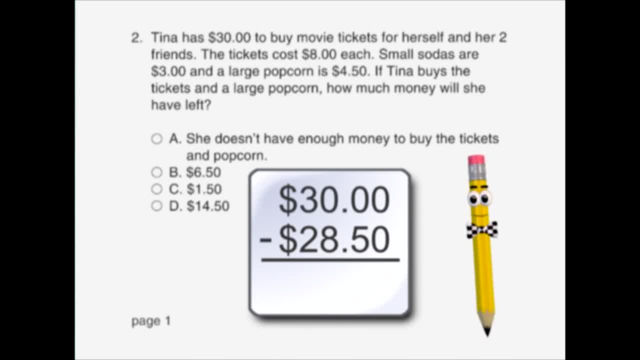 Thirty dollars minus twenty-eight dollars and fifty cents leaves one dollar and fifty cents. Let's see if one of the answers matches that: A- She doesn't have enough money to buy the tickets and popcorn. B- She doesn't have enough money to buy the tickets and popcorn. 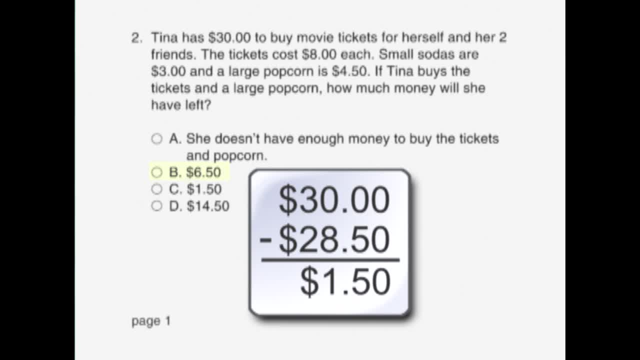 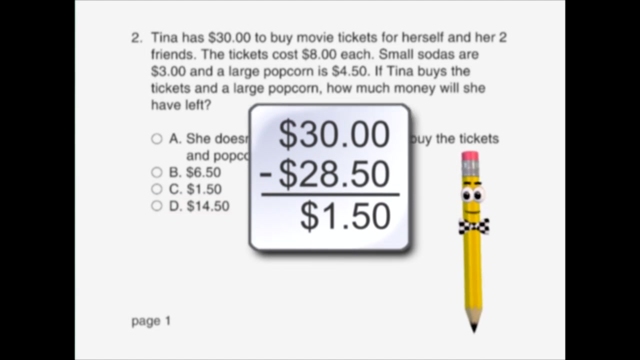 That's not true. B- Six dollars and fifty cents, That's too much. C- One dollar and fifty cents. There's our answer, And the last one, D- Fourteen dollars and fifty cents- is too much as well. So the answer is C- One dollar and fifty cents. 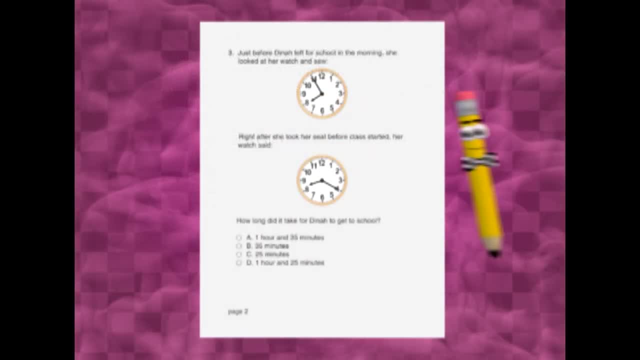 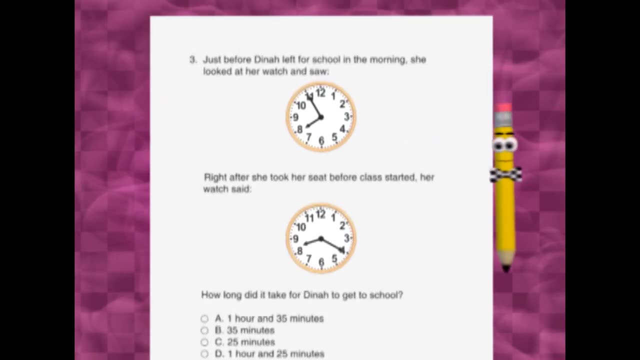 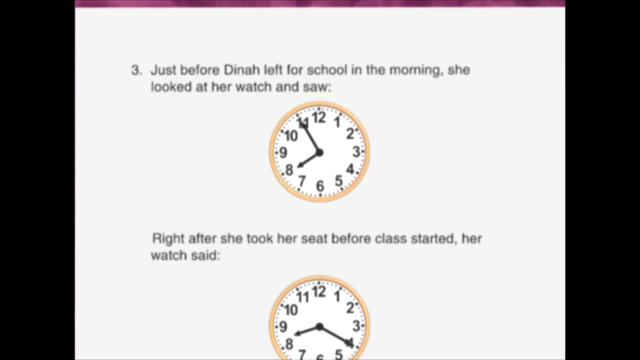 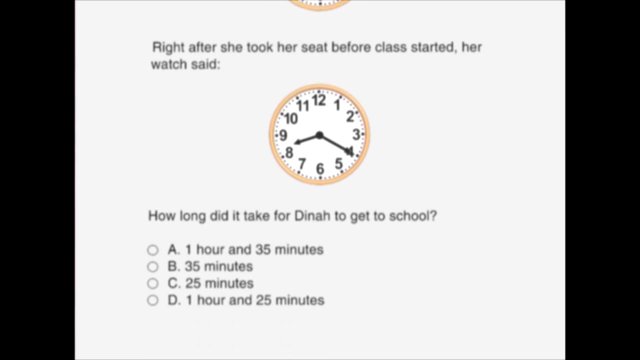 With some problems. it is helpful to draw a picture or diagram. Let's look at some examples. 3. Just before Dinah left for school in the morning, she looked at her watch and saw. Right after she took her seat before class started, her watch said: 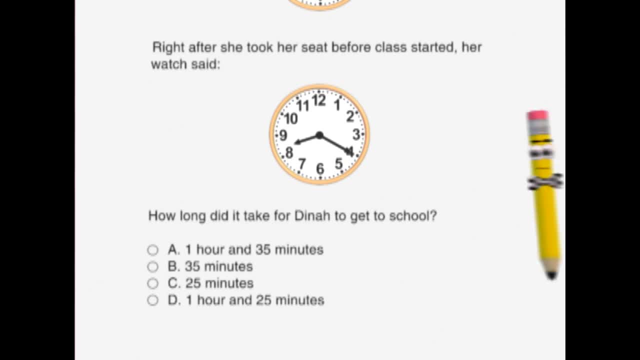 How long did it take for Dinah to get to school? 5 minutes brings us to 8 o'clock, 8.05, 8.10,, 8.15, 8.20.. That's 5, 10, 15,, 20,, 25 minutes. 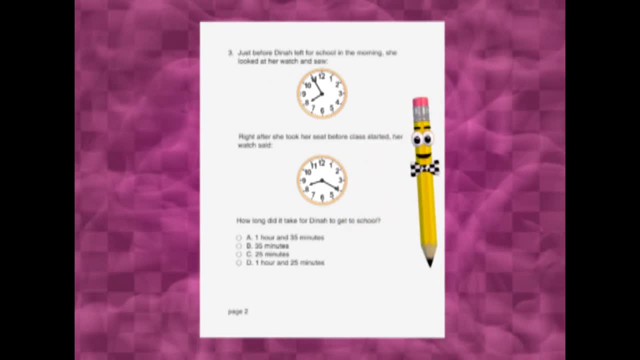 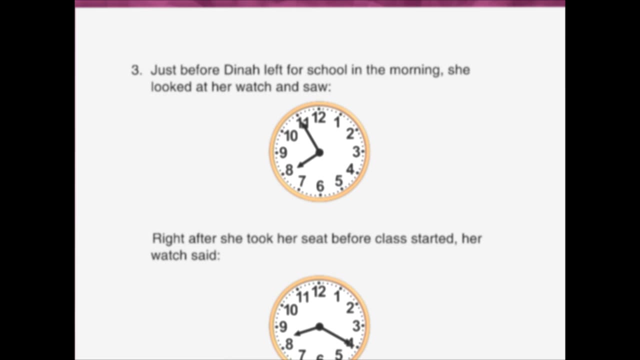 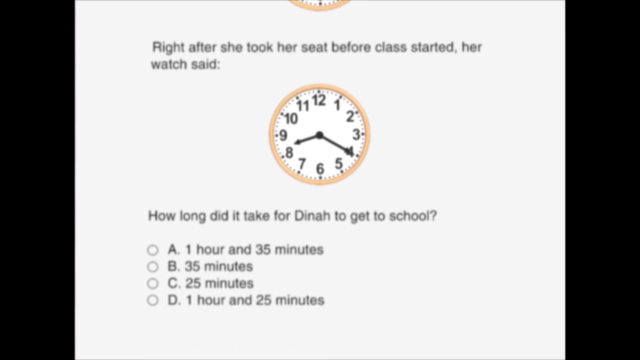 With some problems. it is helpful to draw a picture or diagram. Let's look at some examples. 3. Just before Dinah left for school in the morning, she looked at her watch and saw $7.55.. Right after she took her seat before class started. 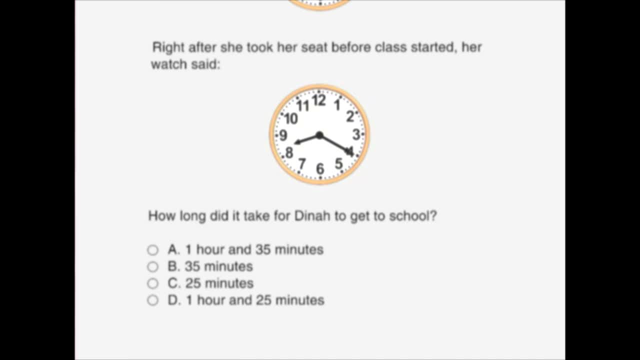 her watch said $8.20.. How long did it take for Dinah to get to school? 5 minutes brings us to 8 o'clock: 8.05,, 8.10,, 8.15,, 8.20., 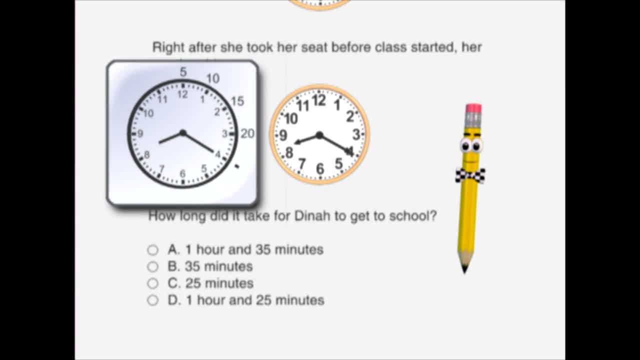 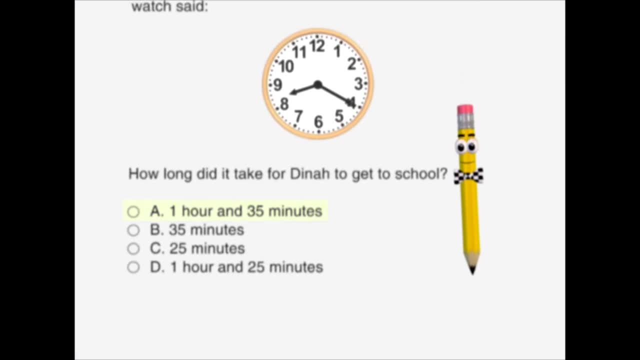 That's 5,, 10,, 15,, 20,, 25 minutes. Which answer matches that? Let's see: A: 1 hour and 35 minutes. No B: 35 minutes, Not that one. C- 25 minutes. 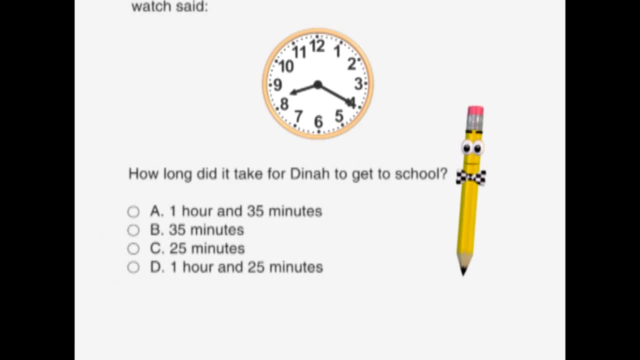 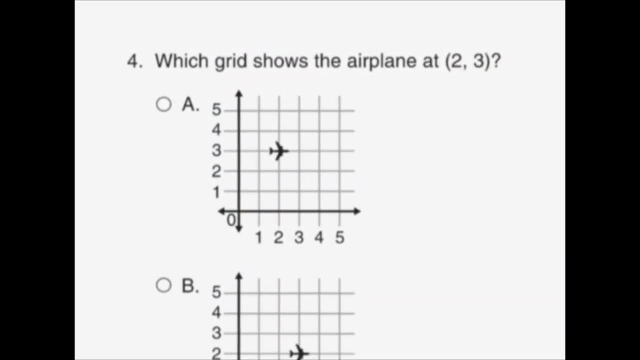 That matches our answer. And the last answer, D, 1 hour and 25 minutes, is much too long. We'll mark C: 25 minutes. 4.. Which grid shows the airplane at 2, 3?? To solve this problem, we need to know that the first number is the one that goes across or horizontally. 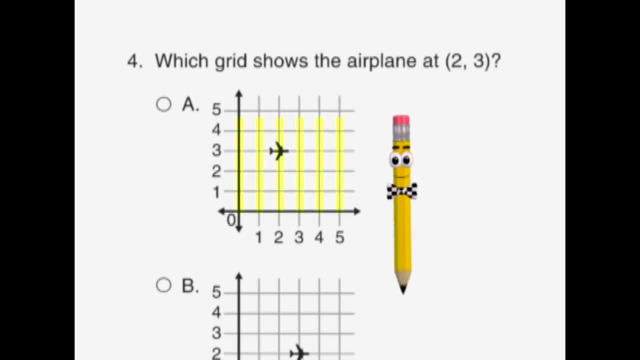 and the second number is the one that goes up and down or vertically. For graph A we get 2 and 3.. Graph A shows the ordered pair, 2, 3.. But go ahead and look at the rest of them. 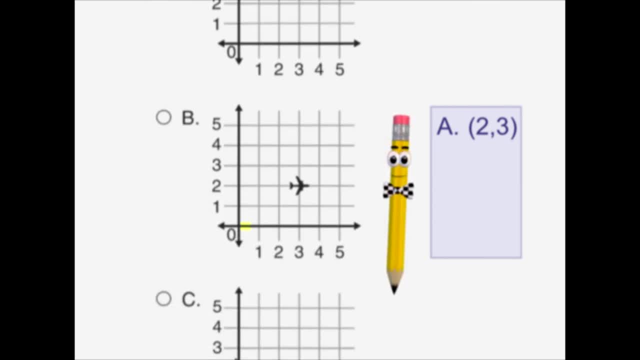 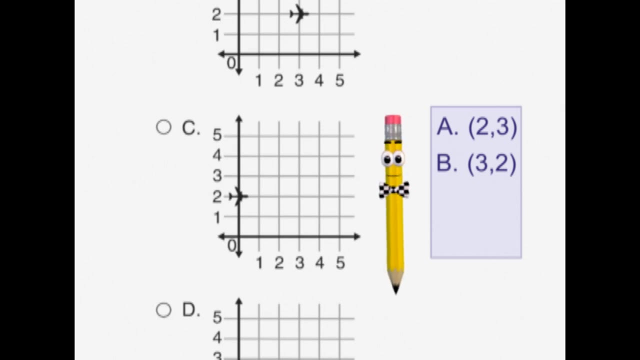 Good idea. For graph B. we get 3 and 2.. Graph B shows the ordered pair 3, 2.. Close, but not quite right. In graph C the plane is directly above the zero, So our ordered pair is: 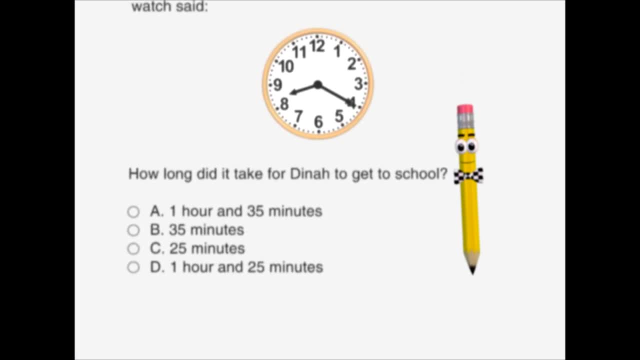 Which answer matches that. Let's see: A- 1 hour and 35 minutes. No, B- 35 minutes, Not that one. C- 25 minutes. That matches our answer And the last answer, D- 1 hour and 25 minutes, is much too long. 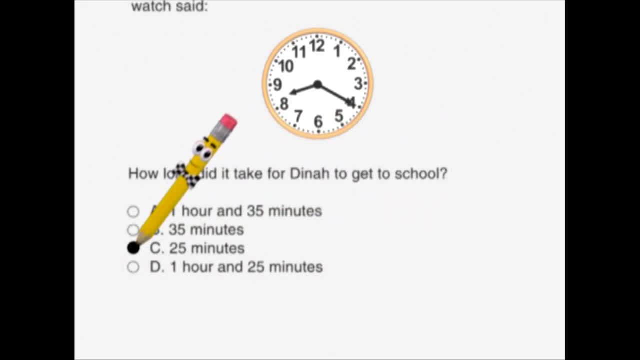 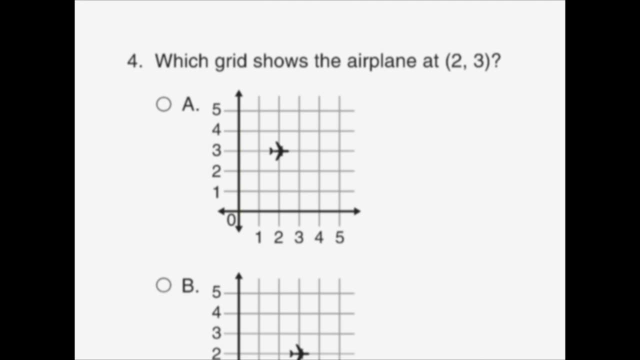 We'll mark C 25 minutes. 4. Which grid shows the airplane at 2, 3?? 1. To solve this problem, we need to know that the first number is the one that goes across, or horizontally, and the second number is the one that goes up and down, or vertically. 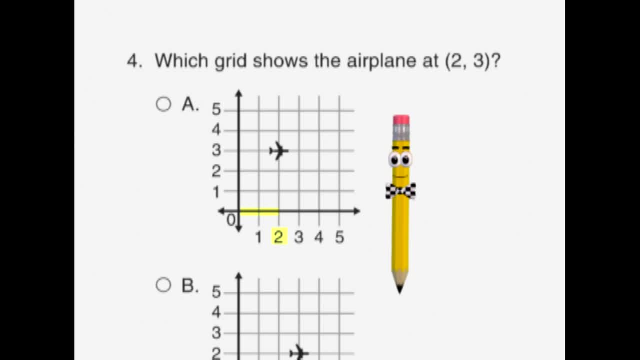 For graph A, we get 2 and 3.. Graph A shows the ordered pair: 2, 3.. But go ahead and look at the rest of them, Good idea. For graph B, we get 2 and 3.. 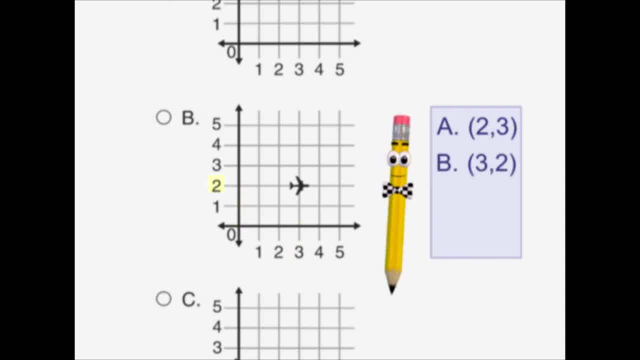 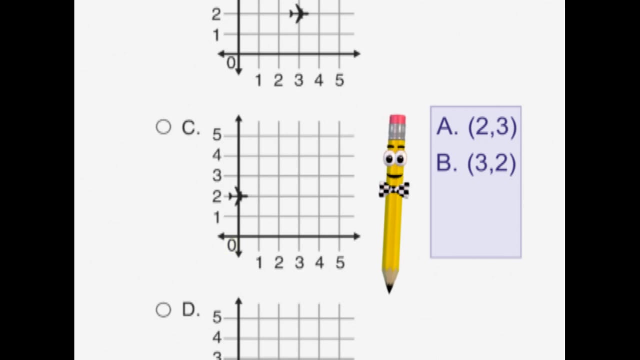 3 and 2.. Graph B shows the ordered pair 3, 2.. Close, but not quite right. In graph C the plane is directly above the zero, So our ordered pair is 0 and 2.. Graph C shows the ordered pair 0, 2.. That's not right. 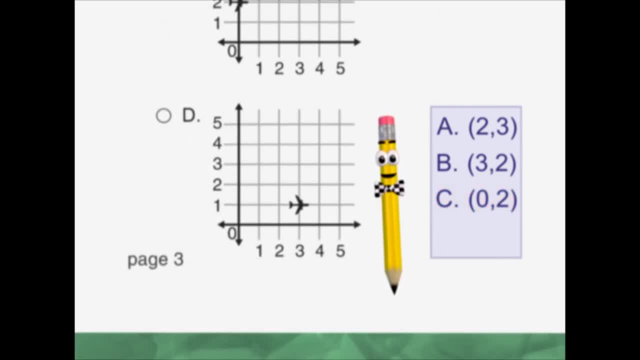 Graph B shows the ordered pair 2, 0 and 2.. That's not right. Graph B shows the ordered pair 2, 3 and 2.. That's not right. For graph D. we get three and one. Graph D shows the ordered pair three: one. 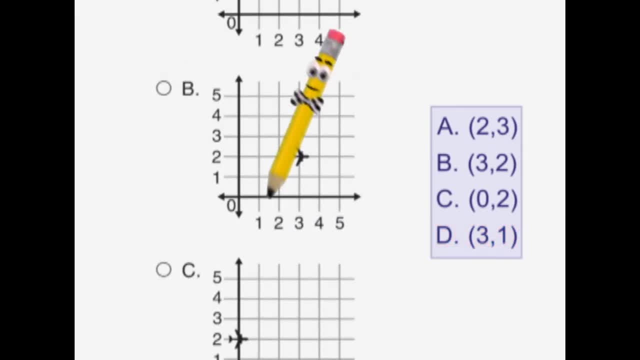 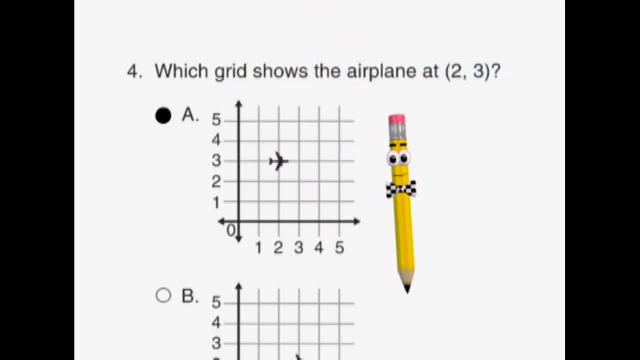 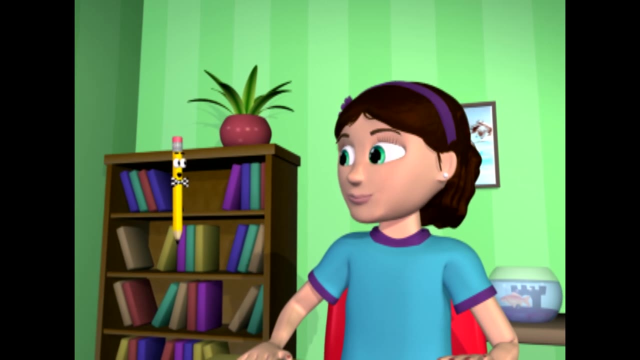 Not this one either. So the correct answer is A Graph A shows the plane at two, three. Hey, Marco. what do jokes and pencils have in common? I'm not sure They're no good without a point. That is a good point. 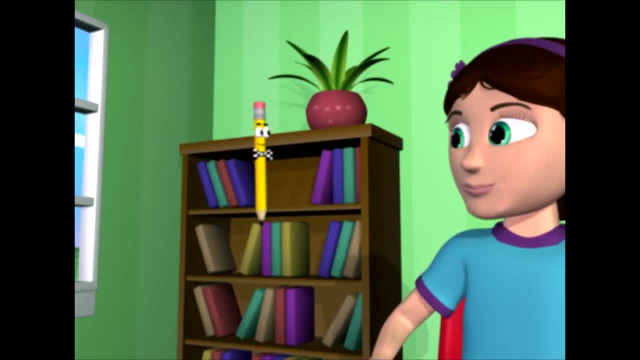 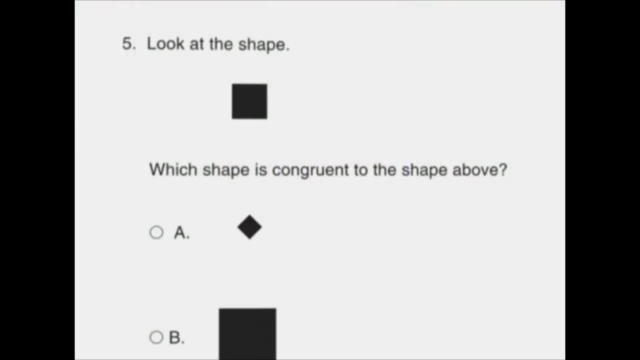 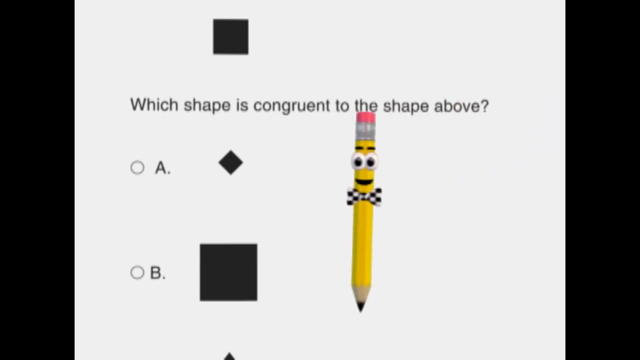 Be sure you have your pencil sharpened before you start the test. Now let's do some more problems with pictures and diagrams. Five: Look at the shape. Which shape is congruent to the shape above? Remember, congruent means the same size and shape. 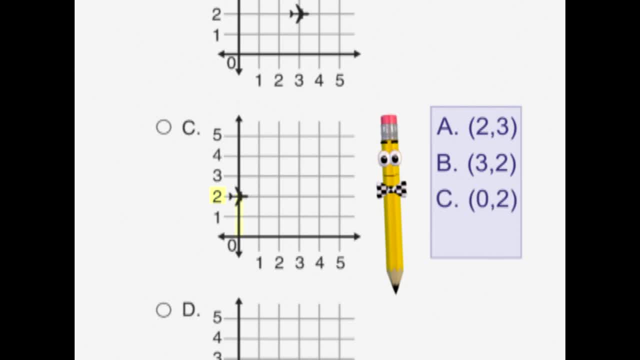 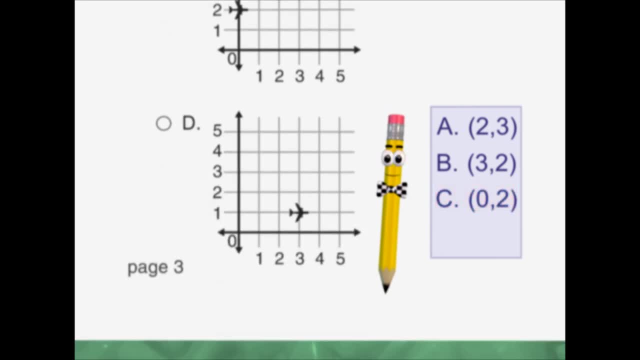 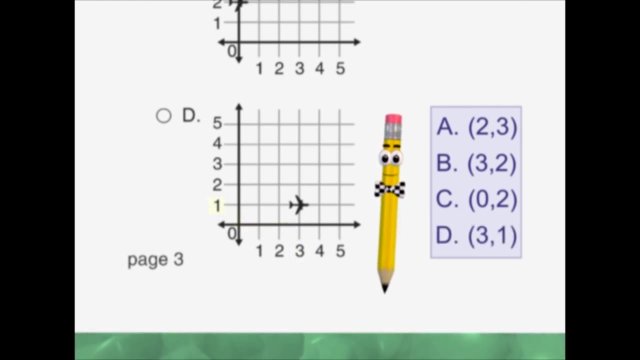 0 and 2.. Graph C shows the ordered pair 0, 2.. That's not right. For graph D we get 3 and 1.. Graph D shows the ordered pair 3, 1.. Not this one either. 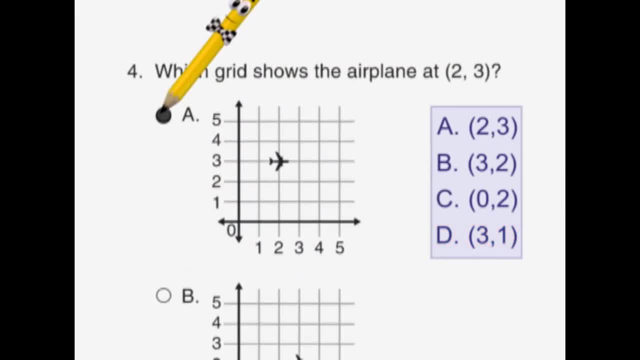 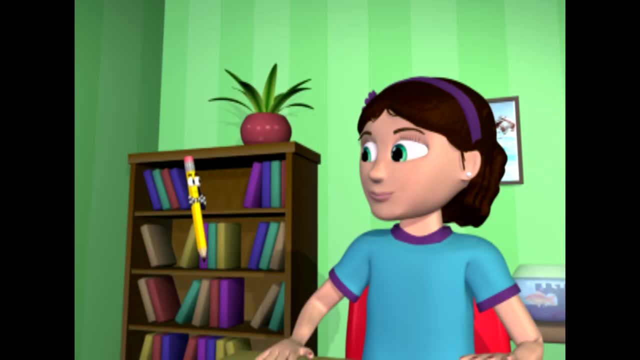 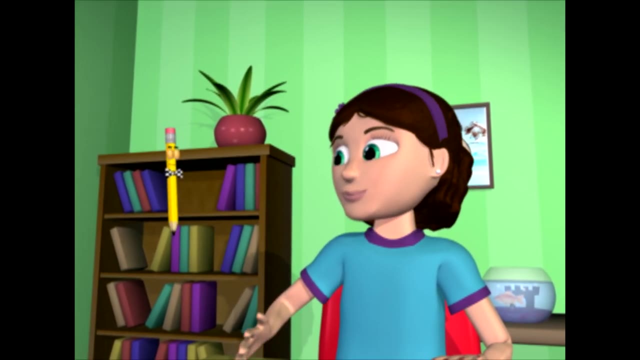 So the correct answer is: A Graph A shows the plane at 2, 3.. That's correct, Hey, Marco. What do jokes and pencils have in common? I'm not sure They're no good without a point. 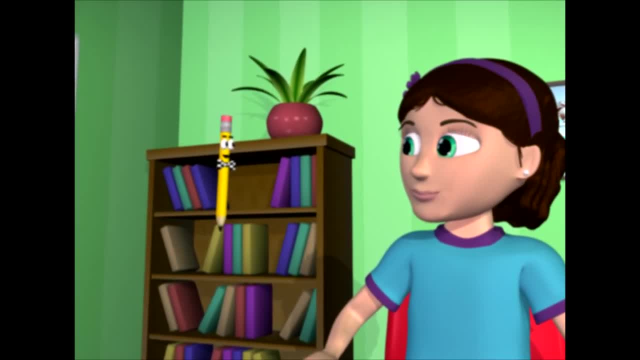 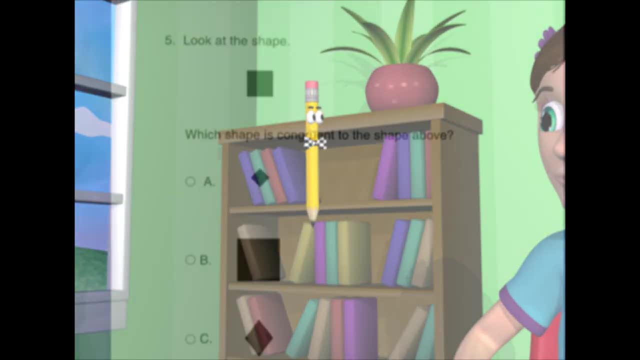 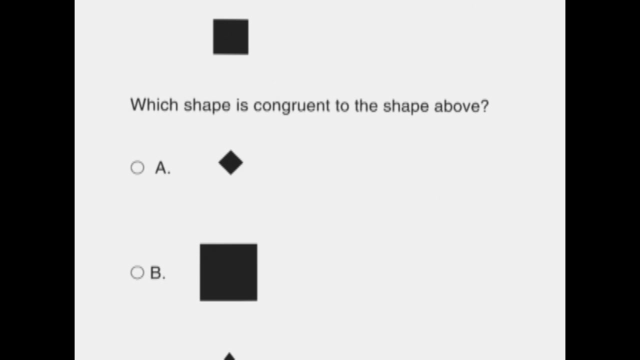 That is a good point. Be sure you have your pencil sharpened before you start the test. Now let's do some more problems with pictures and diagrams. 5. Look at the shape. Which shape is congruent to the shape above? 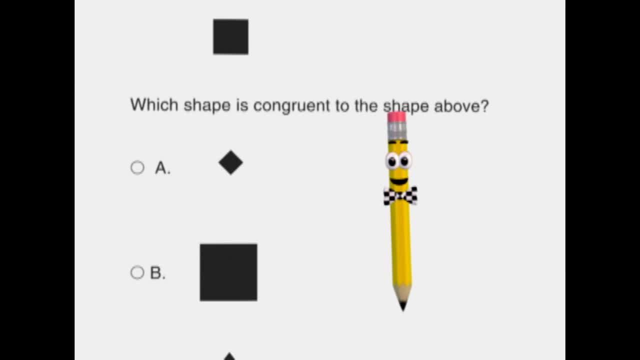 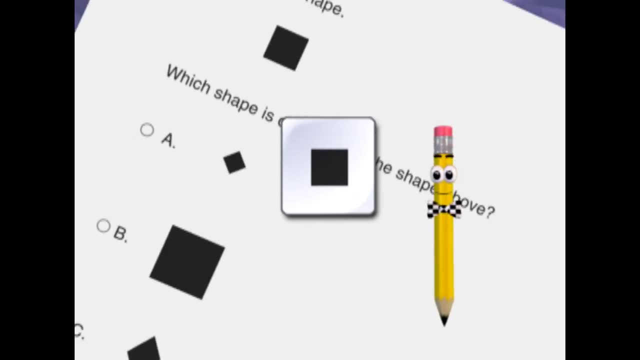 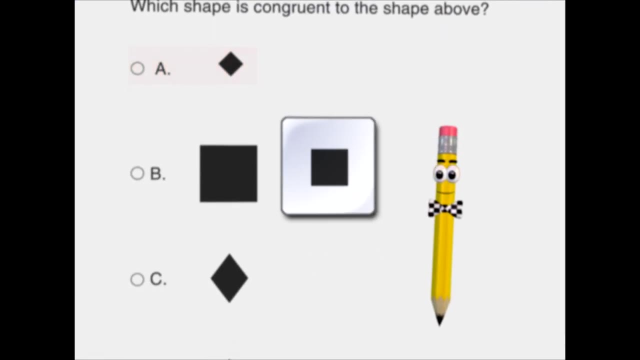 Remember, congruent means the same size and shape, no matter which way the shape is turned. Look at shape A. We can turn the page to see that it is a square, but it is too small. Shape B is a square, but it is too large. 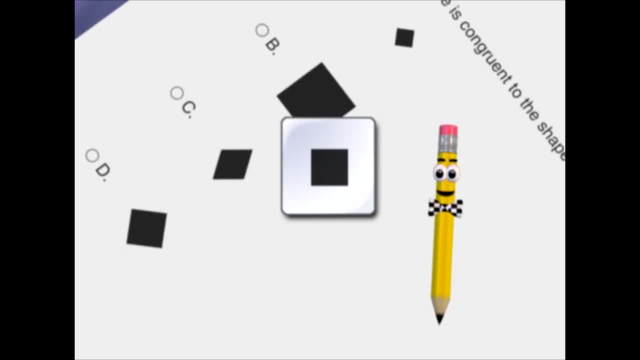 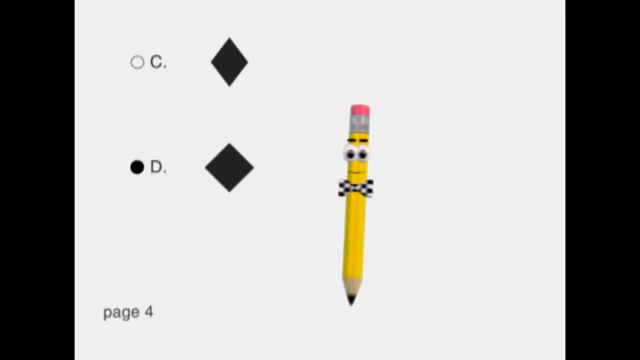 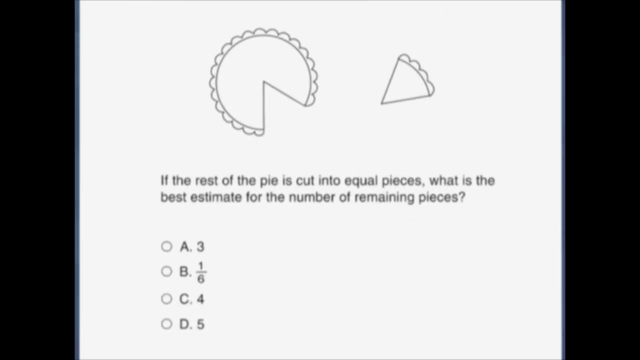 Shape C is a diamond, no matter which way we turn the page, But shape D is a square of the same size turned on its corner. So the answer is D 6.. Judy cut one piece of pie for dessert. If the rest of the pie is cut into equal pieces, what is the best estimate for the number of remaining pieces? 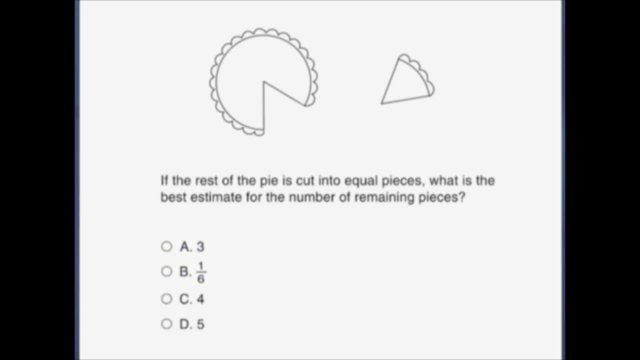 A, 3, B, 1, sixth, C, 4, D, 5. Mike Mechanical, your friendly mechanical pencil, here with a special tip. This would be a great time to use some scratch paper. Sometimes you may not be allowed to write on a test, and you should never write on any test without asking permission. 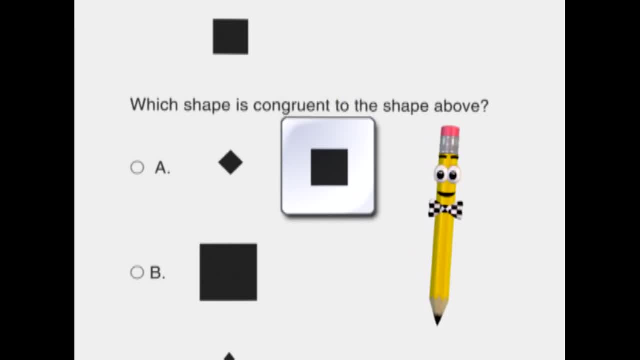 no matter which way the shape is turned. Look, Look at shape A. We can turn the page to see that it is a square, but it is too small. Shape B is a square, but it is too large. Shape C is a diamond. no matter which way we turn the page. 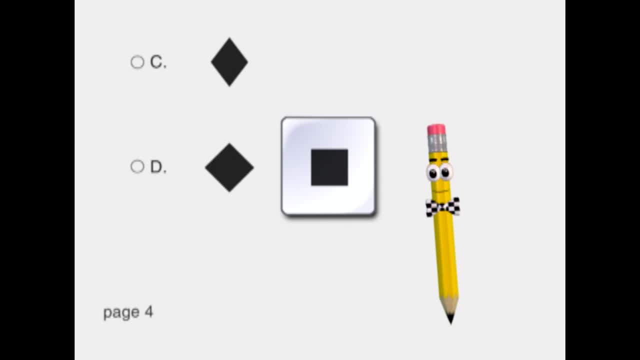 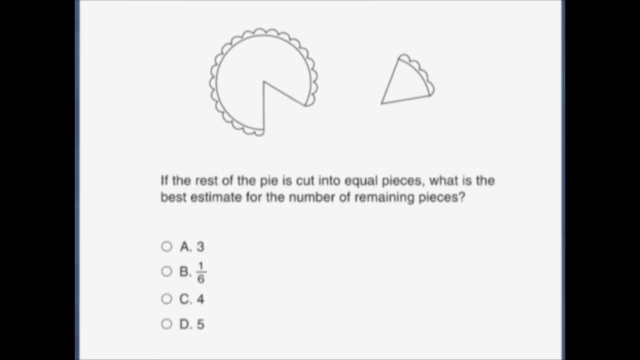 But shape D is a square of the same size turned on its corner. So the answer is D Six. Judy cut one piece of pie for dessert. If the rest of the pie is cut into equal pieces, what is the best estimate for the number of remaining pieces? 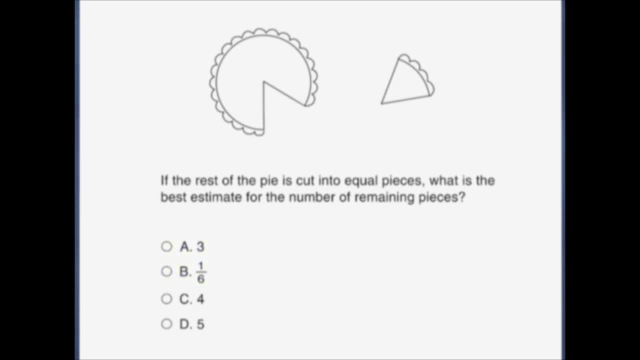 A, Three, B, One-sixth, C, Four, D, Five. Mike Mechanical, your friendly mechanical pencil, here with a special tip. This would be a great time to use some scratch paper. Sometimes you may not be allowed to write on a test. 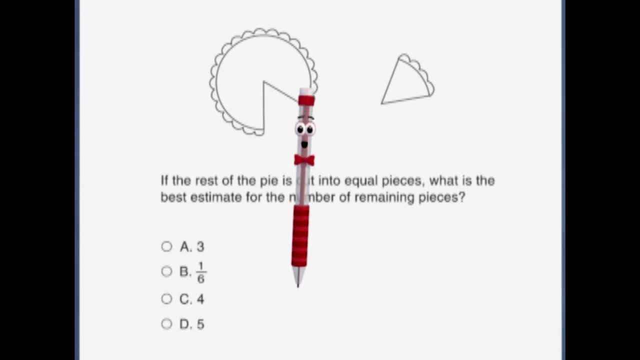 and you should never write on any test without asking permission. But you may be able to use another piece of paper to trace a picture from the test. Good idea. The question is asking for the number of pieces left in the pie If we draw lines out from where the piece is cut, like this: 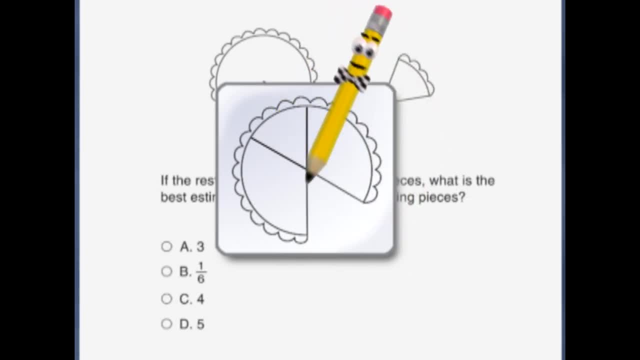 we can see that the pie is cut in half. We can see that the pieces are not yet equal. Let's divide the two larger pieces in half with another line across the pie. Now those pieces look equal to me. Let's count the ones left. 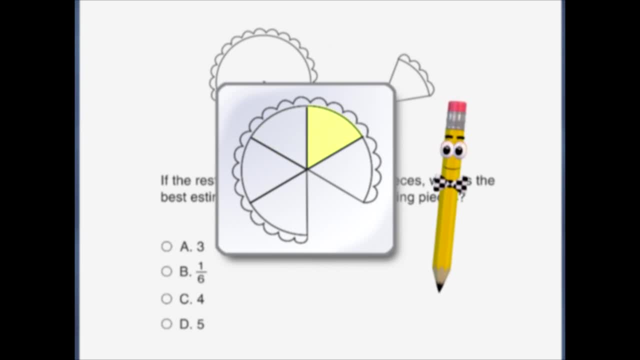 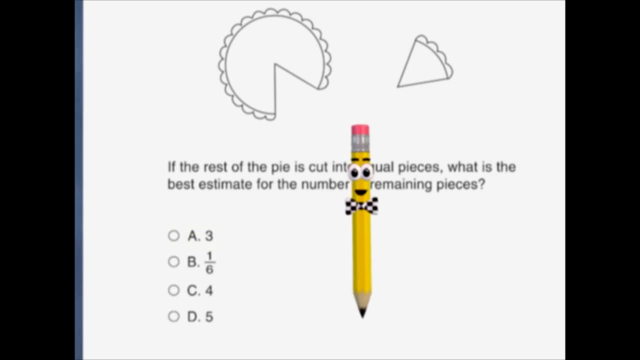 One, Two, Three, Four, Five. Look at our answers. A- Three- No, that is not right. B: One-sixth: That looks like a good estimate for the amount of pie taken out, But we want the number of pieces remaining. 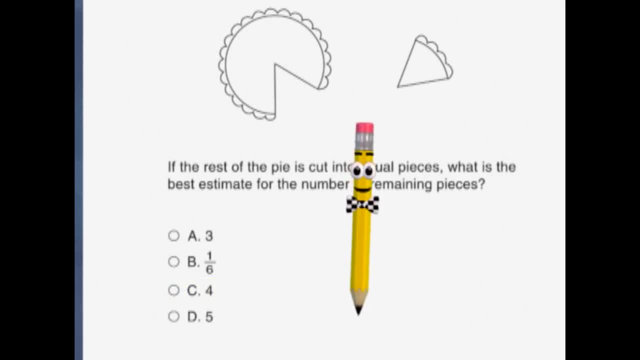 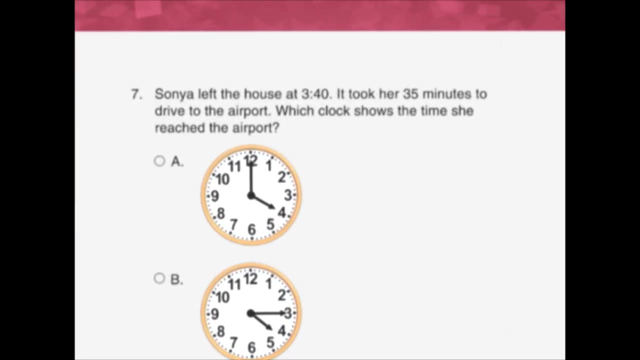 C Four: That's getting closer, but it is still not right. D Five: Ah, that is the right one. Here's another one. Seven: Sonia left the house at 3.40. It took her 35 minutes to drive to the airport. 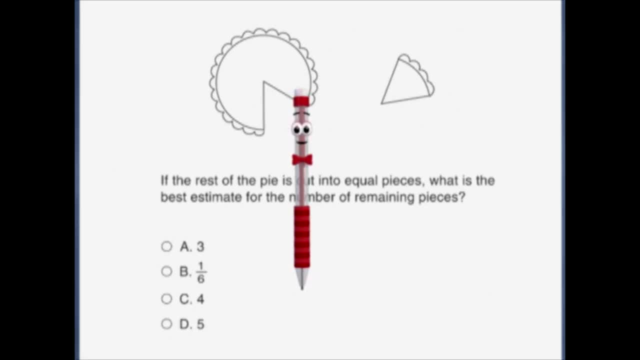 But you may be able to use another piece of paper to trace a picture from the test. Good idea. The question is asking for the number of pieces left in the pie. If we draw lines out from where the pieces cut like this, We can see that the pieces are not yet equal. 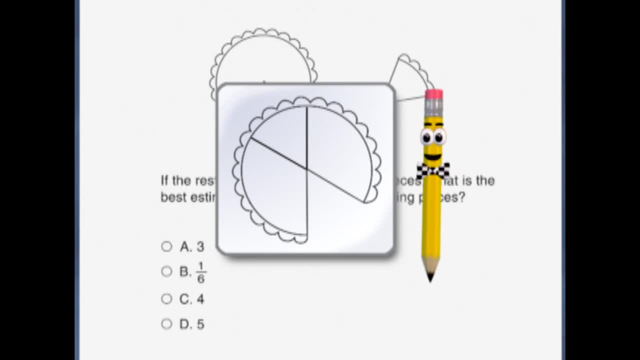 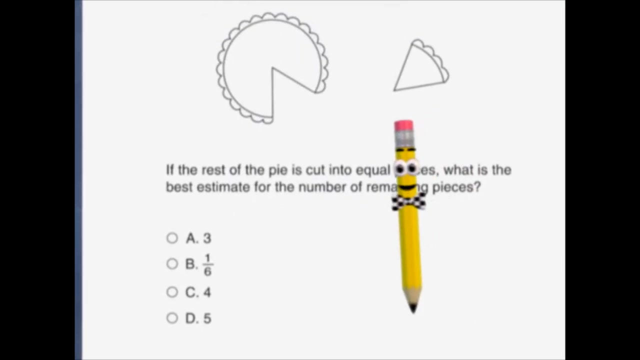 Let's divide the two larger pieces in half with another line across the pie. Now those pieces look equal to me. Let's count the ones left: 1, 2,, 3,, 4, 5. Look at our answers. 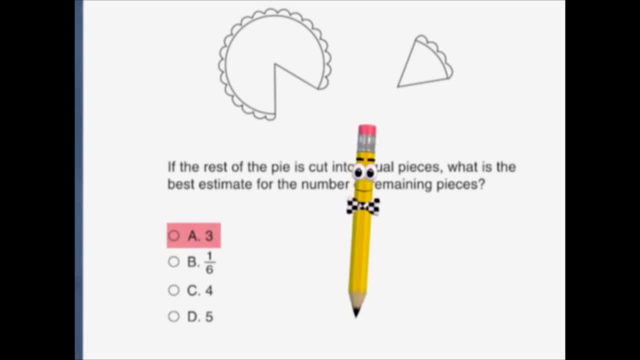 A 3- No, that is not right. B 1- sixth, That looks like a good estimate for the amount of pie taken out, But we want the number of pieces remaining: C 4. That's getting closer, but it is still not right. 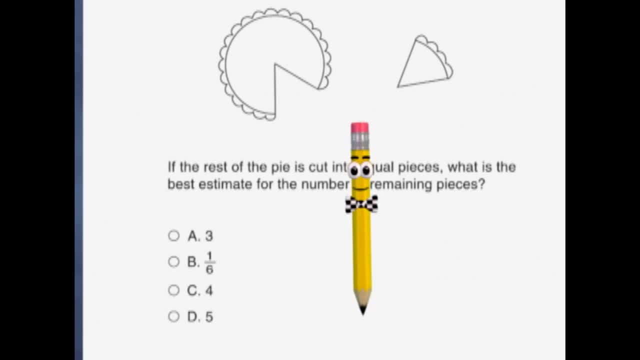 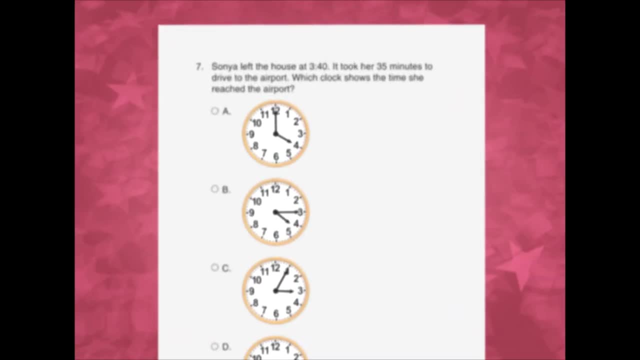 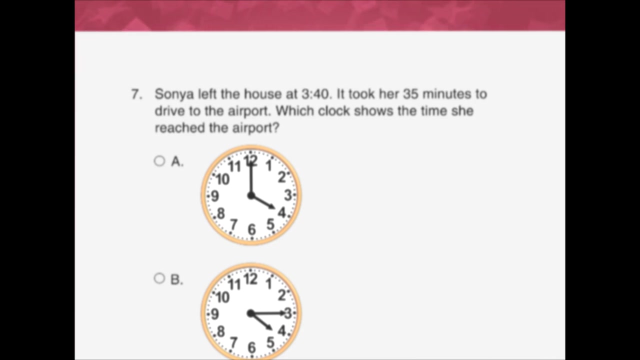 D 5. Ah, that is the right one. Here's another one. 7. Sonia left the house at 3.40. It took her 35 minutes to drive to the airport, Which clock shows the time she reached the airport? 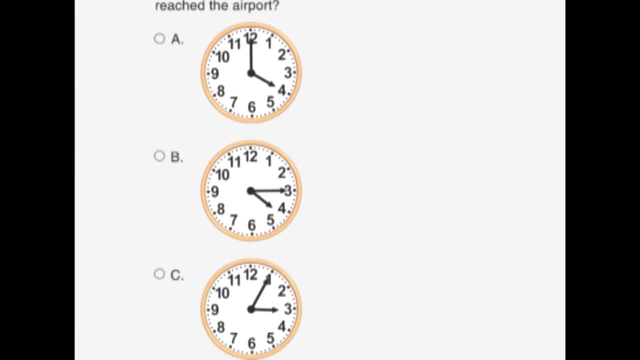 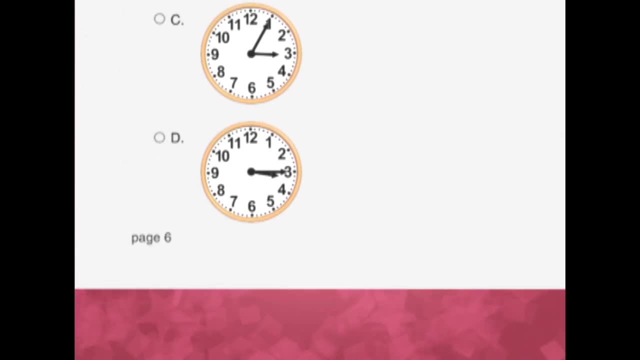 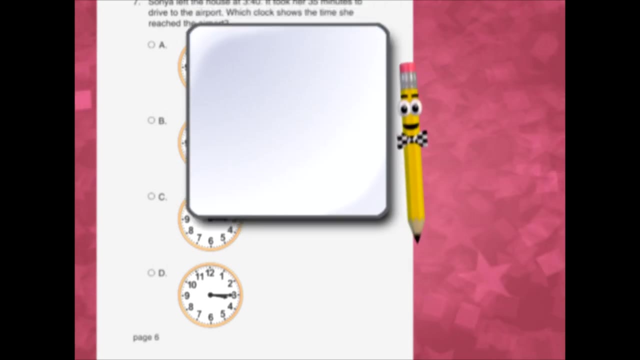 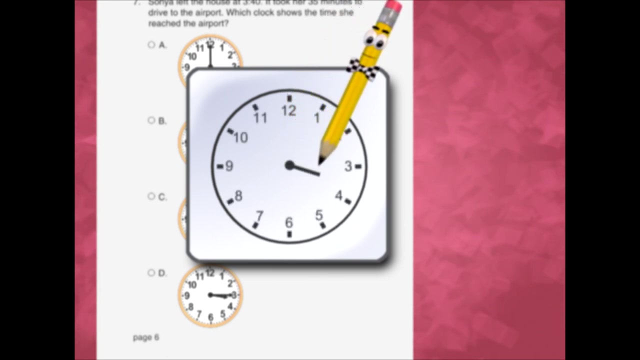 A is 4 o'clock, B is 4.15.. C is 3.05.. And D is 3.15.. Ok, now let's draw a clock that shows the time 3.40.. Next we'll mark off 35 minutes in 5 minute intervals. 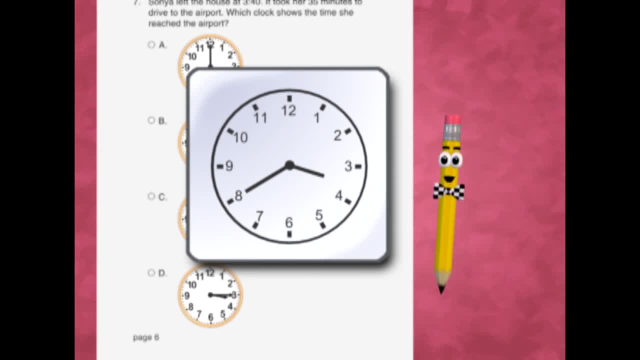 Be sure to go clockwise as you mark, because Sonia is going forward in time 35 minutes. 5,, 10,, 15,, 20,, 25,, 30,, 35.. Ah, notice that we crossed over the 12 at the top of the clock. 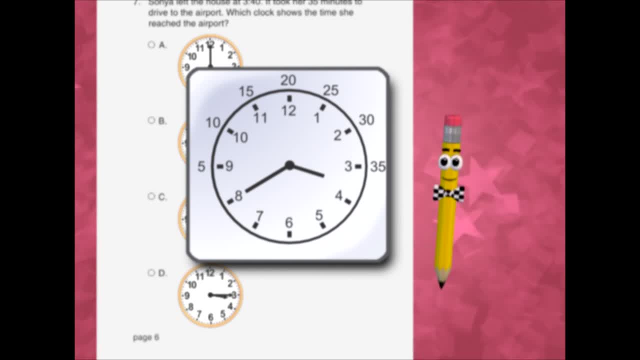 That means we need to move the hour hand forward to 4. And put the minute hand on the 3,, which is the 15 minute mark, So the time will be 4.15.. The clock for answer B shows 4.15.. 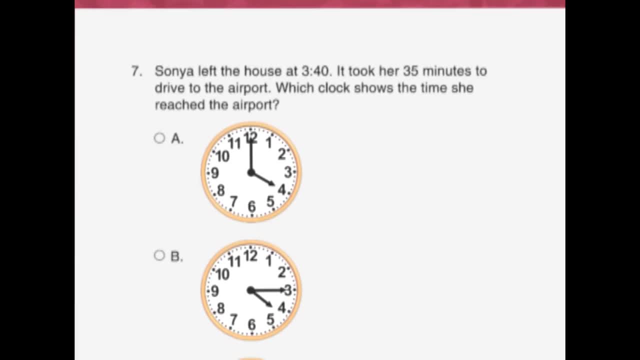 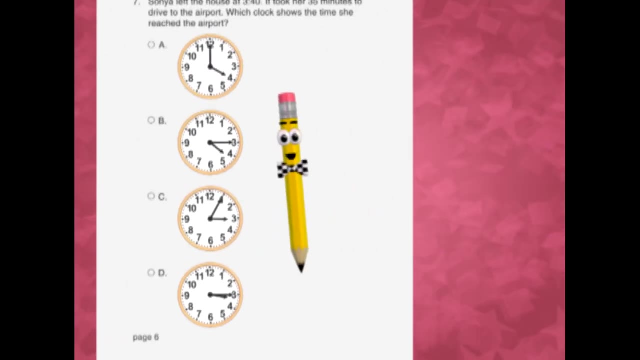 Which clock shows the time she reached the airport. A is 4 o'clock, B is 4.15.. C is 3.05.. And D is 3.15.. Okay, now let's draw a clock that shows the time 3.40.. 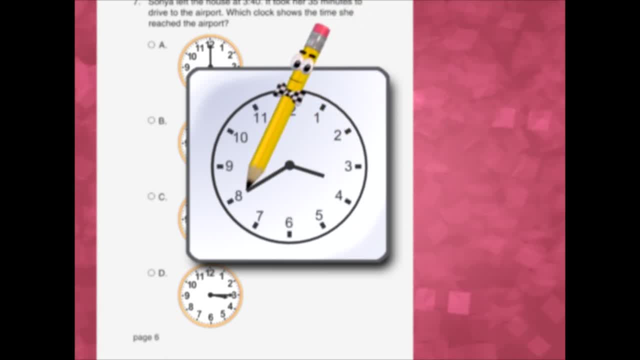 Next we'll mark off 35 minutes in 5-minute intervals. Be sure to go clockwise as you mark, because Sonia is going forward in time. 35 minutes: Five, Ten, Fifteen, Twenty, Twenty-five, Thirty, Thirty-five. 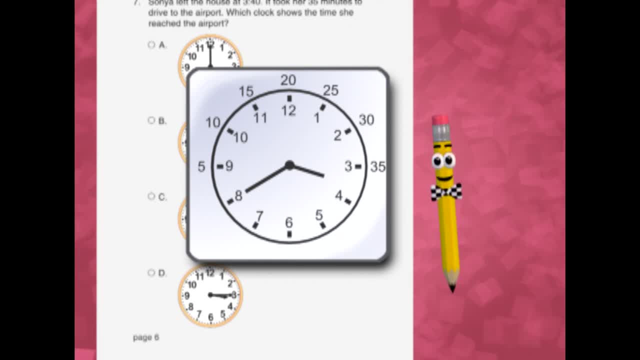 Ah, notice that we crossed over the 12 at the top of the clock. That means we need to move the hour hand forward to four And put the minute hand on the three, Which is the 15-minute mark. So the time will be 4.15.. 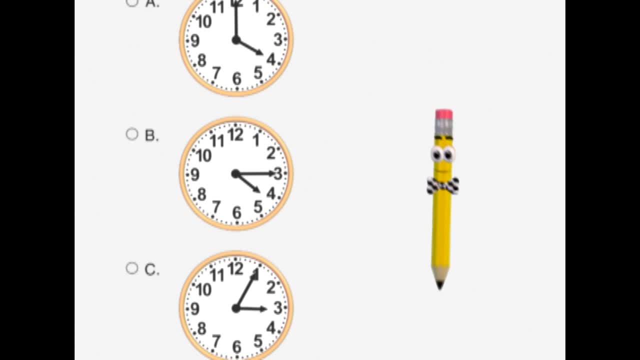 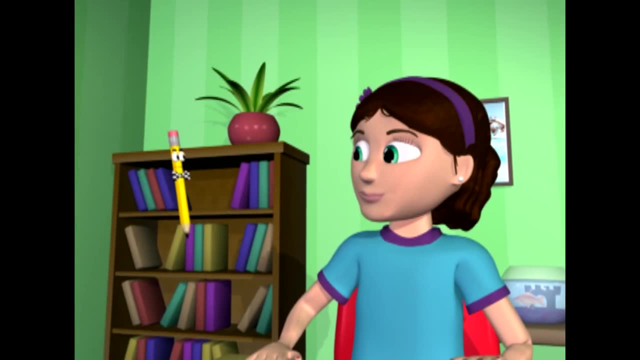 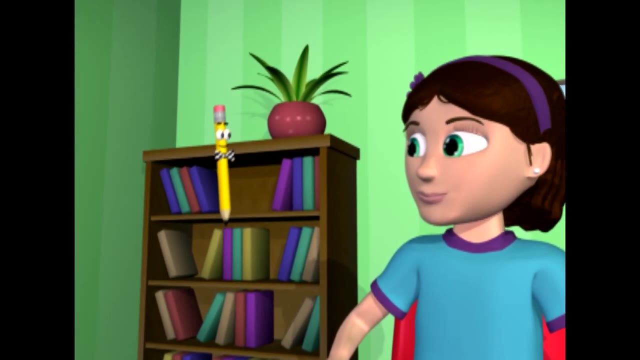 The clock for answer B shows 4.15.. The answer is B. Ooh, If we had forgotten to put the hour hand forward an hour, we would have gotten the answer wrong. That's why it is a lie. That's why it is a good idea to check your drawing every time before you mark your answer. 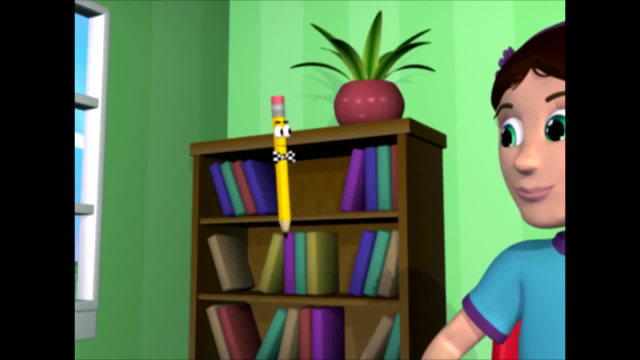 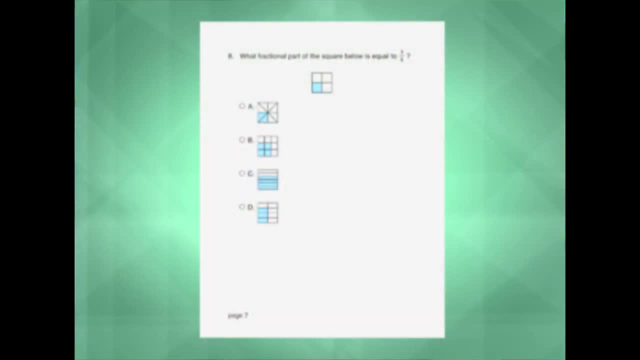 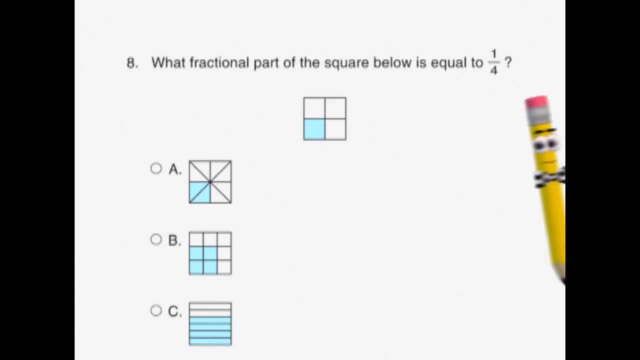 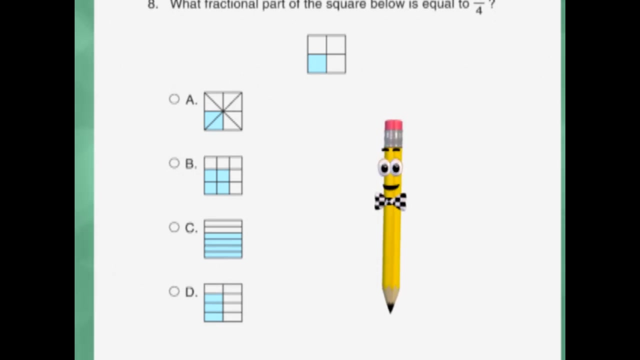 to see if you marked the 12 as you marked the clock. It is good to take your time and think the problems through carefully. Eight: What fractional part of the square below is equal to one-fourth? Looking at the possible answers, B and C have too much area shaded to be one-fourth. 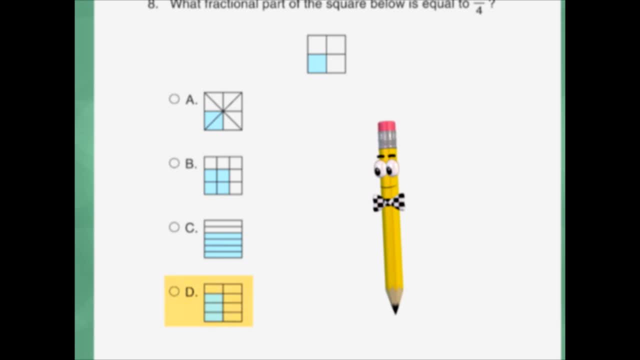 D is very close, But A has exactly the one-fourth shaded that is shown in the example, So the answer is A. Oops, I started feeling in the wrong bubble. I need to be sure and erase it completely So that the right answer will be counted. 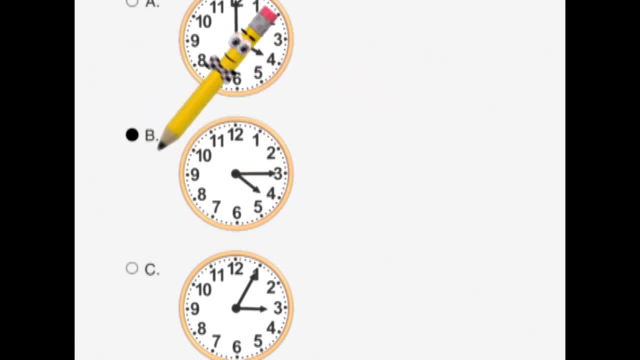 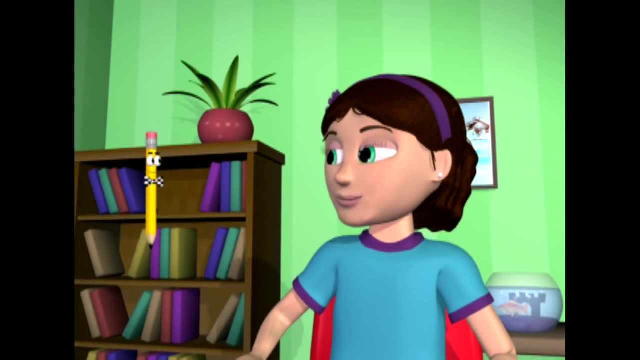 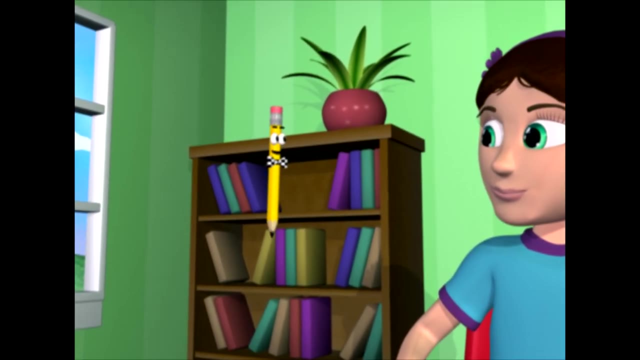 The answer is B. Ooh, if we had forgotten to put the hour hand forward an hour, we would have gotten the answer wrong. That's why it is a good idea to check your drawing every time before you mark your answer to see if you marked the 12 as you marked the clock. 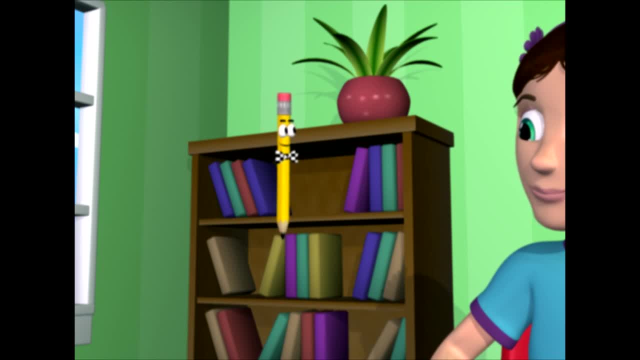 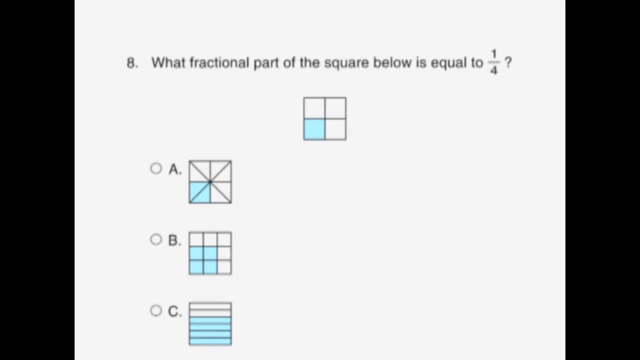 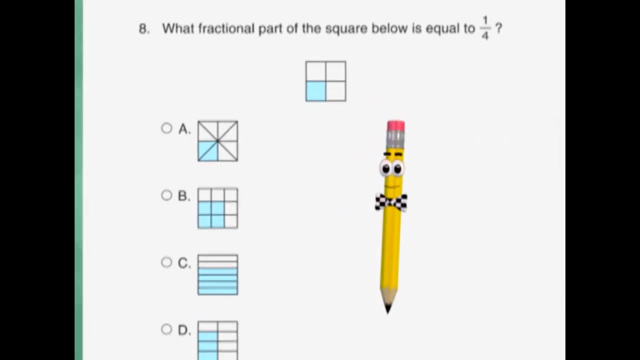 It is good to take your time and think the problems through carefully. 8. What fractional part of the square below is equal to one-fourth? Looking at the possible answers, B and C have too much area shaded to be one-fourth. 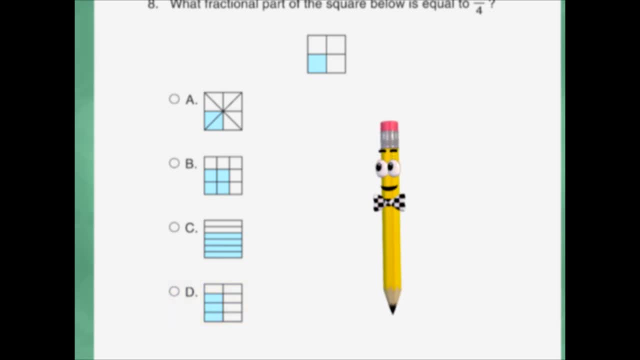 D is very close, But A has exactly the one-fourth shaded that is shown in the example, So the answer is A. Oops, I started filling in the wrong bubble. I need to be sure and erase it completely So that the right answer will be counted. 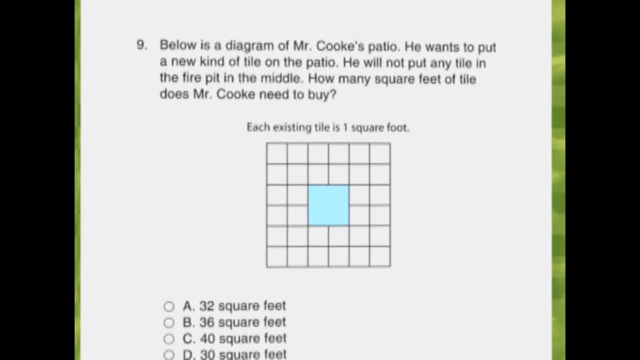 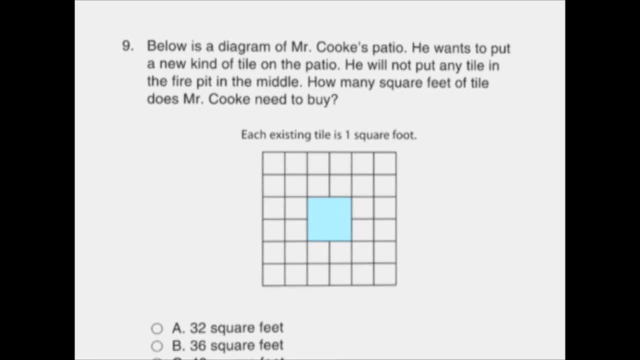 On we go 9.. Below is a diagram of Mr Cook's patio. He wants to put a new kind of tile on the patio. He will not put any tile in the fire pit in the middle. How many square feet of tile does Mr Cook need to buy? 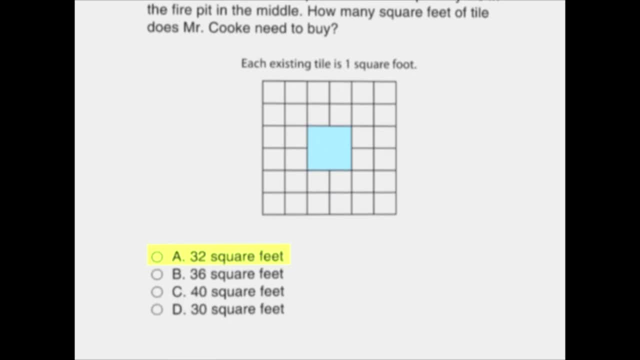 Each existing tile is one square foot, 32 square feet, 36 square feet, 40 square feet D, 30 square feet, Ah. so if the problem is asking for the number of square feet, we need to find the area. 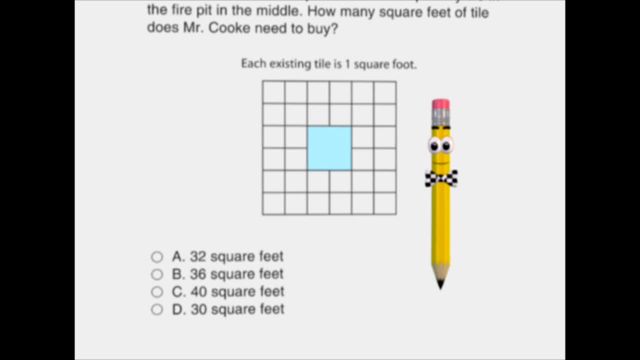 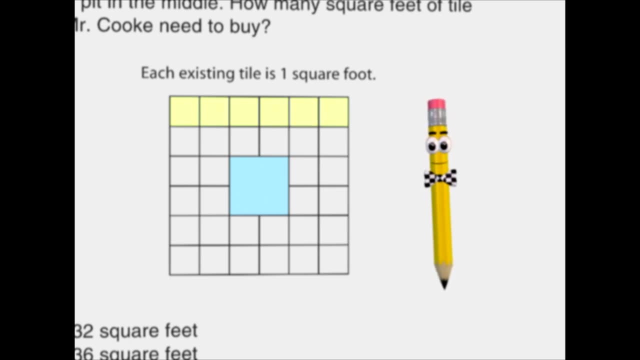 First let's see how many squares we have, including the fire pit: 1,, 2,, 3,, 4,, 5, 6 tiles across 1,, 2,, 3,, 4,, 5, 6 tiles down. 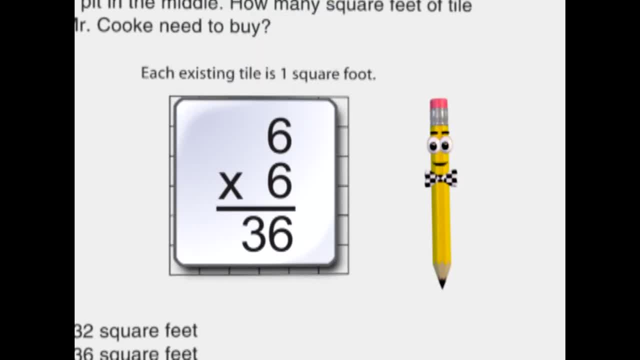 6 times 6 is 36.. But that is not our answer. We need to subtract the fire pit area. The fire pit is 1, 2 tiles across and 1, 2 tiles down. 2 times 2 is 4.. 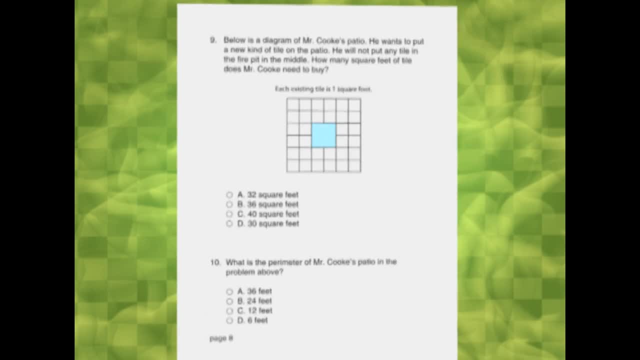 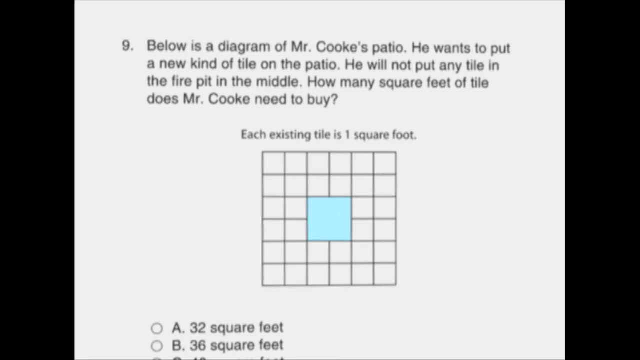 On we go. Nine. Below is a diagram of Mr Cook's patio. He wants to put a new kind of tile on the patio. He will not put any tile in the fire pit in the middle. How many square feet of tile does Mr Cook need to buy? 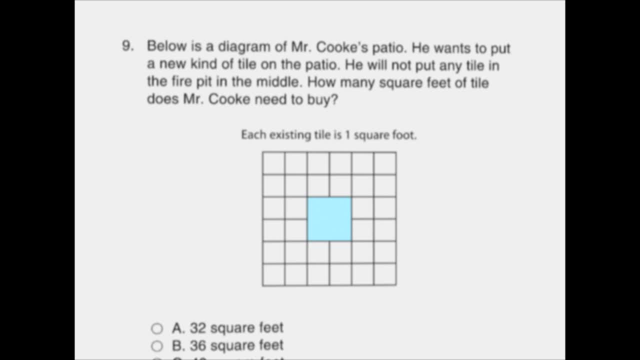 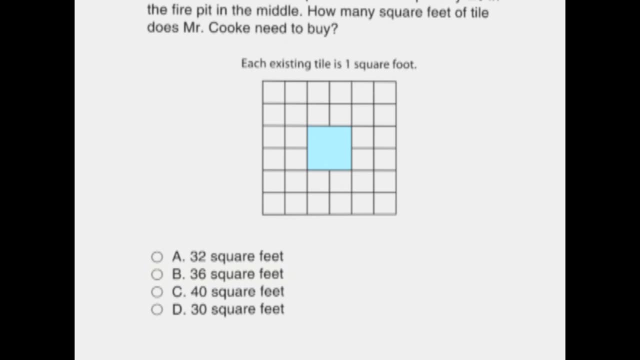 Each existing tile is one square foot. A. Thirty-two square feet B. Thirty-six square feet C. Forty square feet D. Thirty square feet, Ah. So if the problem is asking for the number of square feet, we need to find the area. 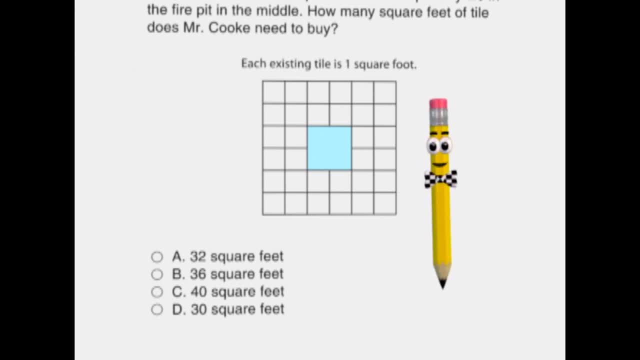 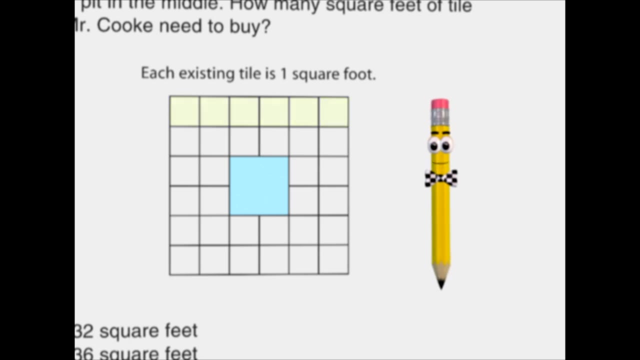 First let's see how many squares we have, including the fire pit: One, two, three, four, five, six, seven, eight, nine, twelve, three, four, five, six tiles across One, two, three. 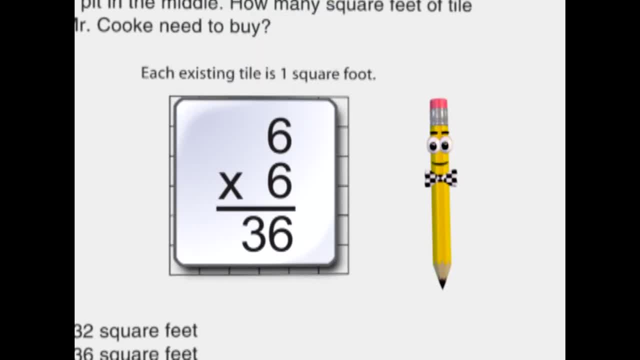 four, five, six tiles down. Six times six is thirty-six. But that is not our answer. We need to subtract the fire pit area. The fire pit is one, two tiles across and one, two tiles down. Two times two is four. 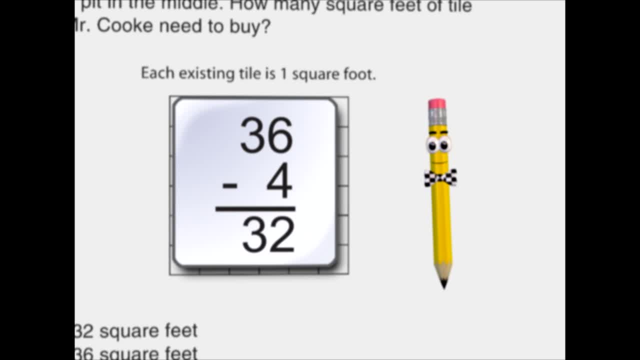 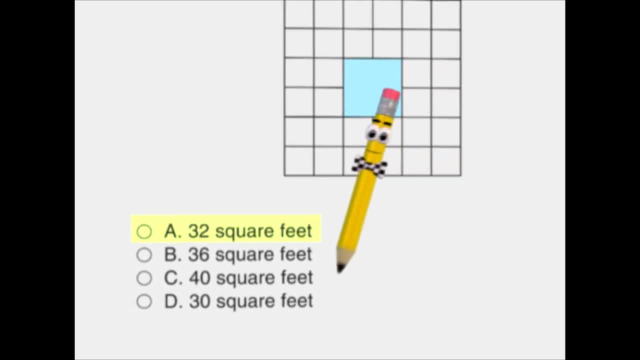 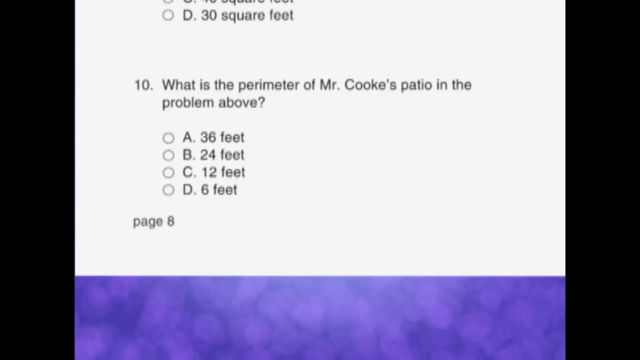 Subtract four from thirty-six to get our answer Thirty-two. We need thirty-two tiles And each tile is one square foot, So the answer is A Thirty-two square feet Ten. What is the perimeter of Mr Cook's patio in the problem above? 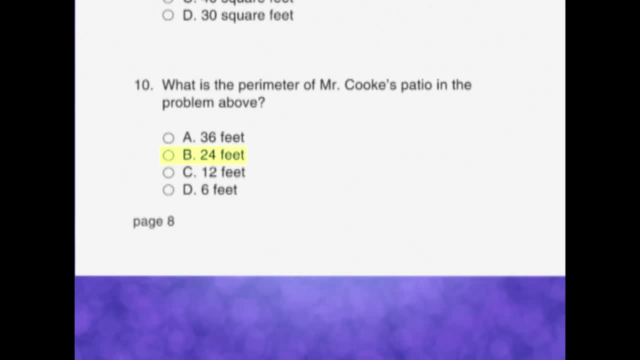 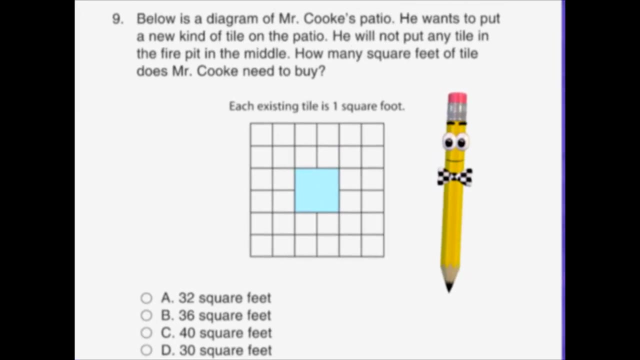 A- Thirty-six feet, B- Twenty-four feet, C- Twelve feet, D- Six feet. The perimeter is the distance around the outside of the patio. The patio is a six by six foot square, So the perimeter is six times four equals twenty-four. 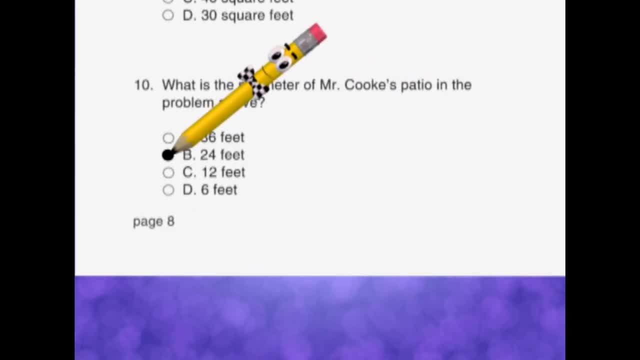 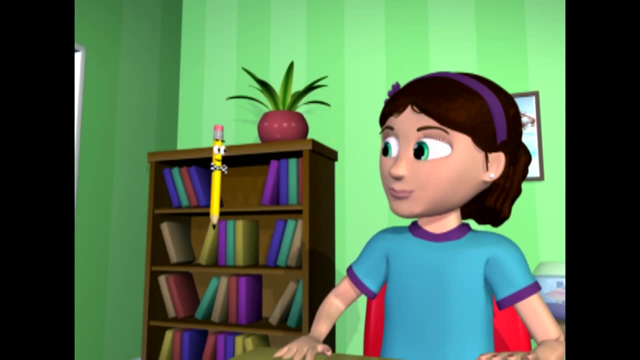 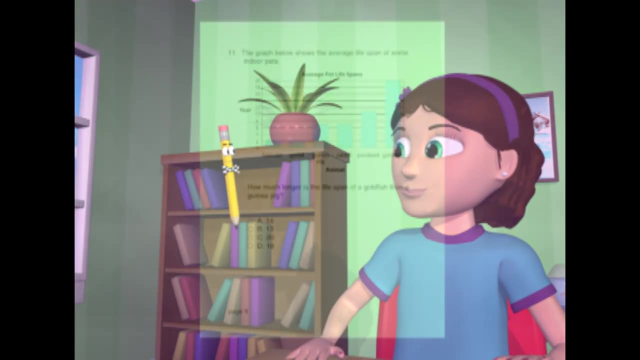 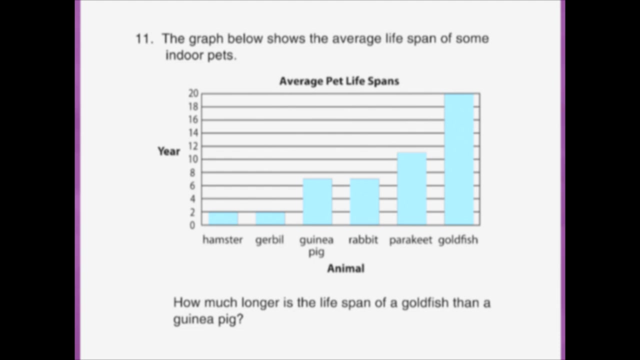 That's answer B. Twenty-four feet, Tell me, do you know why pencils can't grow beards? I don't know, Because they're always shaving Eleven. The graph below shows the average lifespan of some indoor pets. How much longer is the lifespan of a goldfish than a guinea pig? 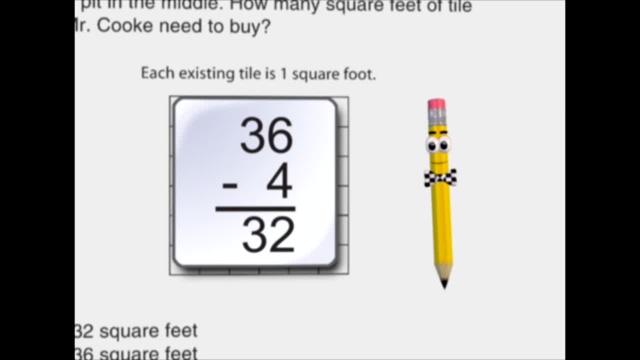 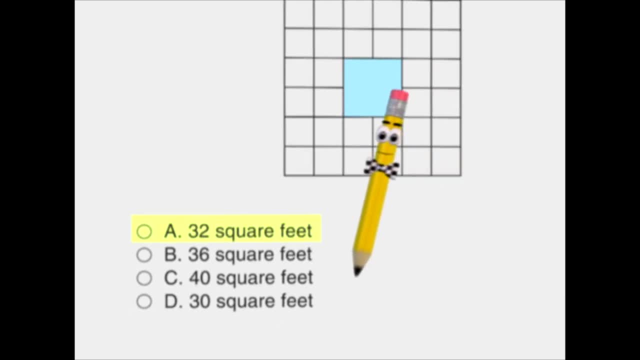 Subtract 4 from 36 to get our answer 32.. We need 32 tiles And each tile is one square foot. So the answer is A 32 square feet: 3,, 4,, 5,, 6,, 7,, 8,, 9,, 10.. 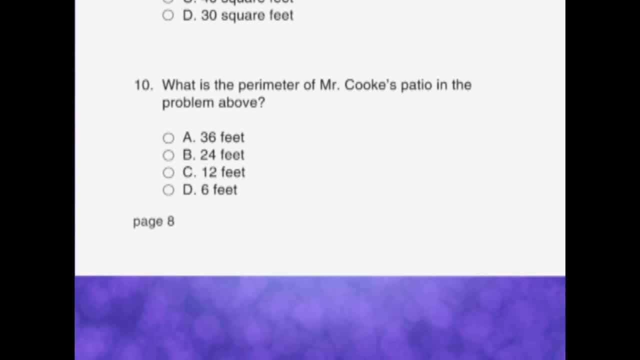 10. What is the perimeter of Mr Cook's patio in the problem above? A- 36 feet. B- 24 feet. C- 12 feet, D- 6 feet. The perimeter is the distance around the outside of the patio. 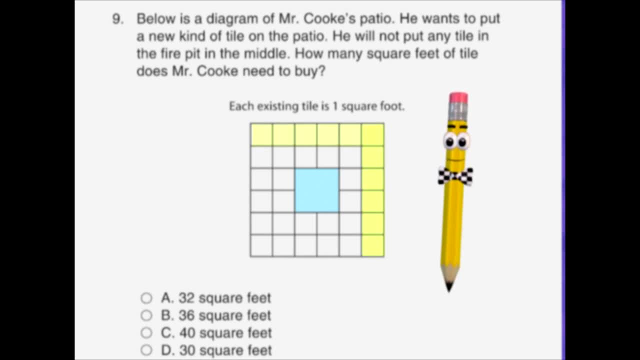 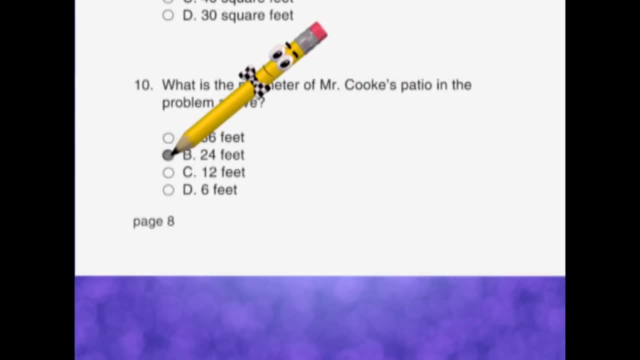 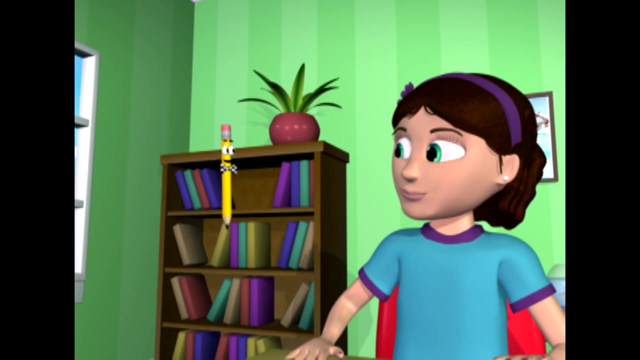 The patio is a 6 by 6 foot square, So the perimeter is 6 times 4 equals 24.. That's answer: B, 24 feet. Tell me, do you know why pencils can't grow beards? I don't know. 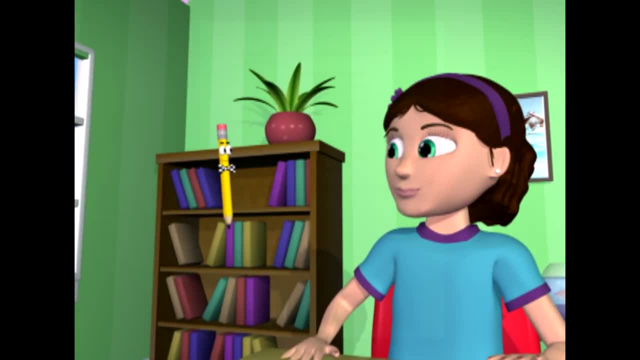 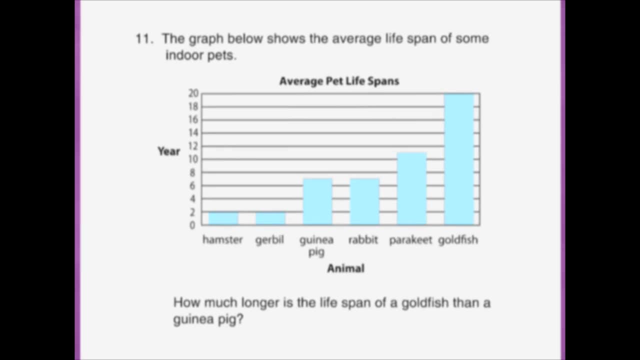 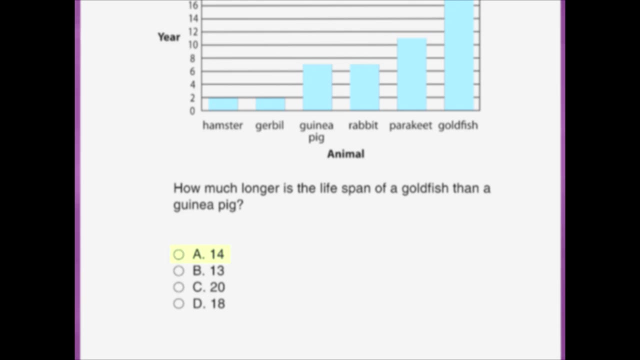 Because they're always shaving 11.. The graph below shows the average lifespan of some indoor pets. How much longer is the lifespan of a goldfish than a guinea pig? A, 14., B, 13., C, 20.. 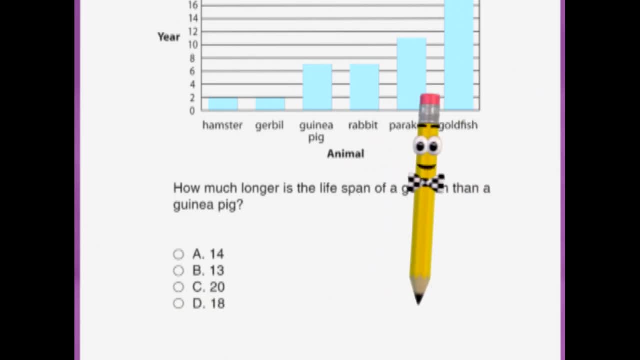 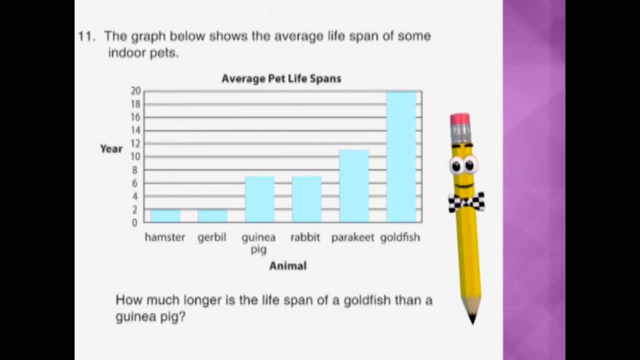 D 18.. Look at the bar graph. The goldfish has a 20 year lifespan, While the guinea pig lives only 7 years. We are comparing them to find out how much longer the goldfish lives. So just subtract 7 from 20.. 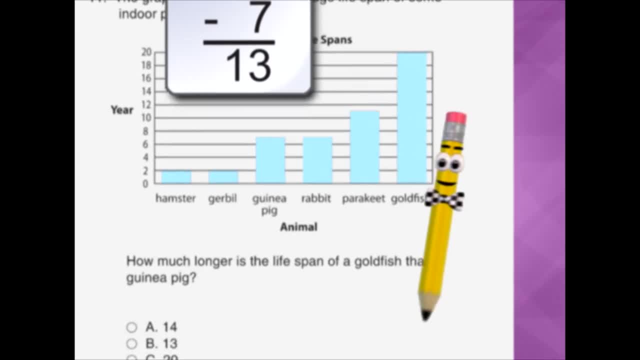 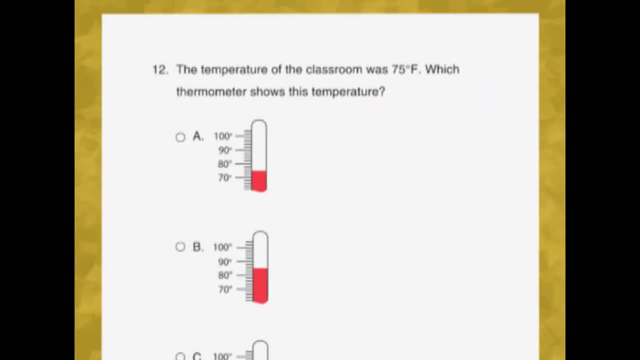 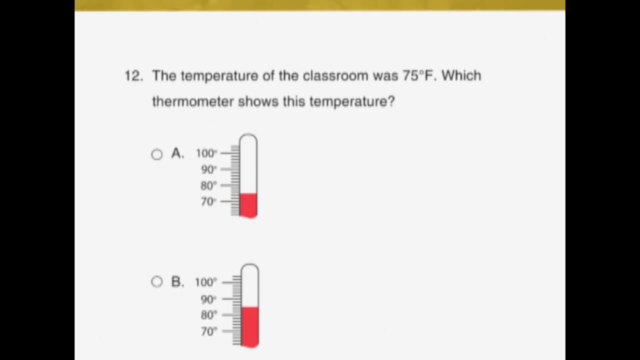 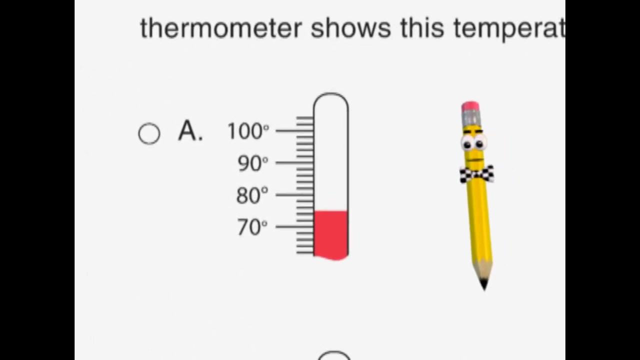 20 minus 7 equals 13.. That's answer B 13. 12. The temperature of the classroom was 75 degrees Fahrenheit. Which thermometer shows this temperature? These thermometers have 5 lines for every 10 degrees Fahrenheit. 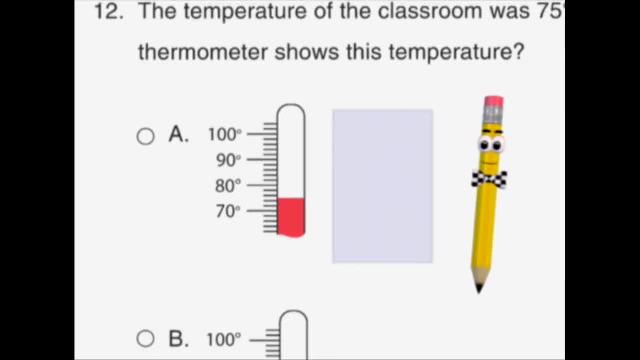 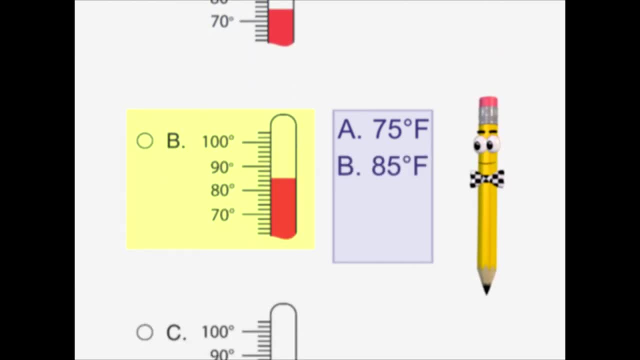 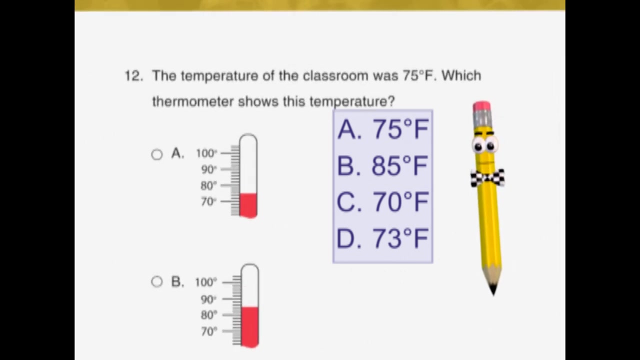 So each line is 2 degrees Fahrenheit, No problem. A is 75 degrees Fahrenheit. B is 85 degrees Fahrenheit. C is 70 degrees Fahrenheit D is 73 degrees Fahrenheit. Thermometer A: 75 degrees Fahrenheit is the correct answer. 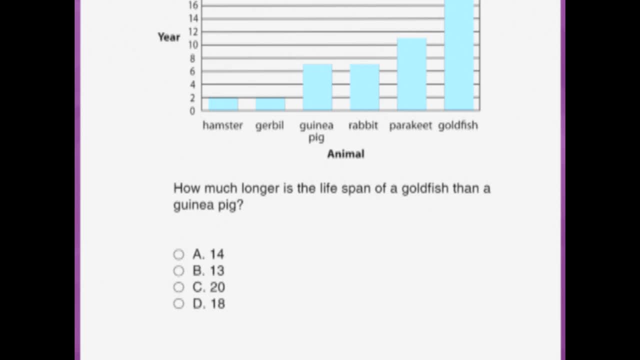 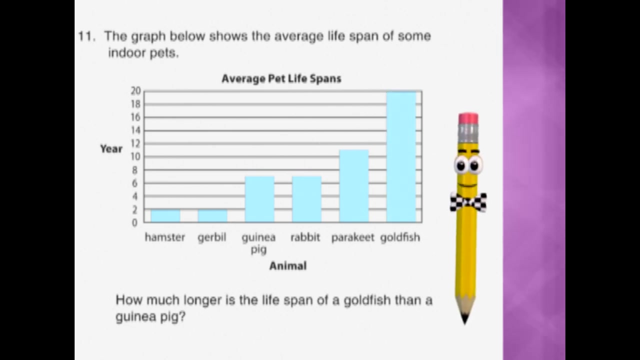 A, Fourteen B, Thirteen C, Twenty D, Eighteen. Look at the bar graph. The goldfish has a twenty year lifespan, while the guinea pig lives only seven years. We are comparing them to find out how much longer the goldfish lives. 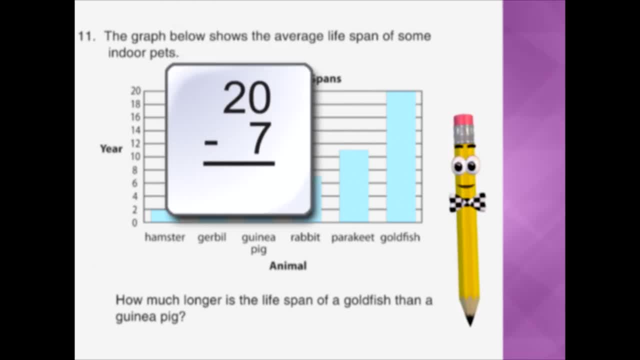 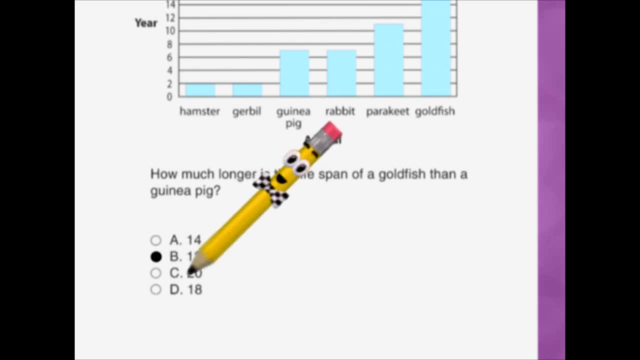 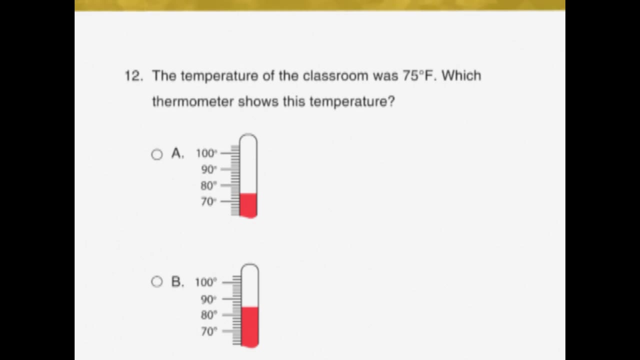 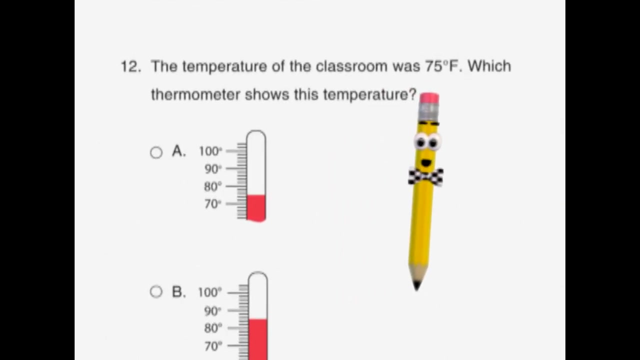 So just subtract seven from twenty. Twenty minus seven equals thirteen. That's answer B Thirteen Twelve. The temperature of the classroom was seventy-five degrees Fahrenheit. Which thermometer shows this temperature? These thermometers have five lines for every ten degrees Fahrenheit. 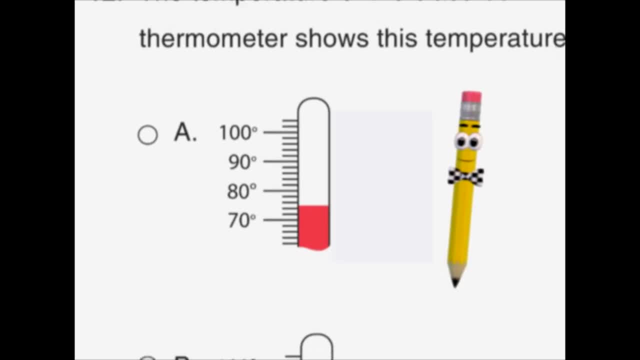 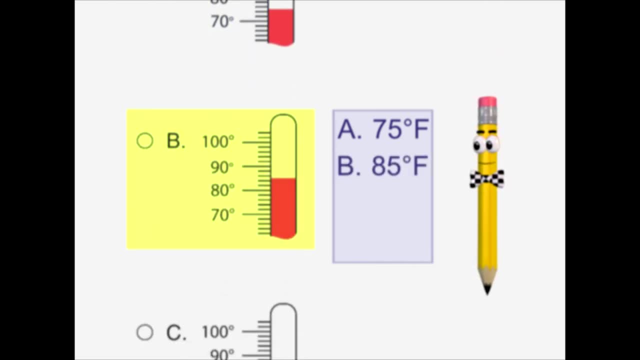 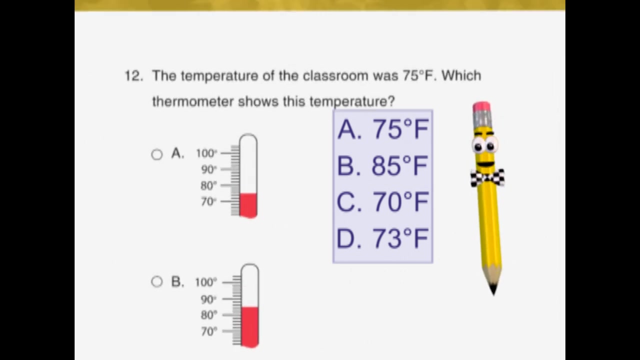 So each line is two degrees Fahrenheit, No problem. A is seventy-five degrees Fahrenheit. B is eighty-five degrees Fahrenheit. C is seventy degrees Fahrenheit D is seventy-three degrees Fahrenheit. Thermometer A: Seventy-five degrees Fahrenheit is the correct answer. 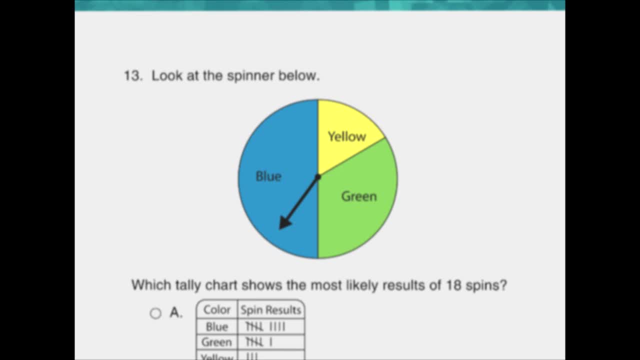 Thirteen: Look at the spinner below, Which tally chart shows the most likely results of eighteen spins. The most likely result of one spin is blue. Since that is the largest part of the spinner, We should look for the answer with the most blue spins. 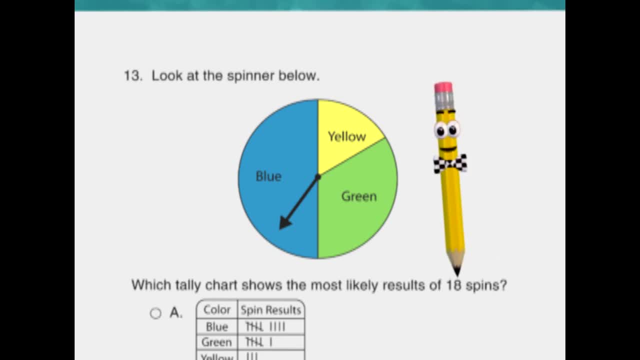 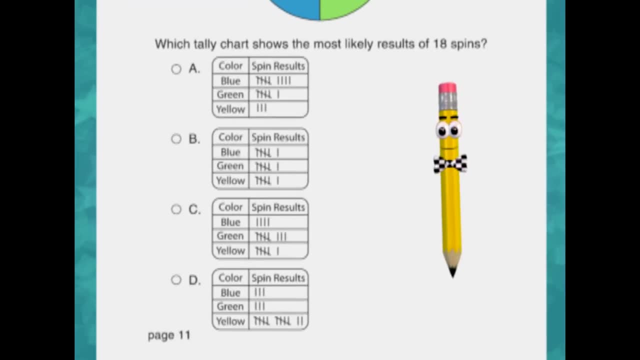 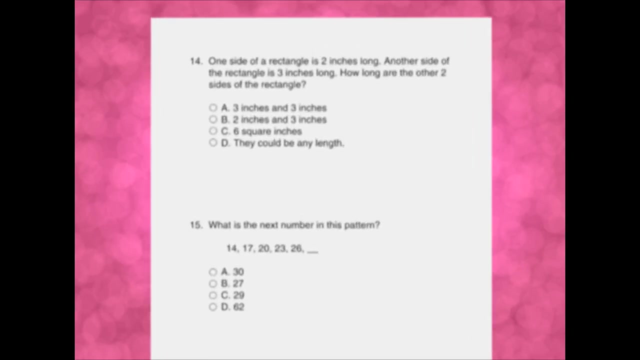 Also, yellow is the smallest area on the spinner, So our yellow spins should be low. Answer: A shows nine blue spins and only three yellow spins. That is the most blue and the fewest yellow spins. So the answer is A Fourteen. 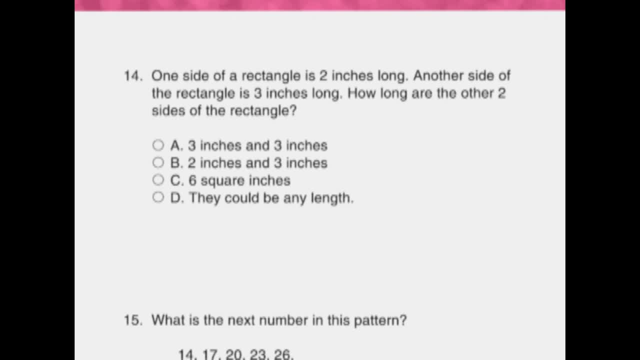 One side of a rectangle is two inches long. Another side of the rectangle is three inches long. How long are the other two sides of the rectangle? A- Three inches and three inches. B- Two inches and three inches. C- Six square inches. 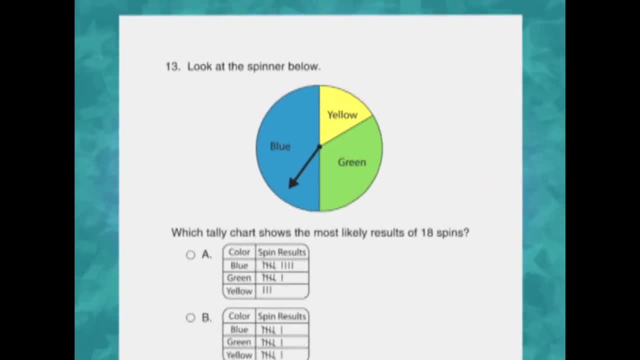 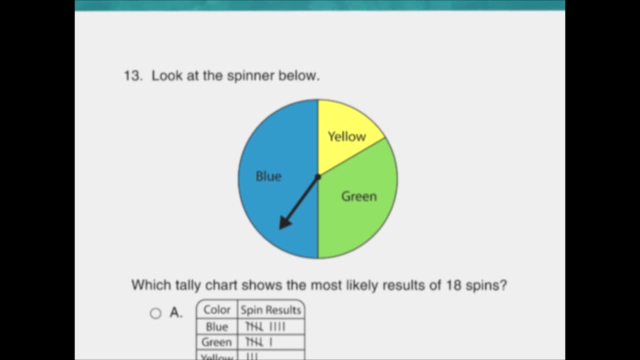 The answer is B 13.. Look at the spinner below, Which tally chart shows the most likely results of 18 spins. The most likely result of one spin is blue. since that is the largest part of the spinner, We should look for the answer with the most blue spins. 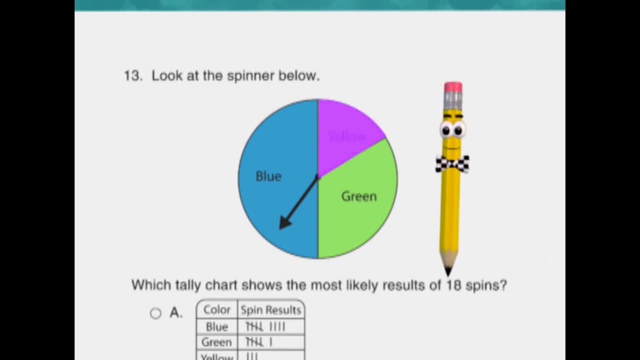 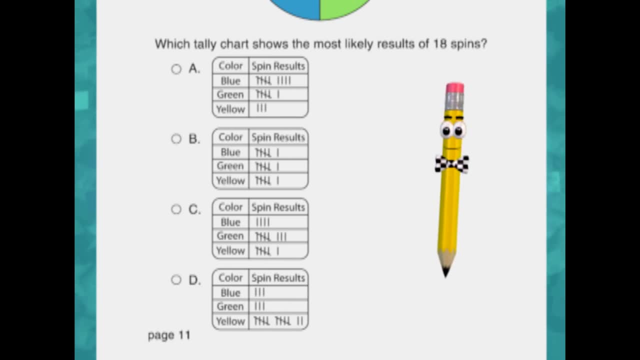 Also, yellow is the smallest area on the spinner, So our yellow spins should be low. Answer: A shows 9 blue spins and only 3 yellow spins. That is the most blue and the fewest yellow spins of any chart. So the answer is: 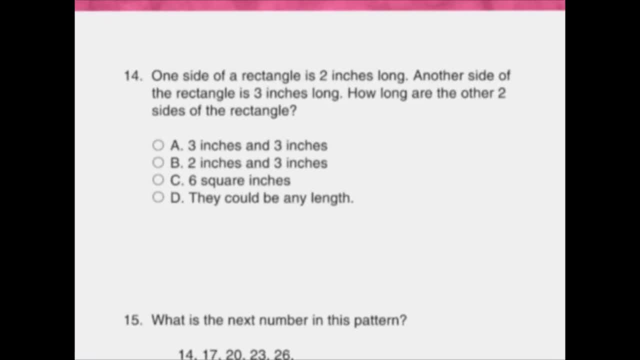 A- 14.. One side of a rectangle is 2 inches long. Another side of the rectangle is 3 inches long. How long are the other two sides of the rectangle? A- 3 inches and 3 inches? B- 2 inches and 3 inches. 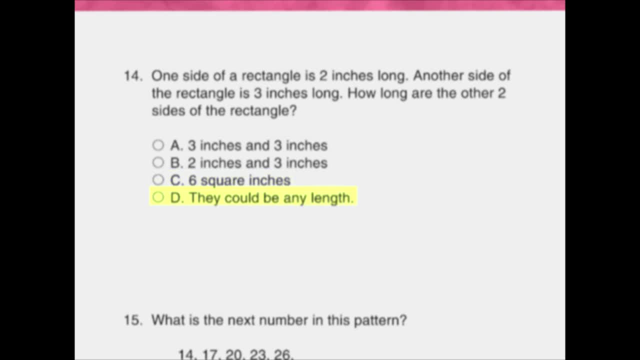 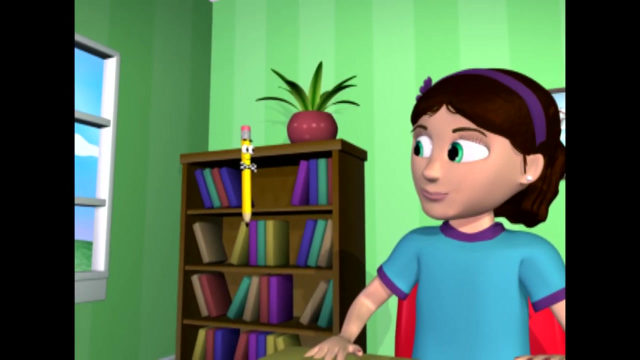 C, 6 square inches. D. They could be any length. A rectangle has two equal sides, so the other sides will be the same as the two. given The answer is B, 2 inches and 3 inches, Do you know why the number 6 ran away from the number 7?? 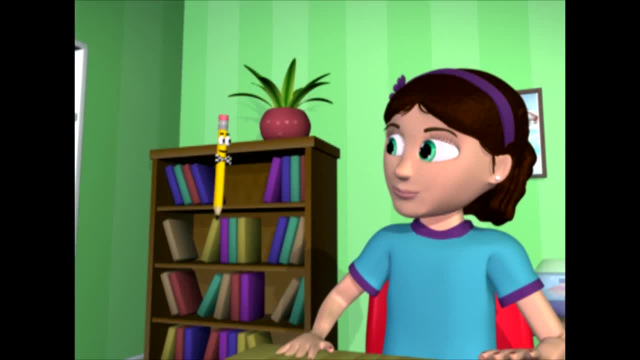 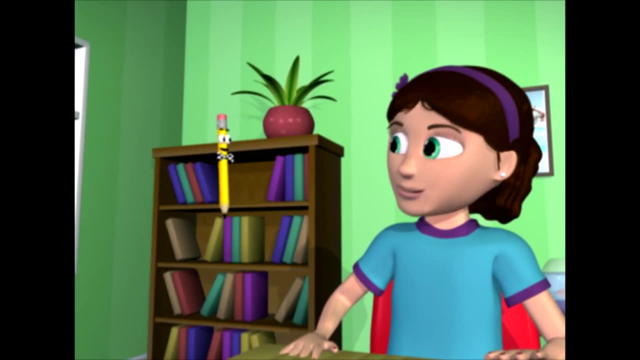 No, Because 7, 8, 9.. Oh brother, Get it. 7, 8, 9! And then 7, 8, 9. numbers are in order. Hey, numbers in certain order are a pattern. 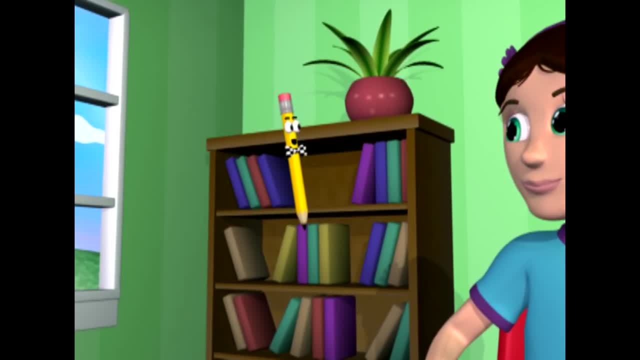 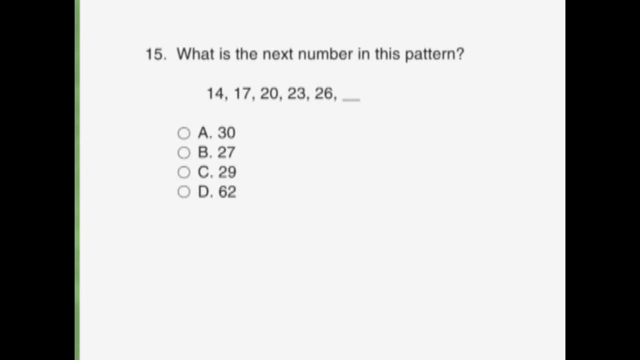 And looking for a pattern can help you solve some problems on a math test. Let me show you what I mean. Look at this problem 15.. What is the next number in this pattern? 14,, 17,, 20,, 23,, 26.. 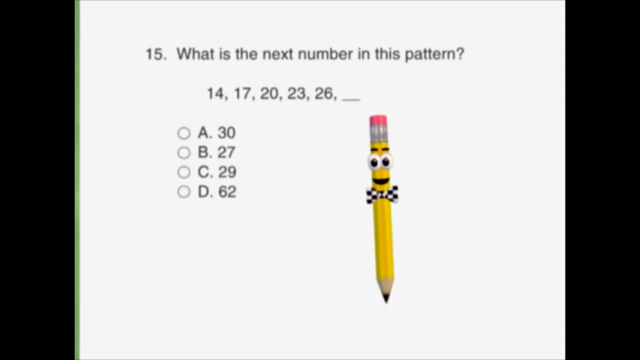 Can you see the pattern? 17 is 3 more than 14.. 20 is 3 more than 17.. 23 is 3 more than 20, and so on. The next number should be 3 more than 26.. That's 29.. 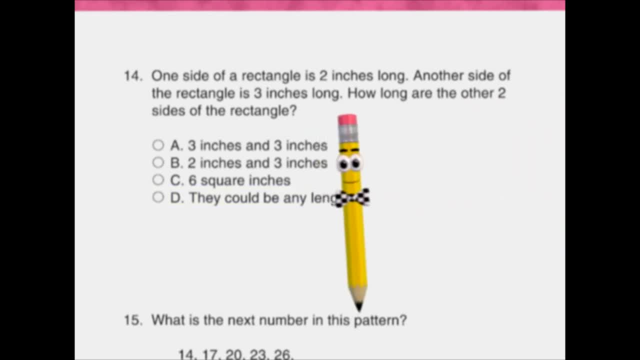 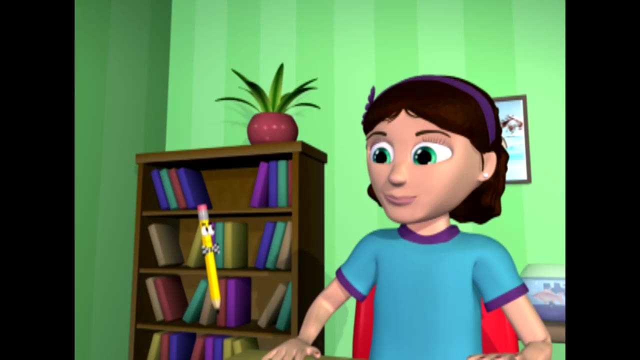 D. They could be any length. A rectangle has two equal sides, So the other sides will be the same as the two given. The answer is B, Two inches and three inches. Do you know why the number six ran away from the number seven? 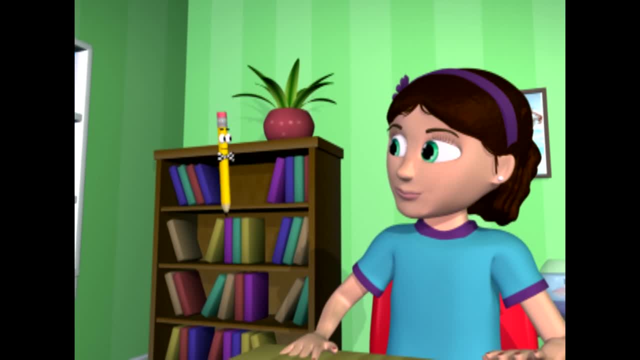 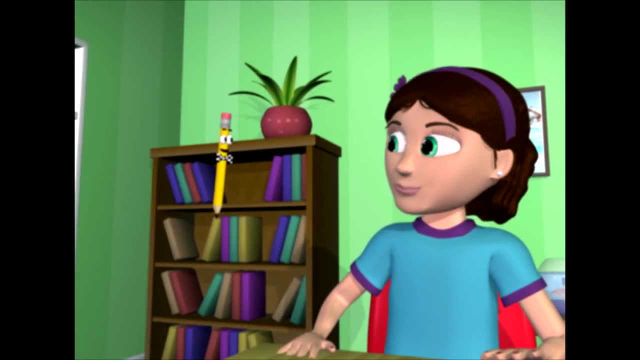 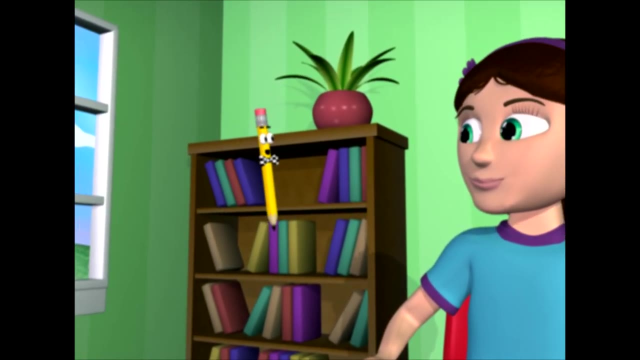 No, Because seven eight nine, Oh brother, Get it. Seven eight nine And then seven eight nine. numbers are in order. Hey, numbers in certain order are a pattern, And looking for a pattern can help you solve some problems on a math test. 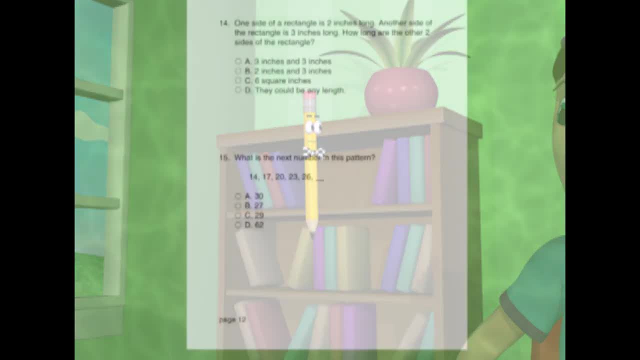 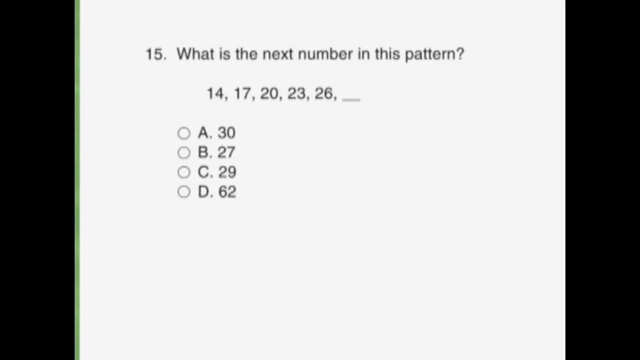 Let me show you what I mean. Look at this problem: Fifteen- What is the next number in this pattern? Fourteen, seventeen, twenty, twenty-three, twenty-six. Can you see the pattern? Seventeen is three more than fourteen. 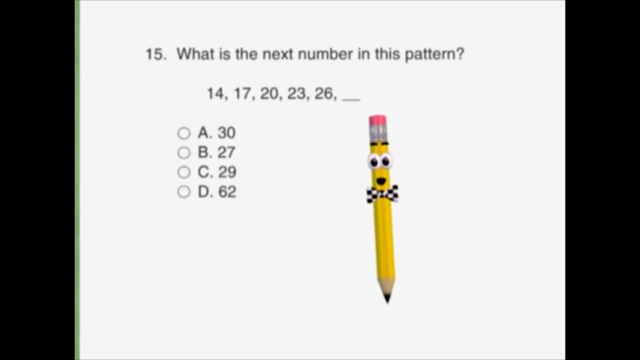 Twenty is three more than seventeen, Twenty-three is three more than twenty, and so on. The next number should be three more than twenty-six. That's twenty-nine. Let's see if that is in the answers. A: thirty, no. B: twenty-seven, not that one. 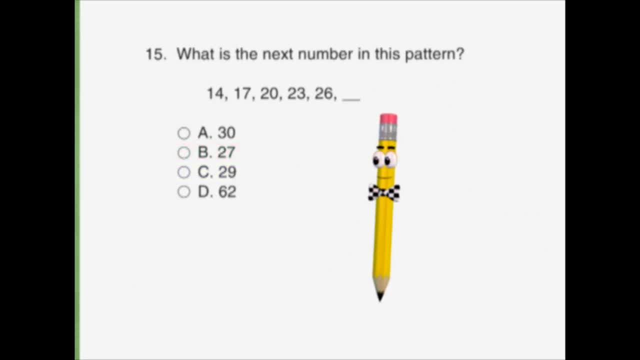 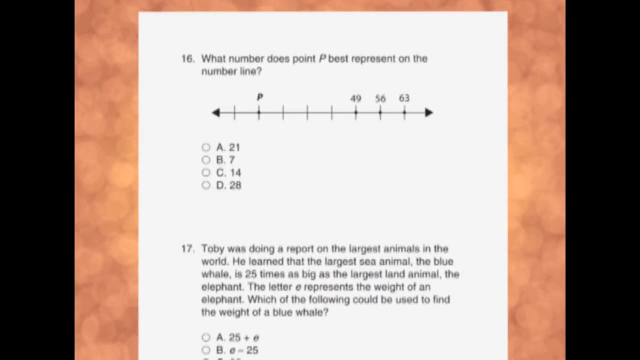 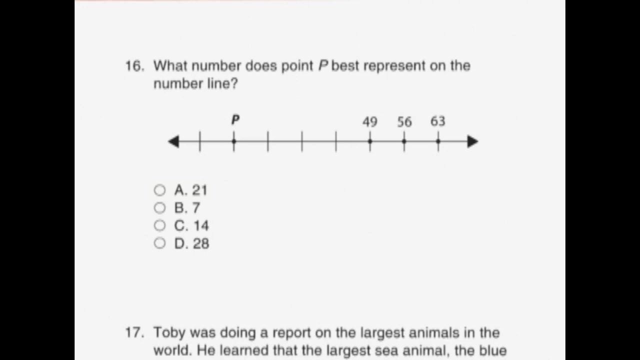 C twenty-nine, there's our answer, And D sixty-two is way off. The answer is C twenty-nine Sixteen. What number does point P best represent on the number line? A twenty-one, B seven. 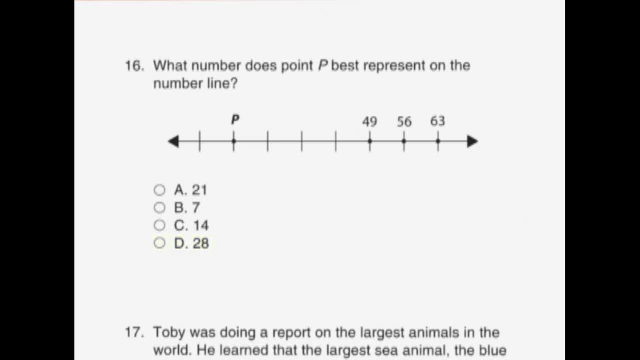 C, fourteen, D, twenty-eight. Let's look for the pattern. Fifty-six is seven less than sixty-three. Forty-nine is seven less than fifty-six. So we seem to be going down by seven as we move left on the number line. 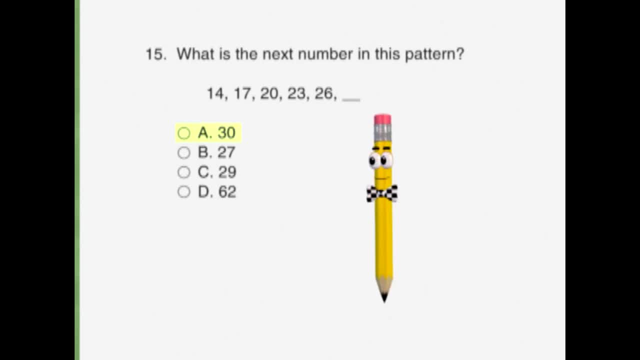 Let's see if that is in the answers: A 30.. No B 27.. Not that one: C 29.. There's our answer, And D 62 is way off. The answer is C 29.. 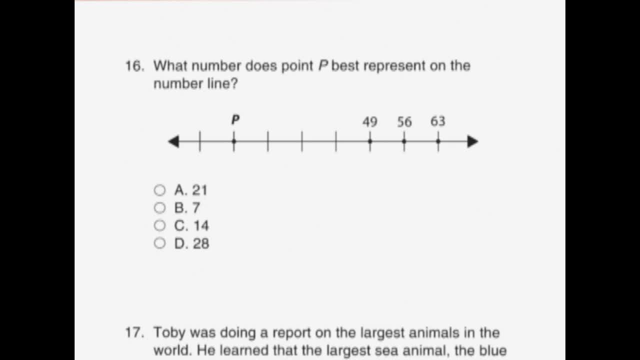 16. What number does point P best represent on the number line A 21. B 7. C 14. D 28.. Let's look for the pattern. 56 is 7, less than 63.. 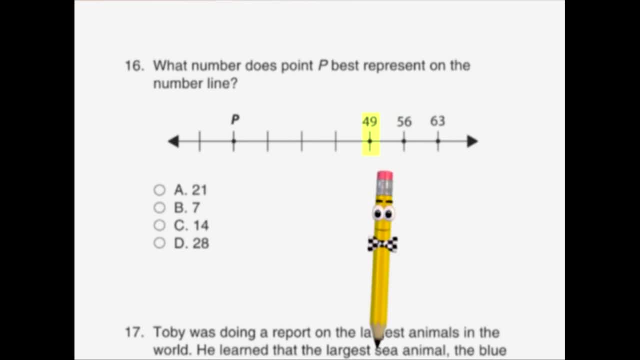 49 is 7 less than 56. So we seem to be going down by 7 as we move left on the number line. Let's fill in the numbers as we move down to point P: 42,, 35,, 28,, 21.. 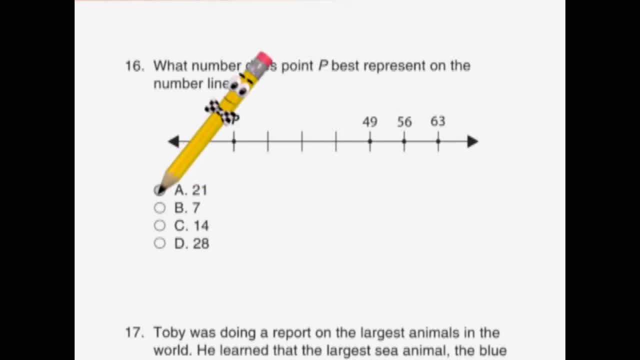 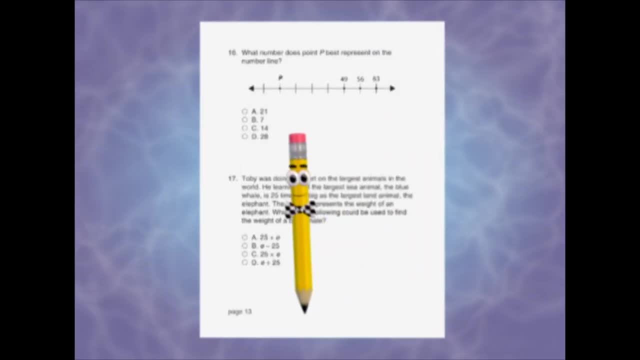 That's our answer. So choice A 21 is the correct answer. Sometimes it is helpful to write a number sentence when you are solving a problem. Let's do some examples 17.. Toby was doing a report on the largest animals in the world. 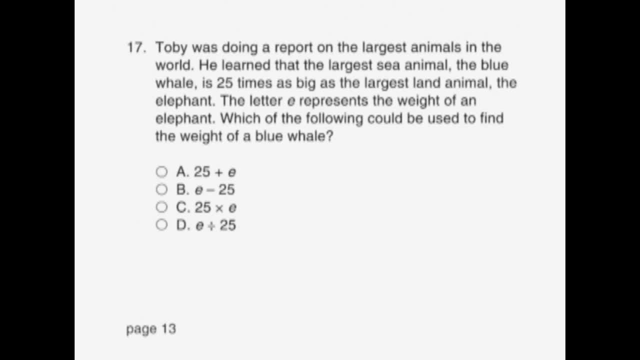 He learned that the largest sea animal, the blue whale, is 25 times as big as the largest land animal, the elephant. The letter E represents the weight of an elephant. Which of the following could be used to find the weight of a blue whale? 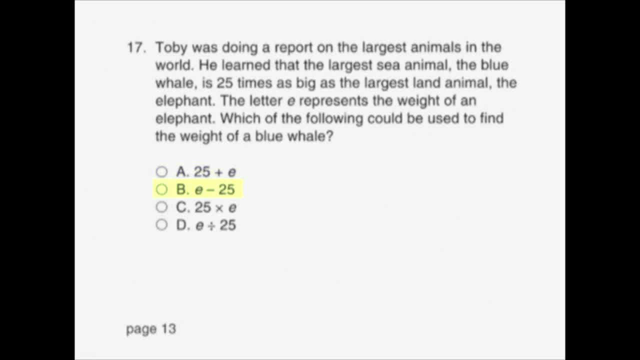 A 25 plus E, B, E minus 25.. C 25 times E, D, E divided by 25.. The blue whale is 25 times as large as the elephant Times means we need to multiply, And since E represents the elephant's weight, the answer is: 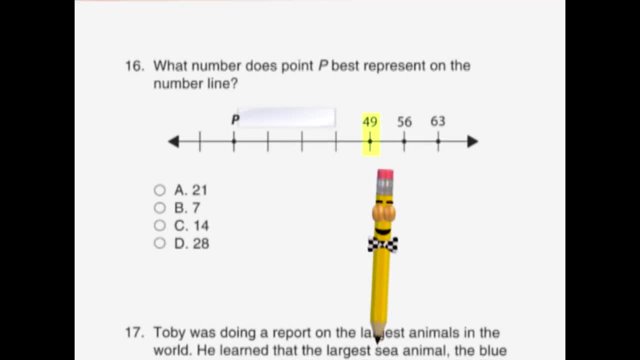 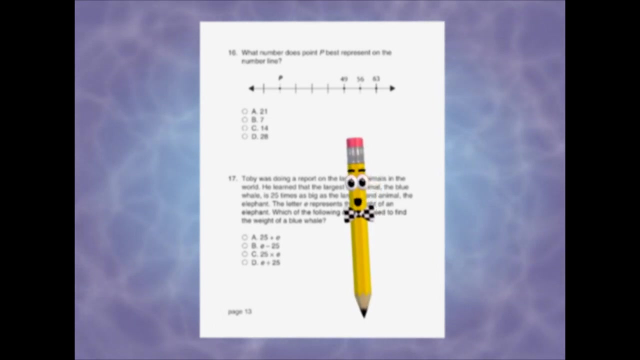 Let's fill in the numbers as we move down to point P. Forty-two, thirty-five, twenty-eight, twenty-one- That's our answer. So choice A, twenty-one, is the correct answer. Sometimes it is helpful to write a number sentence when you are solving a problem. 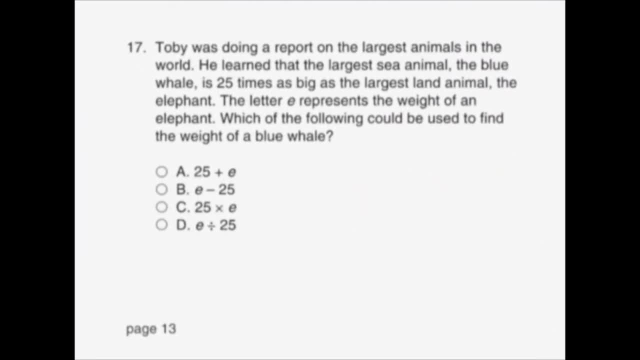 Let's do some examples. Seventeen Toby was doing a report on the largest animals in the world. He learned that the largest sea animal, the blue whale, is twenty-five times as big as the largest land animal, the elephant. The letter E represents the weight of an elephant. 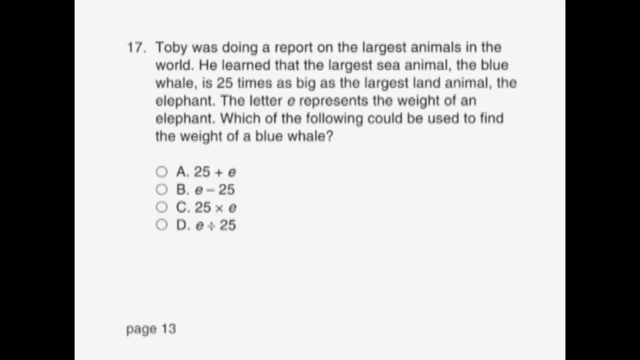 Which of the following could be used to find the weight of a blue whale: A- twenty-five plus E, B, E minus twenty-five, C- twenty-five times E, D, E divided by twenty-five, The blue whale is twenty-five times as large as the elephant. 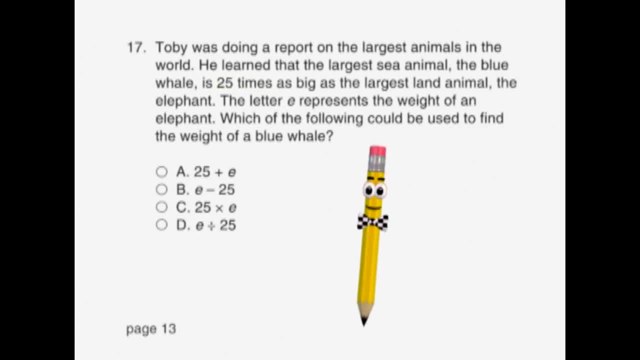 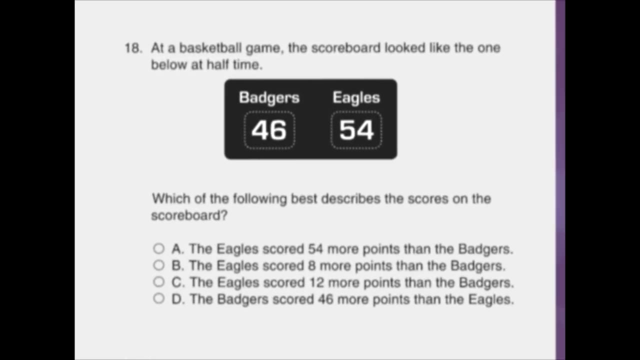 Times means we need to multiply, And since E represents the elephant's weight, the answer is C, twenty-five times E, Let's do another one: Eighteen. At a basketball game, the scoreboard looks like the one below: at halftime: 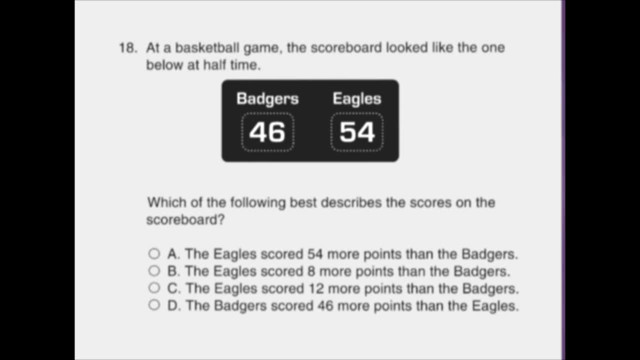 Badgers: forty-six. Eagles: fifty-four. Which of the following best describes the scores on the scoreboard A: the Eagles scored fifty-four more points than the Badgers. No, the Eagles only scored fifty-four points total, Not fifty-four points more than the Badgers. 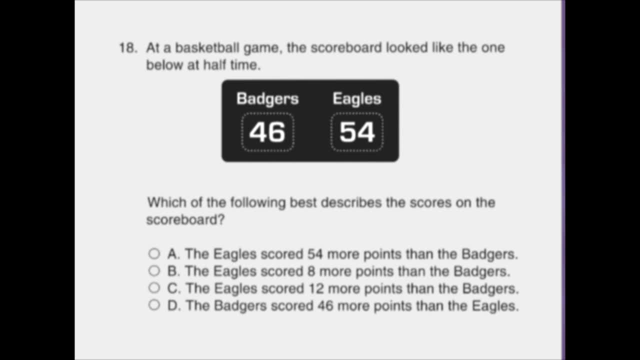 B, the Eagles scored eight more points than the Badgers. Fifty-four is only eight more than forty-six. We can find this by subtracting forty-six from fifty-four. This one looks like the correct answer, But let's check the other two answers just to be sure. 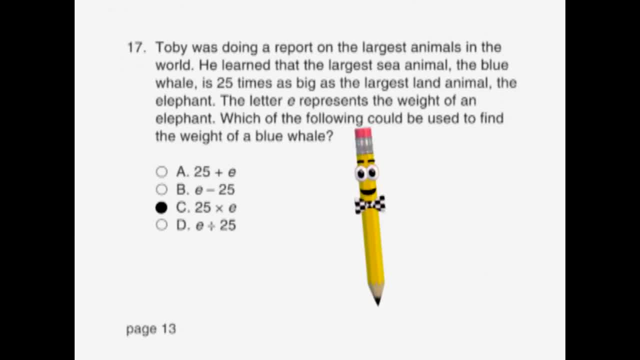 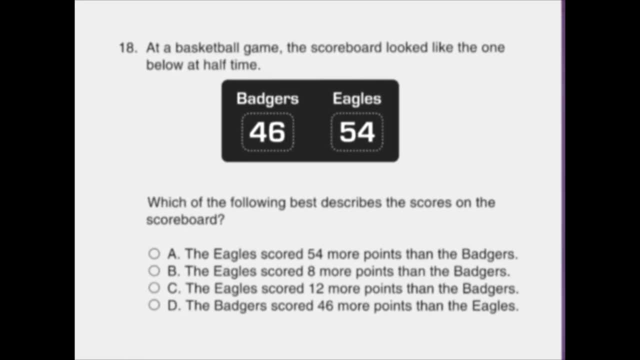 C 25 times E. Let's do another one: 18.. At a basketball game, the scoreboard looks like the one below: at halftime: Badgers 46.. Eagles 54.. Which of the following best describes the scores on the scoreboard? 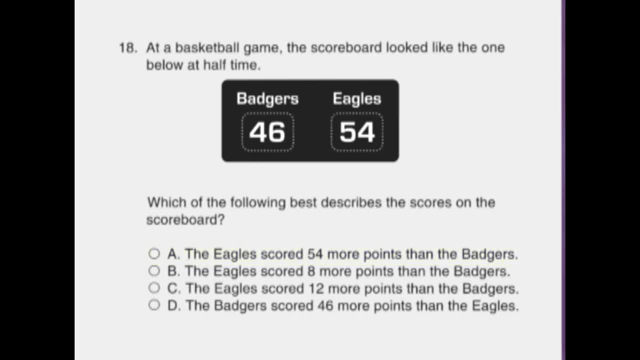 A: The Eagles scored 54 more points than the Badgers. No, the Eagles only scored 54 points total, not 54 points more than the Badgers. B: The Eagles scored 8 more points than the Badgers. 54 is only 8 more than 46.. 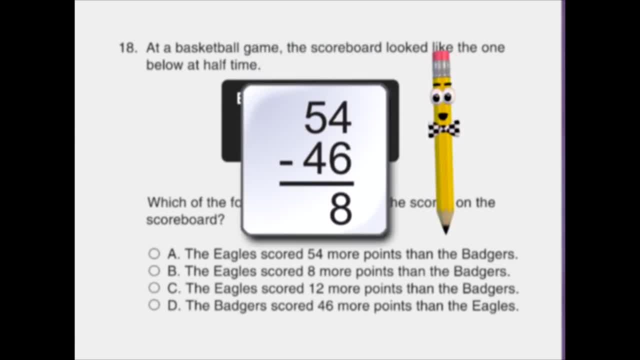 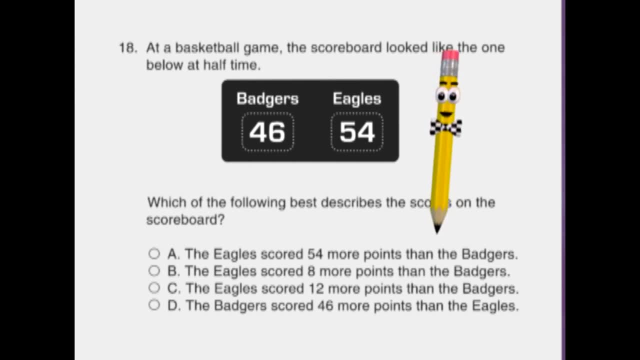 We can find this by subtracting 46 from 54.. This one looks like the correct answer, But let's check the other two answers just to be sure. C: The Eagles scored 12 more points than the Badgers. 46 plus 12 equals 58.. 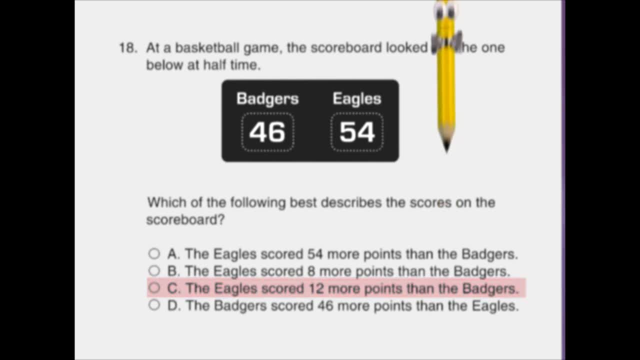 That's not the correct answer. D: The Badgers scored 46 more points than the Eagles. The Badgers scored 46 points total, but the Eagles scored 54. That's the higher score. So the correct answer is B: The Eagles scored 8 more points than the Badgers. 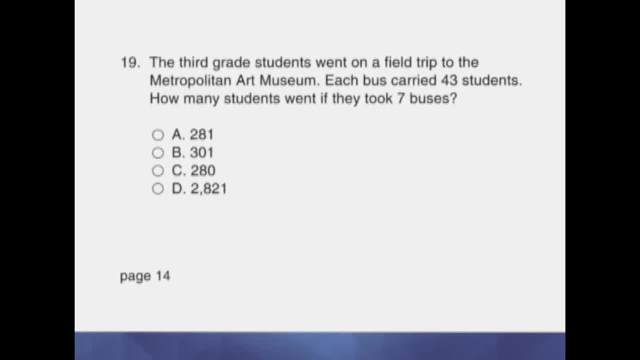 19. The third-grade students went on a field trip to the Metropolitan Art Museum. Each bus carried 43 students. How many students went if they took seven buses? A, 281, B, 301, C, 280, D, 2,821. 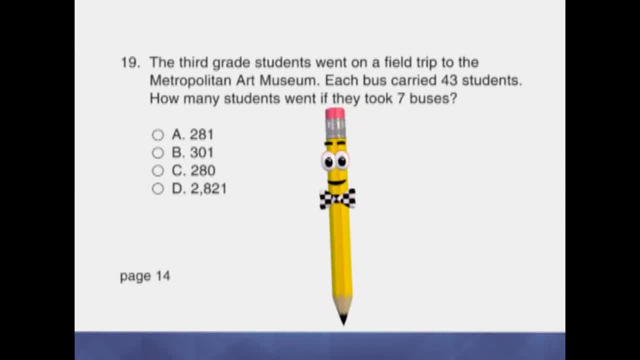 Since each of the seven buses will carry 43 students, the math sentence for this problem is 43 times 7.. We'll just work that out. Let's see: 7 times 3 is 21.. Put the 1 down here in the ones place. 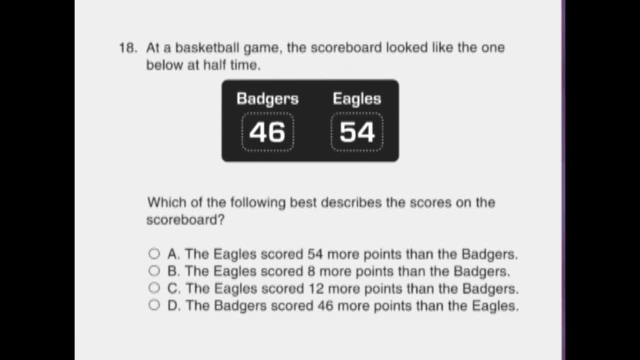 C: the Eagles scored twelve more points than the Badgers. Forty-six plus twelve equals fifty-eight. That's not the correct answer. D: the Badgers scored forty-six more points than the Eagles. The Badgers scored forty-six points total, but the Eagles scored fifty-four. 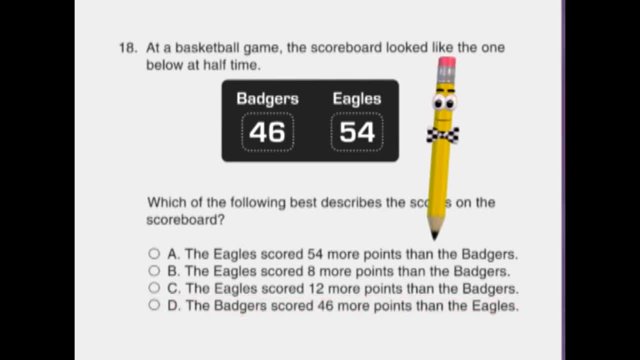 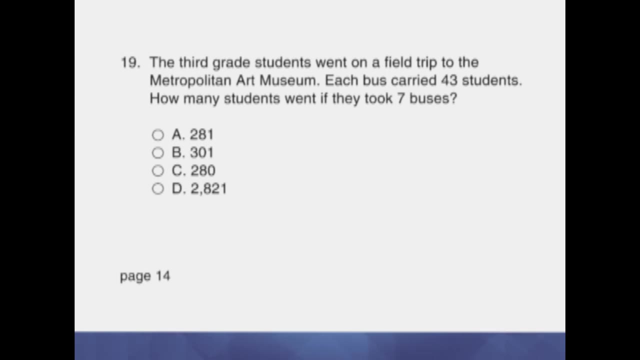 That's the higher score, So the correct answer is B. The Eagles scored eight more points than the Badgers Nineteen. The third grade students went on a field trip to the Metropolitan Art Museum. Each bus carried forty-three students. How many students went if they took seven buses? 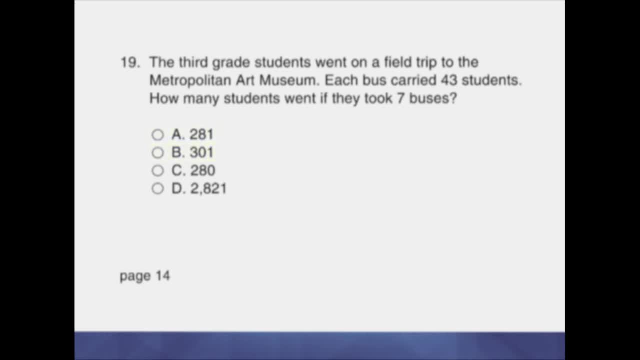 A. two hundred eighty-one, B. three hundred one, C. two hundred eighty. D. two thousand eight hundred twenty-one. Since each of the seven buses will carry forty-three students, the math sentence for this problem is forty-three times seven. 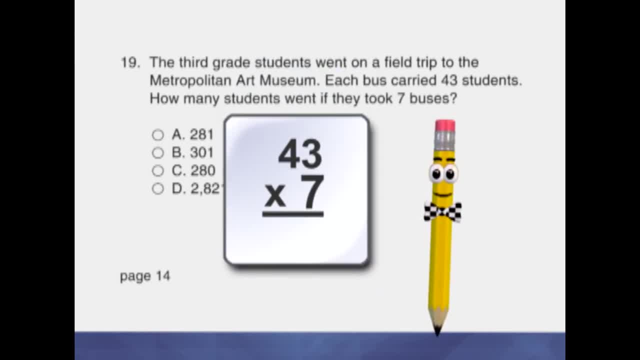 We'll just work that out. Let's see, Seven times three is twenty-one. Put the one down here in the ones place and write the two above the four. So we remember to add it. Now, seven times four is twenty-eight. 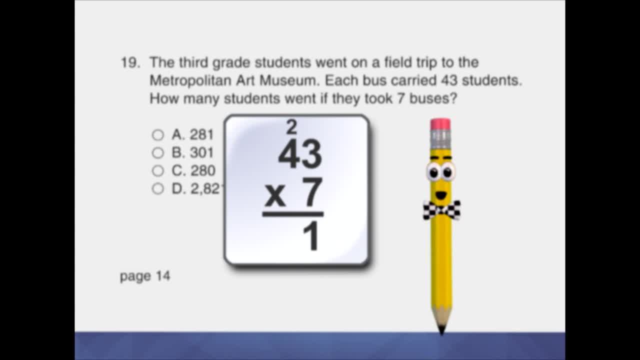 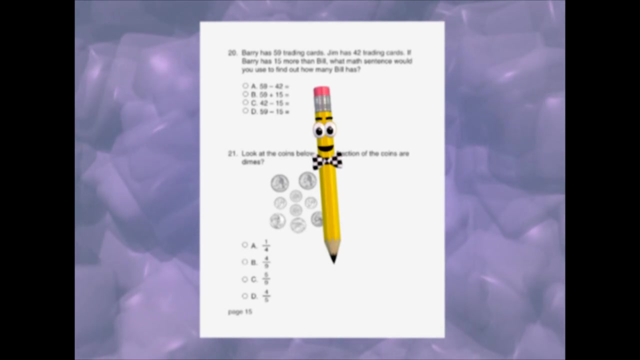 Adding our two gives us thirty. Write that down next to the one. The answer is three hundred one. That matches answer B. The correct answer is B three hundred one. Sometimes it is possible to look for extra information that is not needed and simplify the problem. 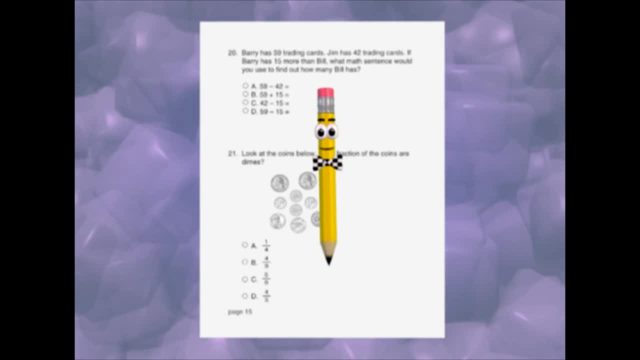 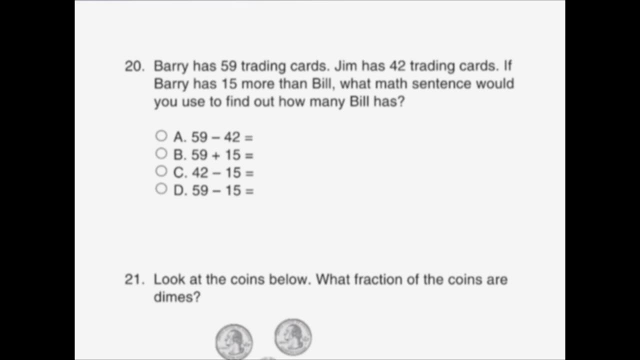 This can really help. Let me show you what I mean with this next problem. Twenty: Barry has fifty-nine trading cards. Jim has forty-two trading cards. If Barry has fifteen more than Bill, what math sentence would you use to find out how many Bill has? 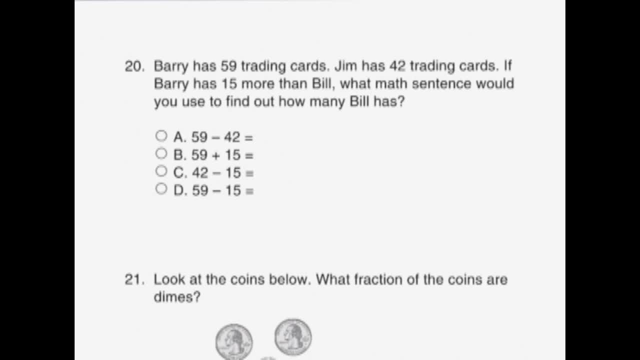 A. fifty-nine minus forty-two equals B. fifty-nine plus fifteen equals C. forty-two minus fifteen equals D. fifty-nine minus fifteen equals Jim's cards do not really matter. Ah, the question mentions both Bill and Barry. 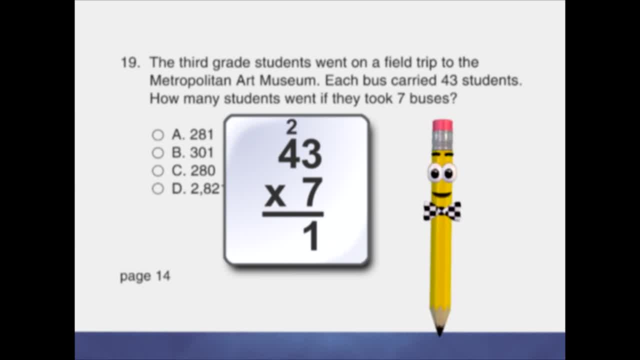 and write the 2 above the 4, so we remember to add it. Now, 7 times 4 is 28.. Adding our 2 gives us 30. Write that down next to the 1.. The answer is 301.. 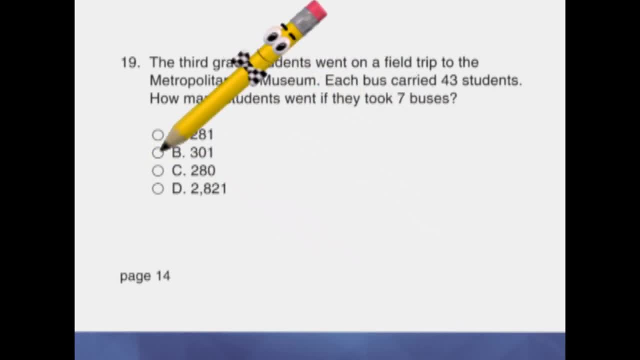 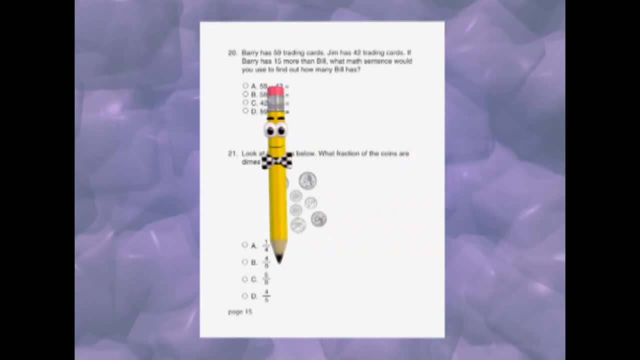 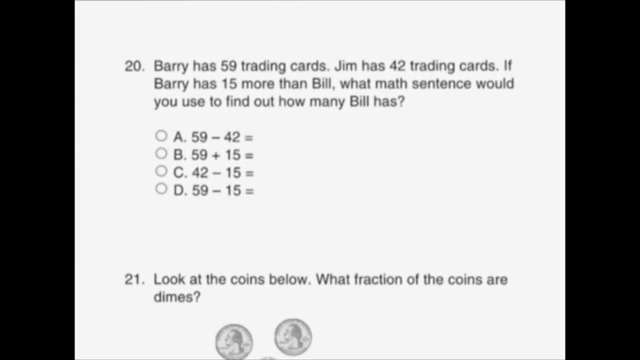 That matches answer B. The correct answer is B 301. Sometimes it is possible to look for extra information that is not needed and simplify the problem. This can really help. Let me show you what I mean with this next problem: 20.. Barry has 59 trading cards. 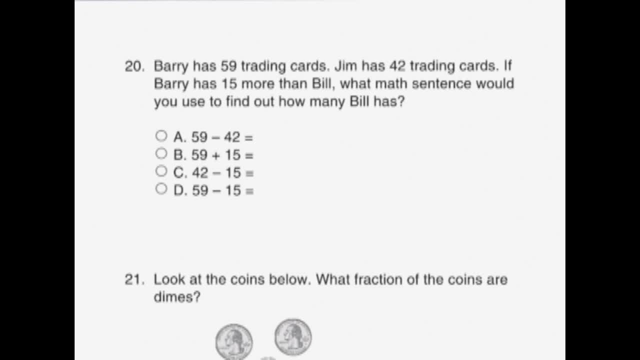 Jim has 42 trading cards. If Barry has 15 more than Bill, what math sentence would you use to find out how many Bill has? A? 59 minus 42 equals. B. 59 plus 15 equals C. 42 minus 15 equals. 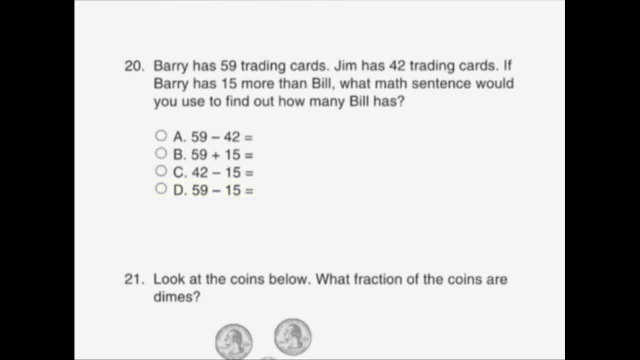 D 59 minus 15 equals Jim's cards do not really matter. Ah, the question mentions both Bill and Barry. Now Barry has 15 more cards than Bill, So Bill has 15 fewer cards than Barry. We should subtract 15 from the 59 cards Barry has. 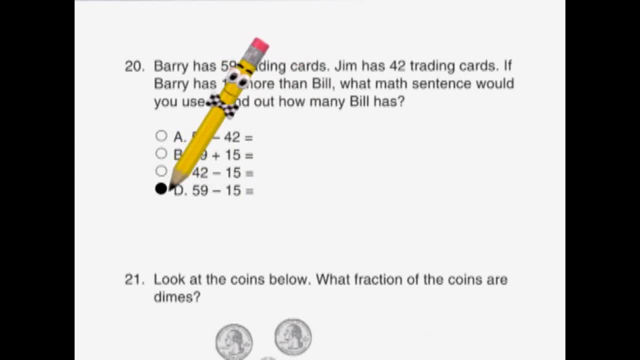 So the answer is D 59 minus 15 equals. But, Marco, what about answer B 59 plus 15 equals? Answer B 59 plus 15 equals is wrong. It might be easy to think we should add. 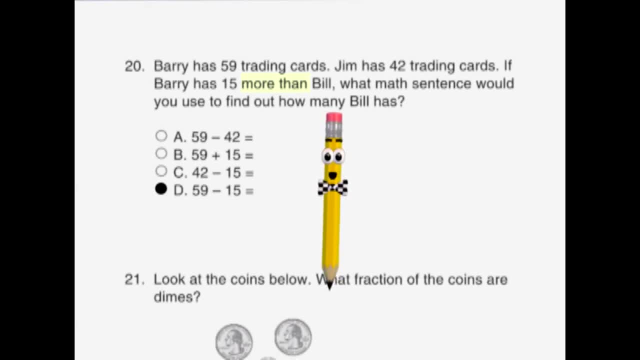 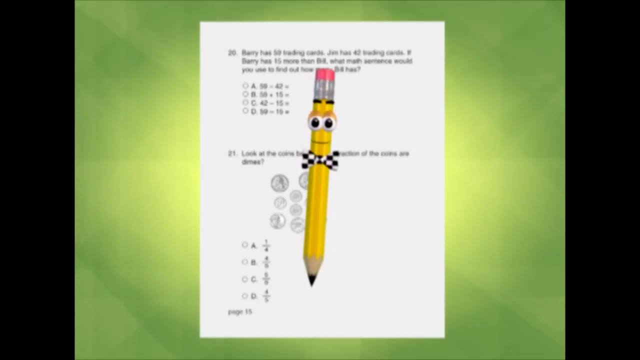 because of the words more than in the question, But it is important to pay attention to who has more cards, and in this case it is Barry, not Bill. Another strategy is to divide the problem into smaller, simpler problems. 21. Look at the coins below. 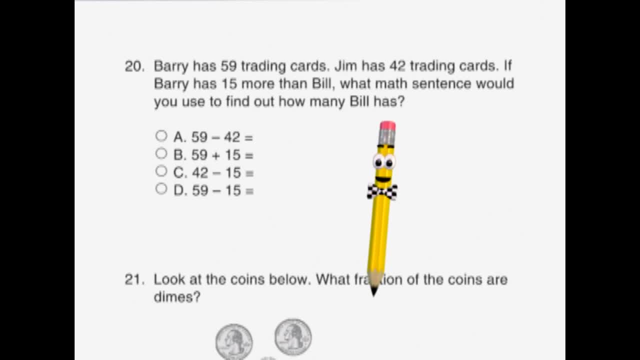 Now Barry has fifteen more cards than Bill, So Bill has fifteen fewer cards than Barry. We should subtract fifteen from the fifty-nine cards Barry has. So the answer is D: fifty-nine minus fifteen equals. But, Marco, what about answer B? 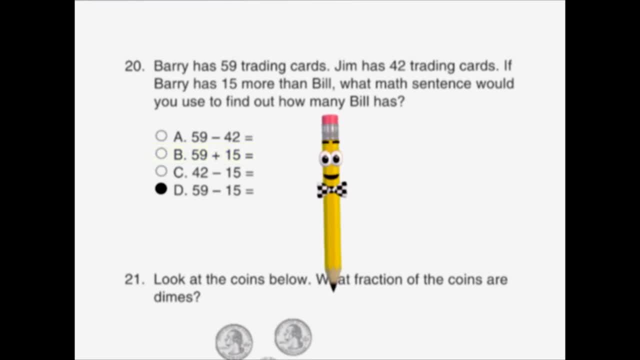 Fifty-nine plus fifteen equals. Answer B: fifty-nine plus fifteen equals is wrong. It might be easy to think we should add because of the words than in the question, But it is important to pay attention to who has more cards, and in this case. 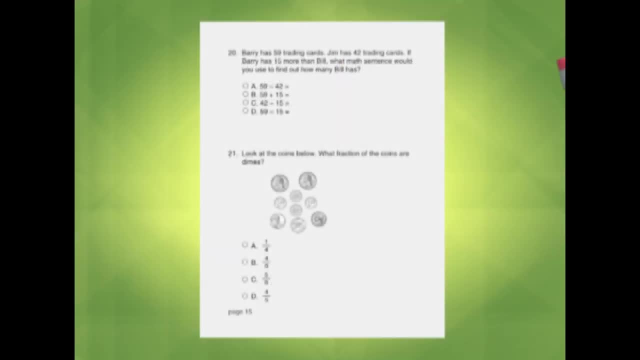 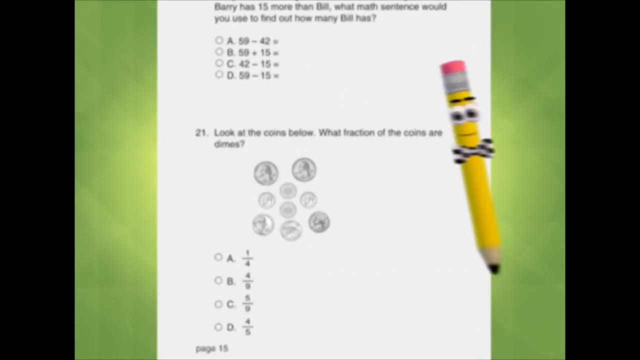 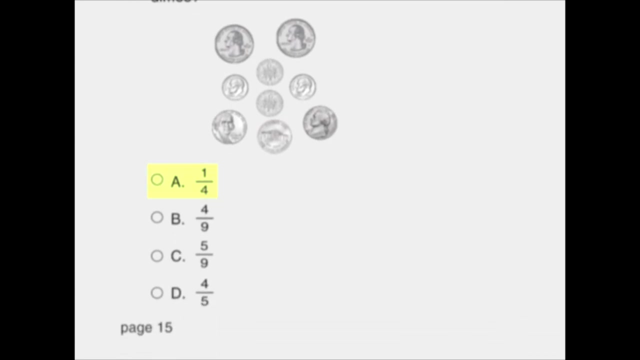 it is Barry, not Bill. Another strategy is to divide the problem into smaller, simpler problems. Twenty-one: Look at the coins below. What fraction of the coins are dimes? A, one-fourth, B, four-ninths. 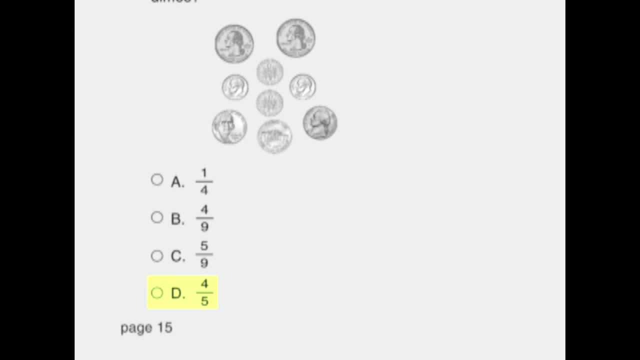 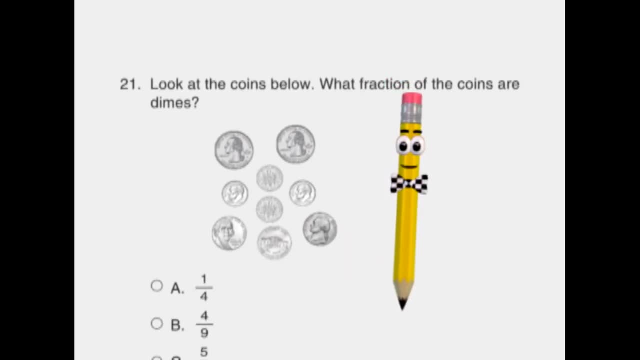 C, five-ninths, D, four-fifths. I always give a little nod to questions about fractions. Nod, Why do you say that? Because nod helps me remember N-O-D, or numerator over denominator. Now, since this is a question, 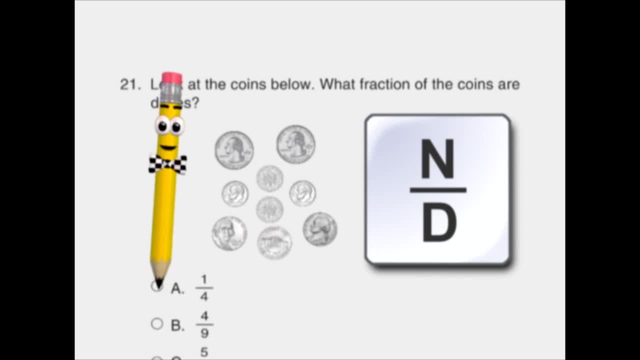 about a fraction of a group. we'll need to find two pieces of information: The number in the group to give us the denominator, and the number of pieces we are looking at to get the numerator. The group in this problem is coins. We have one, two, three, four. 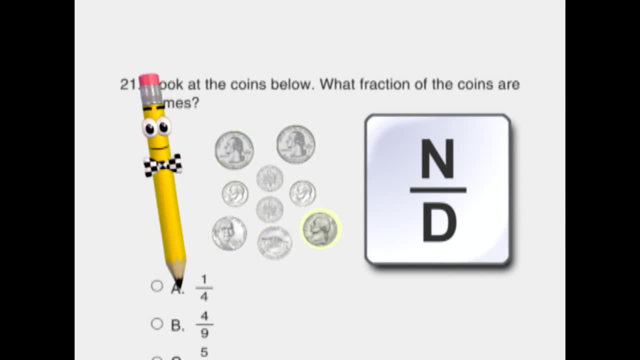 five, six, seven, eight, nine coins. that will be our denominator, And we have one, two, three, four dimes. So the fraction of dimes in our group of coins is four over nine. Four-ninths? The answer is: 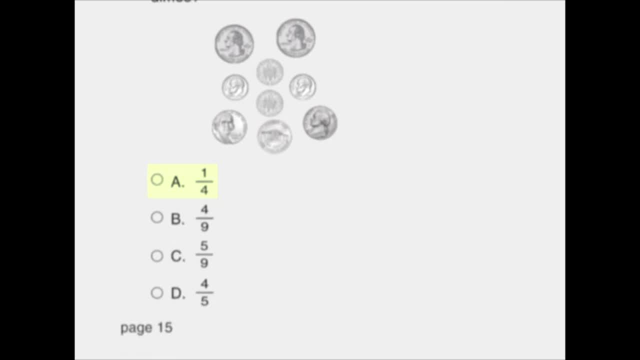 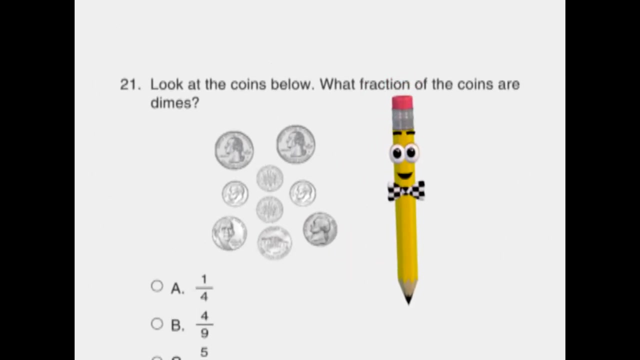 What fraction of the coins are dimes A, 1 fourth, B, 4 ninths, C, 5 ninths, D, 4 fifths? I always give a little nod to questions about fractions. Nod, Why do you say that? 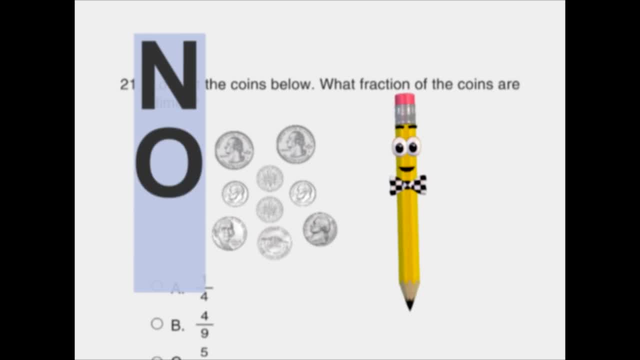 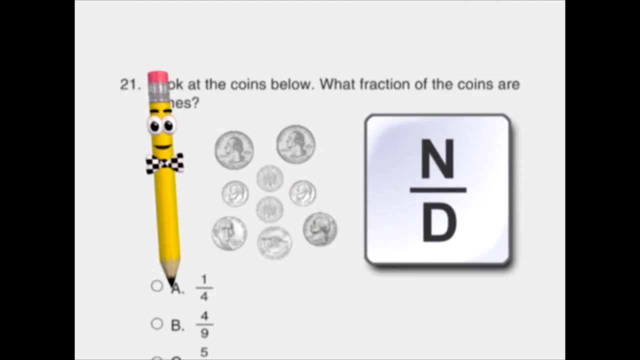 Because nod helps me remember N-O-D, or numerator over denominator. Now, since this is a question about a fraction of a group, we'll need to find two pieces of information: The number in the group to give us the denominator, and the number of pieces we are looking at to get the numerator. 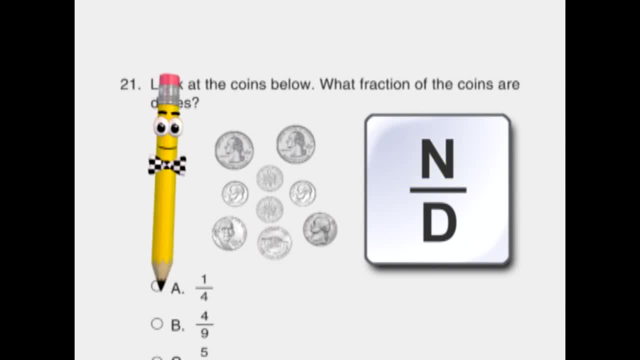 The group in this problem is coins. We have 1, 2, 3, 4, 5, 6, 7, 8, 9 coins That will be our denominator, And we have 1, 2, 3, 4 dimes. 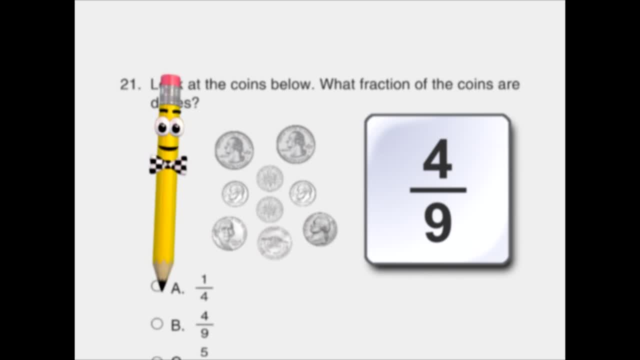 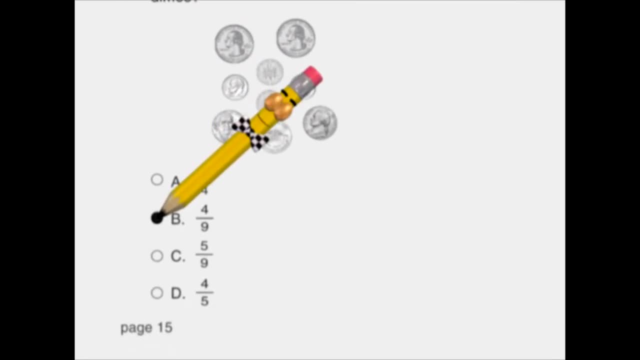 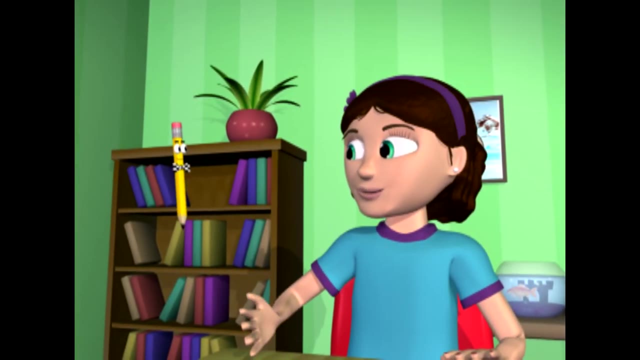 So the fraction of dimes in our group of coins is 4 over 9.. 4 ninths. The answer is B 4 ninths. I have a mystery for you to solve that's not. on the test, A nickel and a dime were rolling across a bridge. 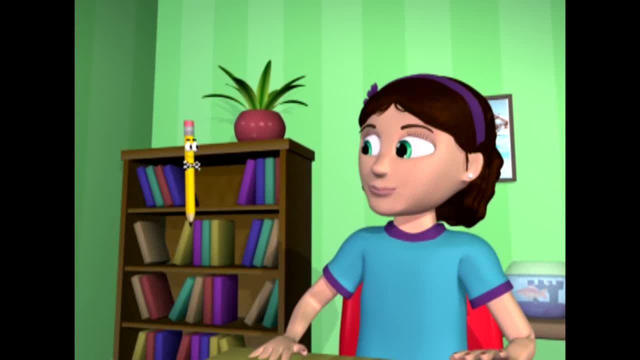 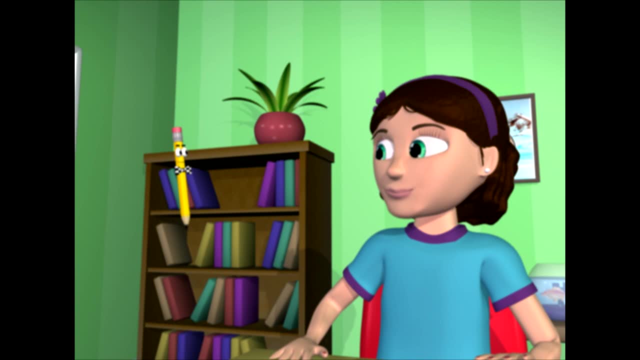 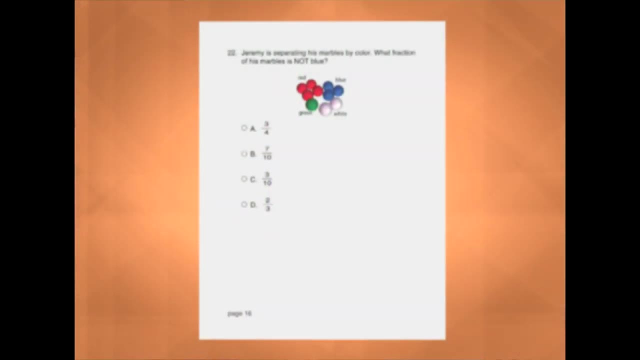 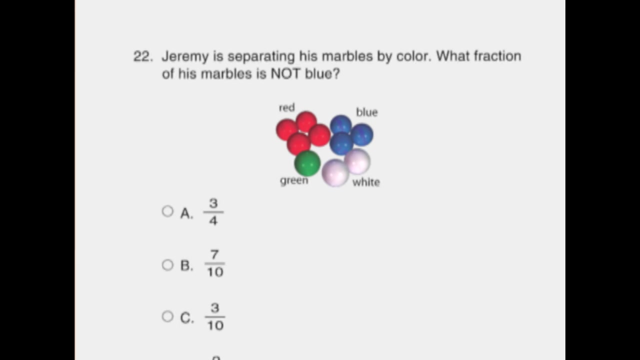 All of a sudden, the nickel fell off. Why? Okay tell me, Because the dime had more cents. That was funny. Let's move on to the next one, 22. Jeremy is separating his marbles by color. What fraction of his marbles is not blue? 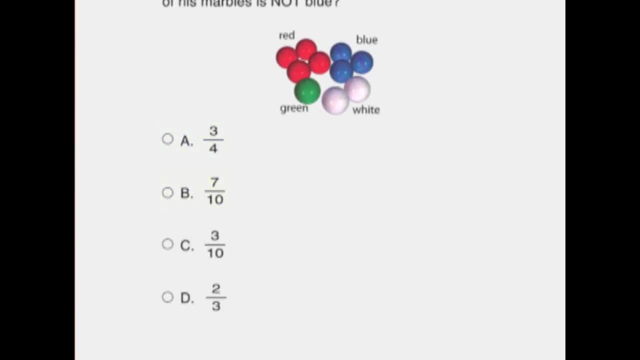 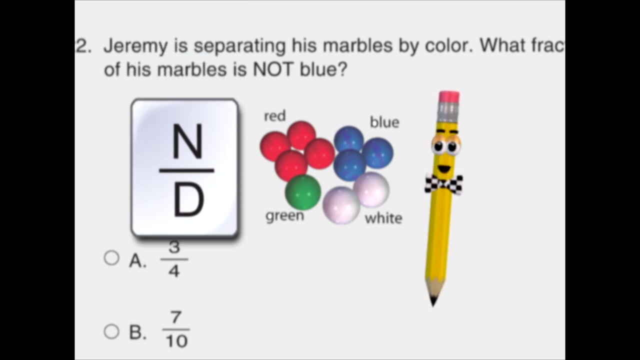 A- 3 fourths, B- 7 tenths, C, 3 tenths, D, 2 thirds. This is very much like the one we just did. First, let's add the marbles together to get our denominator. 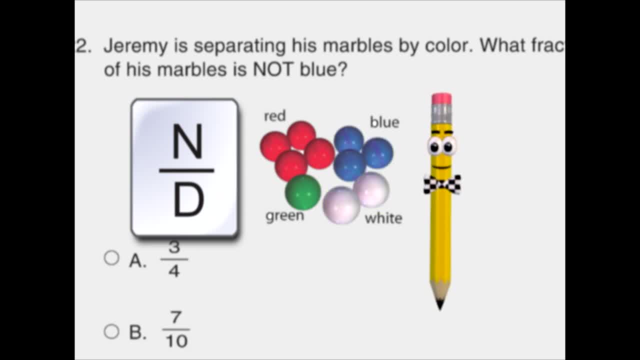 3 plus 2 is 5.. Add 4 and we get 9.. Add one more for 10 marbles. total, The denominator is 10.. But we want to know the fraction of marbles that are not blue, So the numerator will be all of the other marbles added together. 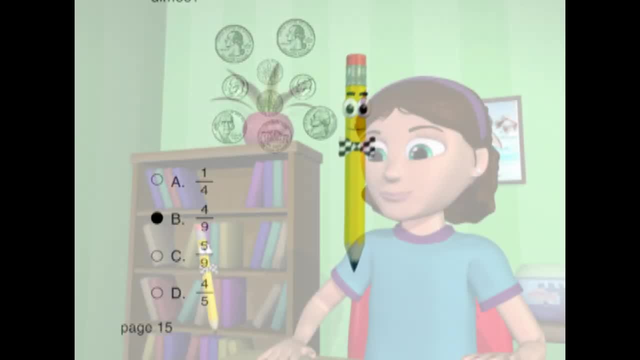 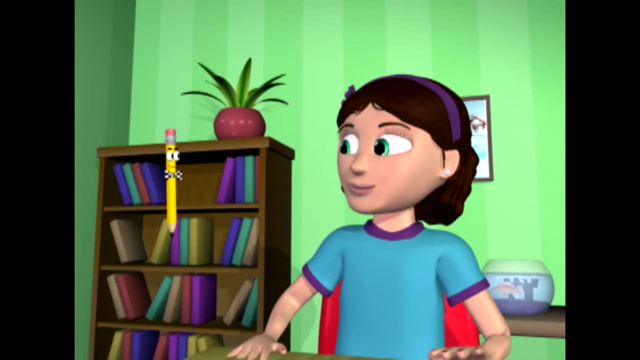 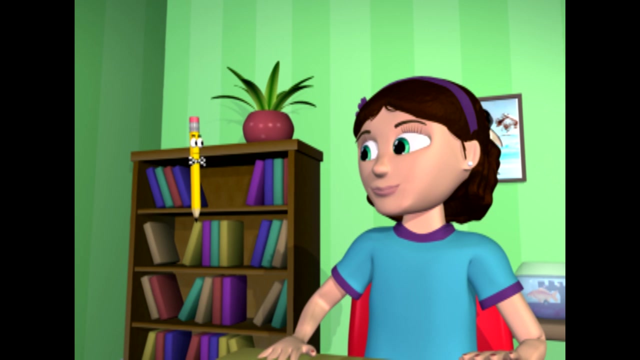 B four-ninths, I have a mystery for you to solve that's not on the test. A nickel and a dime were rolling across a bridge. All of a sudden, the nickel fell off. Why, Okay, tell me, Because the dime had more cents. 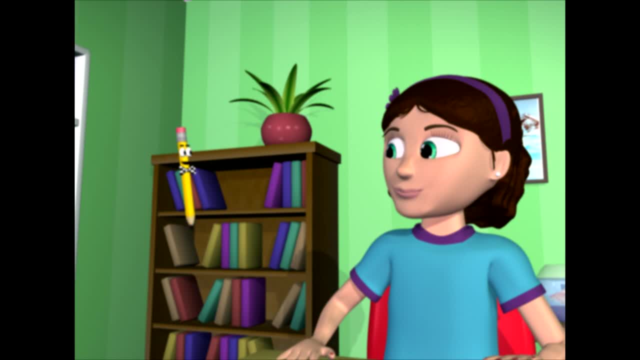 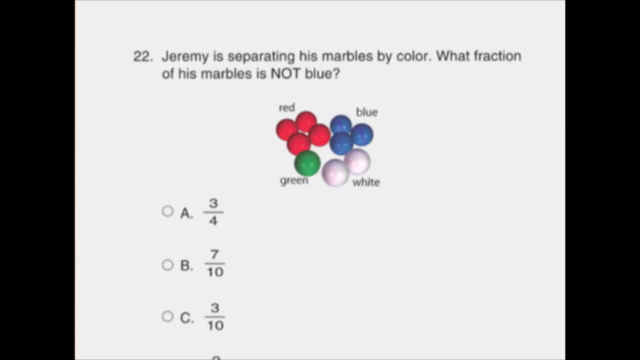 That was funny. Let's move on to the next one. Twenty-two, Jeremy is separating his marbles by color. What fraction of his marbles is not blue? A, three-fourths, B, seven-tenths, C, three-tenths. 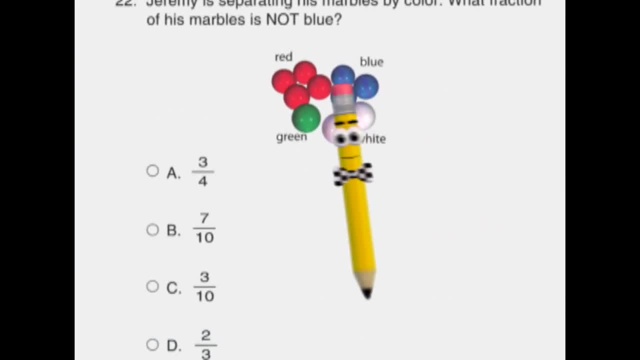 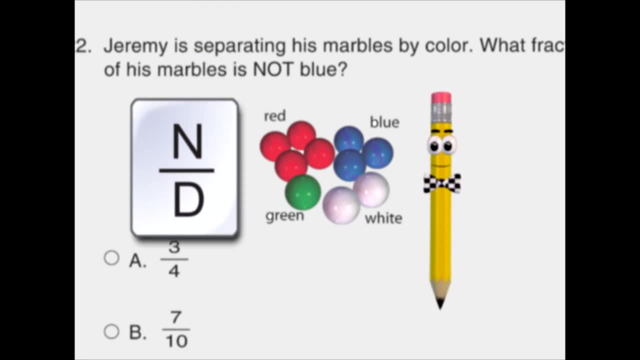 D two-thirds. This is very much like the one we just did. First. let's add the marbles together to get our denominator. Three plus two is five. Add four and we get nine. Add one more for ten marbles total. 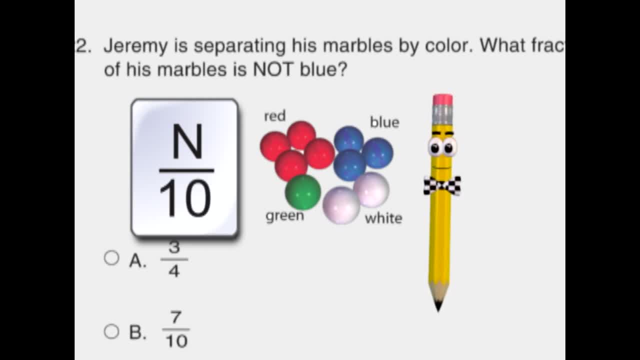 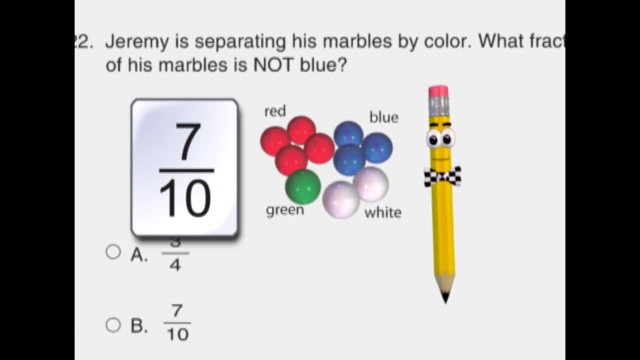 The denominator is ten, But we want to know the fraction of marbles that are not blue. So the numerator will be all of the other marbles added together, One plus four plus two, which is seven. So our answer is B seven-tenths. 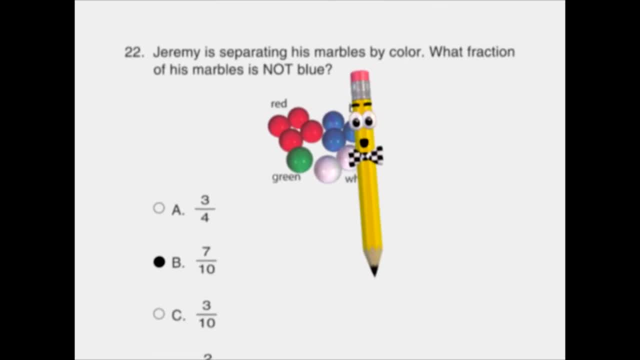 Notice that if we had not read our question carefully and paid close attention to the word not, then we might have chosen C and gotten the wrong answer. Now, let's do this. Let's look at the question that we have for you, Question number twenty-three. 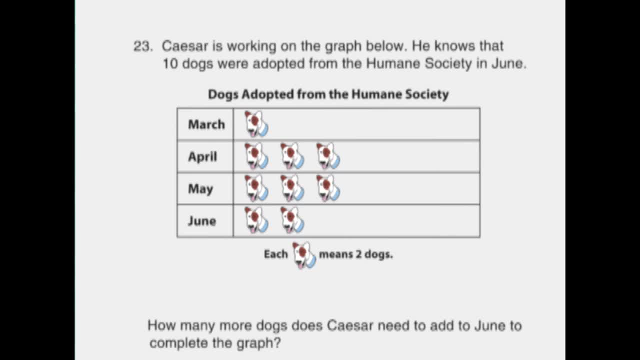 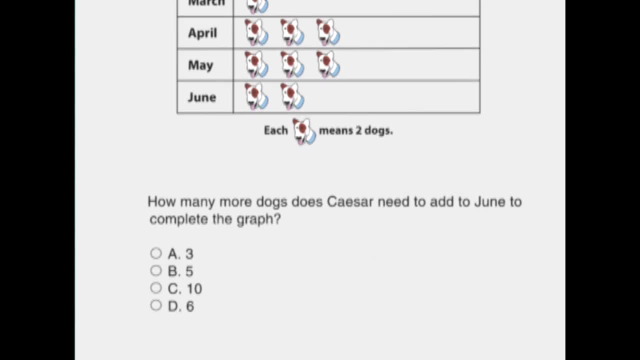 Caesar is working on the graph below. He knows that ten dogs were adopted from the Humane Society in June. How many more dogs does Caesar need to add to June to complete the graph? A, three, B, five, C, ten? 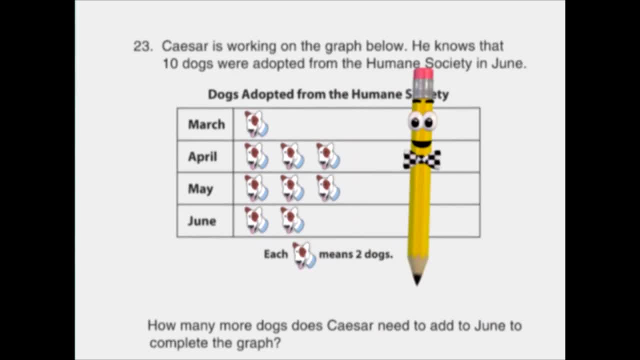 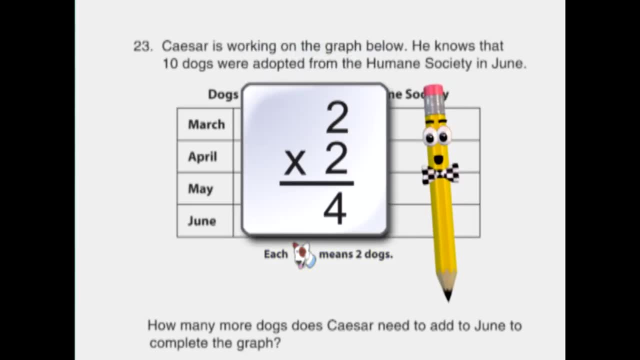 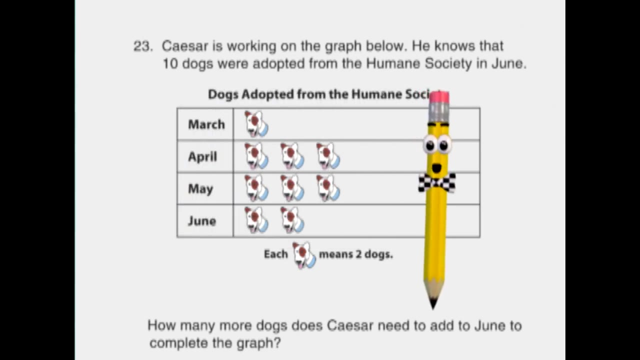 D six. Each dog picture stands for two dogs. We have two already. Two times two is four dogs shown, But we need to show ten. Ten minus four is six, So we have six more dogs to show on the graph. But remember that each dog picture shows two dogs. 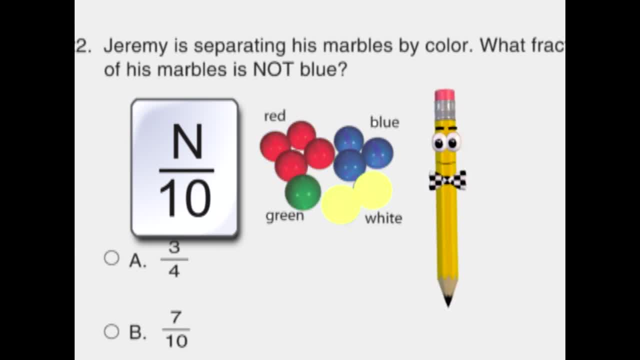 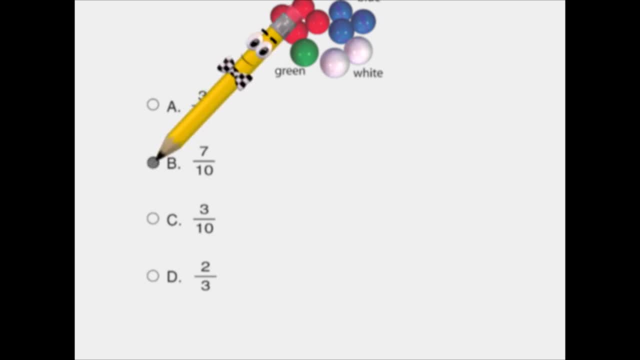 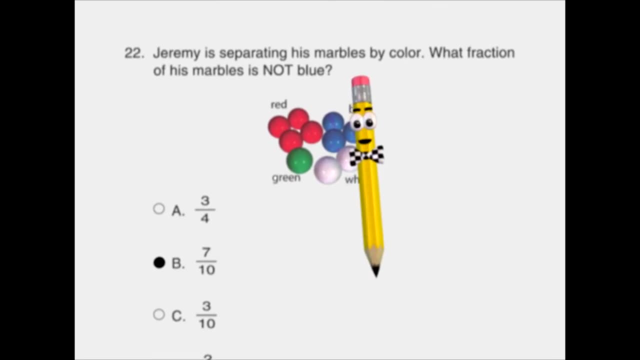 1 plus 4 plus 2, which is 7.. So our answer is B, 7 tenths. Notice that if we had not read our question carefully and paid close attention to the word NOT, then we might have chosen C and gotten the wrong answer. 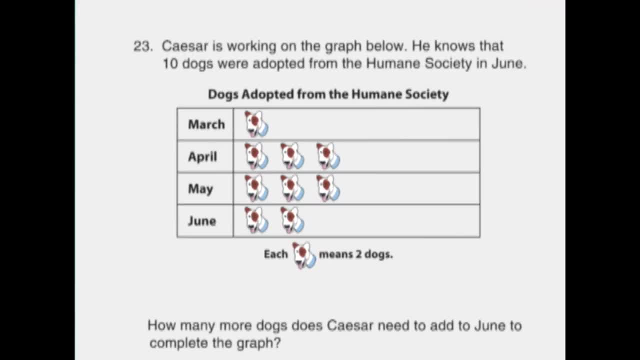 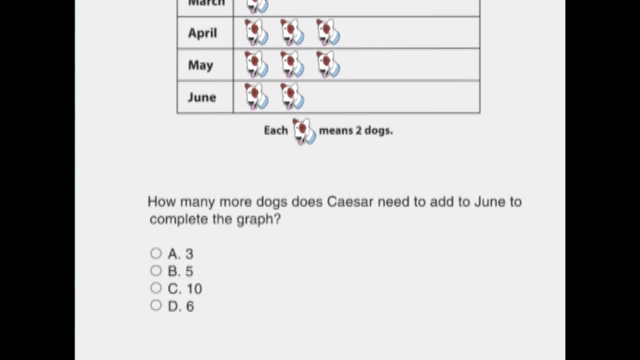 23.. Cesar is working on the graph below. He knows that 10 dogs were adopted from the Humane Society in June. How many more dogs does Cesar need to add to June to complete the graph? A, 3, B, 5. 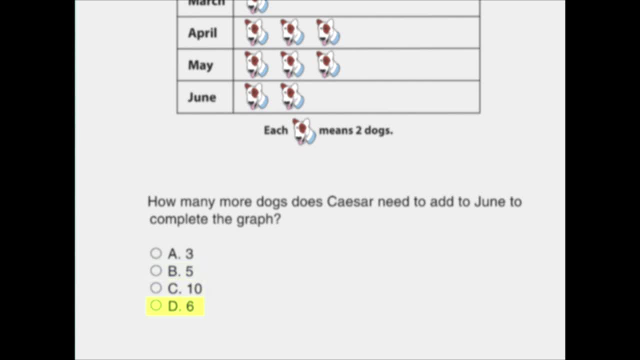 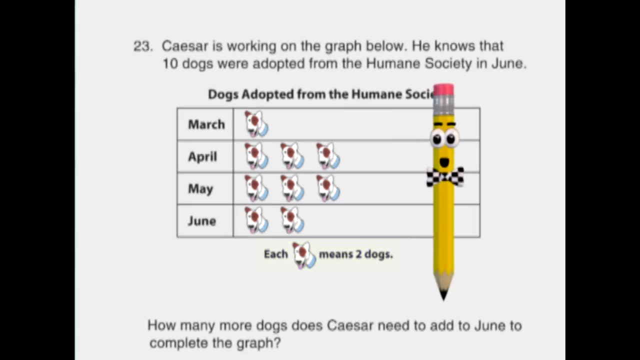 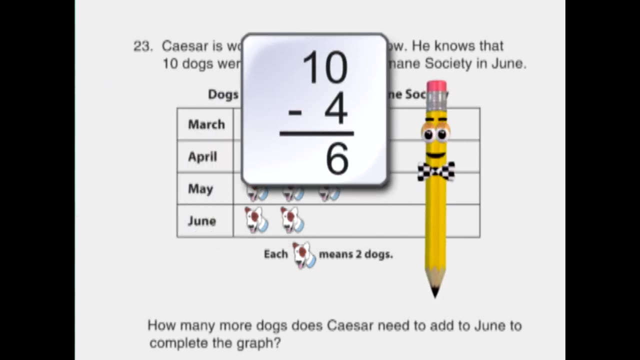 C, 10, D, 6. Each dog picture stands for 2 dogs. We have 2 already. 2 times 2 is 4 dogs shown, But we need to show 10.. 10 minus 4 is 6.. 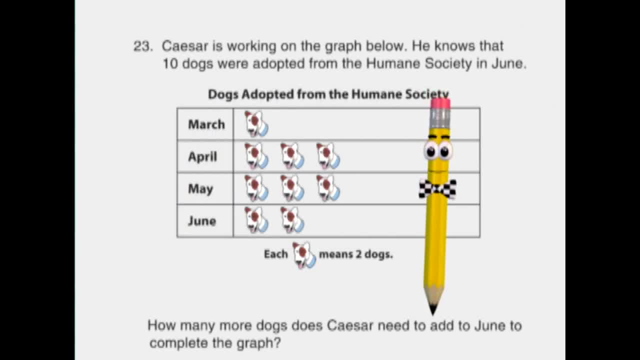 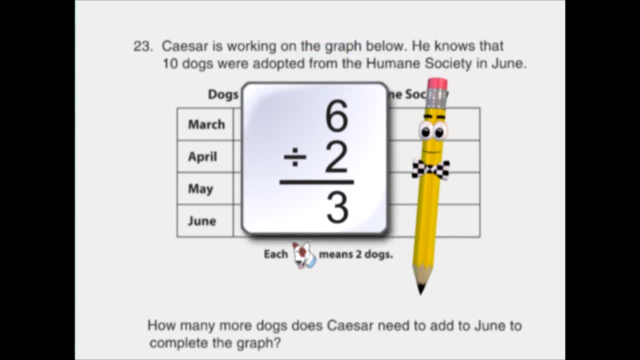 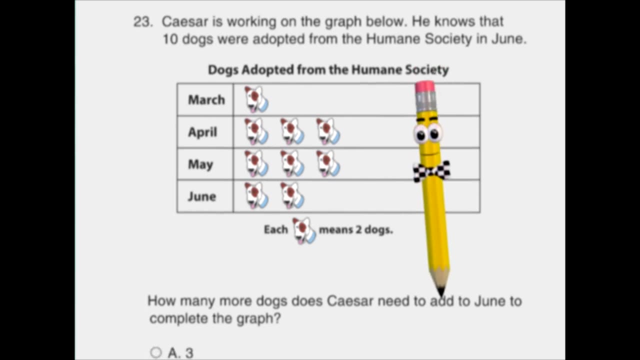 So we have 6 more dogs to show on the graph. But remember that each dog picture shows 2 dogs. That means we need to divide 6. divided by 2 equals 3.. We need 3 more puppy dog pictures. That's answer A. 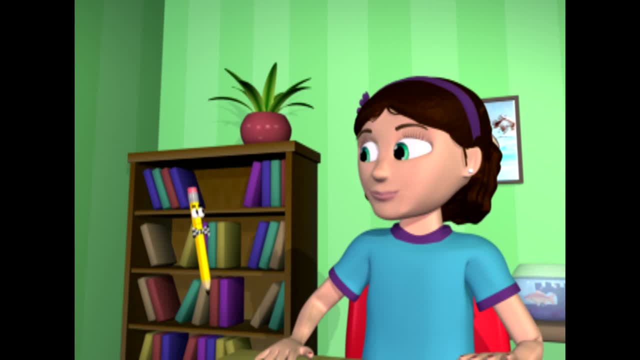 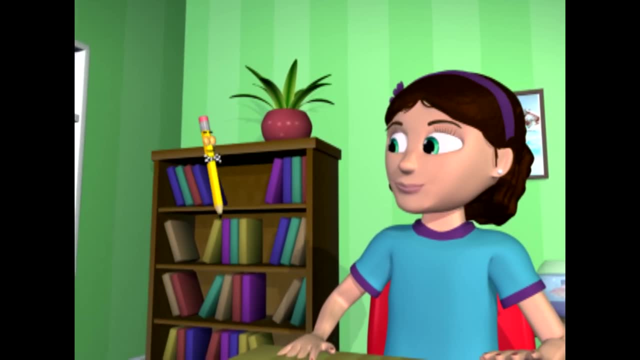 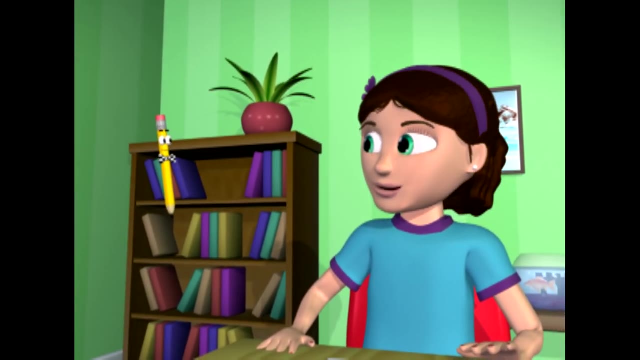 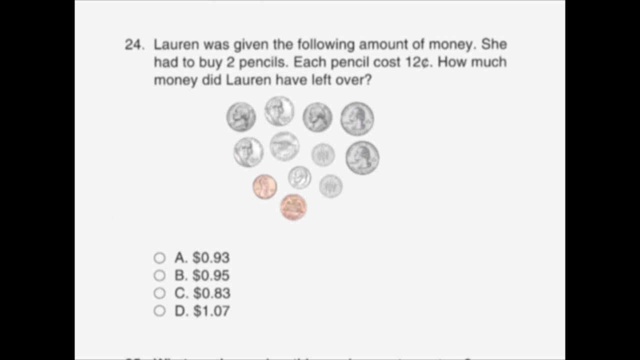 3. Say you're really good at problems with graphs. It's easy when you're a pencil filled with graphite, Get it Graphite, Graphite. Oh my Moving on 24.. Lauren was given the following amount of money: 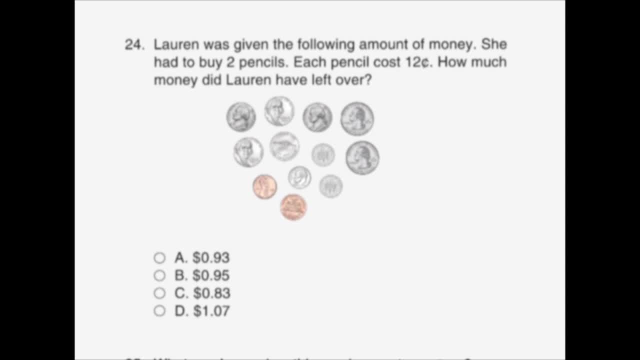 She had to buy 2 pencils. Each pencil cost 12 cents. How much money did Lauren have left over? A, 93 cents, B, 95 cents, C, 83 cents, D, 1 dollar and 7 cents. This one also has several steps. 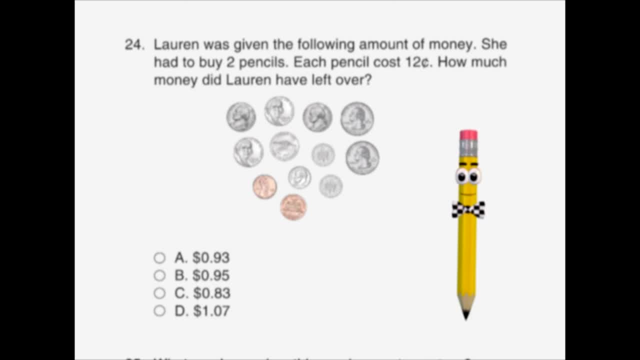 First let's find out how much money Lauren has: 25, 50, 60, 70, 80, 85, 90, 95. 1 dollar. 1 dollar 5 cents. 1 dollar 6 cents. 1 dollar 7 cents. Let's write that down. 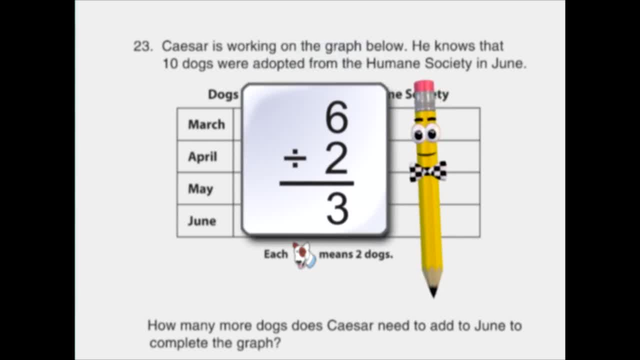 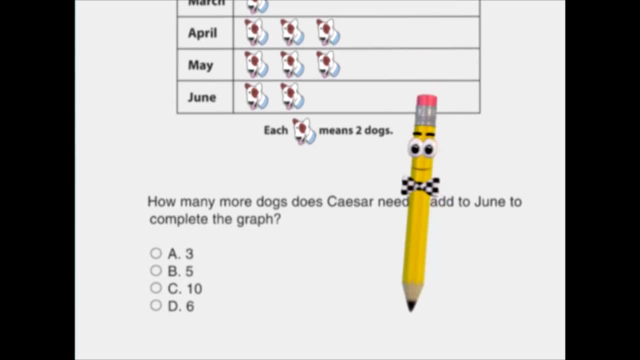 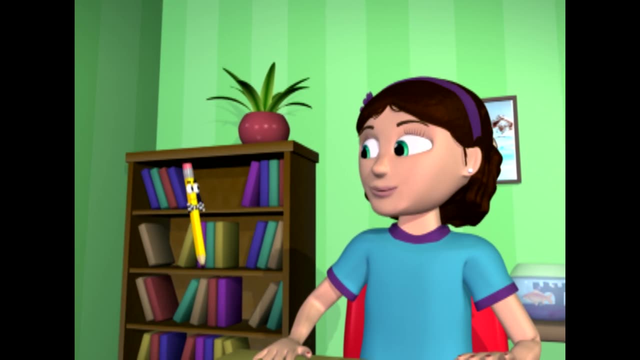 That means we need to divide Six. divided by two equals three. We need three more puppy dog pictures. That's answer. A three Say you're really good at problems with graphs. It's easy when you're a pencil filled with graphite. 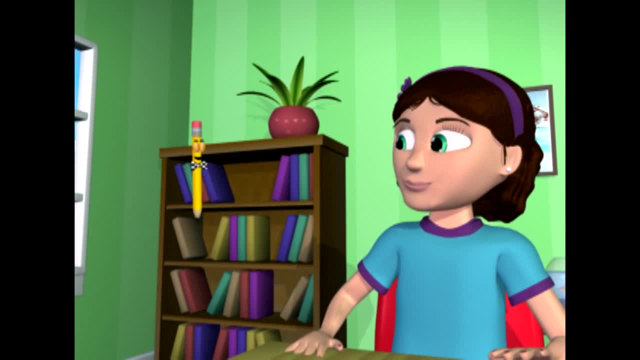 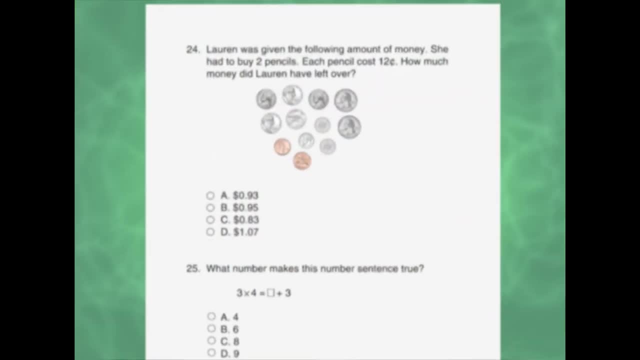 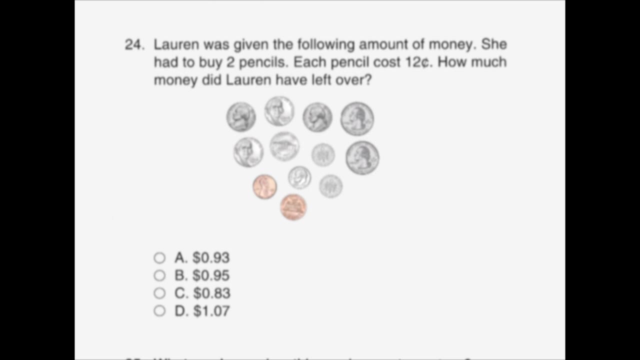 Get it Graphite, graph-ite. Oh, my Moving on. Twenty-five, Twenty-six, Twenty-four. Lauren was given the following amount of money: She had to buy two pencils. Each pencil cost 12 cents. How much money did Lauren have left over? 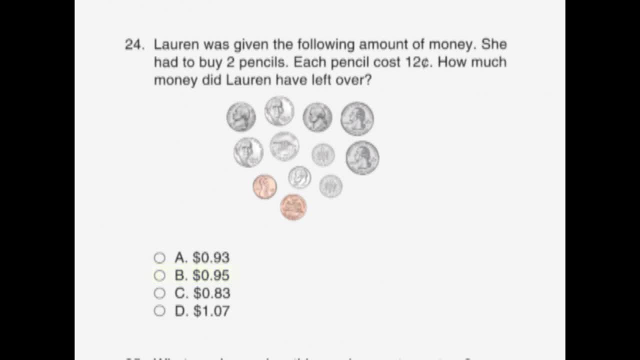 A, 93 cents B, 95 cents C, 83 cents D- $1.07.. This one also has several steps. This one also has several steps. First, let's find out how much money Lauren has. 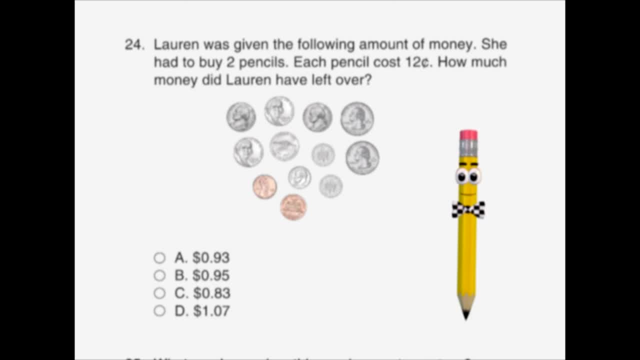 First let's find out how much money Lauren has: 25. 25. 50., 50., 60., 60., 70., 70., 80., 80., 85., 85., 90.. 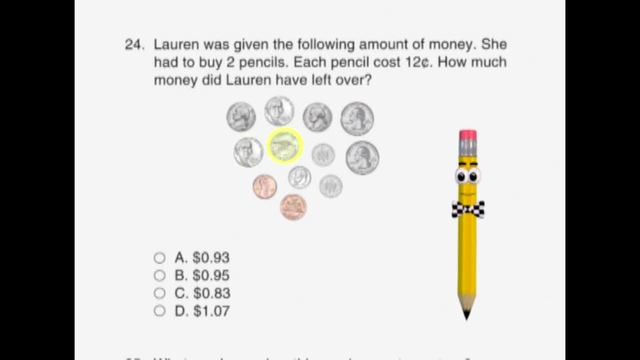 90.. 95.. 95.. $1.. $1.05., $1.05., $1.06., $1.06., $1.07.. Whew, Let's write that down. Now let's find out how much Lauren spent. 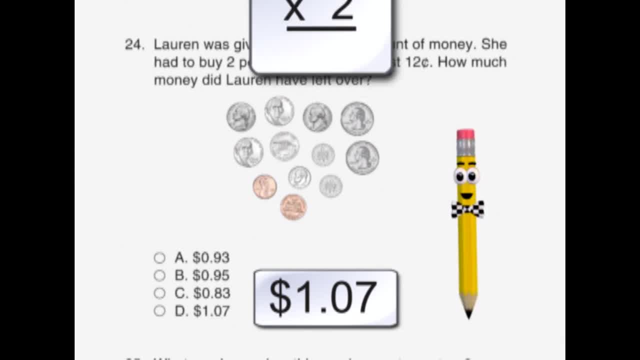 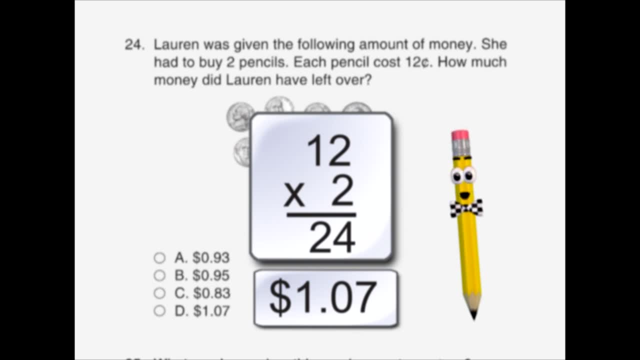 Now let's find out how much Lauren spent. How much Lauren spent? 2 pencils cost 12 cents each. 2 times 12 equals 24.. 2 times 12 equals 24.. Finally, we'll subtract what Lauren spent from the money she had to start. 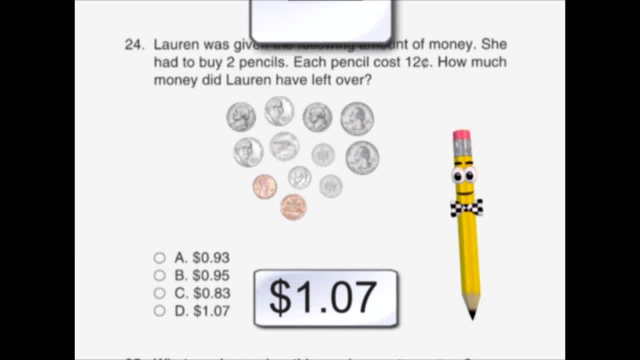 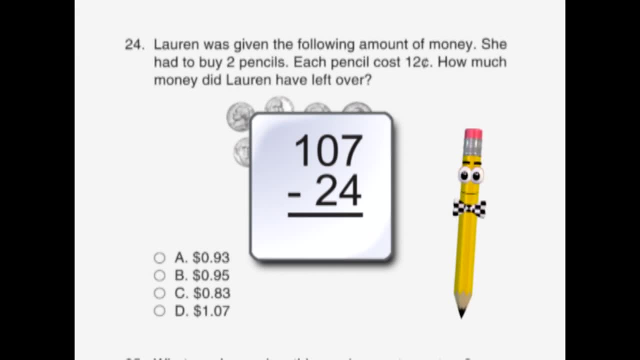 with $1.07 is the same as 107 cents. 107 minus 24 is, let's see: 7 minus 4 is 3.. Put that in the ones place, And 10 minus 2 is 8.. 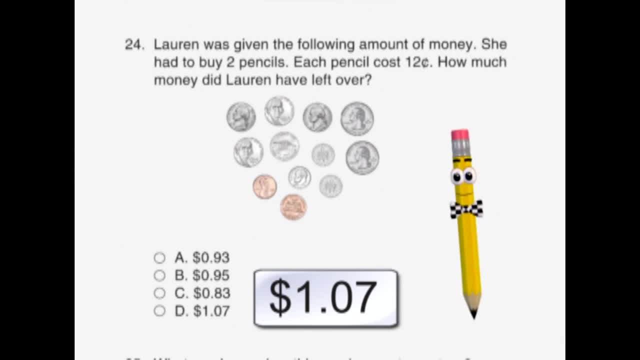 Now let's find out how much Lauren spent. 2 pencils cost 12 cents each. 2 times 12 equals 24.. Finally, we'll subtract what Lauren spent from the money she had to start with. 1 dollar and 7 cents is the same as 107 cents. 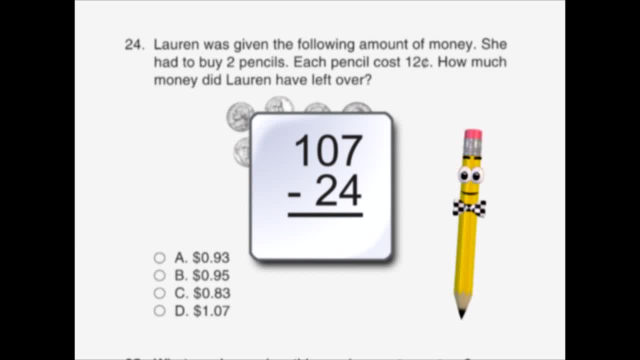 107 minus 24 is. Let's see: 7 minus 4 is 3.. Put that in the ones place, And 10 minus 2 is 8. 83 cents left over. The answer is C 83 cents. 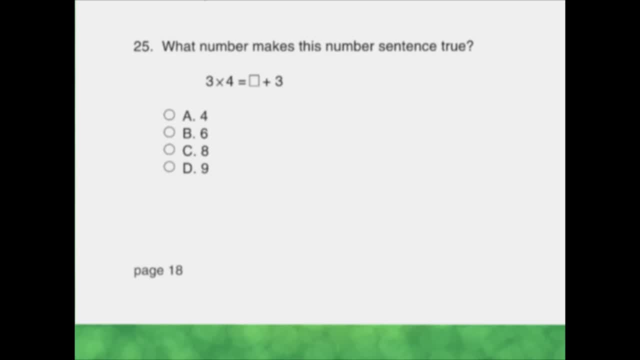 25.. What number makes this number sentence true? 3 times 4 equals blank plus 3.. A, 4, B, 6, C, 8, D, 9. What number can we add to 3 to make it equal to 3 times 4?? 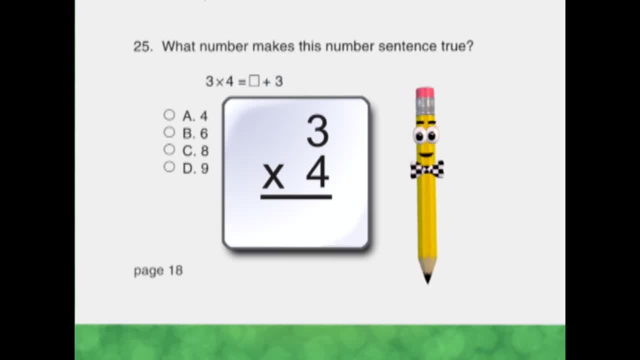 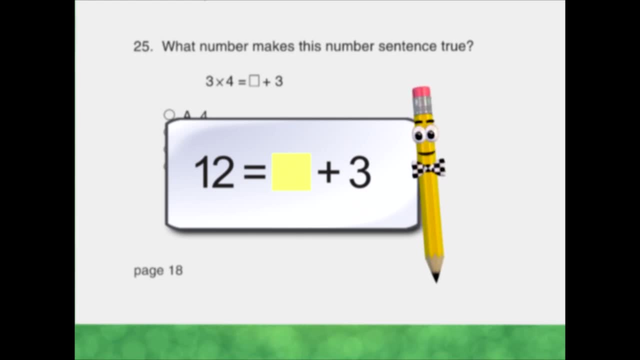 Let's simplify the problem by working out 3 times 4. That equals 12.. So we can write: 12 equals blank plus 3.. My, my, my. What number added to 3 gives us 12?? Let's subtract 3 from 12.. 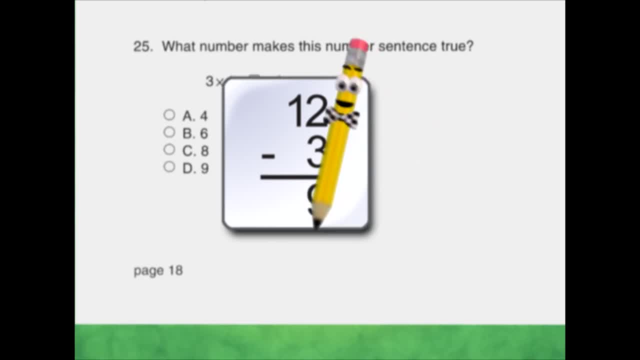 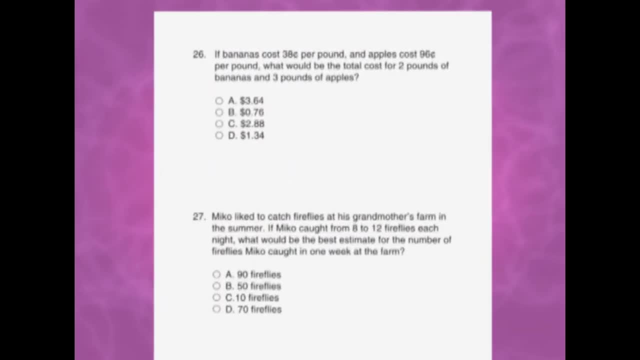 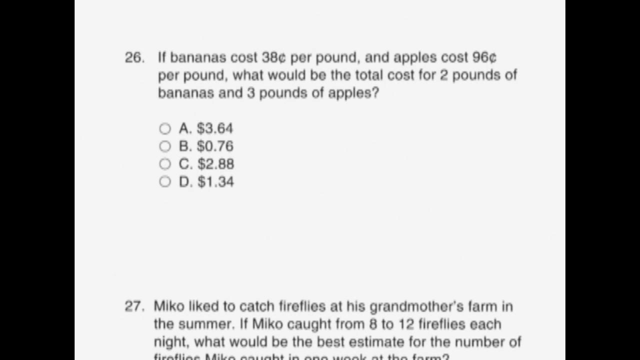 12 minus 3 equals 9.. The answer is D 9- 26.. If bananas cost 38 cents per pound and apples cost 96 cents per pound, what would be the total cost for 2 pounds of bananas and 3 pounds of apples? 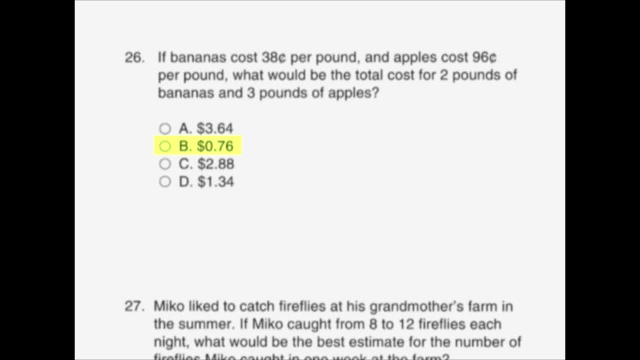 A- 3 dollars and 64 cents. B- 76 cents. C- 2 dollars and 88 cents. D- 1 dollar and 34 cents. We can simplify this problem by finding the prices for the bananas and then for the apples. The 2 pounds of bananas cost 2 times 38 cents. 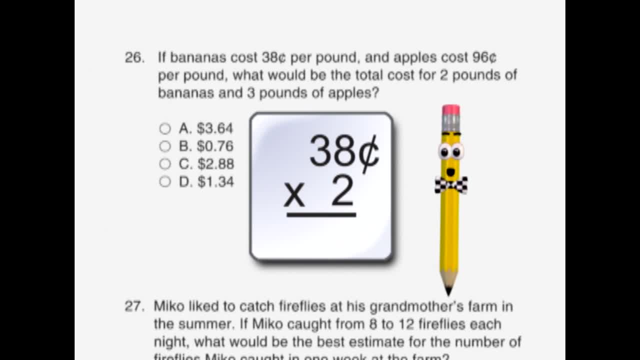 2 times 8 is 16.. Put the 6 in the ones place and write the 1 up here to add in later. 2 times 3 is 6, plus the 1 equals 7.. So the bananas cost 76 cents. 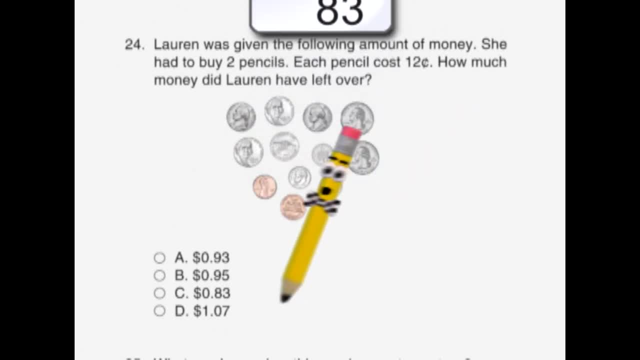 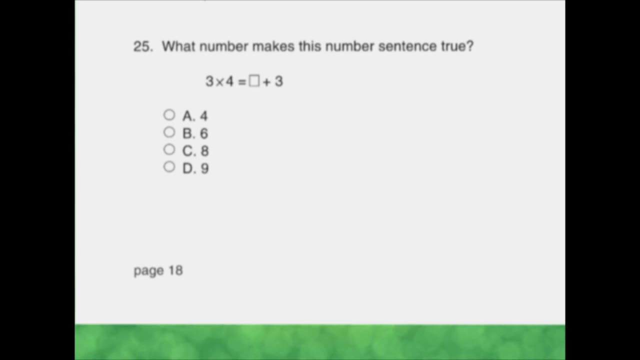 83 cents left over. The answer is C, 83 cents 25.. What number makes this number sentence true? 3 times 4 equals blank plus 3, A, 4, B, 6, C, 8, D, 9. What number can we add to 3 to make it equal to 3 times 4?? 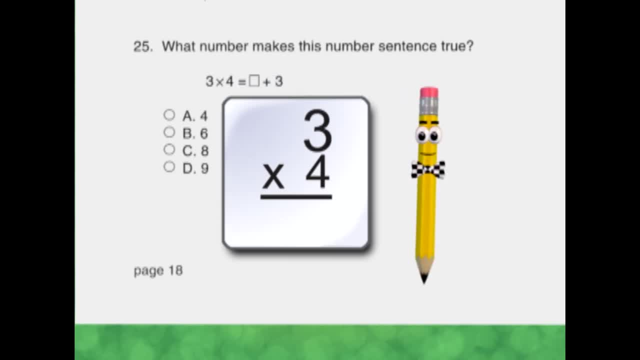 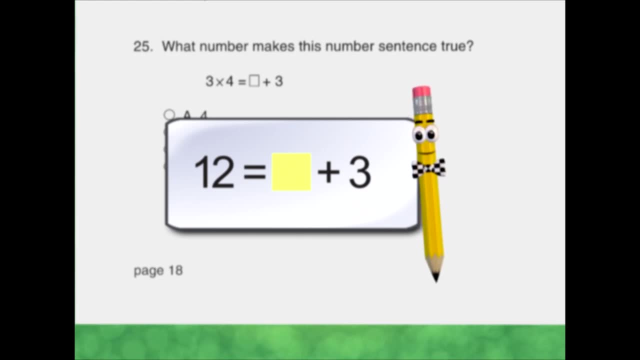 Let's simplify the problem by working out: 3 times 4, That equals 12, So we can write: 12 equals blank, plus 3, My, my, my. what number added to 3 gives us 12?? Let's subtract 3 from 12. 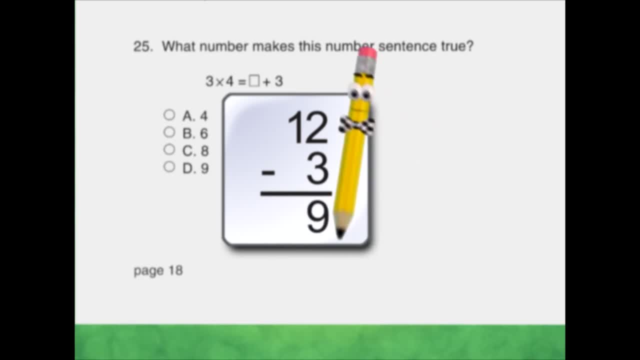 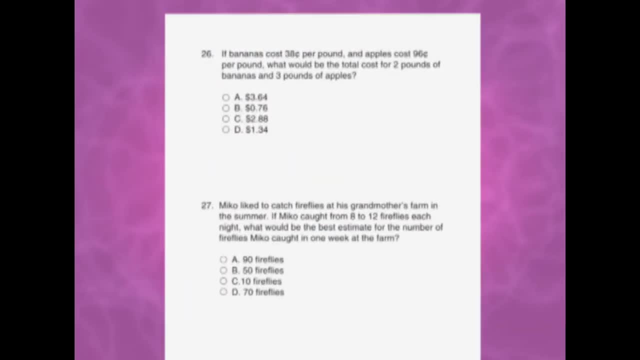 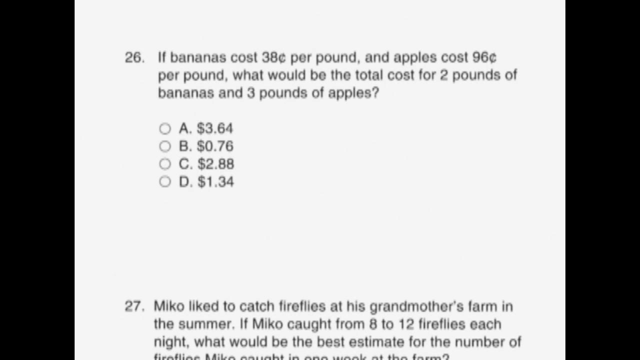 12 minus 3 equals 9. The answer is C D 9, 26.. If bananas cost 38 cents per pound And apples cost 96 cents per pound, What would be the total cost for 2 pounds of bananas and 3 pounds of apples? 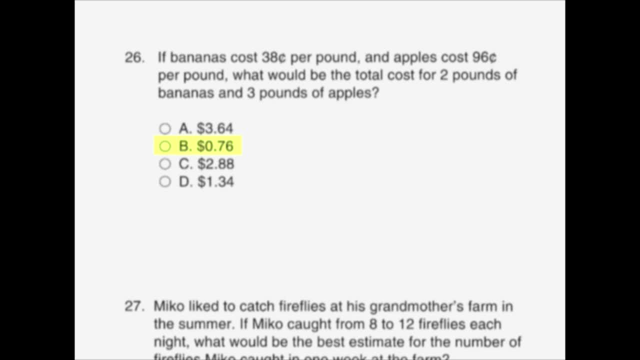 A $3.64, B 76 cents, C $2.88, D 9 D $1.34. We can simplify this problem by finding the prices for the bananas and then for the apples. The 2 pounds of bananas cost 2 times 38 cents. 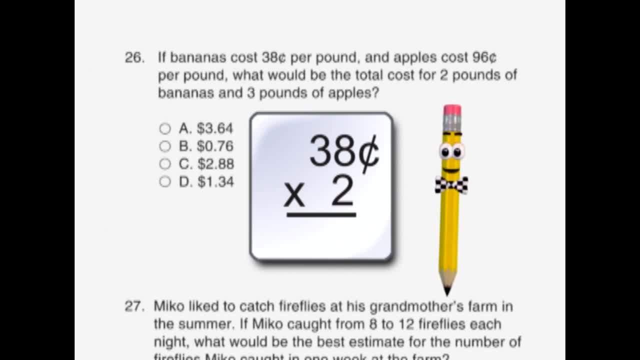 2 times 8 is 16. Put the 6 in the 1's place And write the 1 up here to add in later. 2 times 3 is 6, Plus the 1 equals 7. So the bananas cost 76 cents. 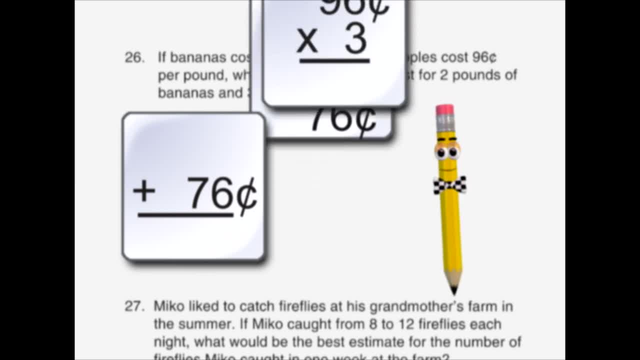 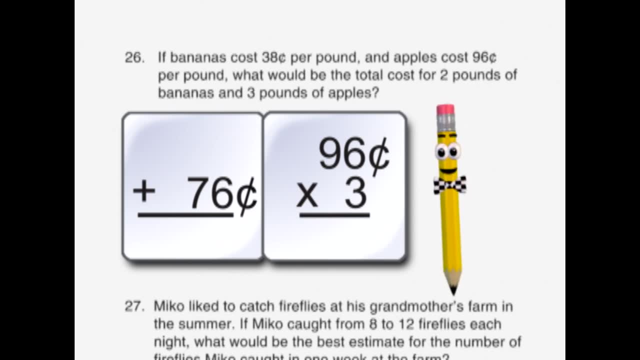 Write that here Now. the 3 pounds of apples will cost 3 times 96 cents. 3 times 6 is 18. The 8 goes down here. Put the 1 up here to add in later. 3 times 9 is 27. 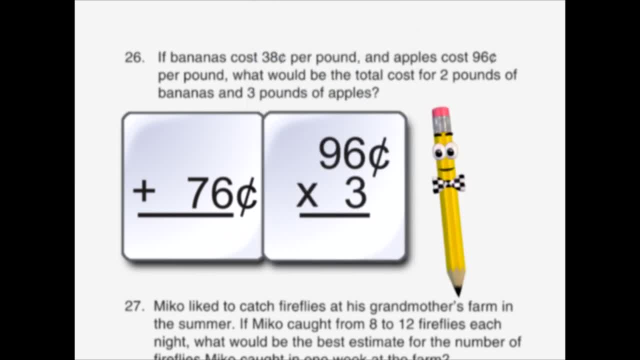 Write that here Now. the 3 pounds of apples will cost 3 times 96 cents. 3 times 6 is 18.. The 8 goes down here. Put the 1 up here to add in later. 3 times 9 is 27.. 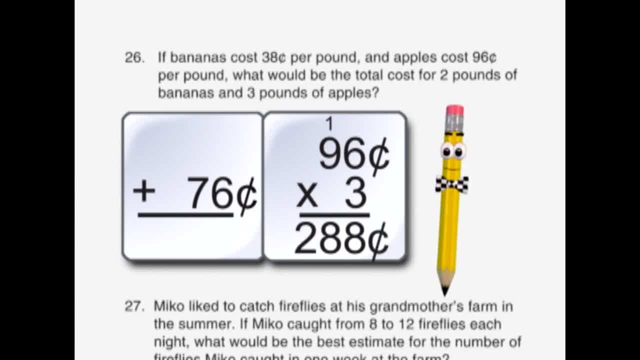 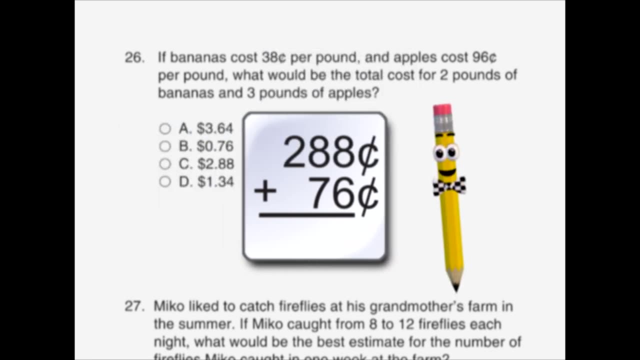 Add the 1 to get 28.. The apples cost 288 cents. We need to add the cost of the apples and the bananas together to get the total cost. Let's add the cents first and then convert them to dollars and cents: 288 plus 76.. 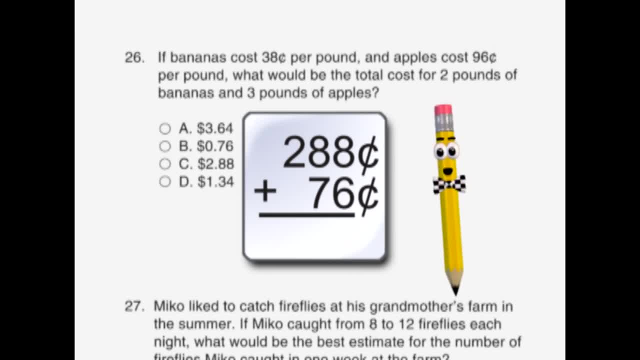 8 plus 6 is 14.. Put down the 4.. Carry the 1.. 8 plus 7 is 15.. Plus the 1 is 16.. Put the 6 here and carry the 1.. 2 plus that 1 is 3.. 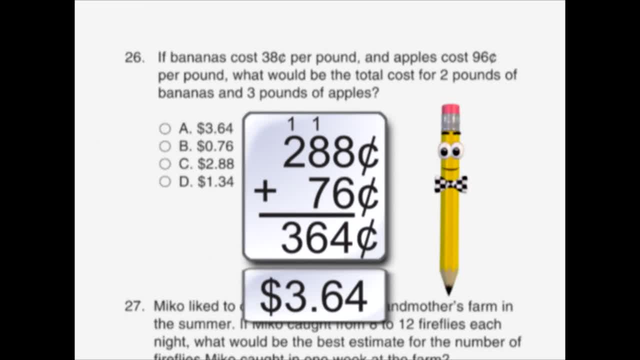 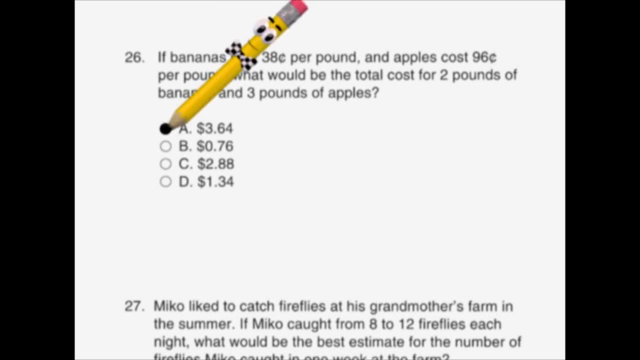 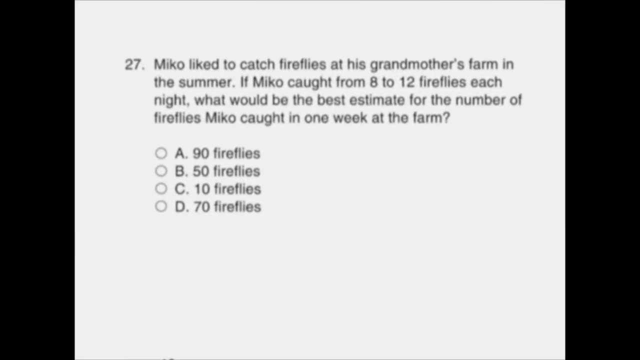 364 cents or 3 dollars and 64 cents? That means the correct answer is A 3 dollars and 64 cents. 27. Miko liked to catch fireflies at his grandmother's farm in the summer. If Miko caught from 8 to 12 fireflies each night, 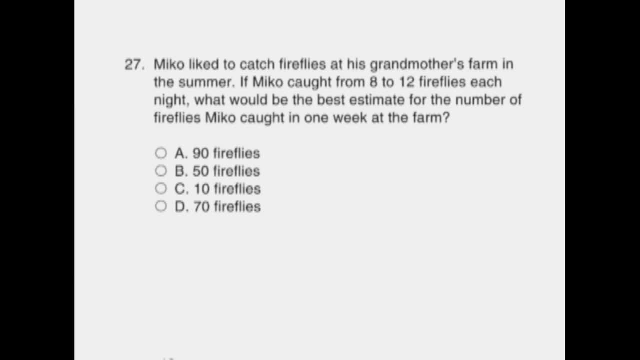 what would be the best estimate for the number of fireflies Miko caught in one week at the farm? A- 90 fireflies. B- 50 fireflies. C- 10 fireflies. D- 70 fireflies. One way to estimate an answer to a problem is to round the numbers before working the problem. 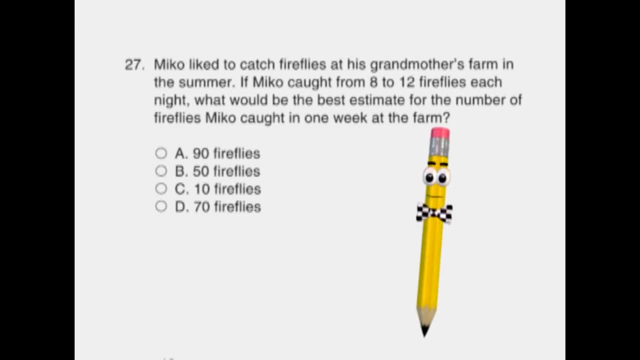 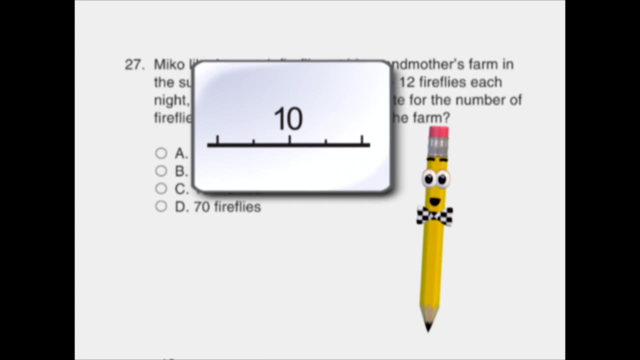 Since all of our answers are rounded to the nearest 10, let's round the number of fireflies Miko catches. Hey look, Both 8 and 12 round to 10.. 8 rounds up and 12 rounds down. That makes this problem very simple, then. 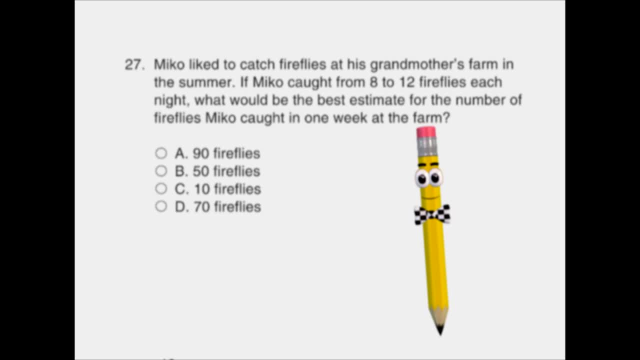 All we need to know is the number of days in a week. That's easy: 7!. Ah, So if we multiply our estimated number of fireflies each night by the number of nights in a week, we get 70. So the answer is: 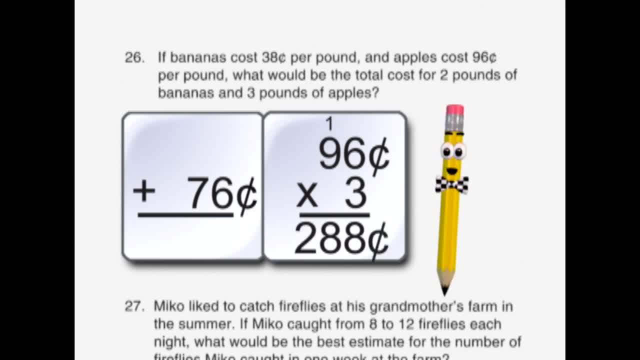 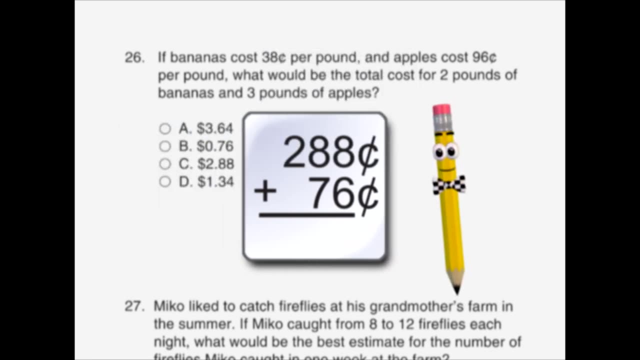 Add the 1 to get 28. The apples cost 288 cents. We need to add the cost of the apples and the bananas together to get the total cost. Let's add the cents first and then convert them to dollars and cents: 288 plus 76. 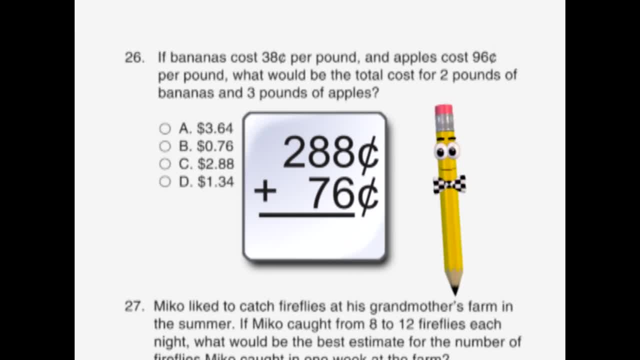 8 plus 6 is 14. Put down the 4, Carry the 1. 8 plus 7 is 15 Plus the 1 is 16. Put the 6 here And carry the 1. 2 plus that 1 is 3. 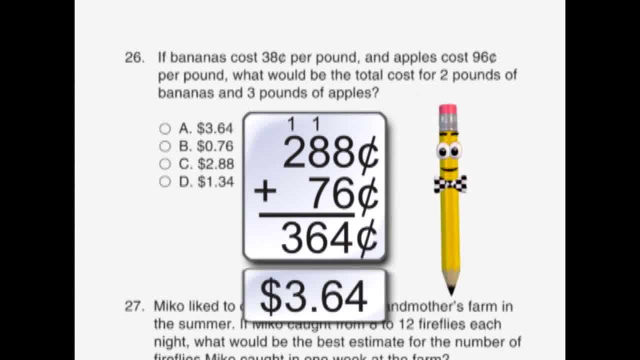 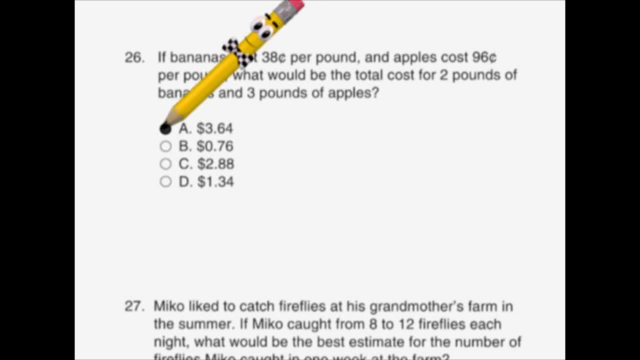 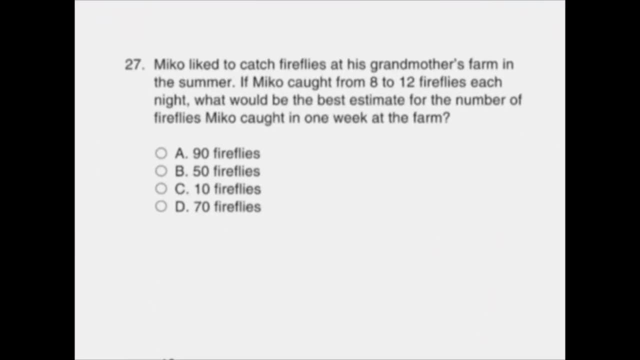 364 cents or $3.64. That means the correct answer is A $3.64 27. Miko liked to catch fireflies at his grandmother's farm in the summer. If Miko caught from 8 to 12 fireflies each night, What would be the best estimate for the number of fireflies Miko caught in one week at the farm? 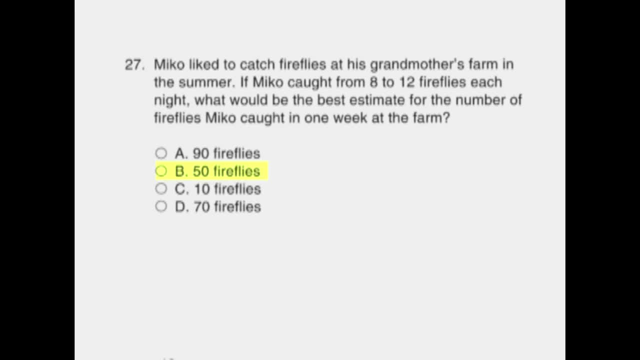 A- 90 fireflies. B- 50 fireflies. C- 10 fireflies. D- 70 fireflies. One way to estimate an answer to a problem is to round the numbers before working the problem. Since all of our answers are rounded to the nearest 10, Let's round the number of fireflies Miko catches. 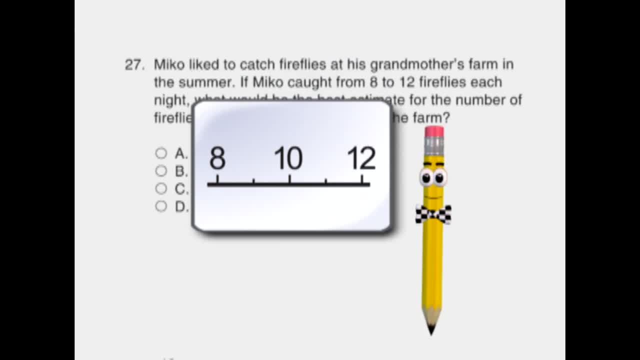 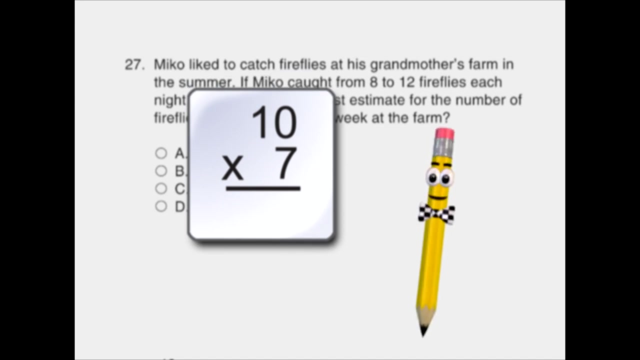 Hey look, Both 8 and 12 round to 10. 8 rounds up And 12 rounds down. That makes this problem very simple. then All we need to know is the number of days in a week. That's easy: 7 Ah. So if we multiply our estimated number of fireflies each night by the number of nights in a week, 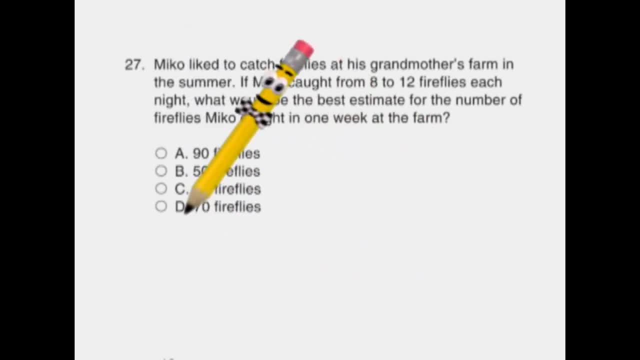 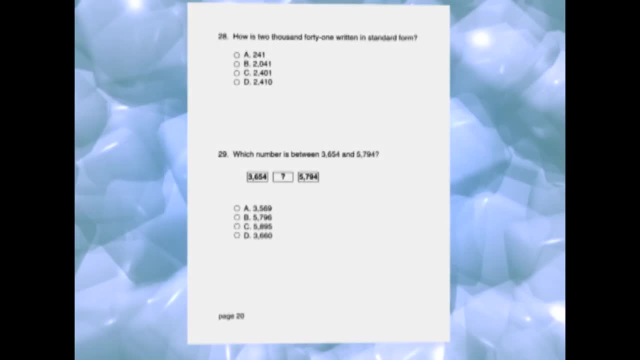 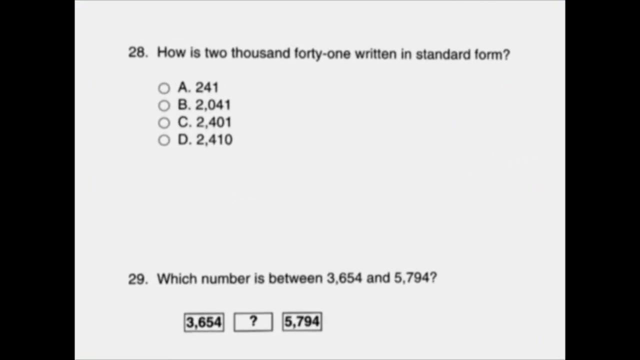 We get 70. So the answer is D 70 fireflies. Sometimes it is helpful to make a list table or chart to help you work out a problem. We'll practice that in the next few questions. 28: How is 2041 written in standard form? 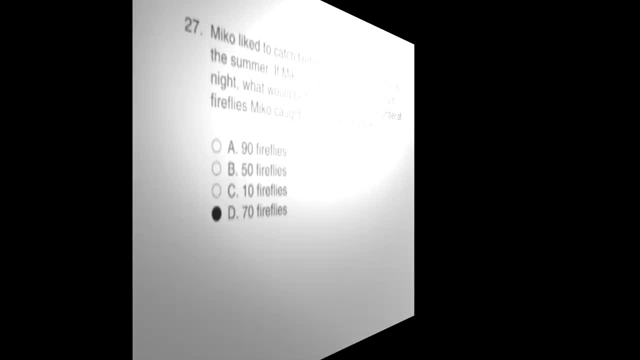 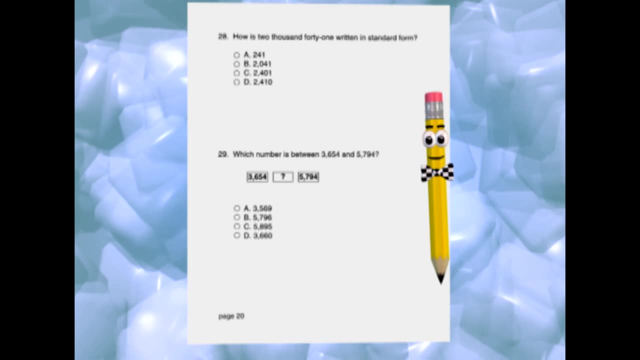 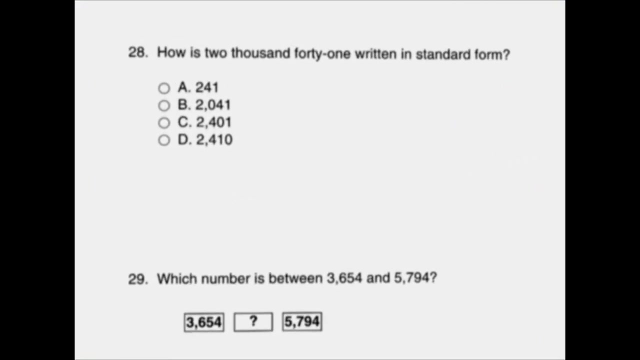 D 70 fireflies. Sometimes it is helpful to make a list table or chart to help you work out a problem. We'll practice that in the next few questions, 28.. How is 2041 written in standard form When doing place value problems? 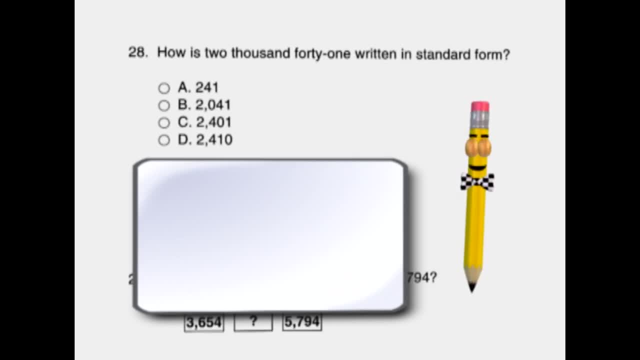 make a little table that shows the place value of all the numbers. In this case we would put a 2 into the thousands column and a 0 into the hundreds column. The tens column gets a 4 and the ones column gets a 1.. 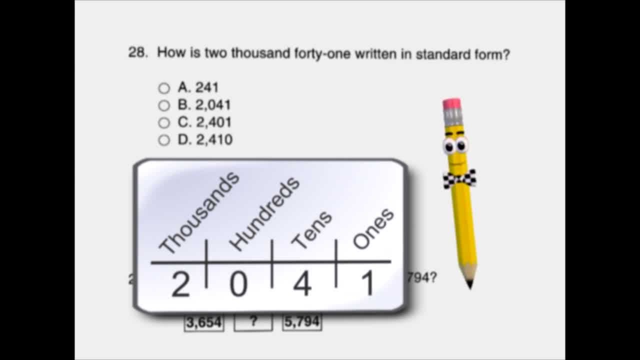 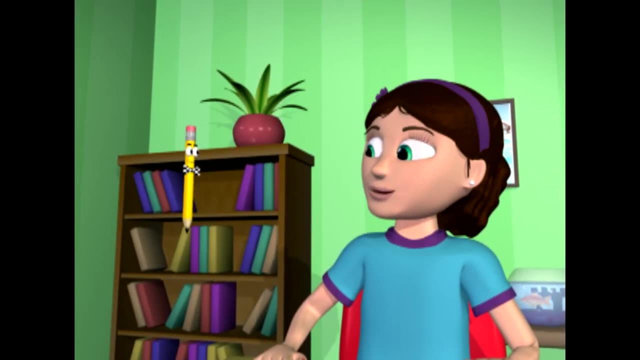 This makes it easy to get the correct number. From our table, we can see that the correct answer is B 2041.. Wow, Making a table makes figuring out a problem much easier. This is true, But do you know who invented the round table? 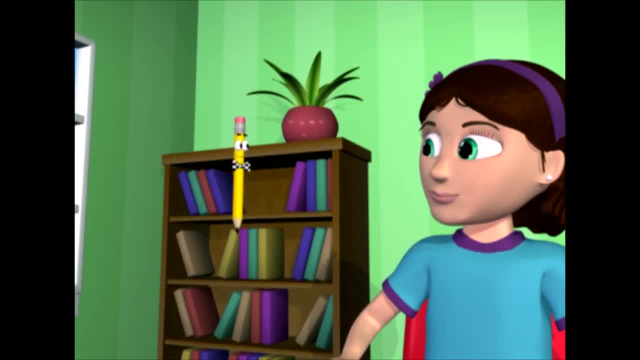 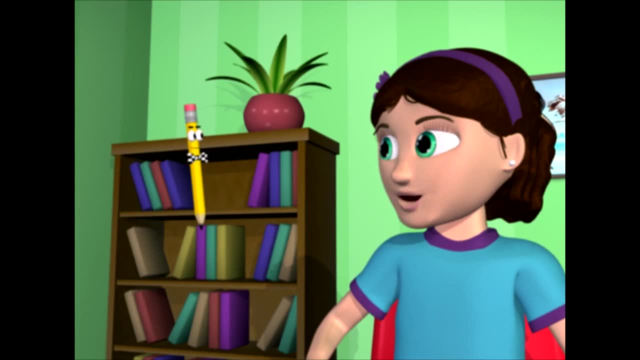 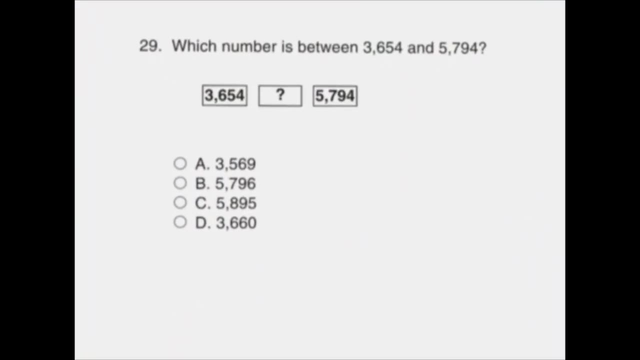 No, Who It was, Sir Cole. No, You circle, you get Sir Cole. You have some silly jokes. I think I'm ready to move on 29.. Which number is between 3,654 and 5,794?? 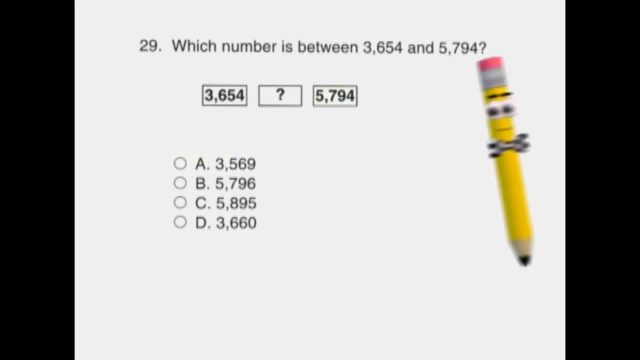 A- 3,569. This number is less than 3,654.. B- 5,796. This number is higher than 5,794.. C- 5,895. This number is higher than 5,795.. And this one is too high as well. 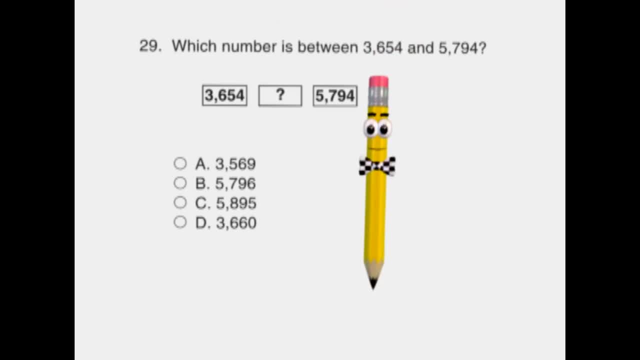 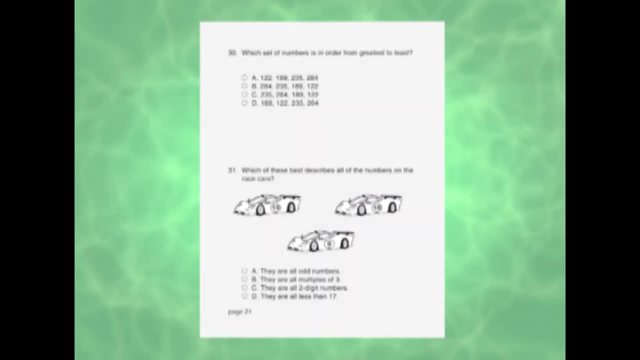 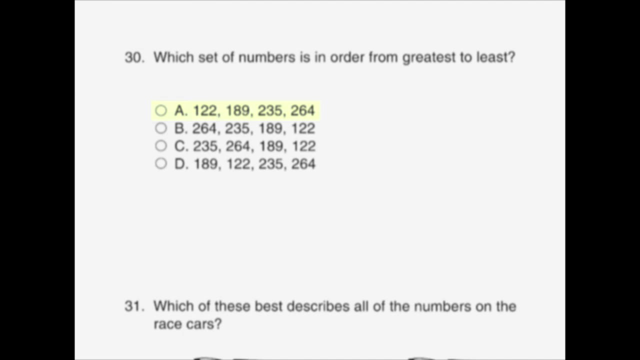 D: 3,660. That's the correct one. 30.. Which set of numbers is, in order from greatest to least? A, 122, A, 189, B, 235, C, 264. 189 is more than 122.. 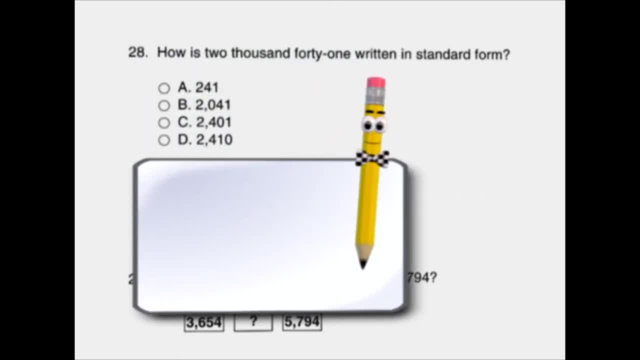 When doing place value problems. Make a little table that shows the place value of all the numbers. In this case we would put a 2 into the thousands column And a 0 into the hundreds column. The tens column gets a 4 And the ones column gets a 1. 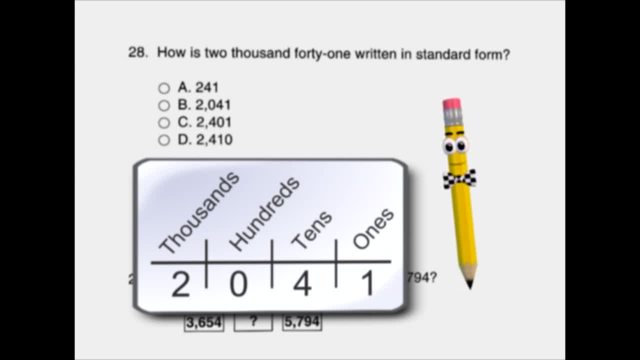 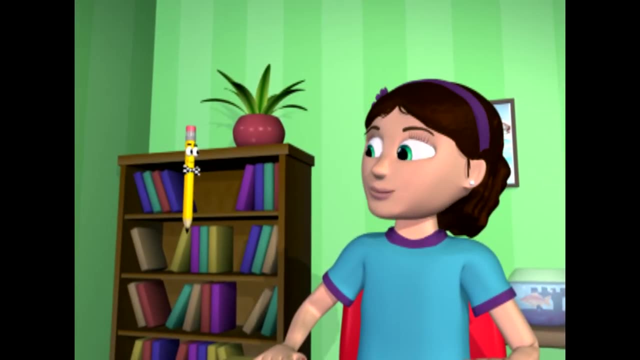 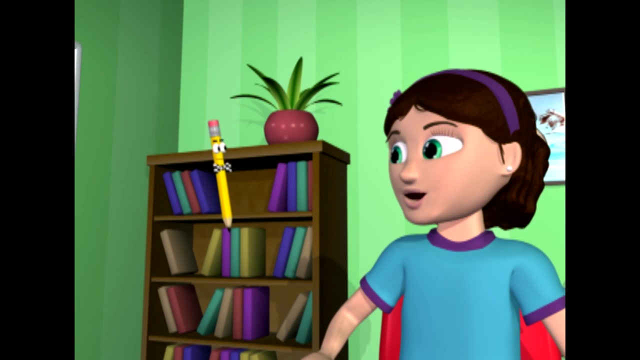 This makes it easy to get the correct number. From our table, we can see that the correct answer is B 2041. Wow, Making a table makes figuring out a problem much easier. This is true, But do you know who invented the round table? No, Who? 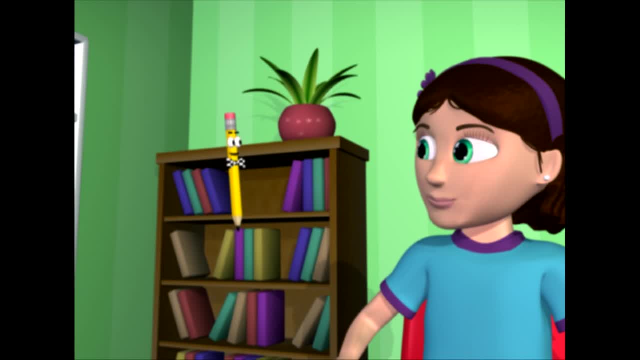 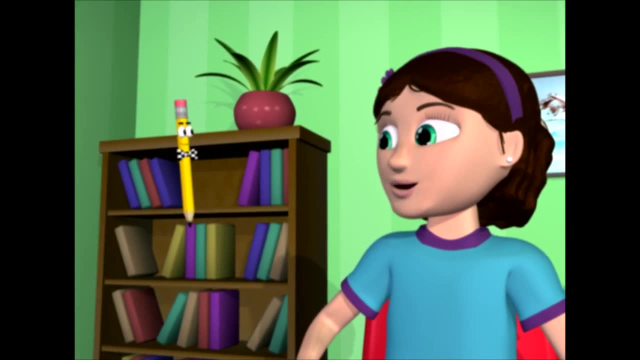 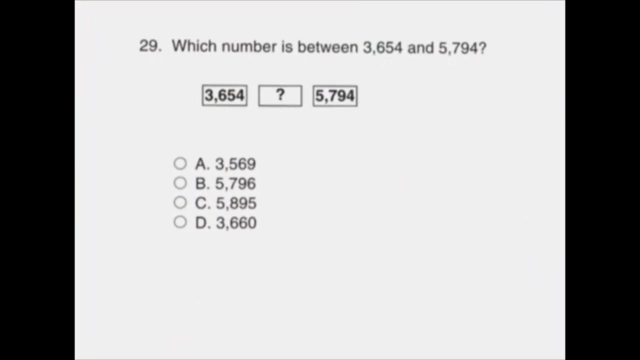 It was Sir Cole. You circle, You get sir Cole. You have some silly jokes. I think I'm ready to move on. 29, Which number is between 3,654 and 5,794?? A 3,569. This number is less than 3,654. 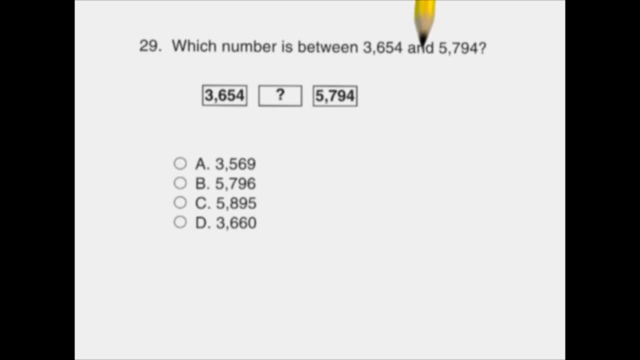 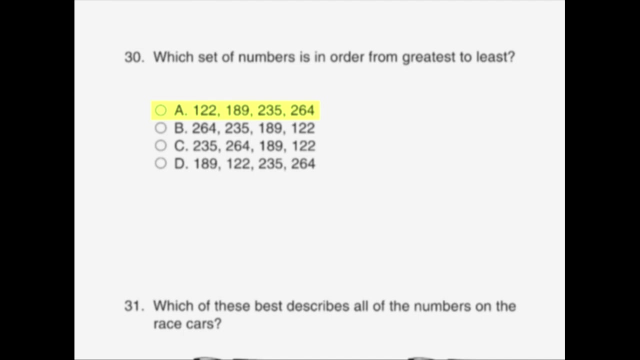 B 5,796. This number is higher than 5,794. C 5,895, And this one is too high as well. D 3,660, That's the correct one. 30, Which set of numbers is in order from greatest to least? 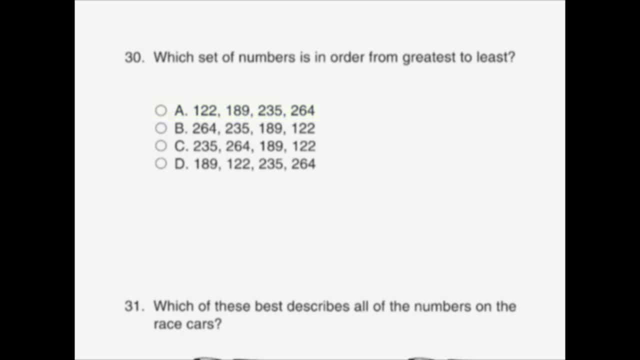 A 122,189,235,264. 189 is more than 122 And 235 is more than 182, And 264 is the highest in the list. These are in order from least to greatest. That's the opposite of what this question is asking. 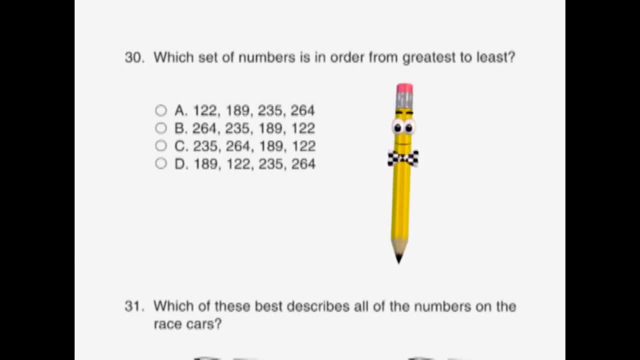 And 235 is more than 189.. And 264 is the highest in the list. These are in order from least to greatest. That's the opposite of what this question is asking: B 264, B 235, C, 289. 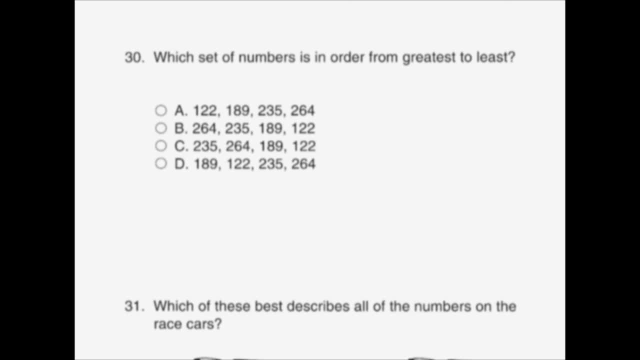 D, 122, 235 is less than 264.. And 189 is less than 235.. And 122 is the smallest in the list. These are in order from greatest to least. That is what this question is asking. I think this is the answer. 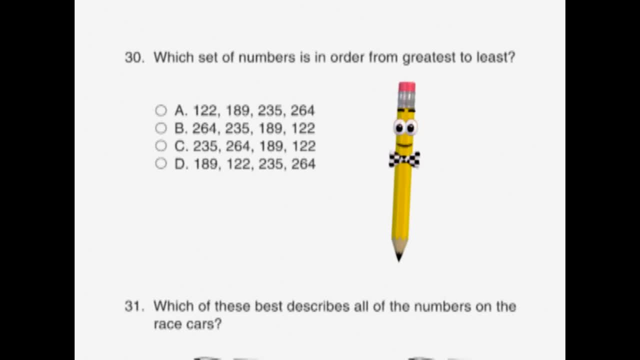 But let's look at the other two just to see if they are correct. Let's look at the other two just to see if they are correct: B 3,690, C 3,690, D, 3,690, D 3,690. 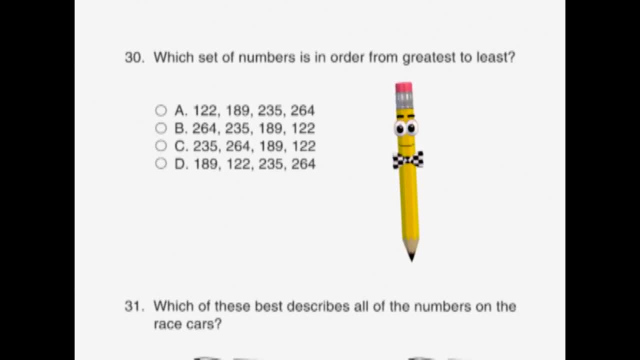 B 3,690 C 3,690 D 3,690. B 3,690 C 3,690 D 3,690 B 3,690. Let's look at the other two just to be sure. 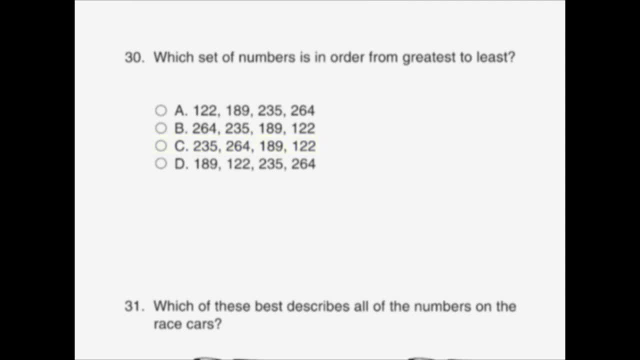 C 235. C. 235, 264, 189, 122. 264 is greater than 235.. So this cannot be right. D 189, 122, 235, 264. 122 is less than 189.. 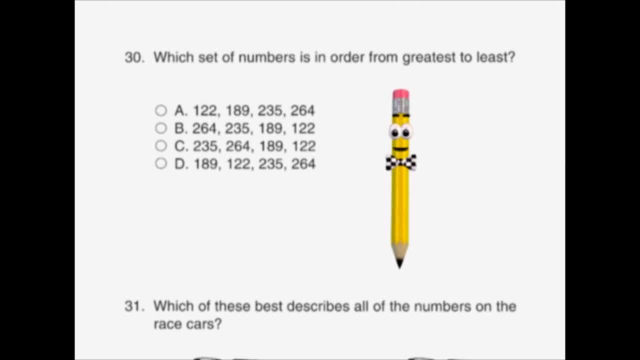 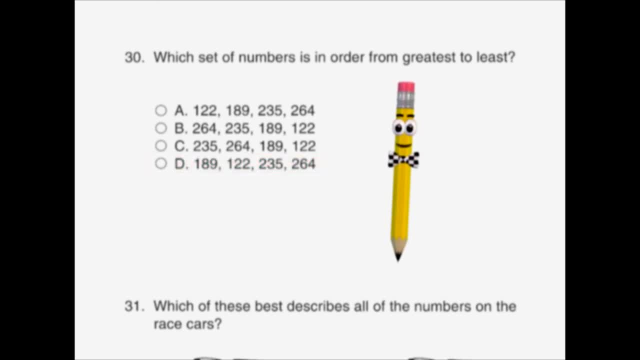 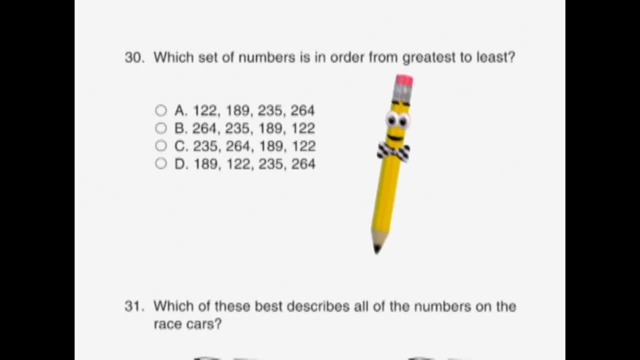 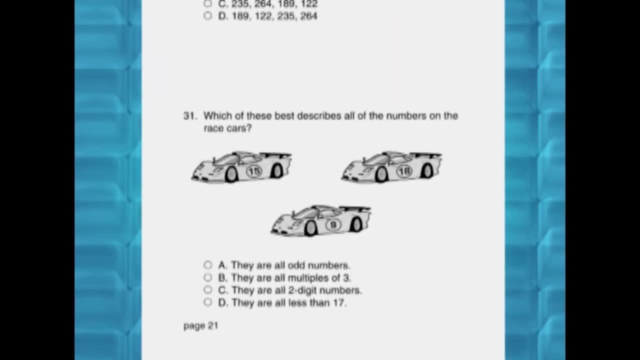 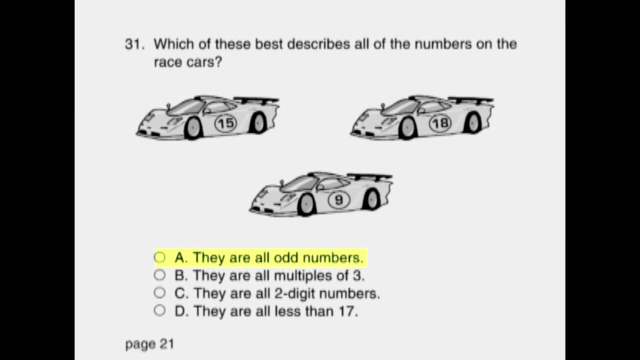 135,, 189, 122.. On we go, 31.. Which of these best describes all of the numbers on the race cars? A- They are all odd numbers. Well, no, 18 is an even number. B- They are all multiples of 3.. 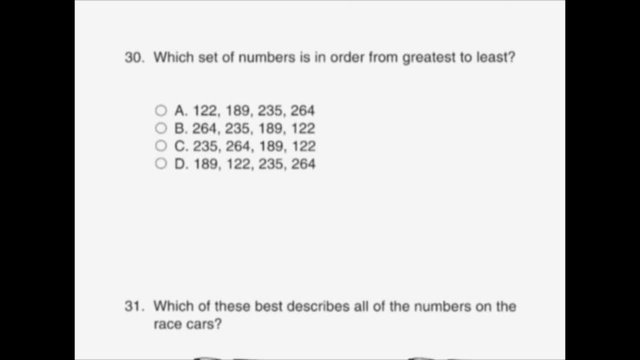 B 264,235,189,122. 235 is less than 264 And 189 is less than 235, And 122 is the smallest in the list. These are in order from greatest to least. That is what this question is asking. I think this is the answer. 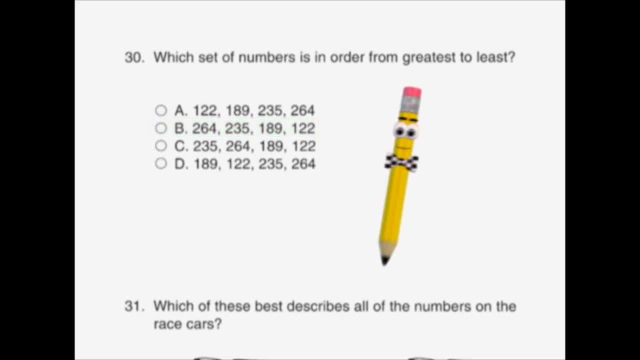 But let's look at the other two just to be sure. C 235,264,189,122, 264 is greater than 235, So this cannot be right. D 189,122,235,264, 122 is less than 189, But 235 is more than 122. 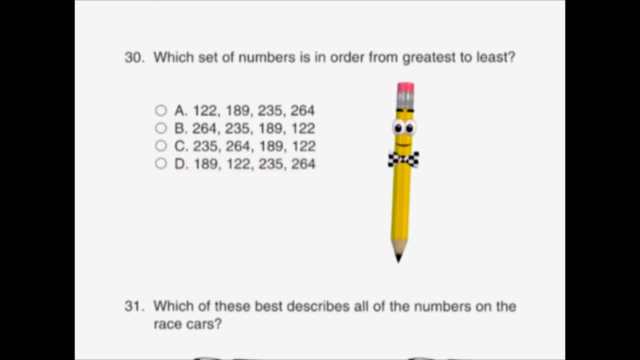 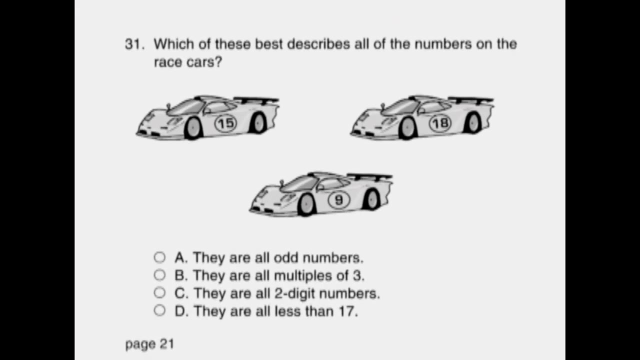 Our answer is, in fact B- 264,235,189,122. On we go 31. Which of these best describes all of the numbers on the race cars? A- They are all odd numbers. Well, no, 18 is an even number. B- They are all multiples of 3. 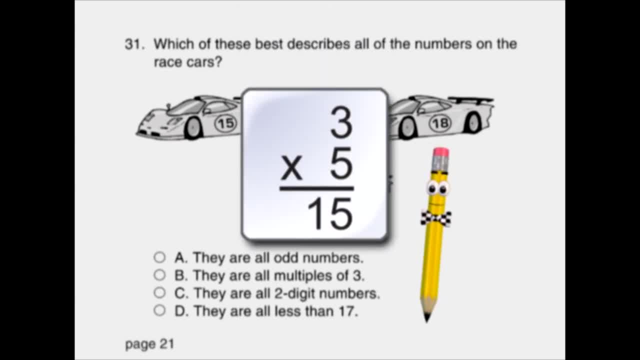 Hmm, let's check: 3 times 5 is 15, 3 times 3 is 9 And 3 times 6 is 18. They are all multiples of 3. Let's read through the other answers before marking our choice C. They are all two-digit numbers. 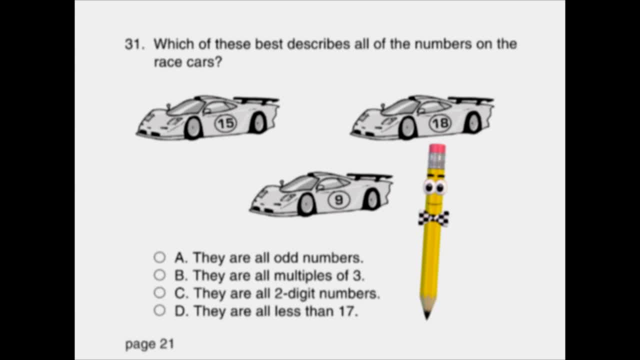 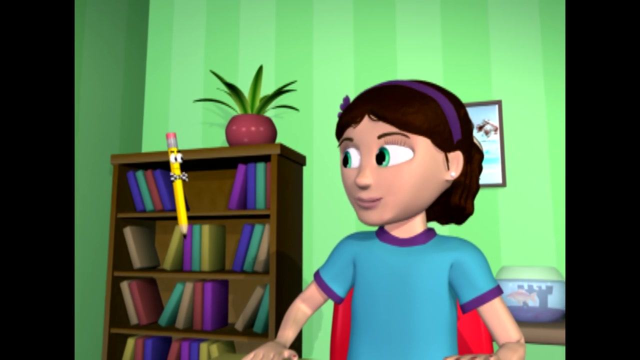 Incorrect. 9 is a single-digit number, D. They are all less than 17. 18 is one greater than 17. Our answer really is B. They are all multiples of 3. Hey Marco, why did the math test go to see the school counselor? 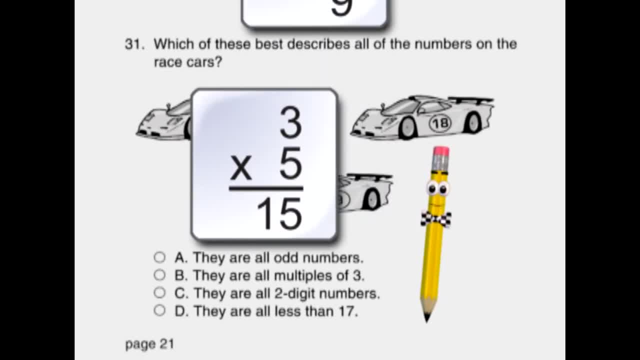 Let's check: 3 times 5 is 15.. 3 times 3 is 9. And 3 times 6 is 18.. They are all multiples of 3.. Let's read through the other answers before marking our choice. 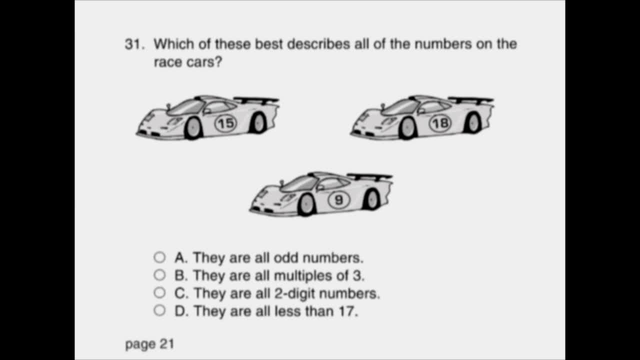 C: They are all two-digit numbers. Incorrect: 9 is a single-digit number. D: They are all less than 17.. 18 is one greater than 17.. Our answer really is B. They are all multiples of 3.. 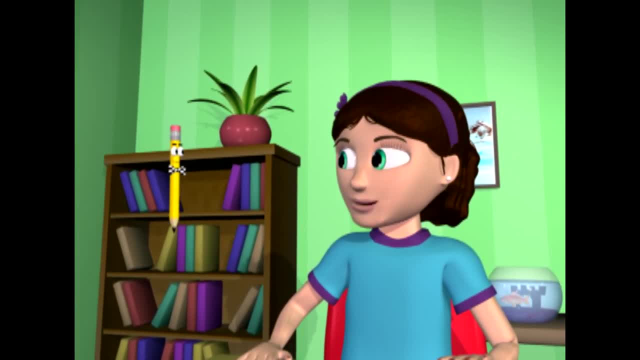 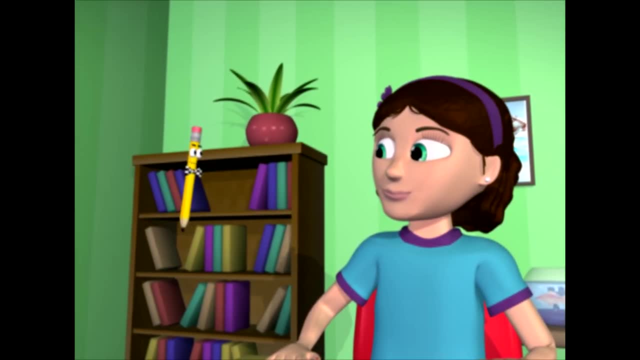 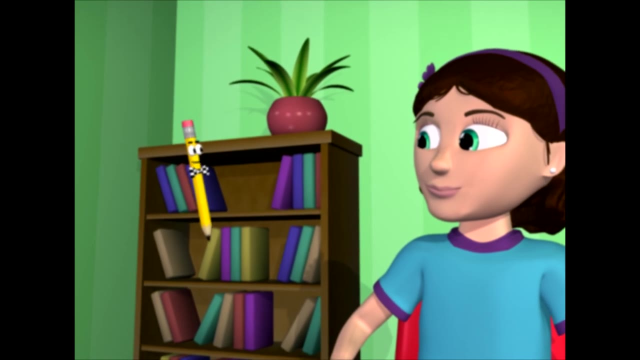 Hey Marco, Why did the math test go to see the school counselor? I don't know. Why did the math test go to see the school counselor? He had a lot of problems. Well then, let's work some more of these problems. 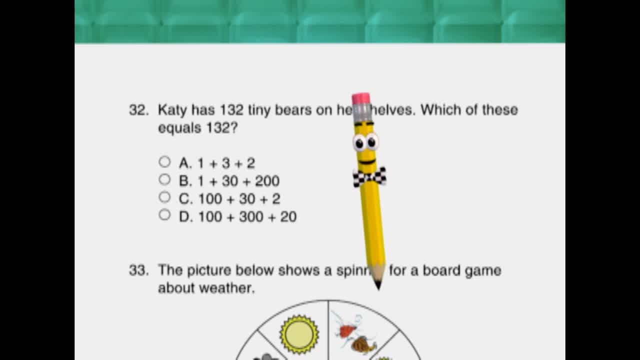 Remember. when possible, you should check your answers to see if they are reasonable. Your answers should make sense: 32.. Cady has 132 tiny bears. They are all on her shelves. Which of these equals 132?? A, 1 plus 3 plus 2.. 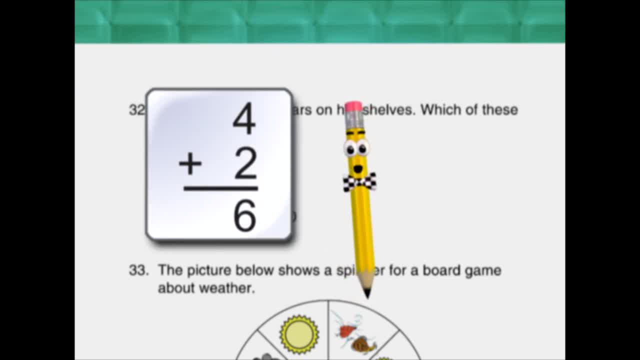 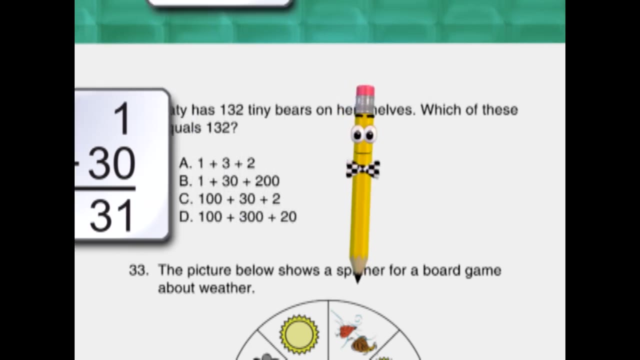 1 plus 3 is 4.. 4 plus 2 is 6.. This is much too small B: 1 plus 30 plus 200.. 1 plus 30 is 31.. Add 200 to get 202.. 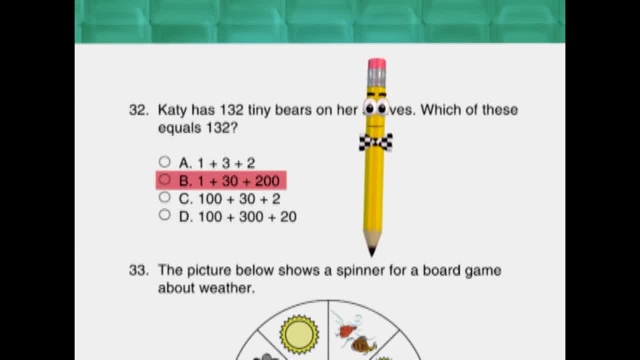 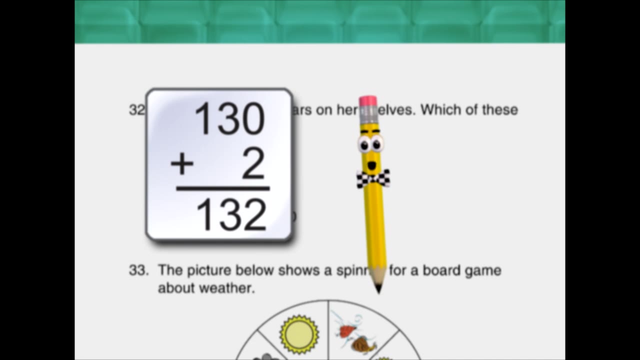 B: 1 plus 30 plus 200.. It's 131.. Not correct. C: 100 plus 30 plus 2.. 100 plus 30 equals 130.. Add 2 to get 132.. Here's our answer. 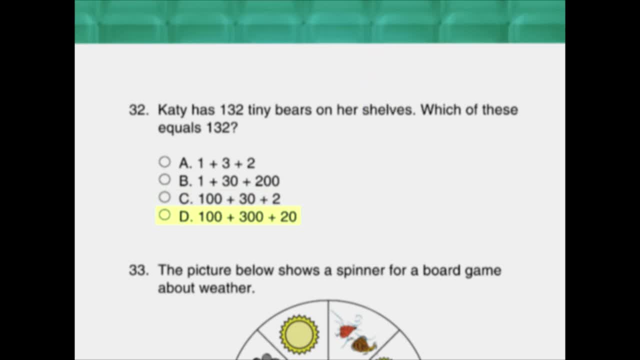 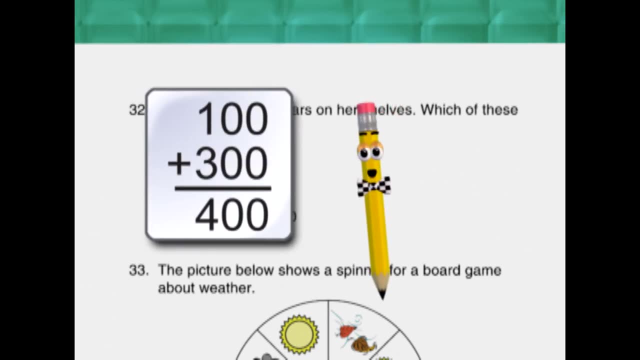 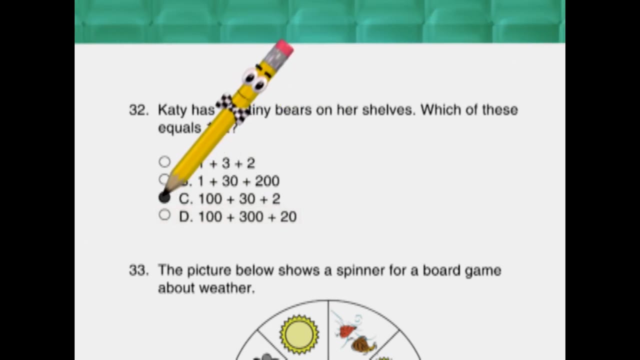 But let's look at the last one: D 100 plus 300 plus 20.. 100 plus 300 is 400.. That's already too high. The answer is: C 100 plus 30 plus 2. That equals 132.. 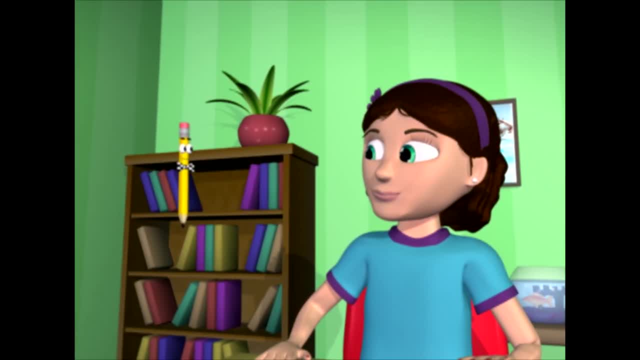 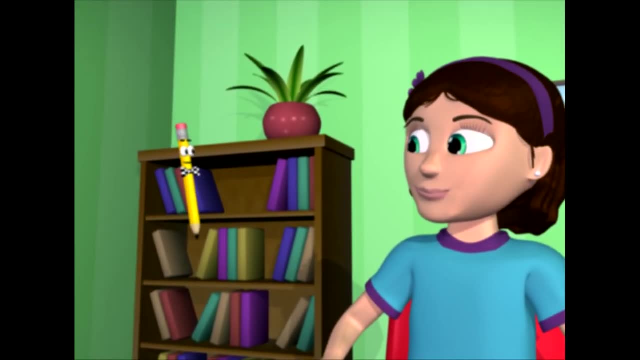 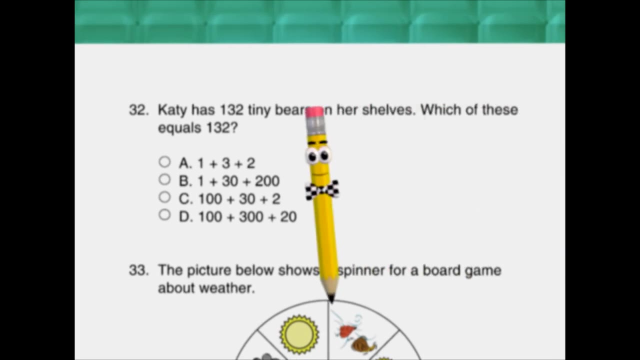 I don't know Why did the math test go to see the school counselor? He had a lot of problems. Well then, let's work some more of these problems. Remember: when possible you should check your answers to see if they are reasonable. Your answers should make sense. 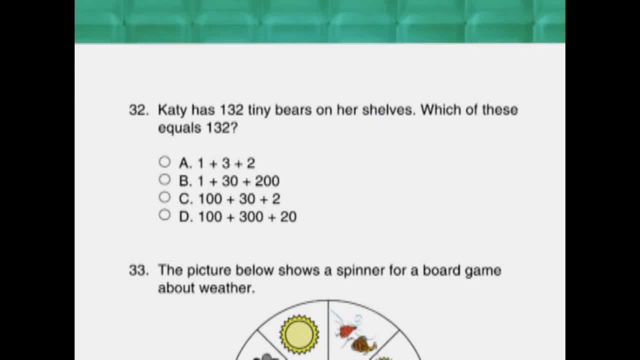 32. Katie has 132 tiny bears on her shelves. Which of these equals 132?? A: 1 plus 3 plus 2. 1 plus 3 is 4. 4 plus 2 is 6. This is much too small. B: 1 plus 30 plus 200. 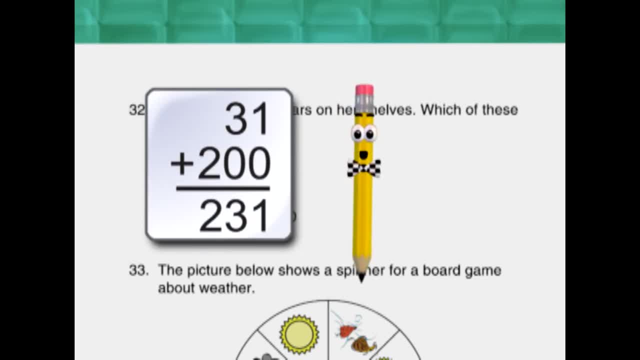 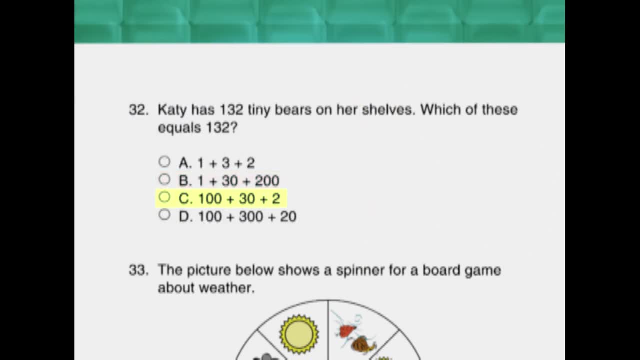 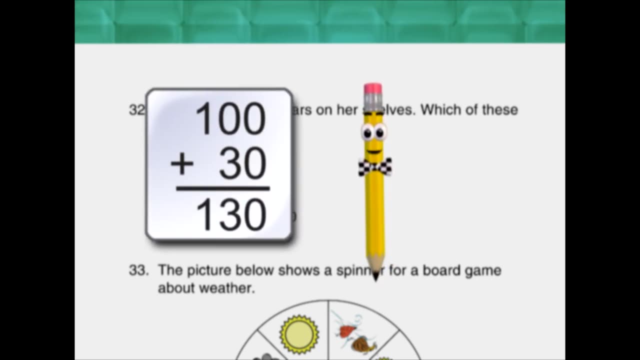 1 plus 30 is 31. Add 200 to get 231. Not correct C: 100 plus 30 plus 2. 100 plus 30 equals 130. Add 2 to get 132. Here's our answer. But let's look at the last one. 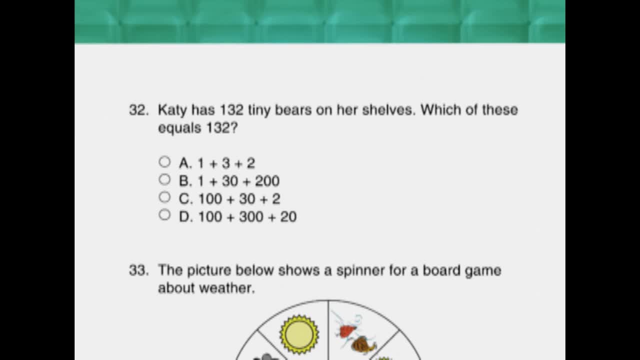 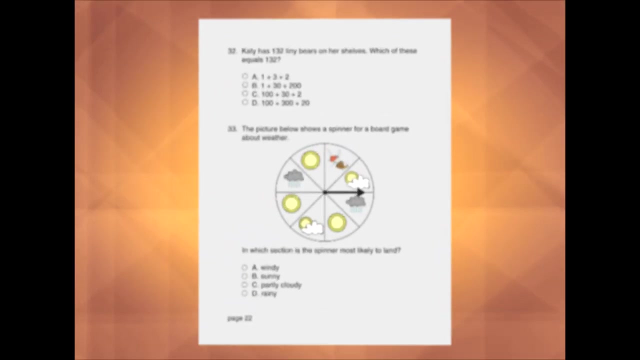 D 100 plus 300 plus 20, 100 plus 300 is 400. That's already too high. The answer is: C 100 plus 30 plus 2, That equals 132- 33. The picture below shows a spinner for a board game about weather. 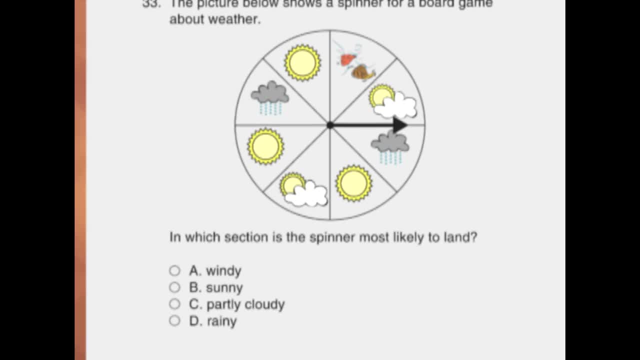 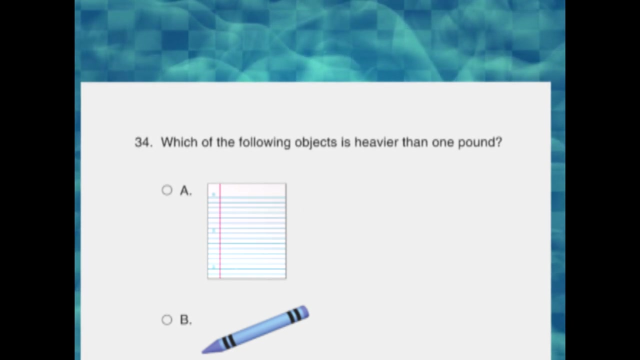 In which section is the spinner most likely to land? A- Windy, B- Sunny, C- Partly cloudy, D- Rainy. The spinner is most likely to land on the section with the most pieces, So the answer is B- Sunny, 34. Which of the following objects is heavier than one pound? 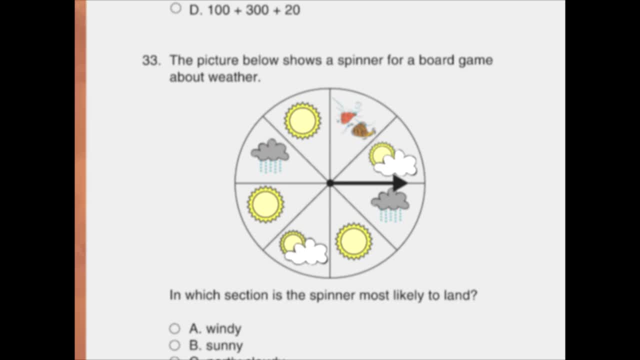 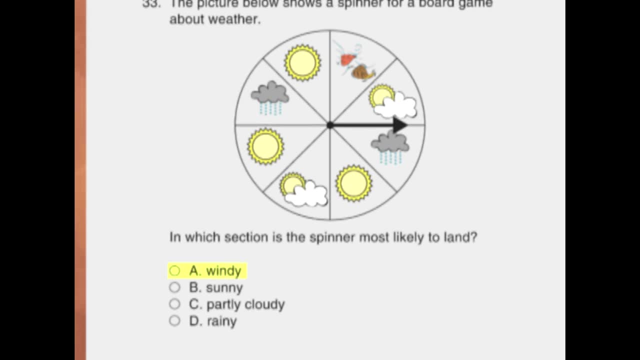 33.. The picture below shows a spinner for a board game about weather. In which section is the spinner most likely to land? A- Windy, B. Sunny, C. Partly cloudy, D- Rainy. The spinner is most likely to land on the section with the most pieces. 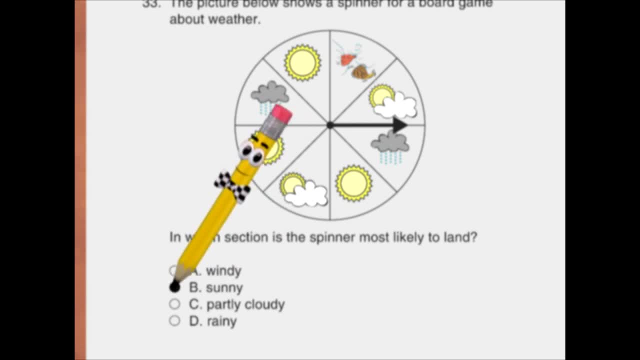 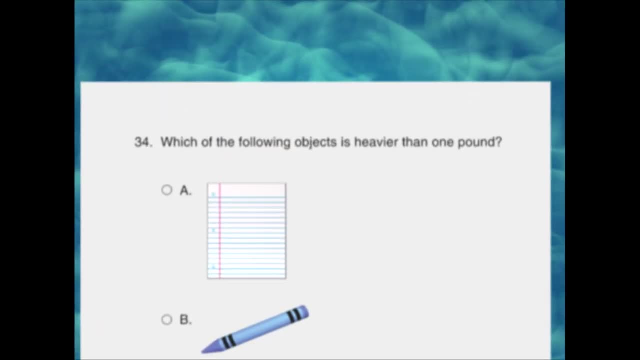 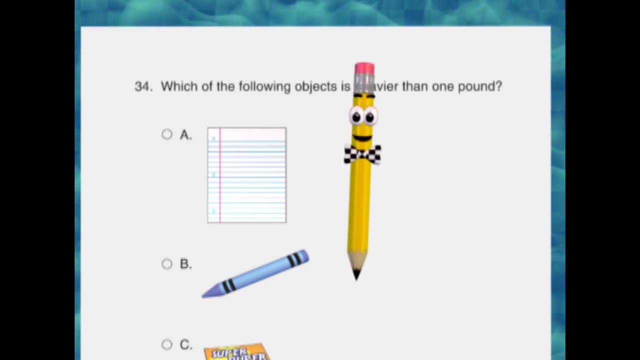 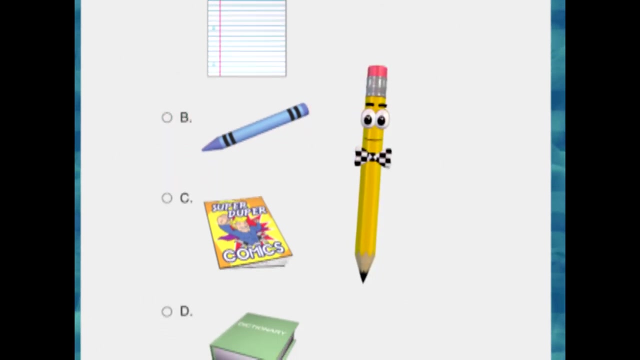 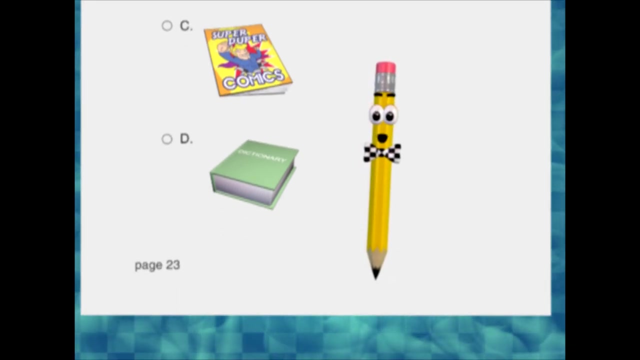 So the answer is B Sunny 34.. Which of the following objects is heavier than one pound? Now, a piece of paper is very light And a crayon is not very heavy either. A comic book might weigh a pound. But the last answer- a thick dictionary would definitely weigh more than a pound. 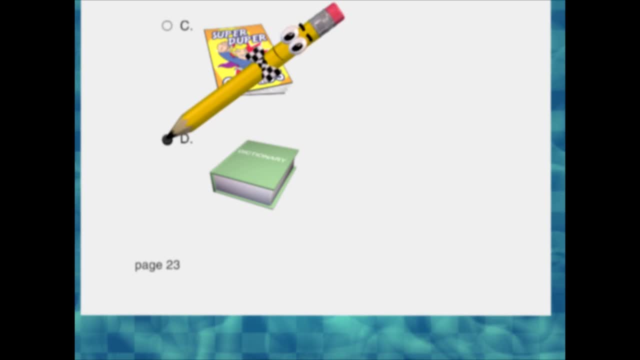 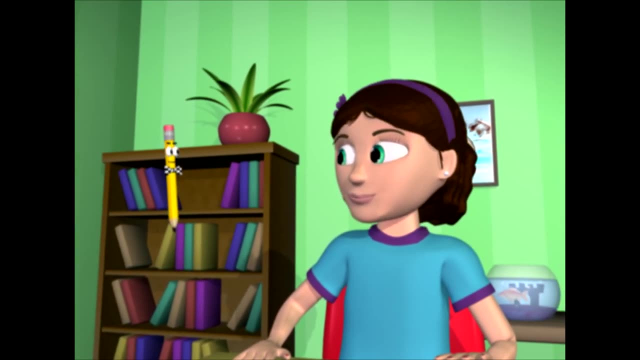 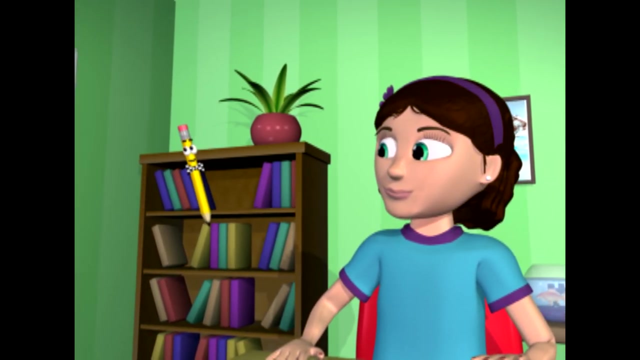 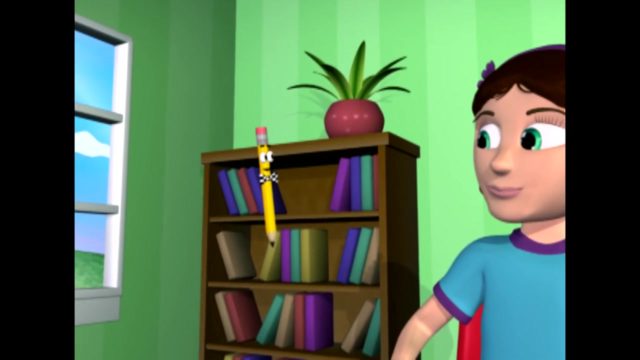 Will Mark answered D. Do you know what bird can lift the heaviest weight? Which bird would that be? The crane, That was a good one. Did you know that math tests may have questions that require you to know the meanings of words used in math? 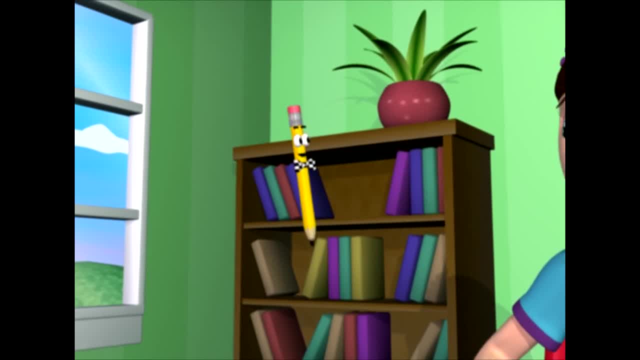 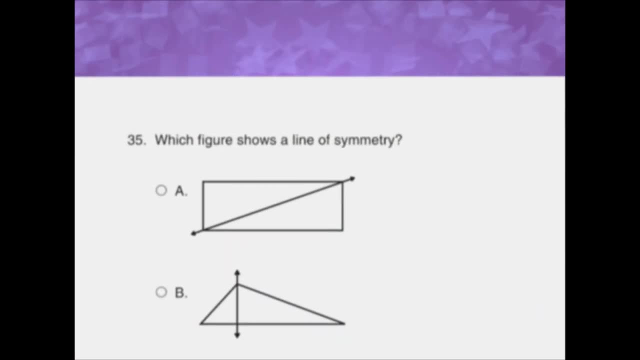 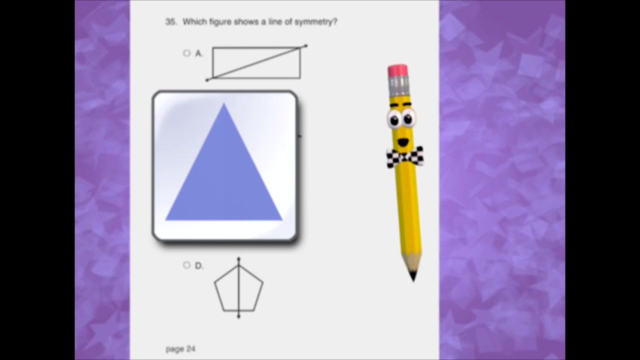 Be sure you review the math terms and definitions that you have learned. Here are a few examples: 35.. Which figure shows a line of symmetry? A line of symmetry divides a shape into two equal parts that are mirror images. If you were to fold a shape on a line of symmetry, the two halves would match up. 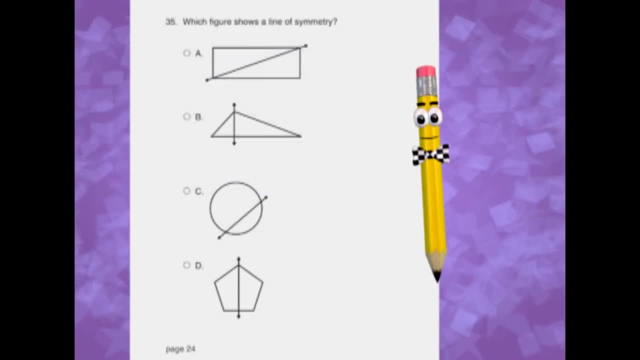 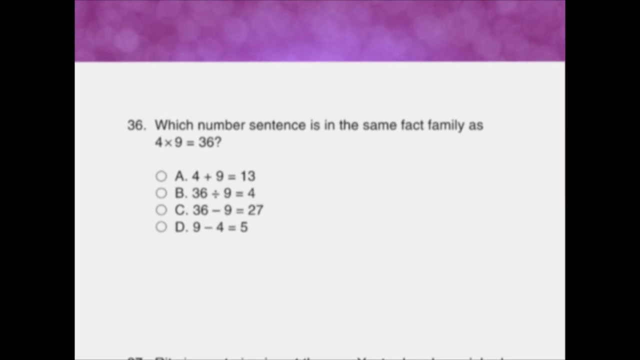 The only example of this in these pictures is D, The Pentagon, 36.. Which number sentence is in the same fact family as 4 times 9 equals 36? A: 4 plus 9 equals 13.. Addition cannot be in the same fact family as multiplication. 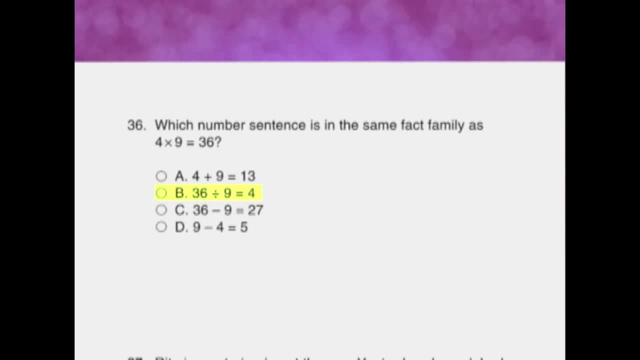 B: 36 divided by 9 equals 4.. This one is in the same fact family. Let's check the last two answers: C: 36 minus 9 equals 27.. Or D: 9 minus 4 equals 5.. 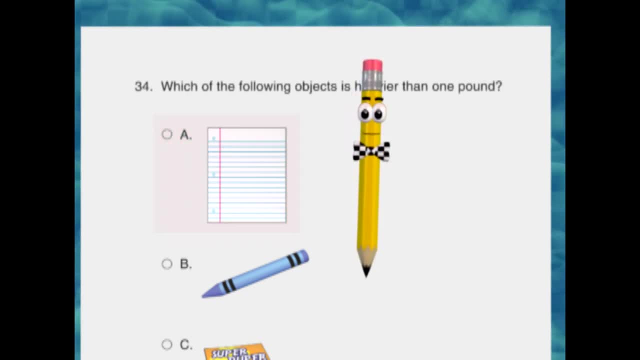 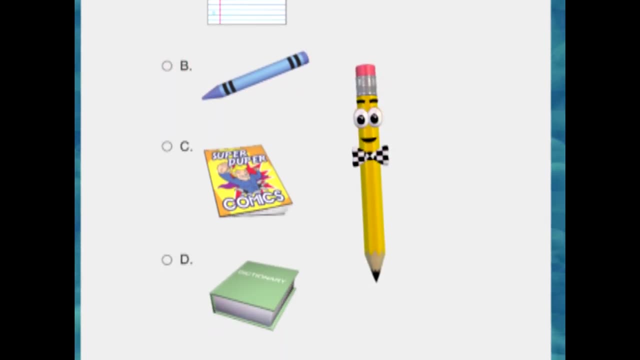 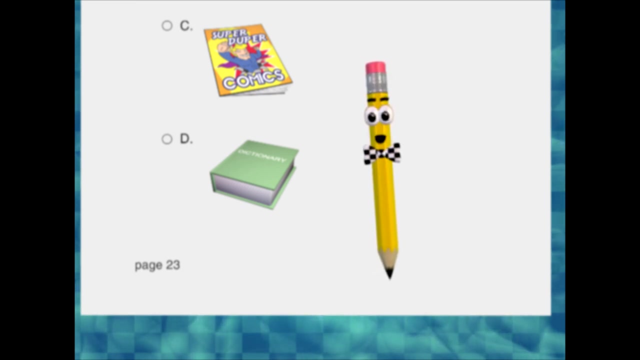 Now, a piece of paper is very light And a crayon is not very heavy either. A comic book might weigh a pound, But the last answer- A thick dictionary- would definitely weigh more than a pound. We'll mark answer D. Do you know what bird can lift the heaviest weight? 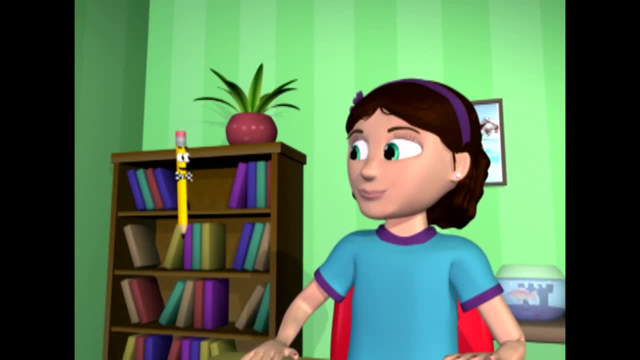 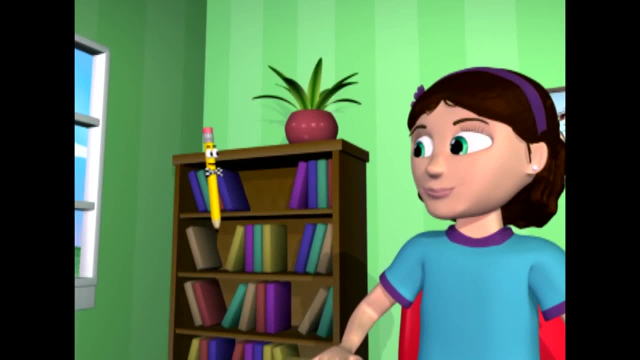 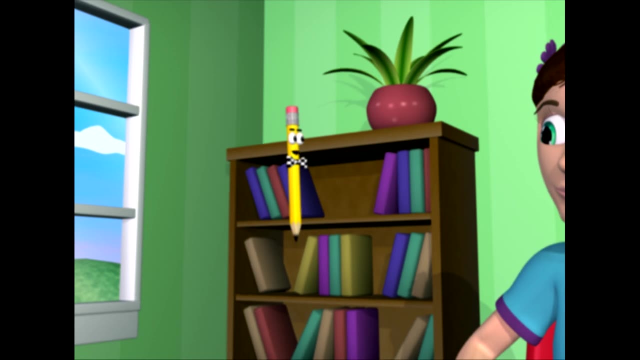 Which bird would that be? The crane? That was a good one. Did you know that math tests may have questions That require you to know the meanings of words used in math? Be sure you review the math terms and definitions that you have learned. Here are a few examples. 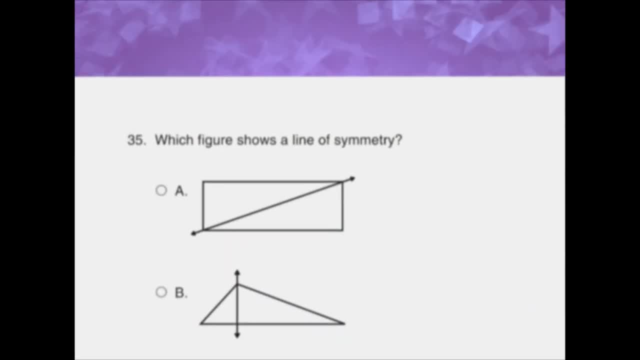 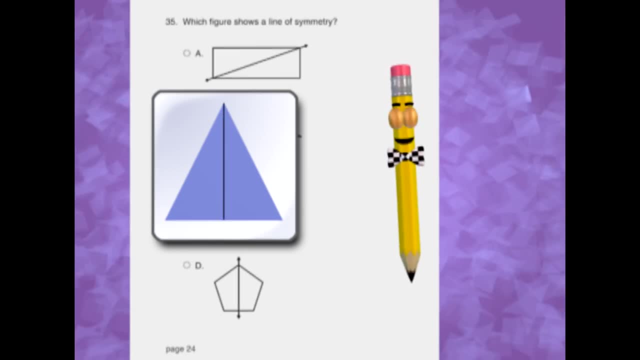 35, Which figure shows a line of symmetry. A line of symmetry divides a shape into two equal parts that are mirror images. If you were to fold a shape on a line of symmetry, The two halves would match up. The only example of this in these pictures is: 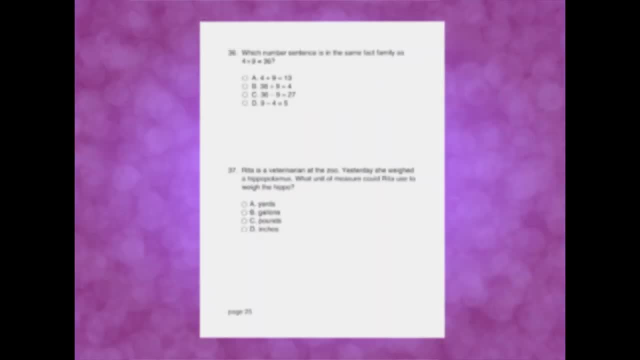 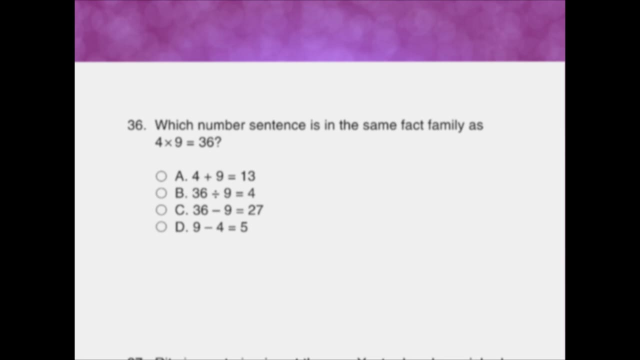 D, The Pentagon. 36. Which number sentence is in the same fact? family as 4 x 9 equals 36. 4 plus 9 equals 13. Addition cannot be in the same fact family as multiplication. 36 divided by 9 equals 4. This one is in the same fact family. 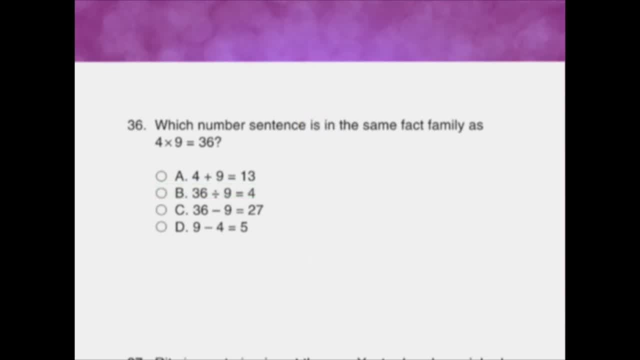 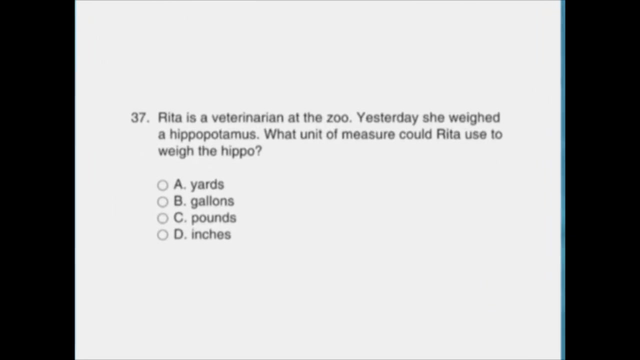 Let's check the last two answers: C 36 minus 9 equals 27. D 9 minus 4 equals 5. Subtraction cannot be in the fact family with multiplication. The correct answer is: B 36 divided by 9 equals 4 37. 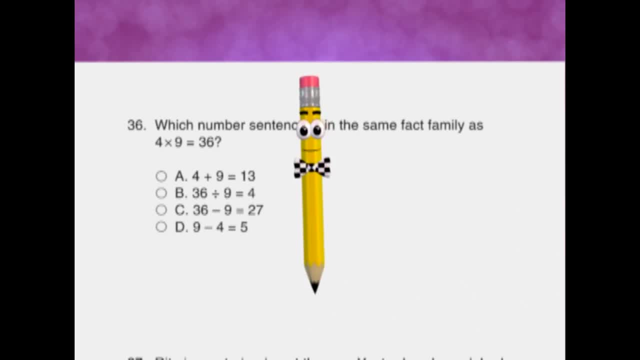 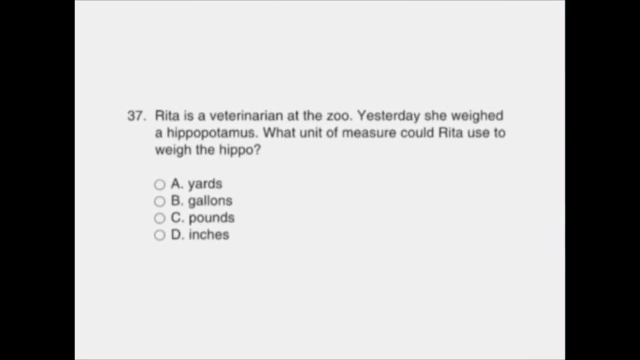 Subtraction cannot be in the fact family with multiplication. The correct answer is B 36 divided by 9 equals 4.. 37. Rita is a veterinarian at the zoo. Yesterday she weighed a hippopotamus. What unit of measure could Rita use to weigh the hippo? 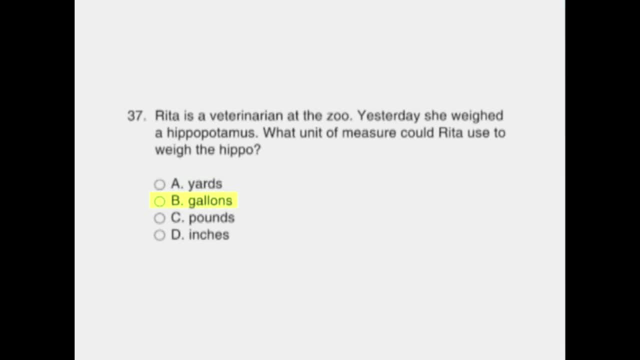 A Yards, B Gallons, C Pounds, D Inches. Let's see. Yards are used to measure length. Gallons are used to measure a volume of liquid. Pounds are used to measure weight or mass. So that could be it. 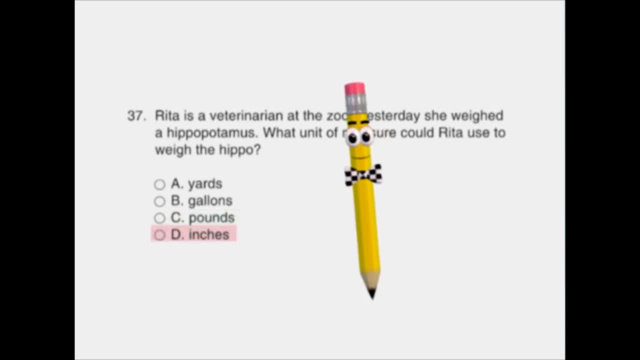 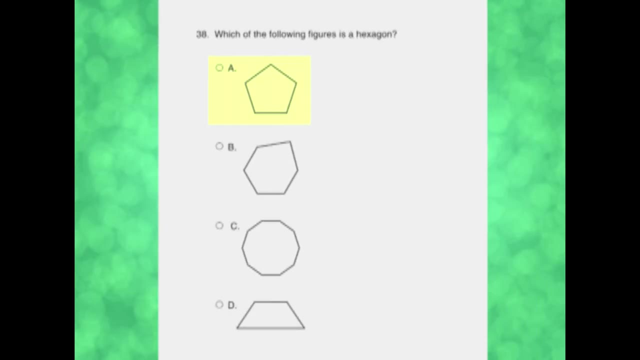 And inches are used to measure length, So the correct answer is C Pounds 38.. Which of the following figures is a hexagon? A shows a pentagon. C shows an octagon. D shows a trapezoid. 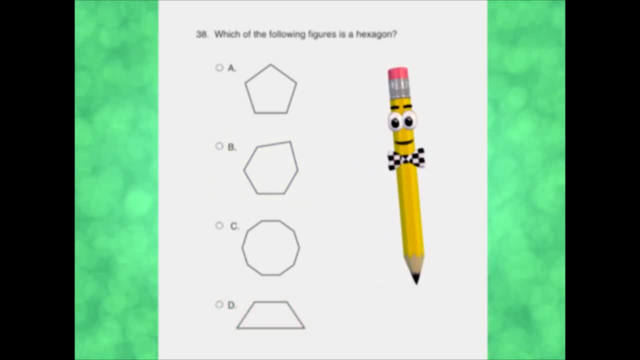 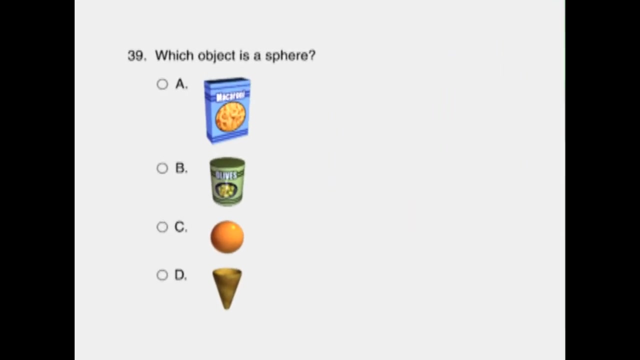 But look at B A hexagon has six sides: One, two, three, four, five, six. The answer is B 39.. Which object is a sphere? A shows a box, And a box is also called a rectangular prism. 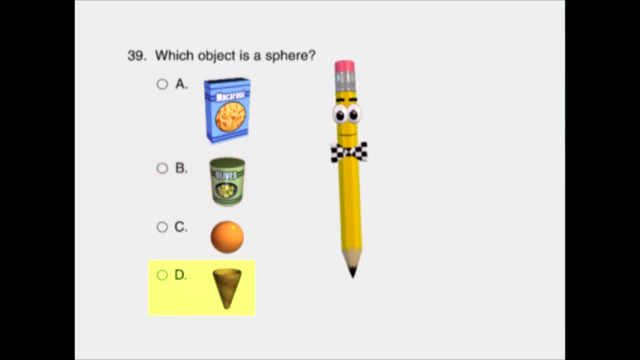 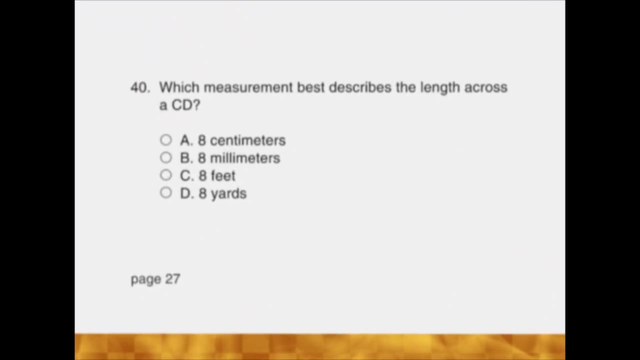 B is a cylinder, D is a cone, But C is a sphere. The answer is C. Now for the last question, 40.. Which measurement best describes the length across a CD? A, 8 centimeters, That sounds about right for a CD. 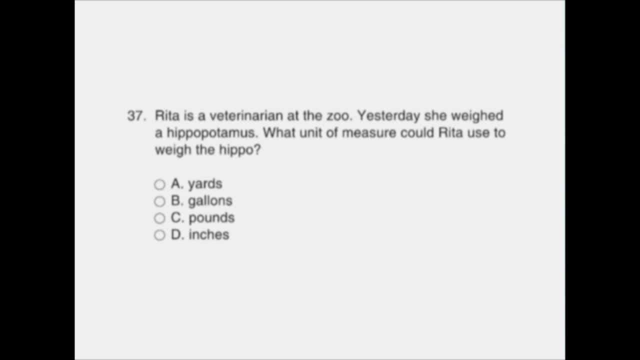 Rita is a veterinarian. at the zoo Yesterday she weighed a hippopotamus. What unit of measure could Rita use to weigh the hippo? A Yards, B Gallons, C Pounds, D Inches. Let's see. Yards are used to measure length. 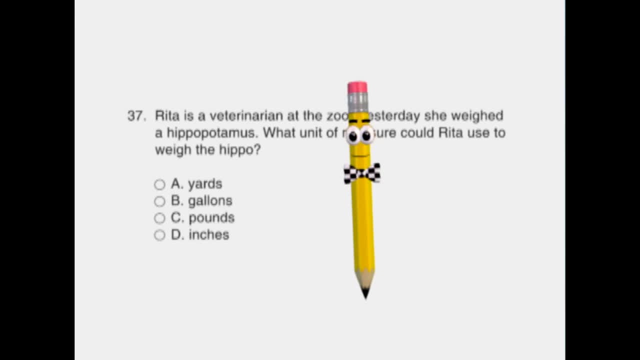 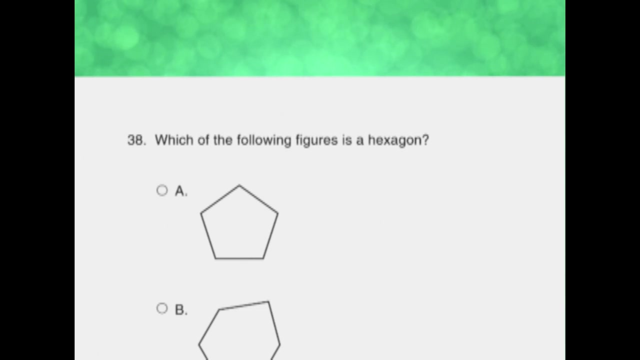 Gallons are used to measure a volume of liquid. Pounds are used to measure weight or mass, So that could be it. And inches are used to measure length, So the correct answer is C. Pounds 38. Which of the following figures is a hexagon? 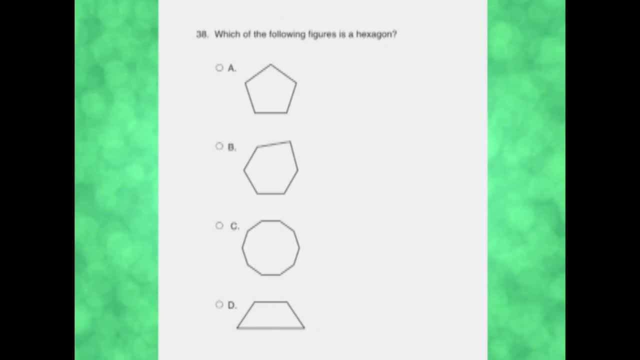 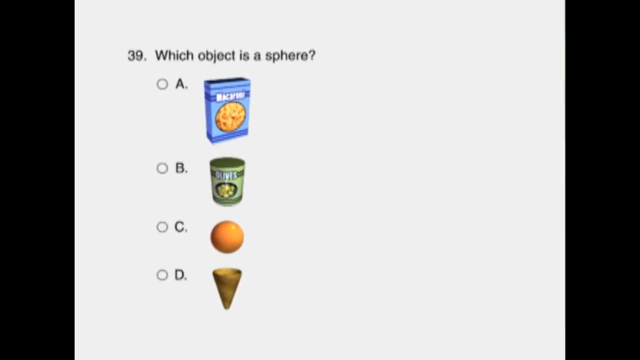 A shows a pentagon, C shows an octagon, D shows a trapezoid. But look at B. A hexagon has six sides: 1, 2, 3,, 4,, 5, 6. The answer is B 39. Which object is a sphere? 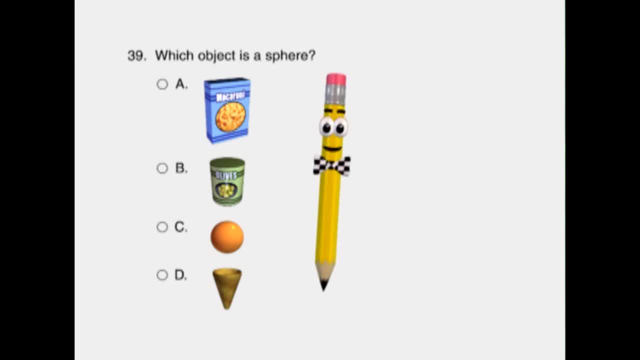 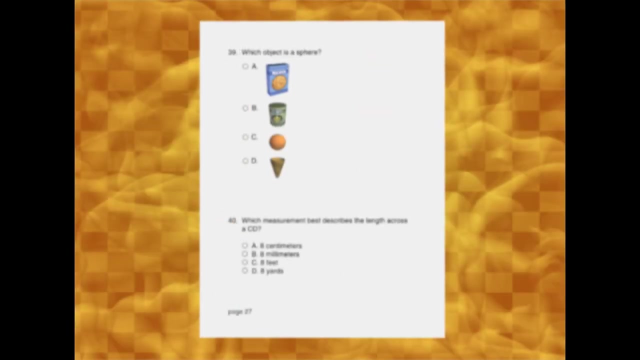 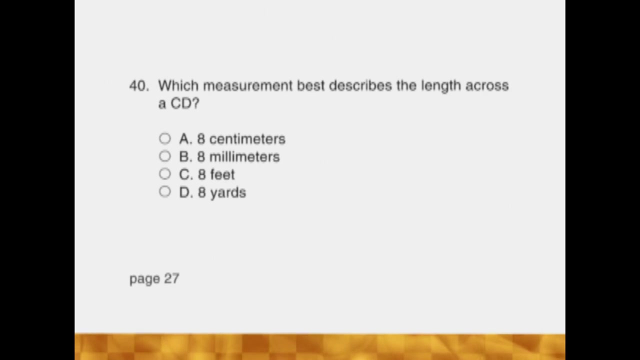 A shows a box, And a box is also called a rectangular prism. B is a cylinder, D is a cone, But C is a sphere. The answer is C. Now for the last question, 40: Which measurement best describes the length across a CD? A, 8 centimeters. 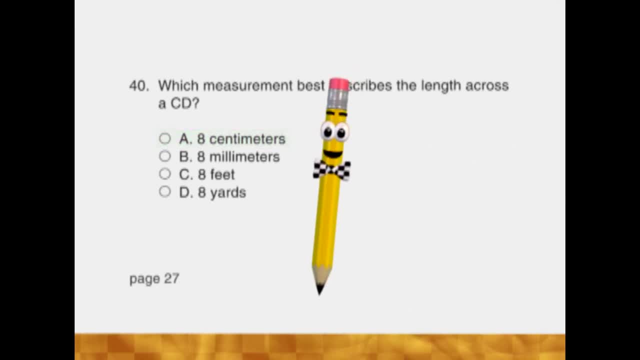 That sounds about right for a CD. Let's consider the other answers before we decide. B- 8 millimeters, That's not very much at all. 8 millimeters might not even be the width of your finger. C- 8 feet- This is wider than a car. 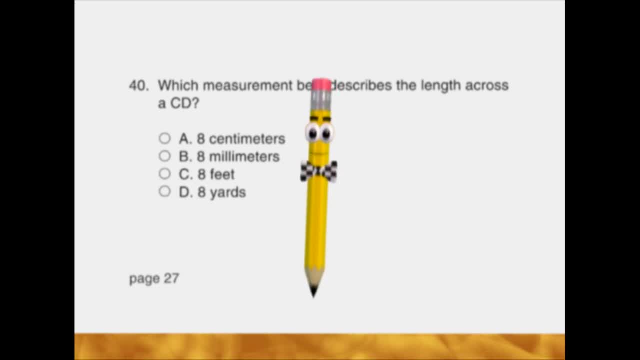 Let's consider the other answers before we decide. B- 8 millimeters- That's not very much at all. 8 millimeters might not even be the width of your finger. C- 8 feet- This is wider than a car. D- 8 yards. 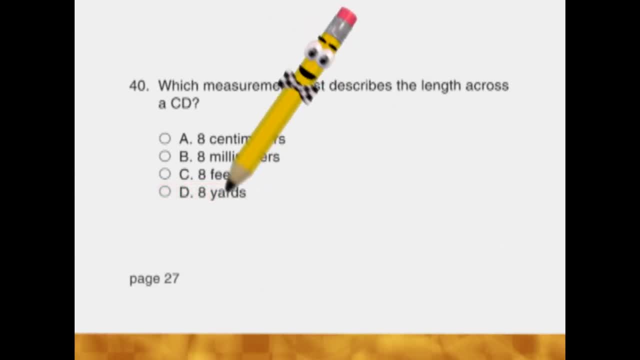 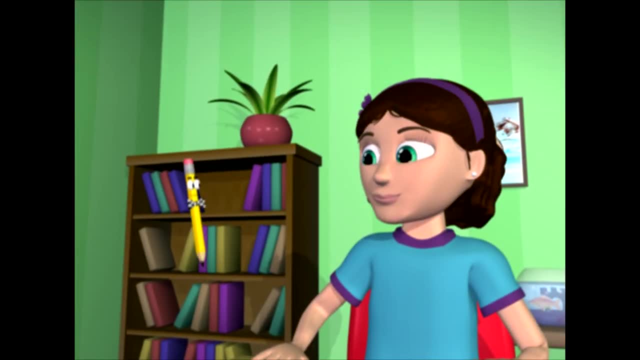 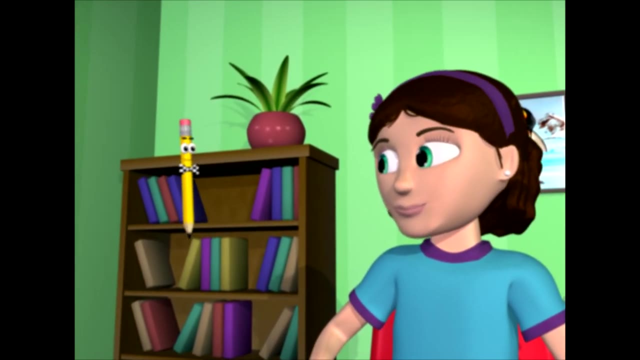 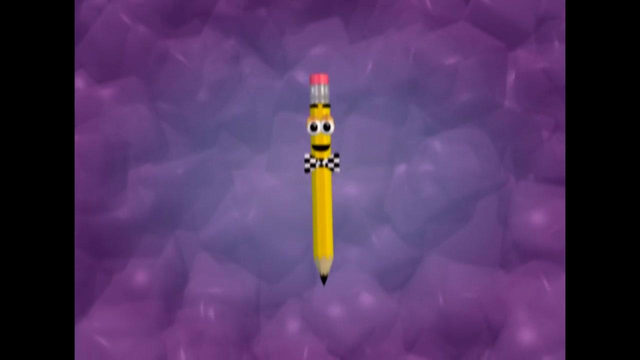 Way too much. The answer is A 8 centimeters. Wow, Marco, we did it. I'm really glad that you led the way. Led, Oh, I get it Very funny. And now that we've been through some sample questions, 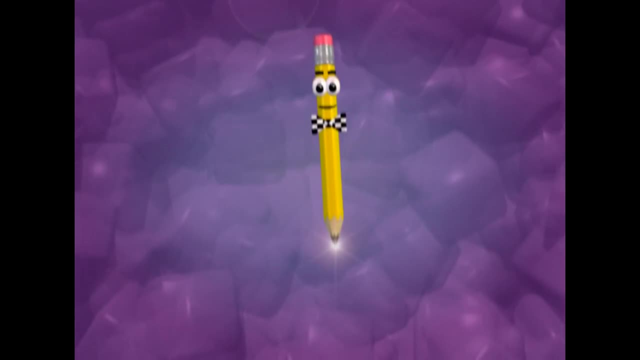 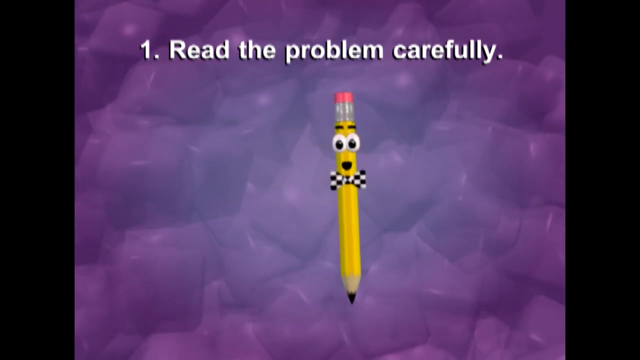 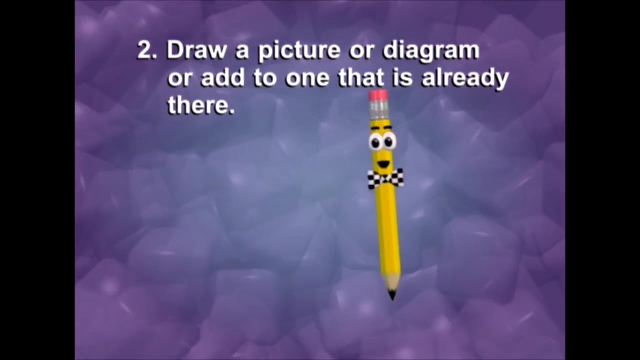 I want to remind you of the tips we learned for taking math tests. Read the problem carefully, Draw a picture or diagram, or add to one that is already there, But remember not to write on a test without permission. You might be able to use a piece of scratch paper if you are not allowed to write on the test. 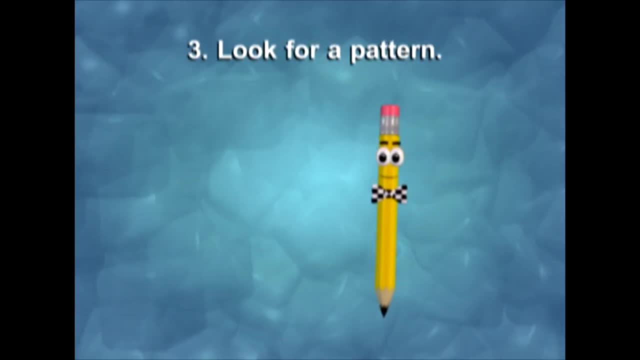 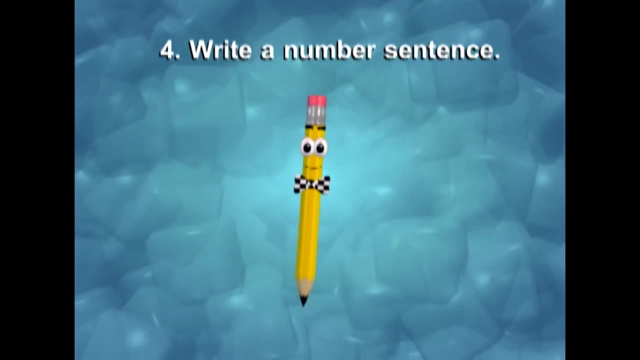 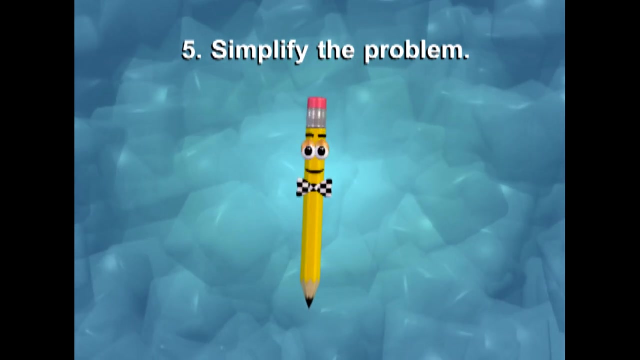 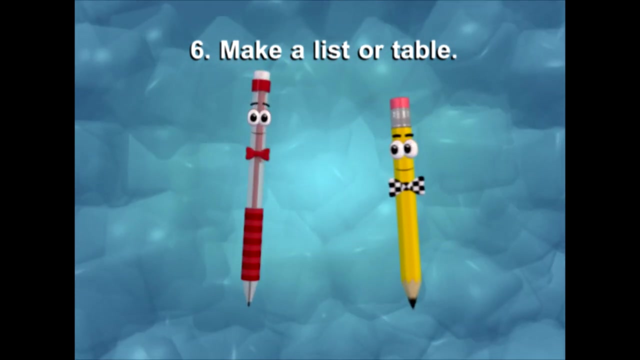 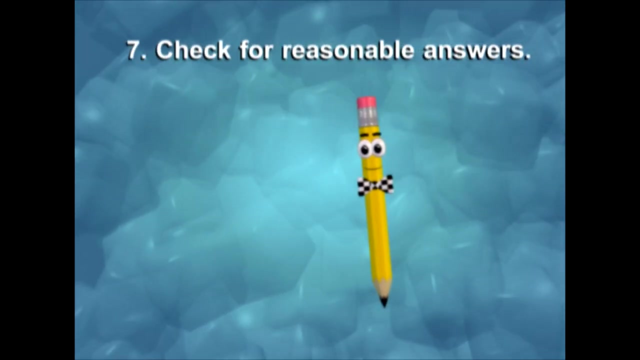 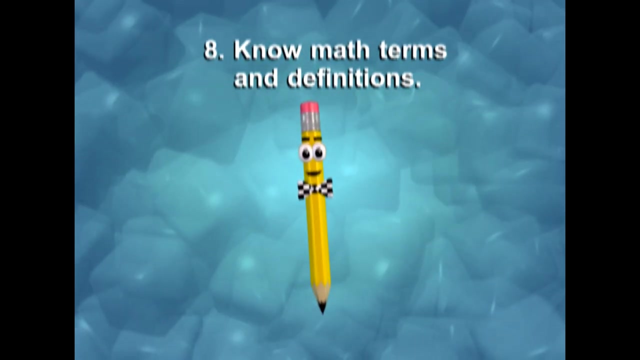 You're right. Look for a pattern. Write a number sentence. Simplify the problem. Make a list or table. Remember: only write on your test if your teacher says it's OK. Check your answers to see if they are reasonable. Know your math terms and definitions. 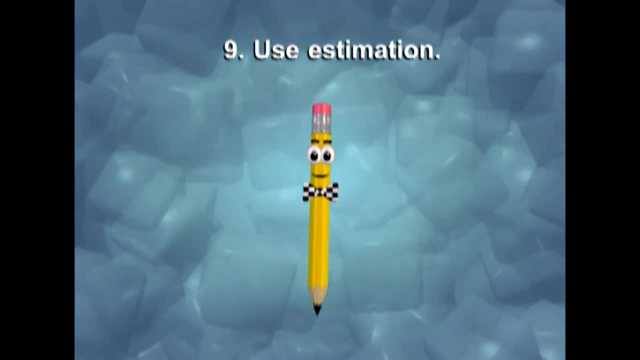 Estimation is a real-life skill that pays off when it comes to tests. Sometimes students have trouble with estimation skills because they want to be 100% accurate, But remember that when a test fails, remember that when a test question asks for an estimate. 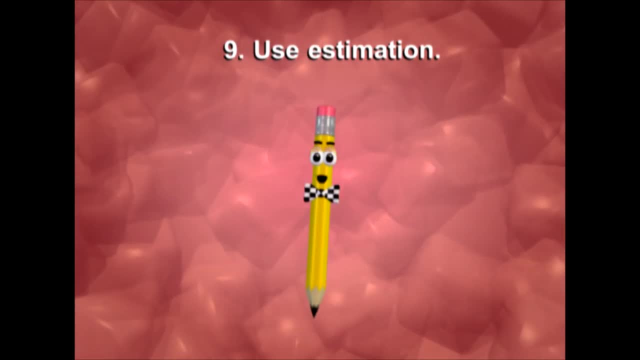 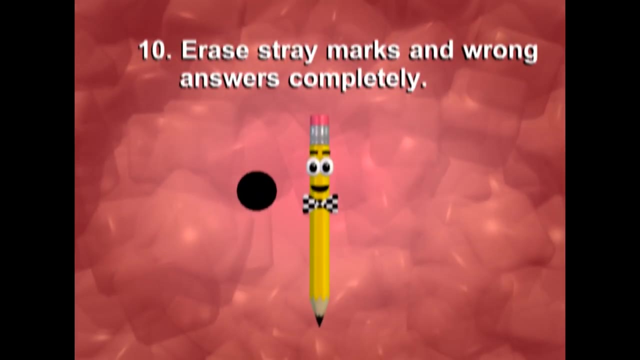 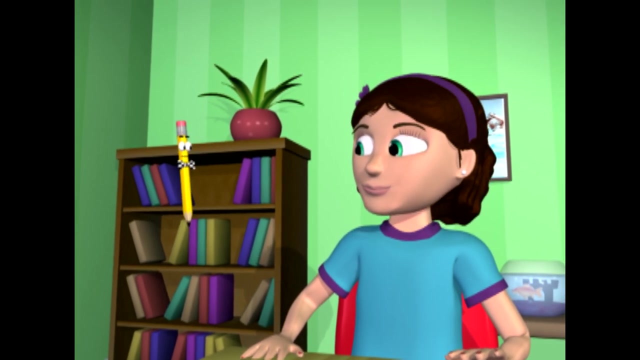 you only need to give an approximate value. You know something that's in the ballpark And, last but not least, be sure to erase any stray marks or wrong answers completely. Our time went by really fast, Marco. Yes, yes, And do you know why I am always so fast? 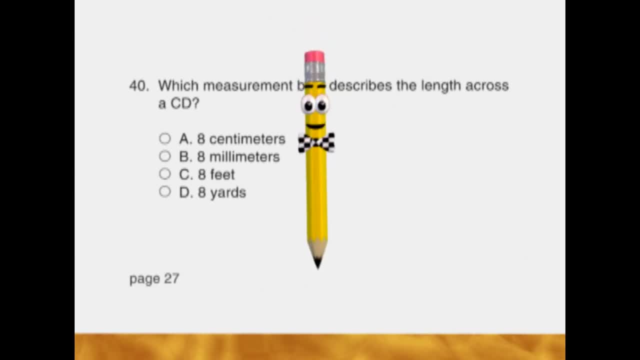 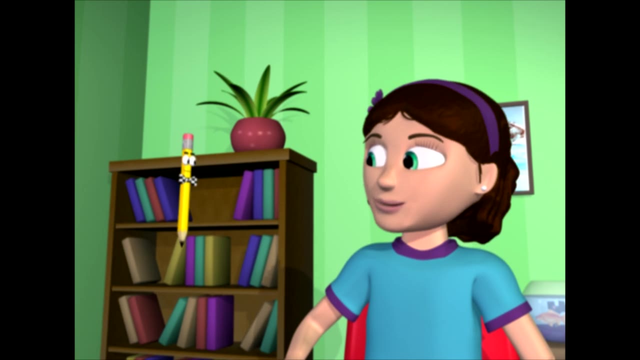 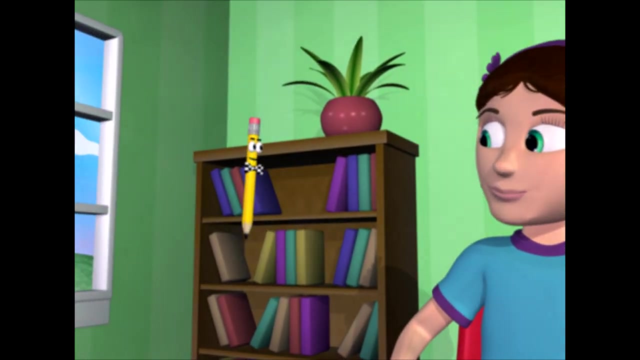 D- 8 yards- Way too much. The answer is A- 8 centimeters. Wow, Marco, We did it. I'm really glad that you led the way. Led, Oh, I get it Very funny. And now that we've been through some sample questions, 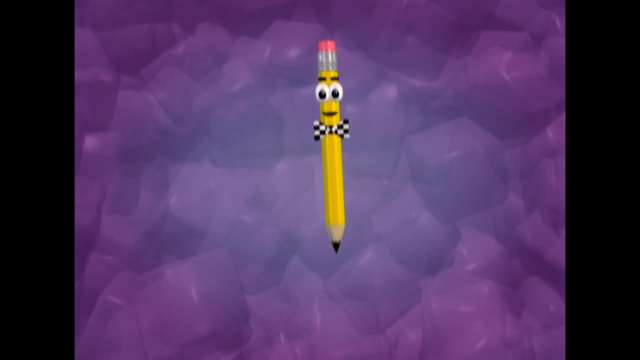 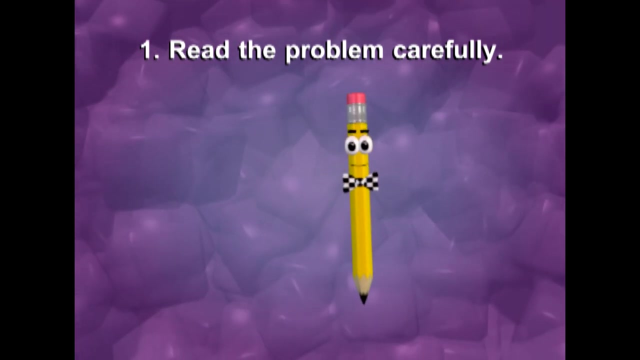 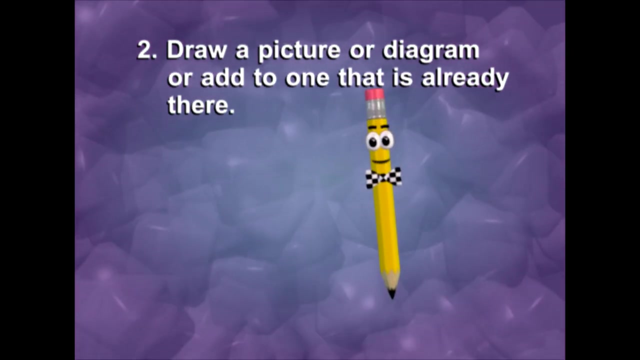 I want to remind you of the tips we learned for taking math tests. Read the problem carefully, Draw a picture or diagram, Or add to one that is already there, But remember not to write on a test without permission. You might be able to use a piece of scratch paper. 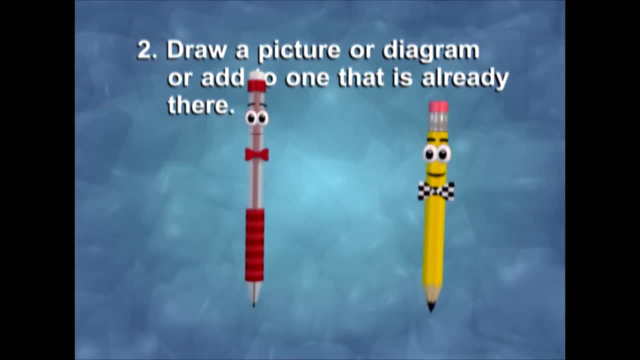 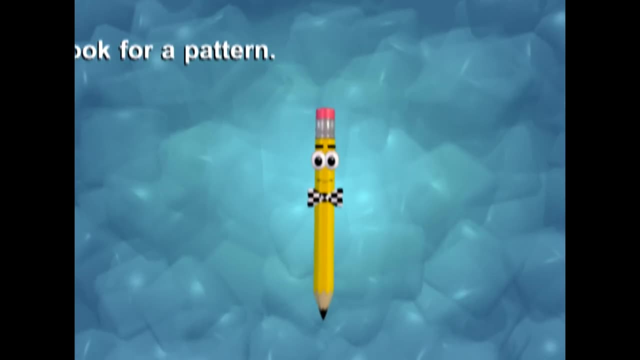 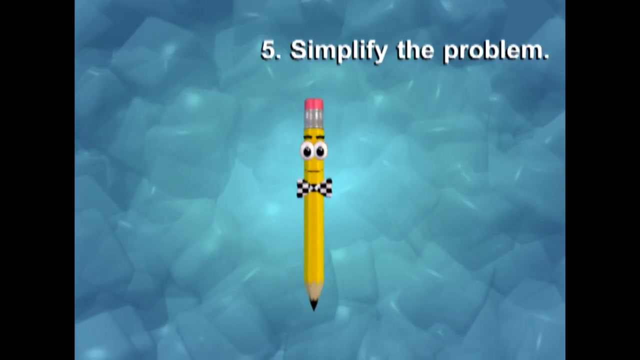 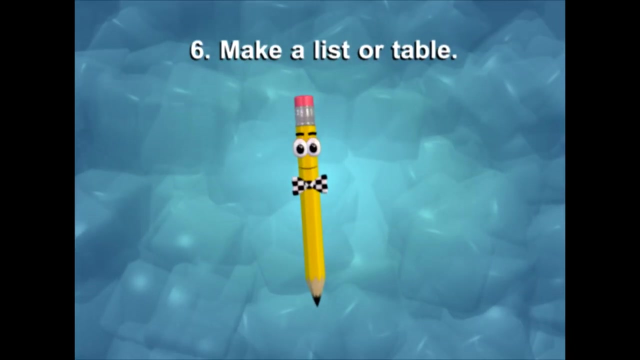 if you are not allowed to write on the test, You're right. Look for a pattern. Write a number sentence. Simplify the problem. Make a list or table. Remember: only write on your test if your teacher says it's OK. Check your answers to see if they are reasonable. 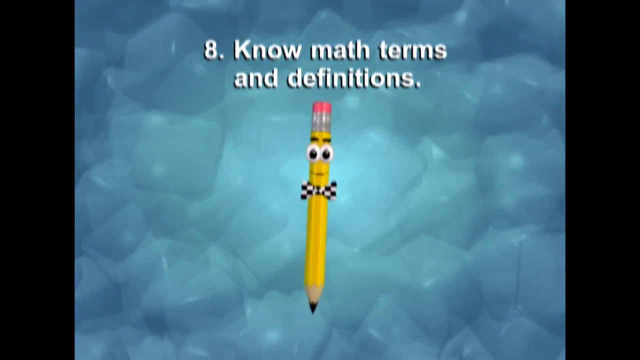 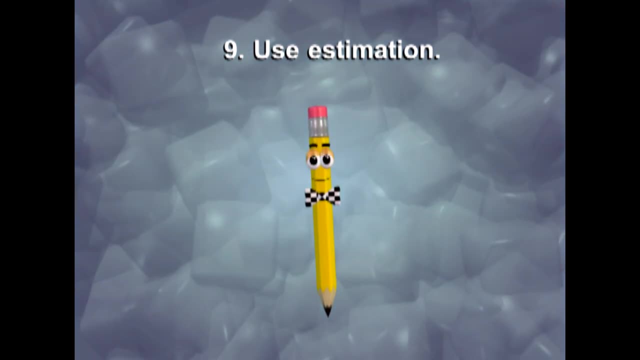 Know your math terms and definitions. Estimation is a real life skill that pays off when it comes to tests. Sometimes students have trouble with estimation skills because they want to be 100% accurate. But remember that when a test question asks for an estimate, you only need to give an approximate value. 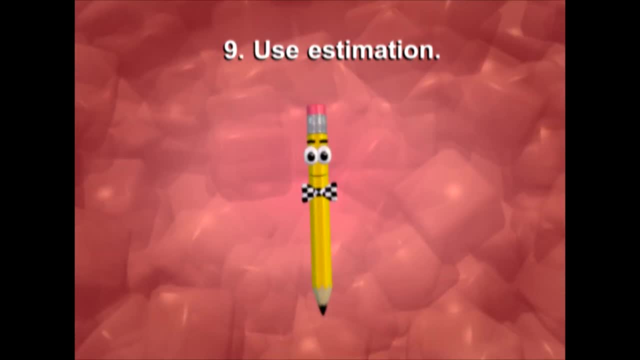 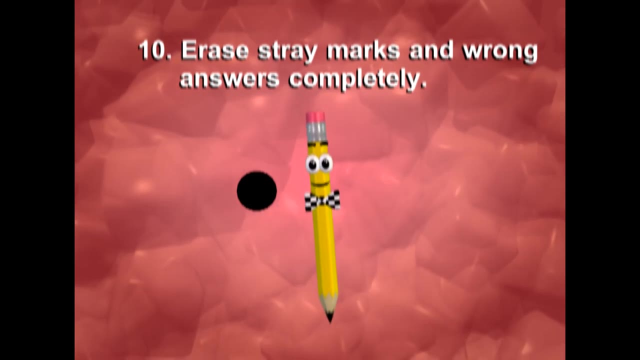 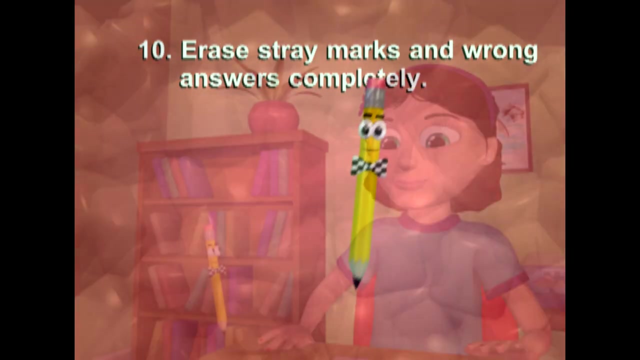 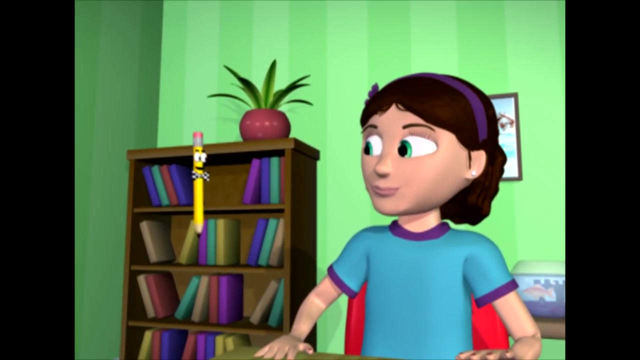 You know something that's in the ballpark? And, last but not least, be sure to erase any stray marks or wrong answers completely. Our time went by really fast, Marco. Yes, yes, And do you know why I am always so fast? No, why. 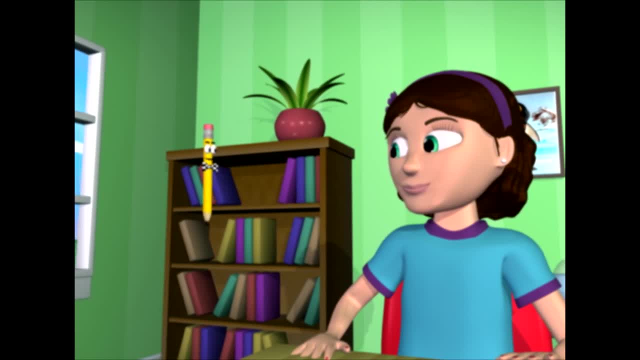 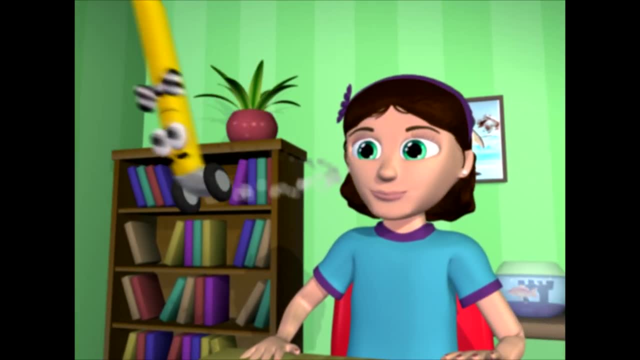 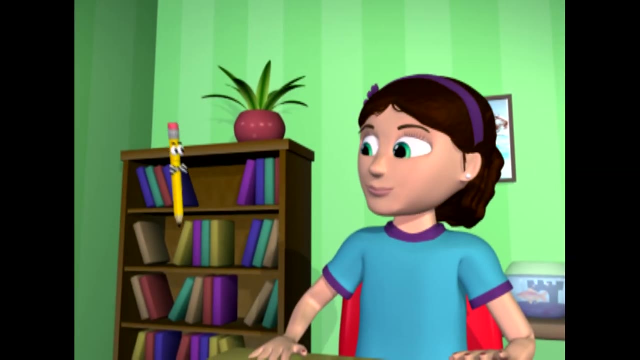 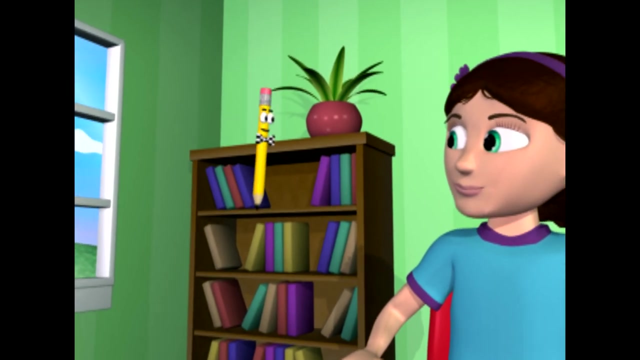 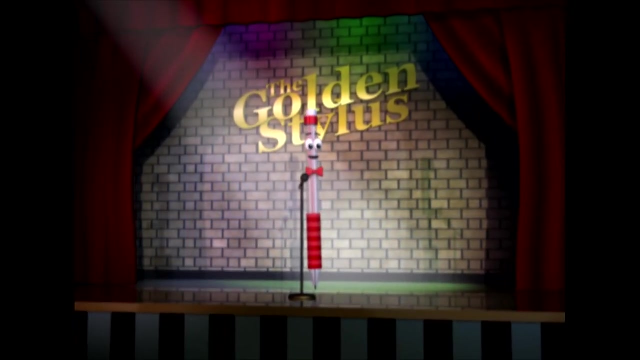 No, Why? Because everywhere I go I have my eraser. So, Marco, what do you do when you're not helping kids learn how to do better on tests? Well, let's just say I have a little night job. Ladies and gentlepins, Mike Mechanical here. 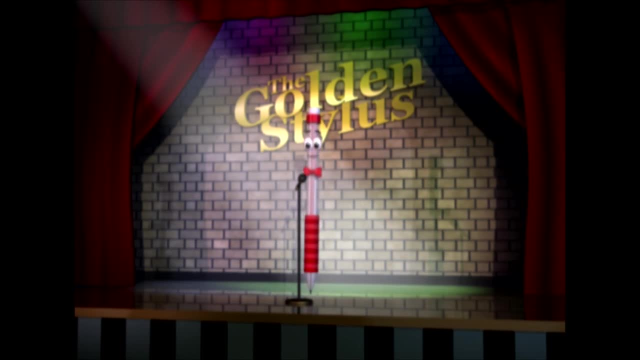 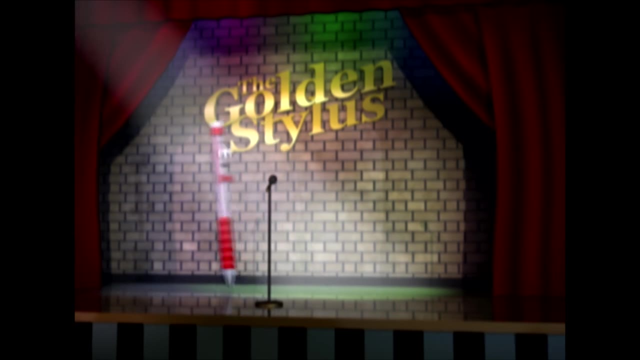 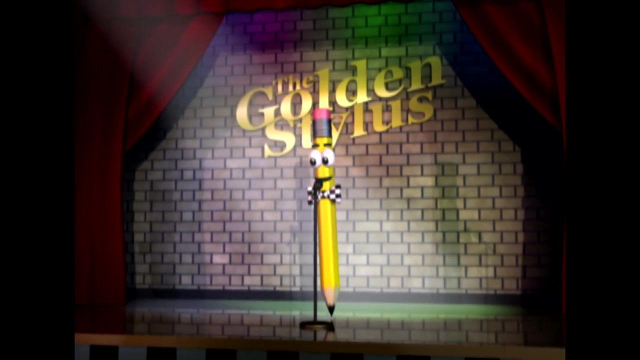 and we're in for a special treat tonight at the Golden Stylus Comedy Room, All the way from Pennsylvania. can you please welcome the king of one-liners, Marco the Pencil. Hey there everyone. Oh my my, It's so great to be back at the Golden Stylus. 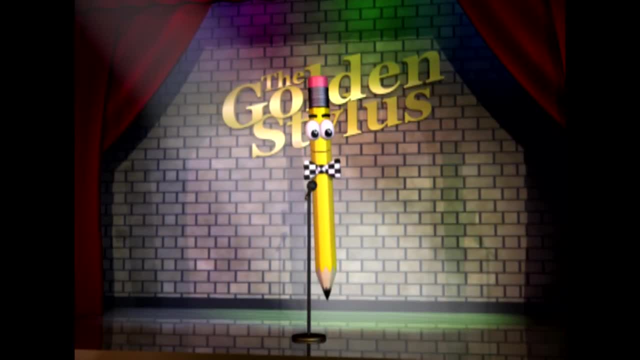 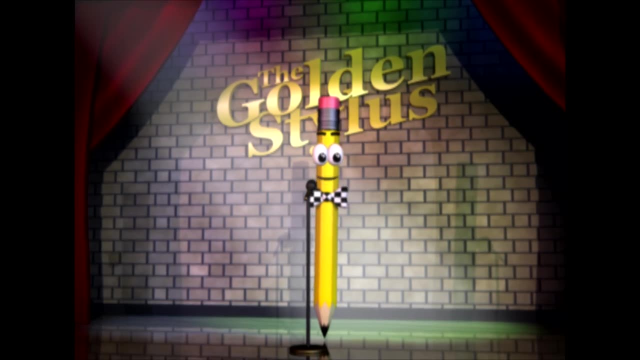 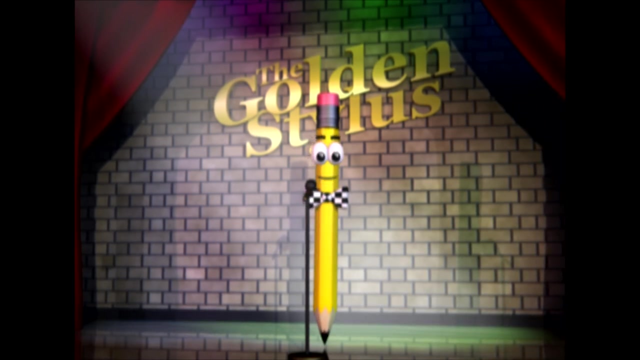 I'm feeling really sharp tonight. Say sir, Yeah, the pencil in the front row. You're looking a bit chewed on. Do yourself a favor and try to stay away from those mouths, okay? Why did the boy's mother buy him three socks? 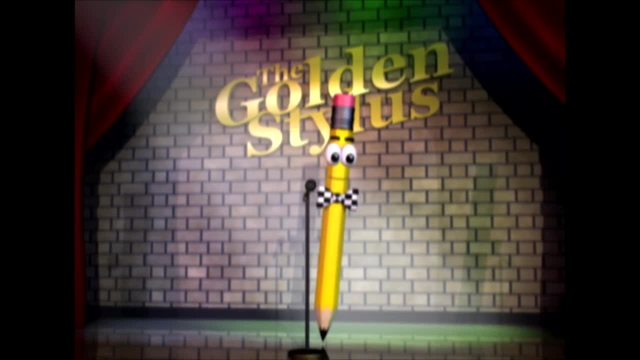 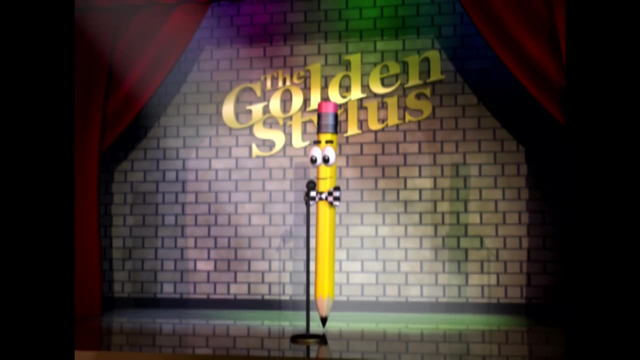 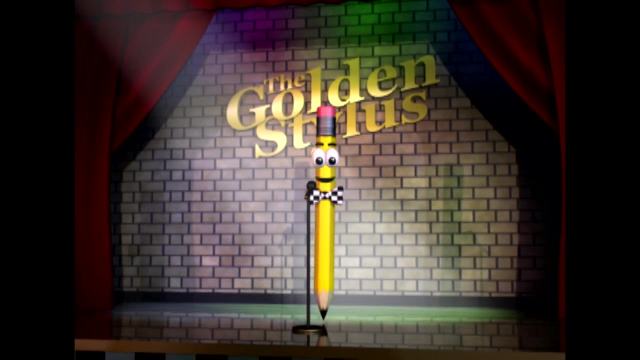 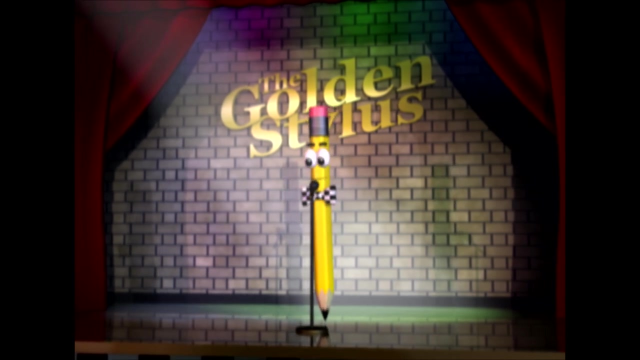 Because he said he grew another foot. What has three feet but can't walk? A yardstick? What table has no legs? A times table? What has two hands but can't carry anything? A clock? Did you hear the joke about the brand new pencil? 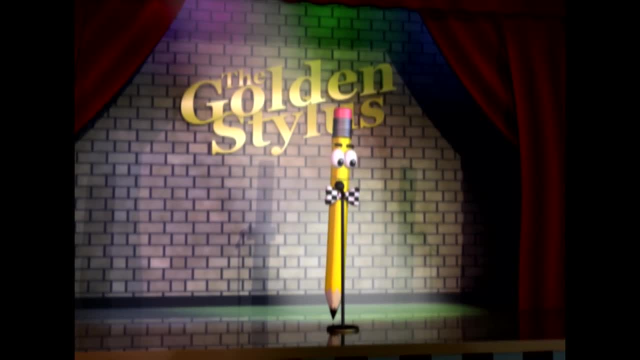 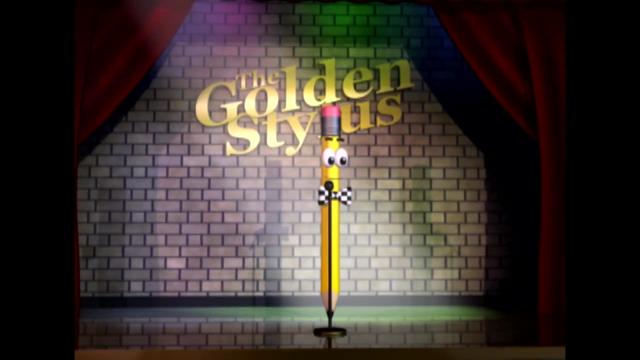 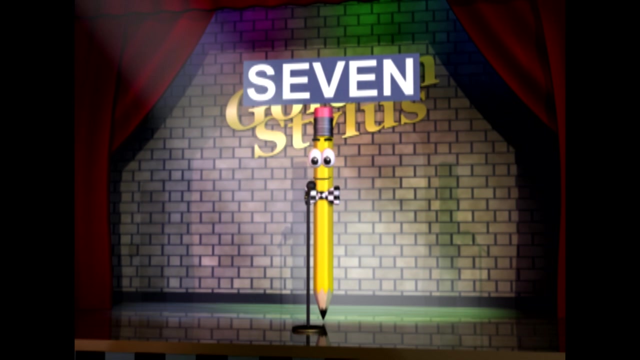 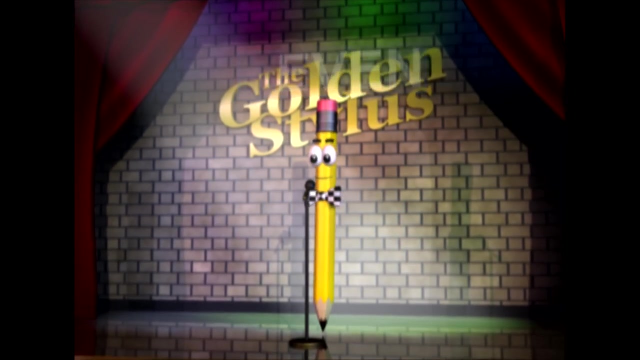 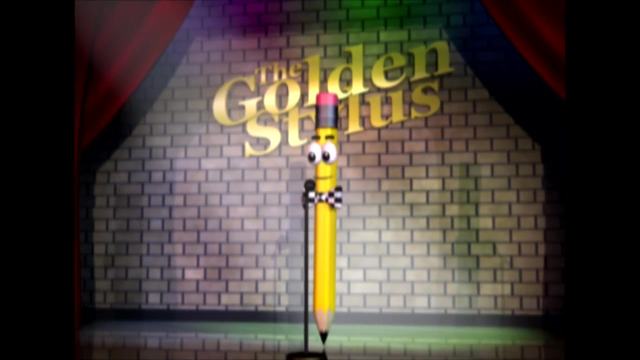 No, it's pointless. What did the zero say to the eight? Nice belt. How can you make seven? even Remove the S. You see Why is the pencil the heaviest thing in your backpack? Because it's full of lead. 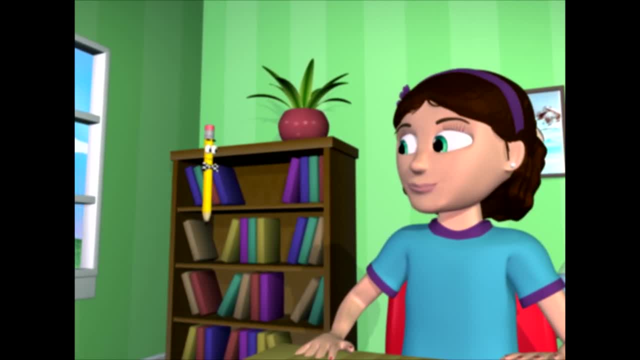 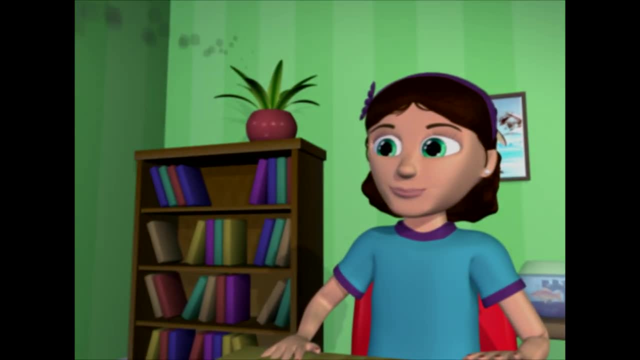 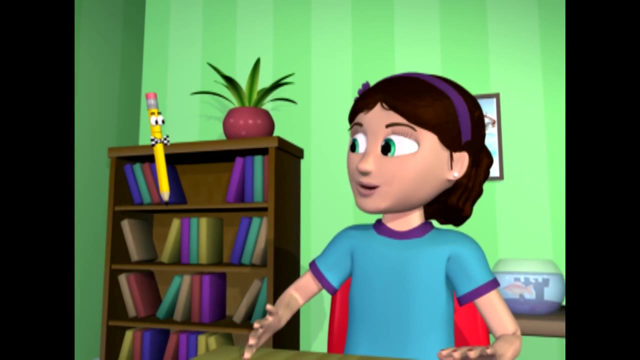 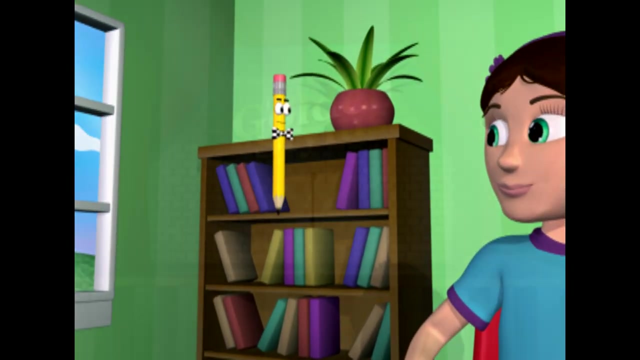 Because everywhere I go I have my eraser. No, So, Marco, what do you do when you're not helping kids learn how to do better on tests? Well, let's just say I have a little night job. Ladies and gentlemen, Mike Mechanical here. 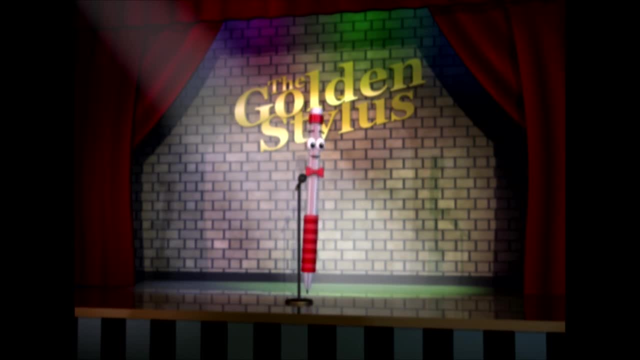 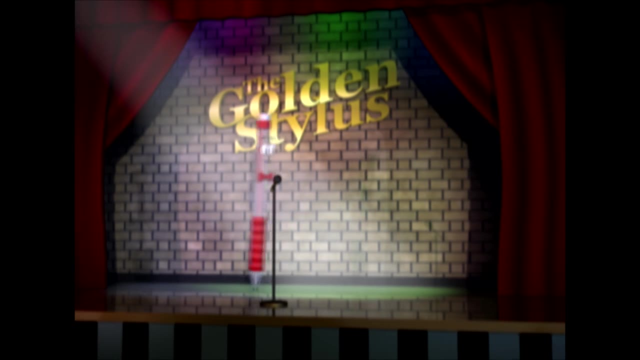 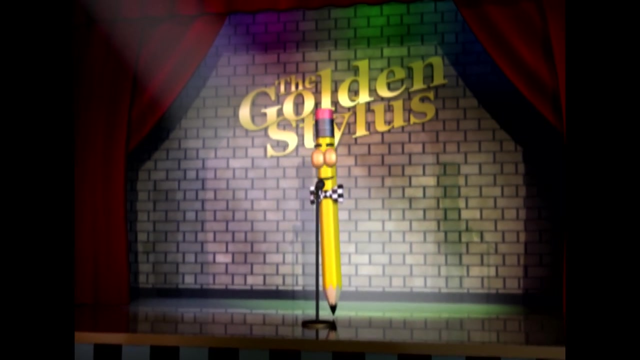 And we're in for a special treat tonight at the Golden Stylus Comedy Room, All the way from Pennsylvania. Will you please welcome the king of one-liners, Marco the Pencil. Marco the Pencil, Hey there everyone. Oh my, my. 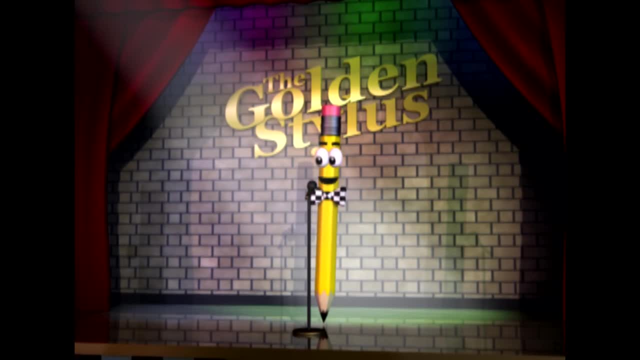 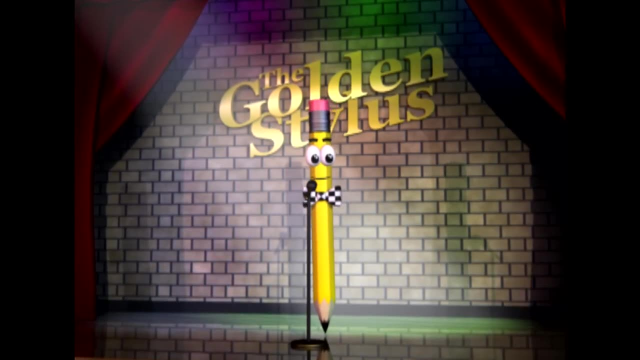 It's so great to be back at the Golden Stylus. I'm feeling really sharp tonight. Say, sir, Yeah, the pencil in the front row. You're looking a bit chewed on. Do yourself a favor and try to stay away from those mouths, okay. 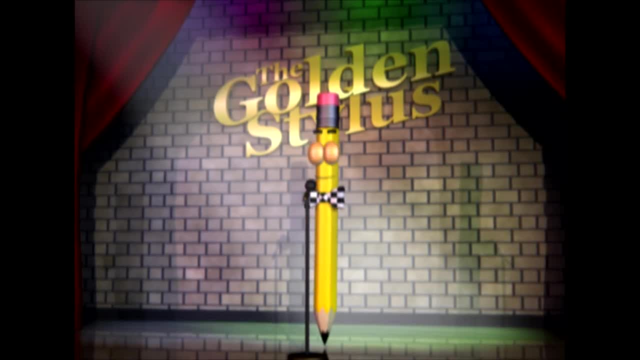 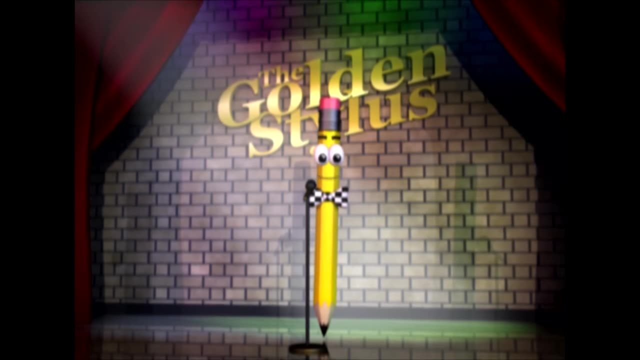 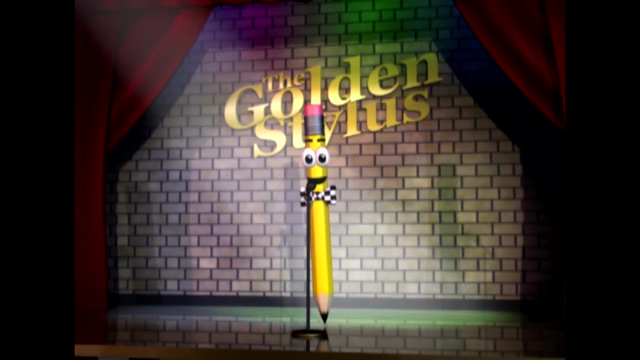 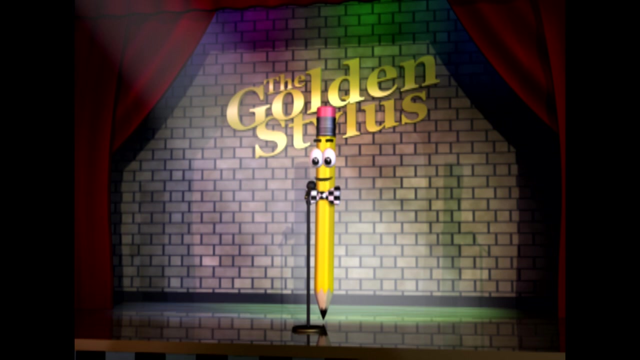 Why did the boy's mother buy him three socks Because he said he grew another foot? What has three feet but can't walk? A yardstick? What table has no legs? A times table? What has two hands but can't carry anything? 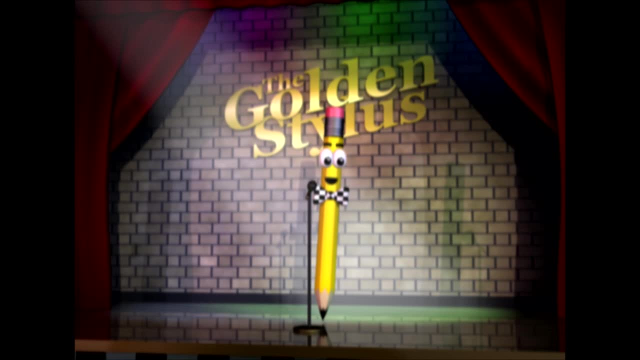 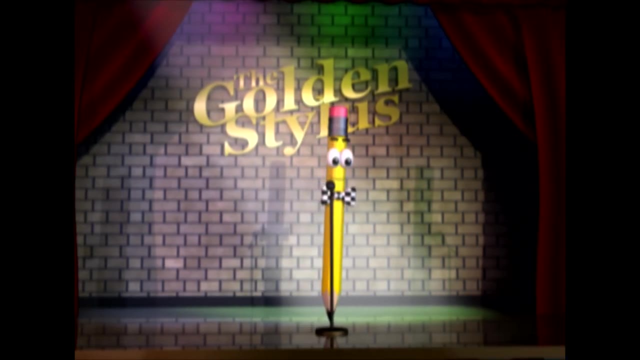 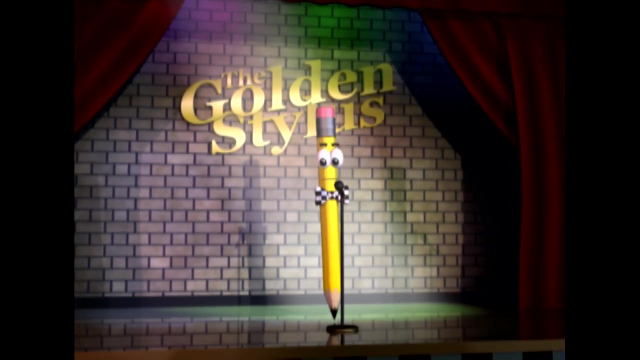 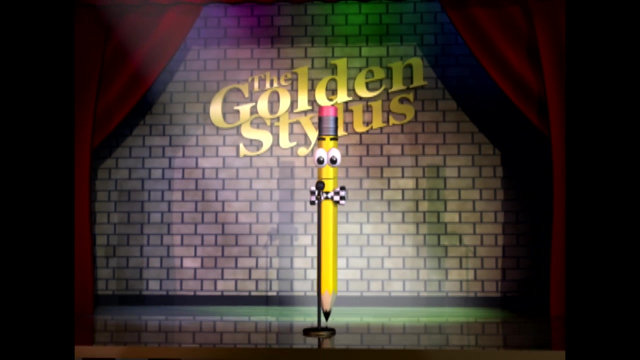 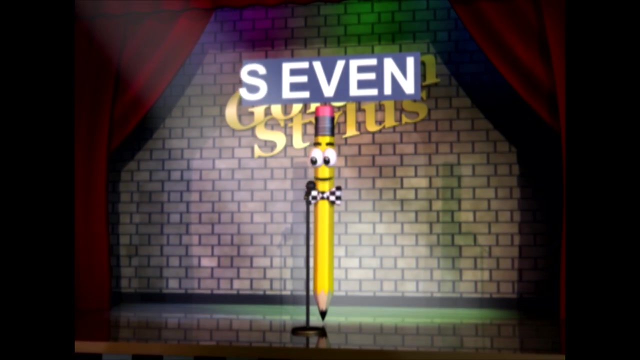 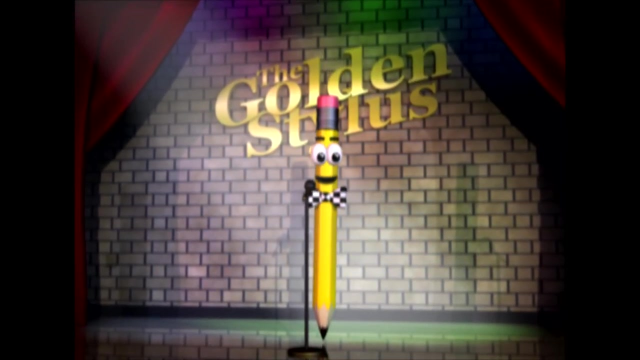 A clock. Did you hear the joke about the brand new pencil? No, it's pointless. What did the zero say to the eight Nice belt? How can you make seven? even Remove the S. You see Why is the pencil the heaviest thing in your backpack.